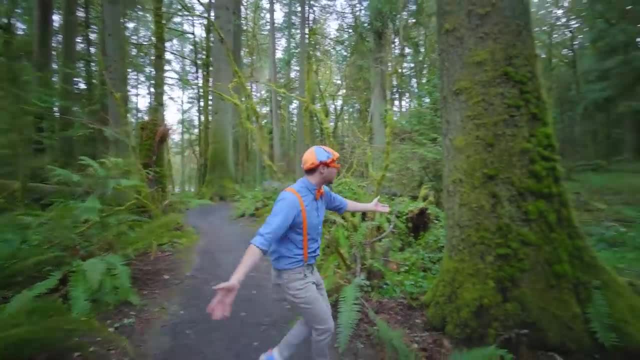 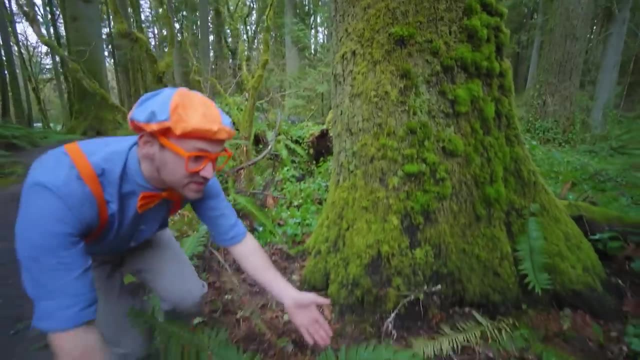 in Olympia, Washington, Whoa, and look at this place. Wow, there's some moss on this giant tree. Oh, look, here's some shrubs. Yeah, this is actually a fern. Wow, and this is a big tree. Wow, and this is a big tree. Wow, and this is a big tree. Wow, and this. 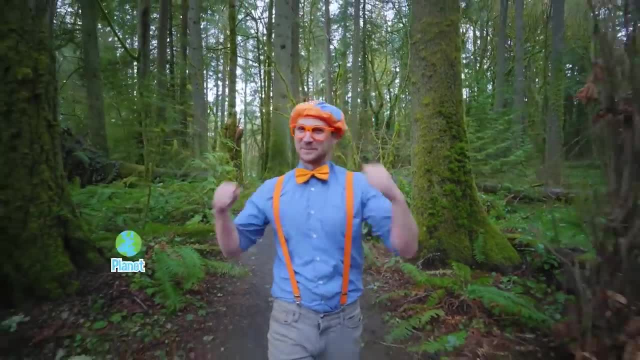 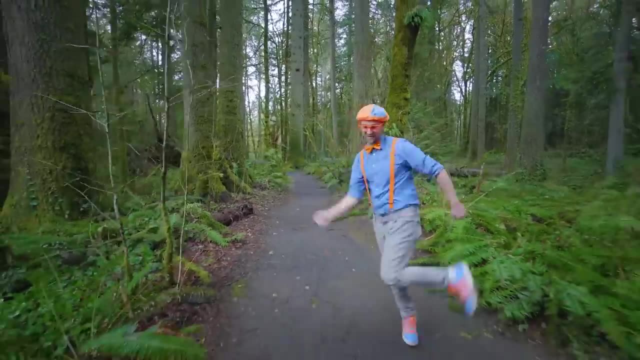 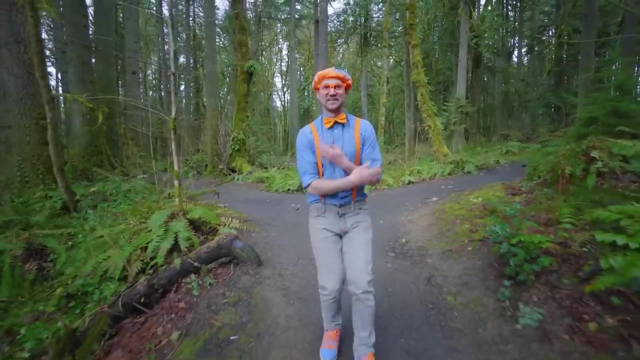 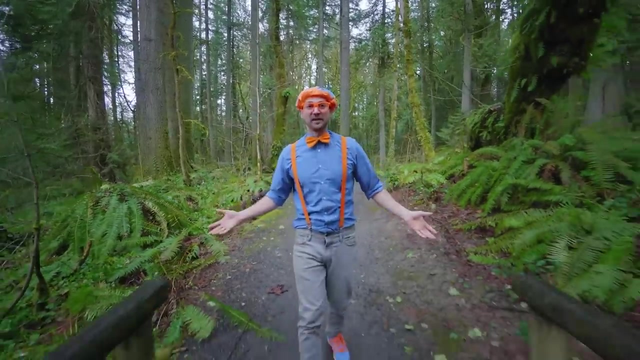 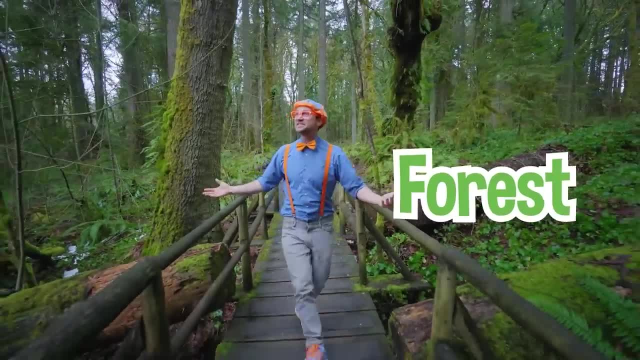 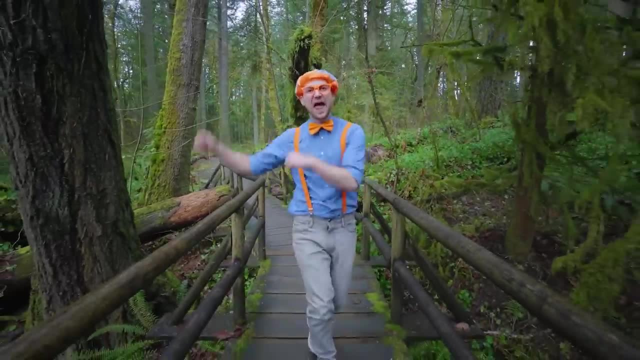 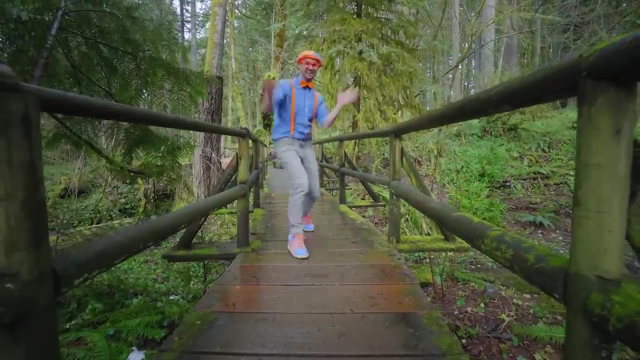 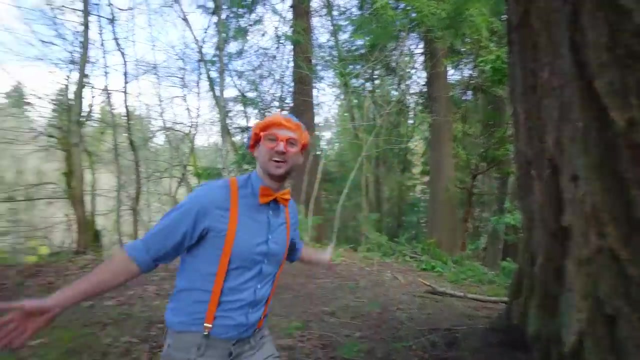 a rainy forest Forest. Wow, this is so cool. Oh, it's really pouring now. Makes me so happy. Woo, Oh, ho, ho, ho, ho, Oh, jeez, I love being in nature. Wow, it's such a great place to be. 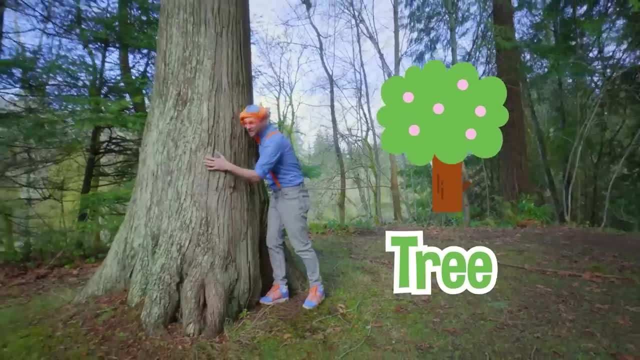 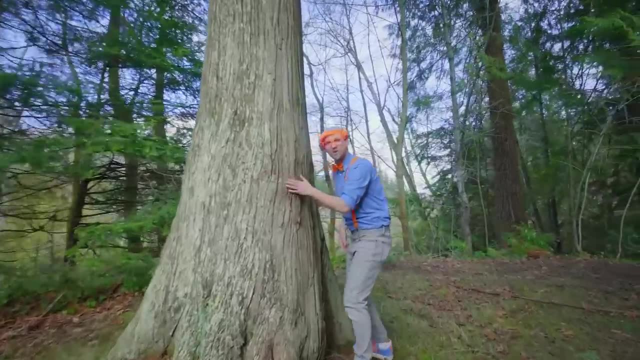 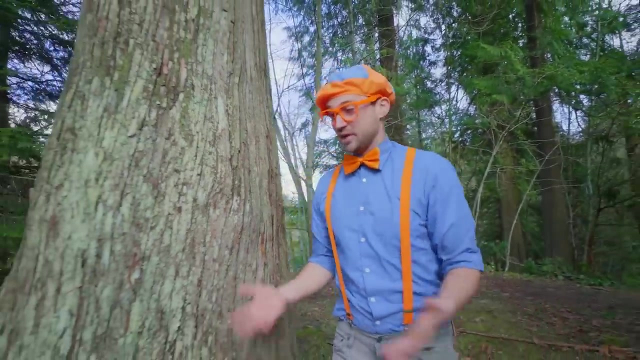 Whoa, look at this massive tree. Whoa, its bark feels so cool on my hands. Whoa, it's so textured. Whoa, that's really cool. Wow, I love plants, Trees, shrubs, flowers, yeah. 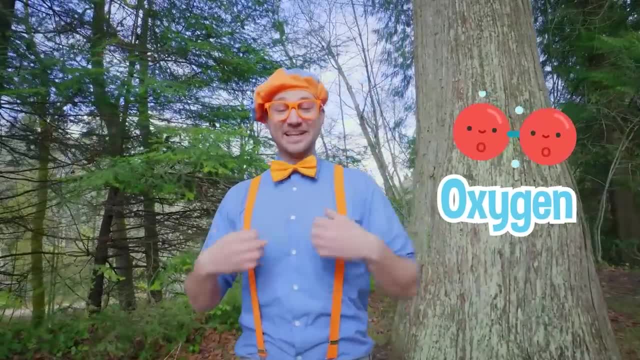 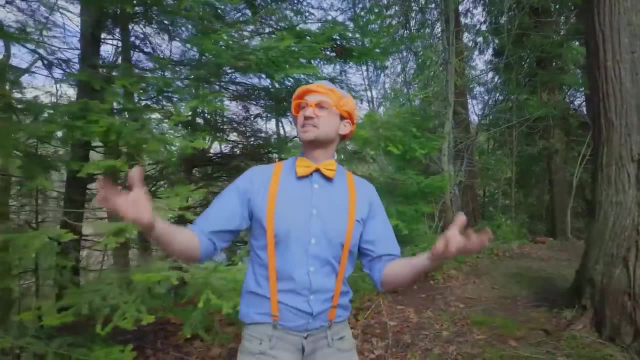 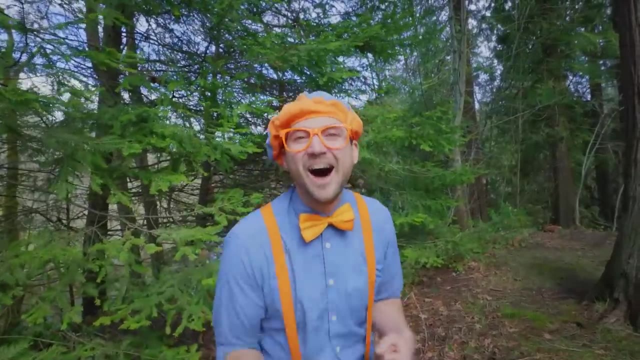 There's so many great plants- because they provide us oxygen, Yeah, and other things like vegetables, fruit. But it's not all about us enjoying nature. We need to give back as well. Yeah, have you ever planted a plant before? Yeah, it is so much fun. 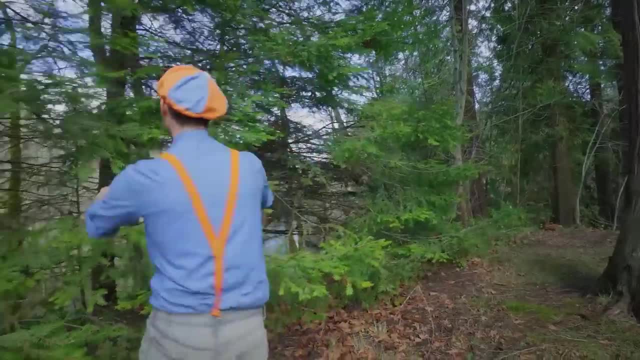 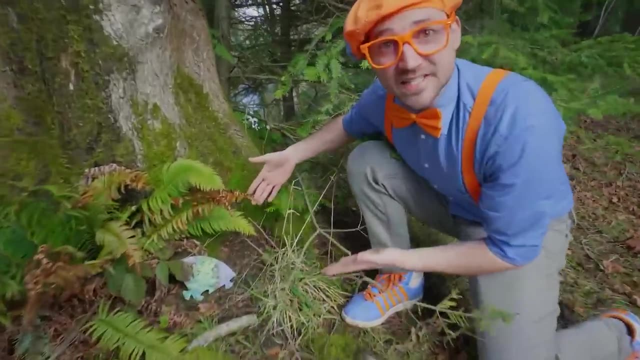 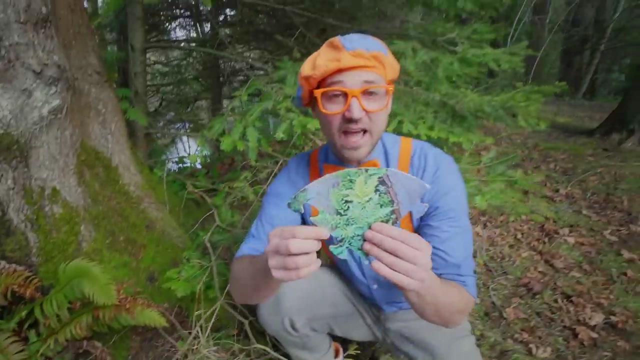 Digging in the dirt, planting the plant, watching it grow. Whoa, oh, What is this? Do you see what I see? Yeah, this is a puzzle piece. Whoa, check it out. I love puzzles. Huh, look at it. 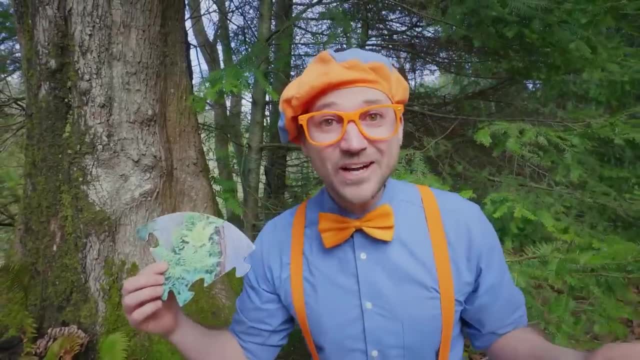 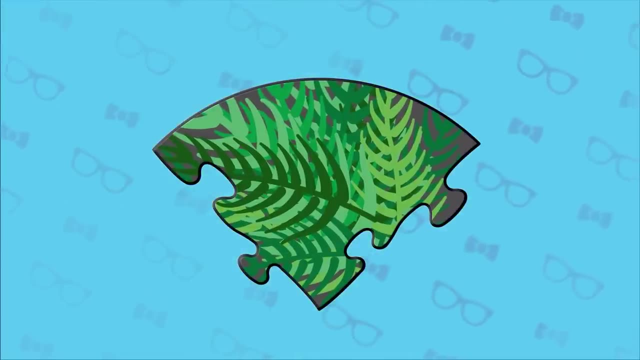 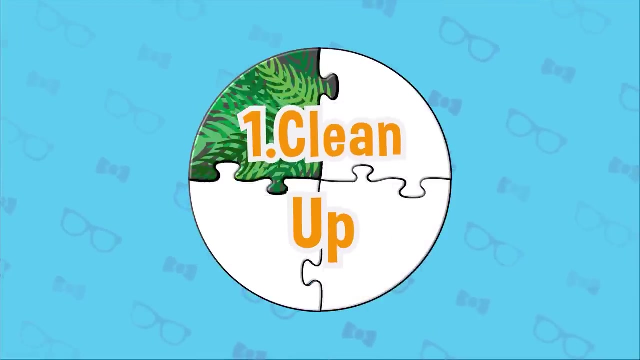 I wonder if there's more puzzle pieces around here. Will you help me look? Hey, it's our first puzzle piece on a great green adventure And our first step in learning how to keep the earth healthy. Step number one is to clean up. 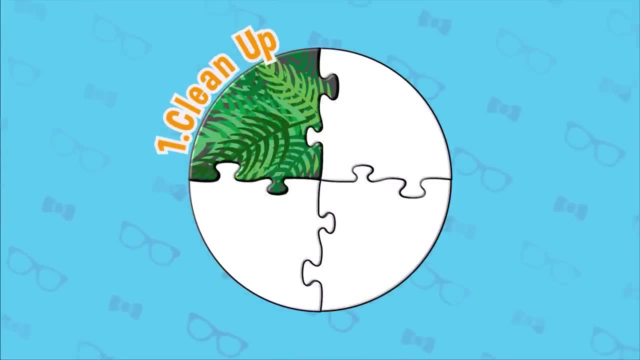 Cleaning up helps get rid of pollution. Pollution is when you make the land, water or air dirty. So by cleaning up we're getting rid of pollution, And that's good for our earth. Yeah, Woo-hoo-hoo-hoo. 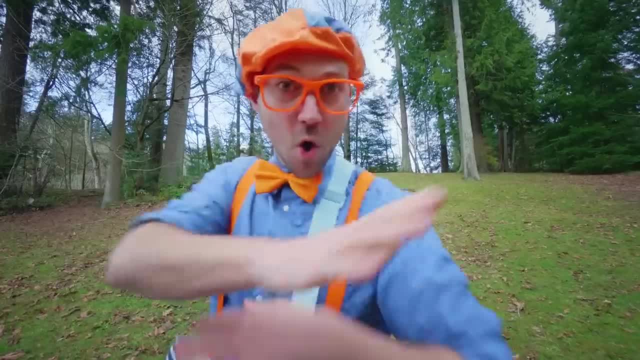 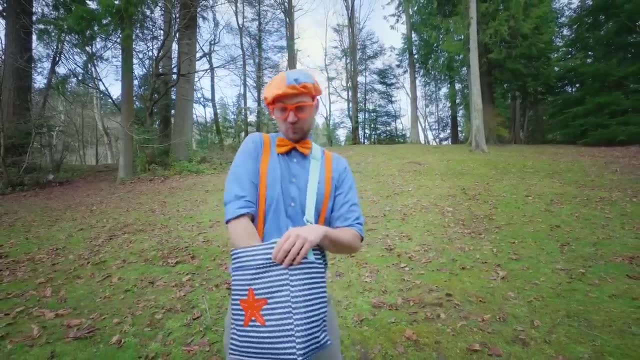 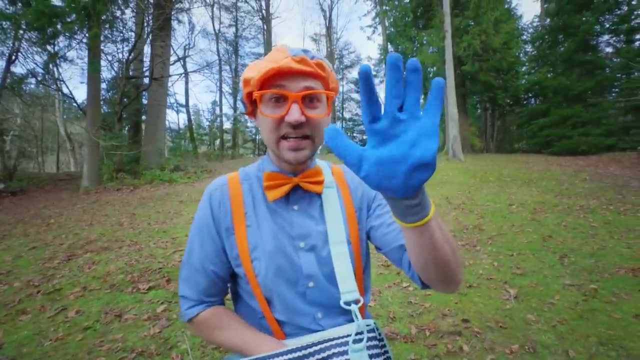 The Blippi Cleanup Crew is here to party. Woo, Yeah, I'm so excited to make sure this place is nice, clean and tidy. Yeah, it's really good for our planet to make sure that it's clean and tidy. All right, first thing we need is our cleanup gloves. 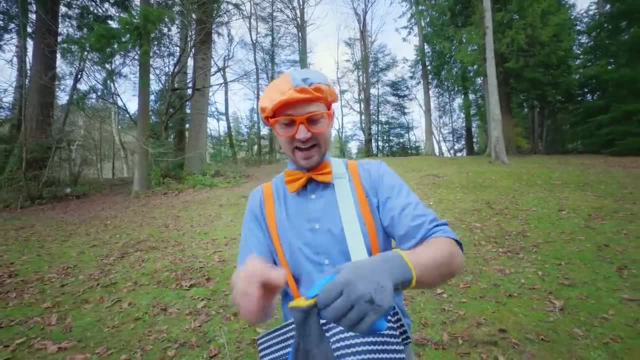 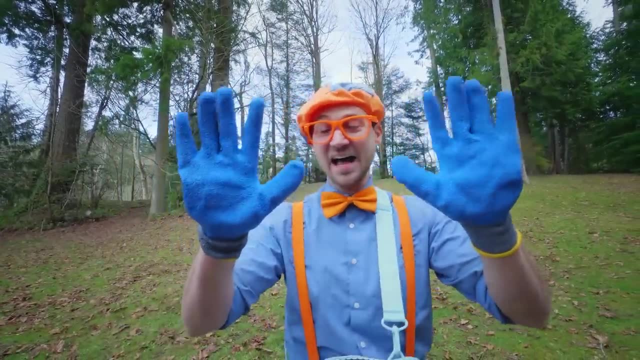 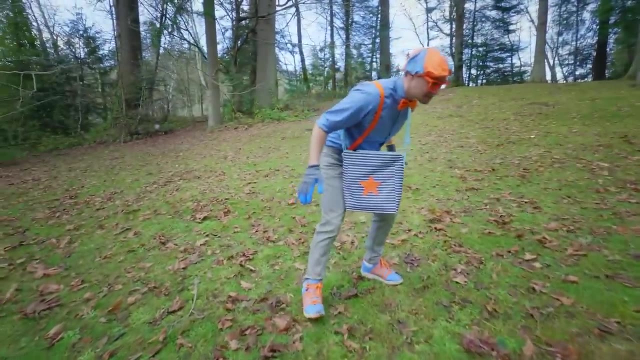 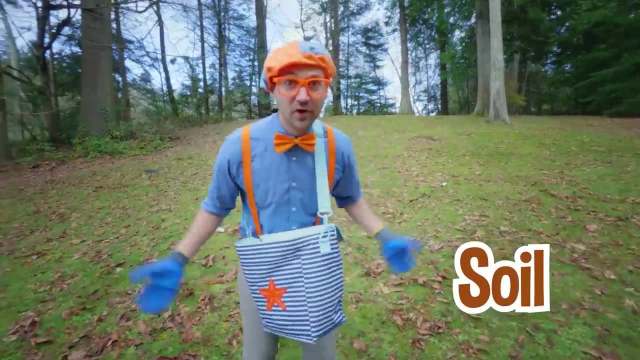 And there is the first glove And here is our second glove. Hey, what color are these? Yeah, the color blue Woo. All right, let's see if we can find some trash. Hmm, let's see. Looks like a bunch of leaves and grass and soil. 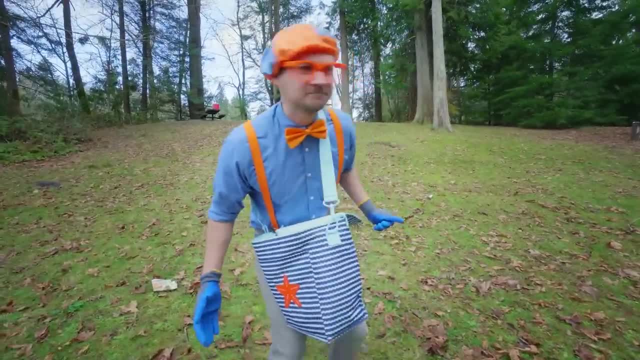 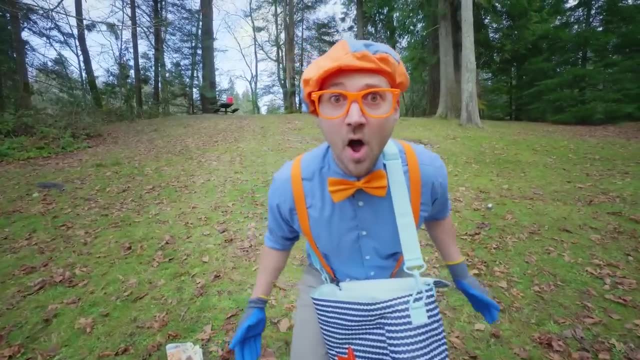 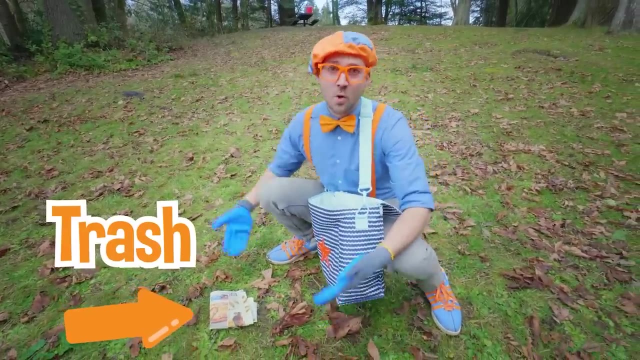 That's all good, All right. hmm, do you see any? I'm not seeing any. Oh, you see some? Oh, down there, Oh yeah, we found some trash. Well, when this is here and it's not supposed to be here, 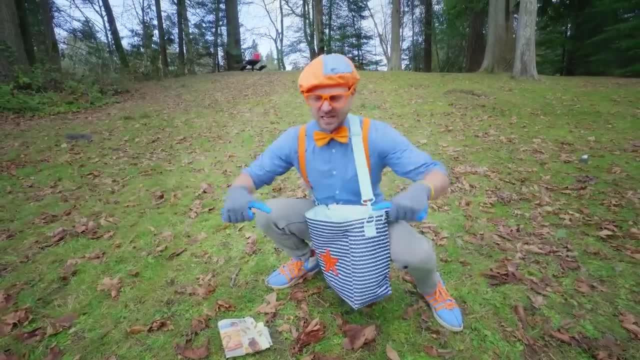 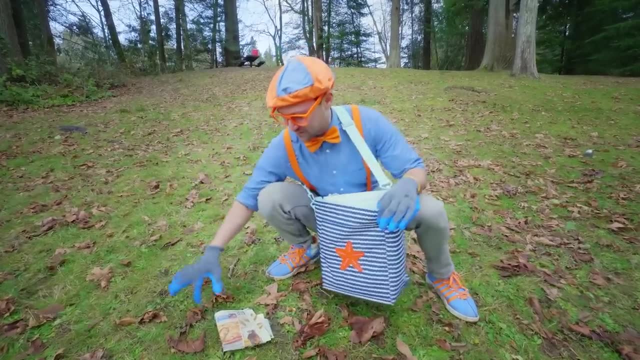 it's called littering, and littering is bad And that makes me angry, But you and I are here to help. All right, first let's pick it up, Yeah, and put it in here, But do you know what this is? 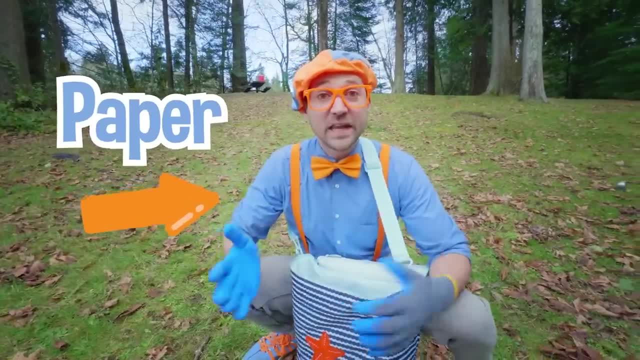 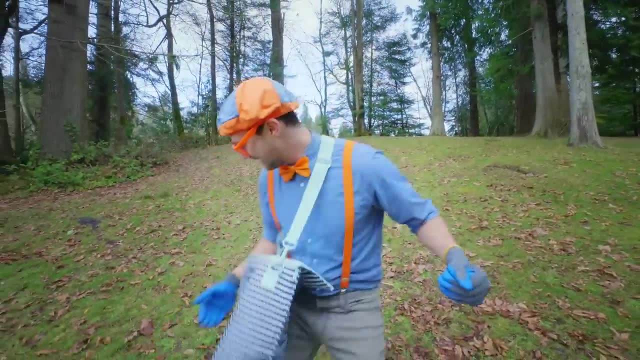 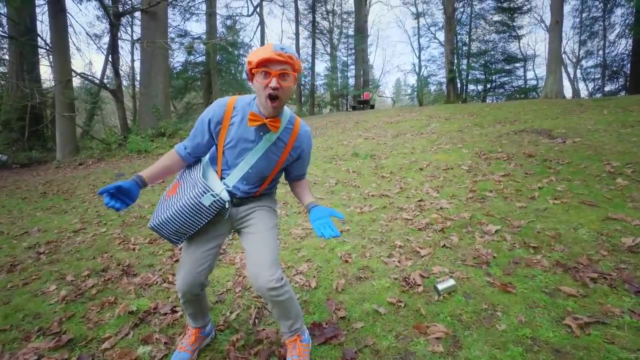 Yeah, this is paper, And paper we can actually recycle it. That means that we'll be able to reuse it later. All right, see if we can find some more. Oh, you see some more Oh down here. Wow, good find. 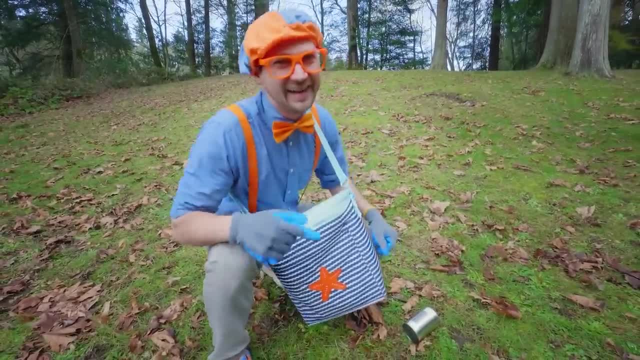 It should not be here though, Ugh. But like I said, you and I we're gonna find it. But, like I said, you and I we're gonna find it. But, like I said, you and I we're gonna find it. 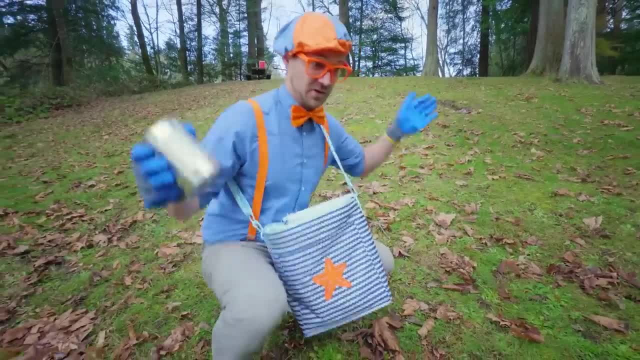 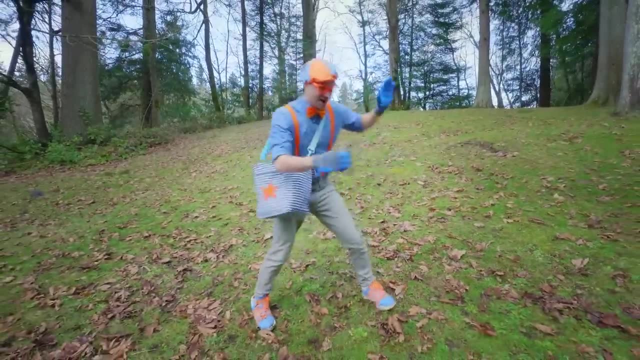 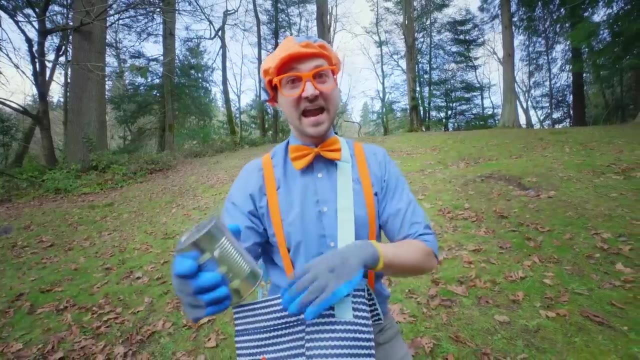 All right, let's see what is this. All right, let's see what is this. Is it a musical instrument? Is it a musical instrument? Is it a musical instrument? Yep, it's a musical instrument, and it was also litter. 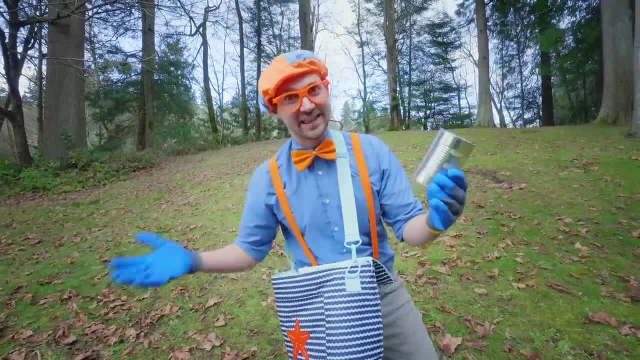 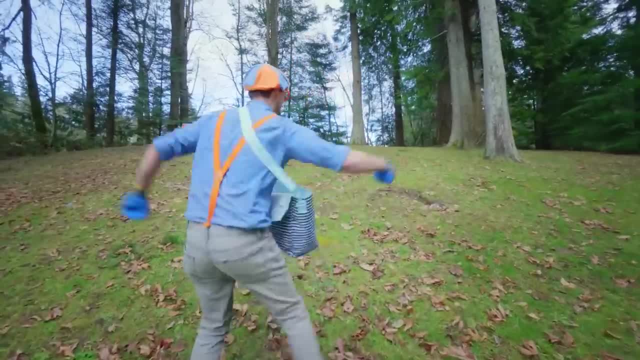 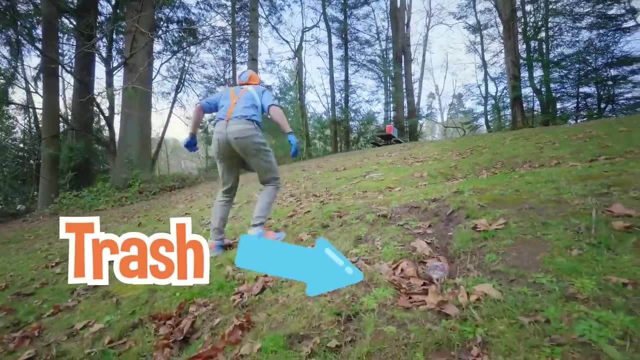 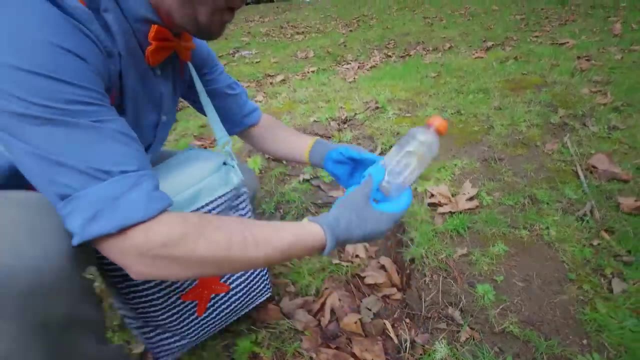 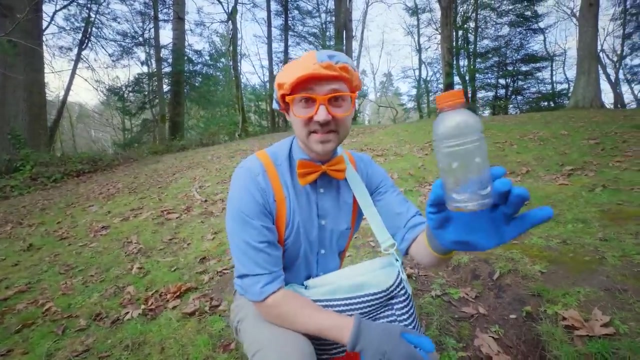 Good job. Do you see any? Oh, back there. Oh yeah, We found another piece. Wow, Good job, We are doing such great work today. Whoa, And this is a plastic bottle, And this is a plastic bottle. 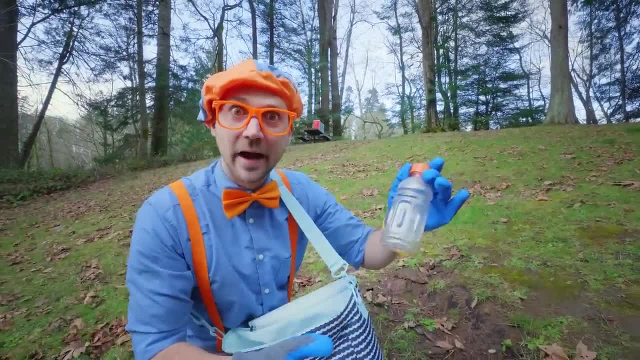 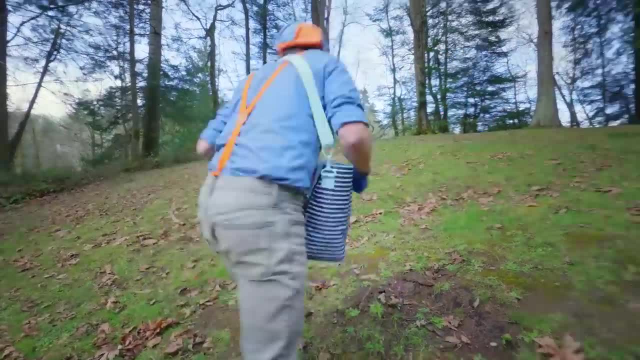 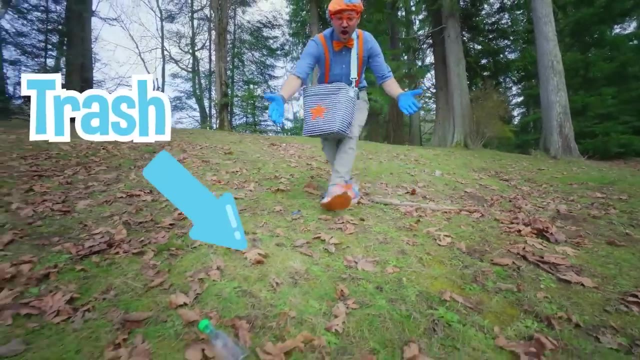 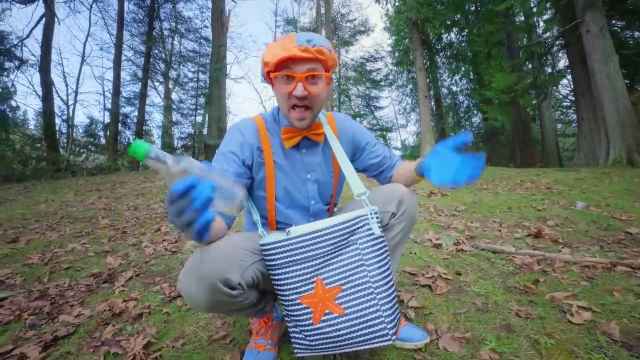 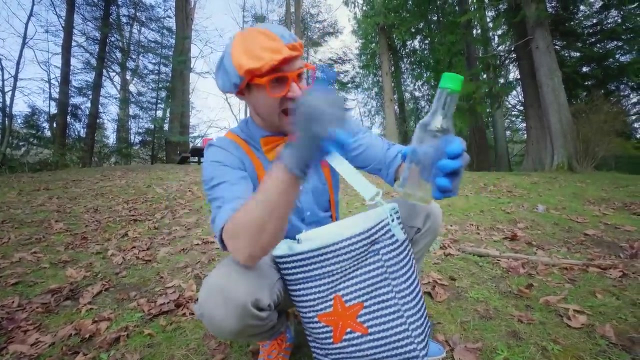 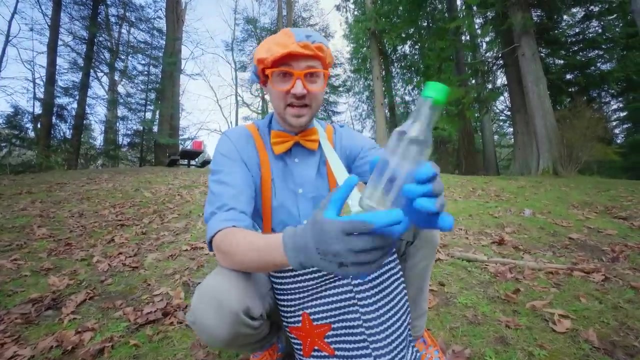 Oh, I wonder what was in here at one time, who knows? and we're too busy gonna recycle this. yeah, another thing to recycle. yeah, we have found so many things in this park that we can recycle, yep, and reuse in this park. this is a glass bottle. yeah, glass is also recyclable, so let's put it in the bag. 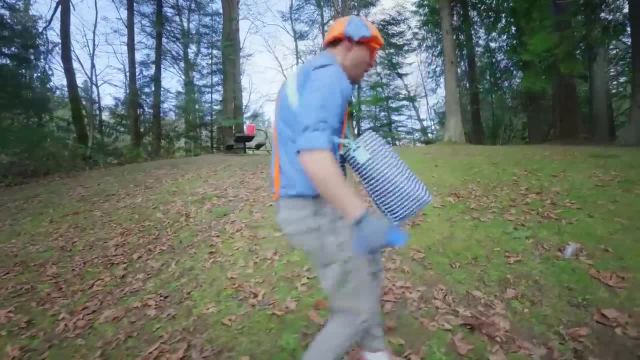 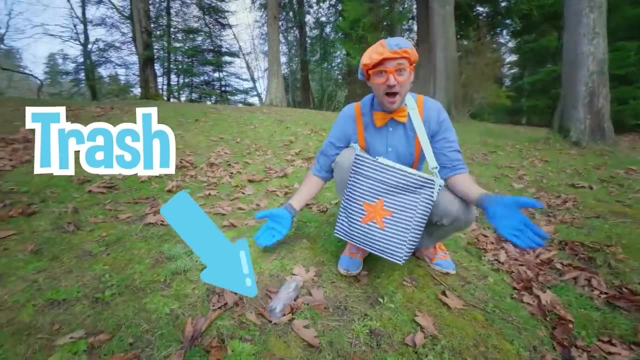 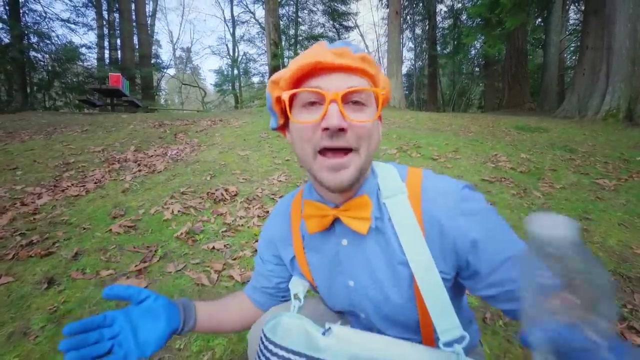 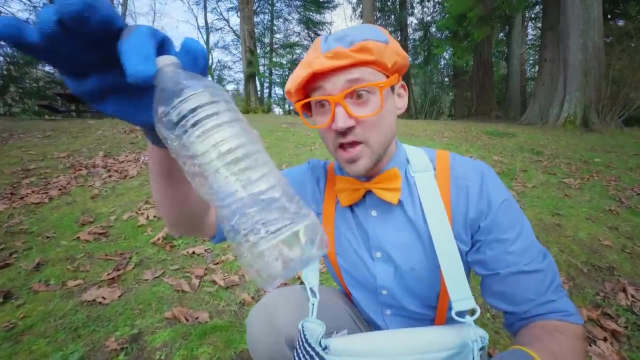 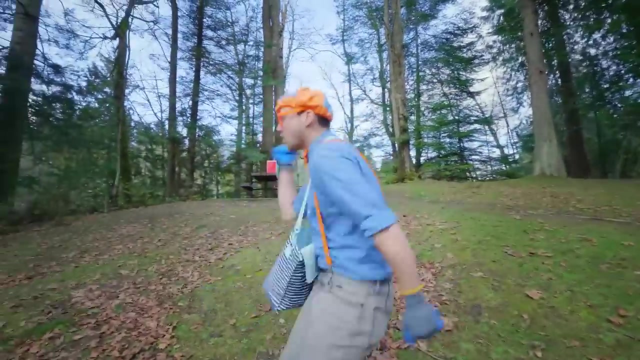 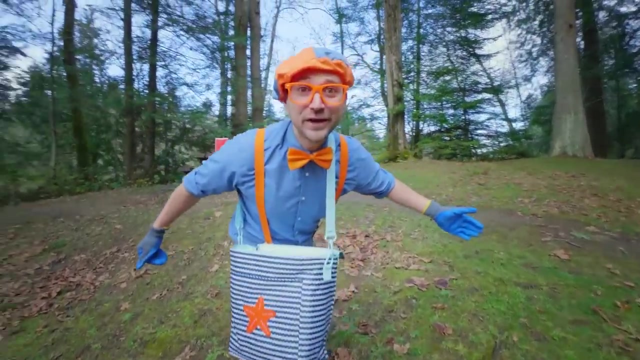 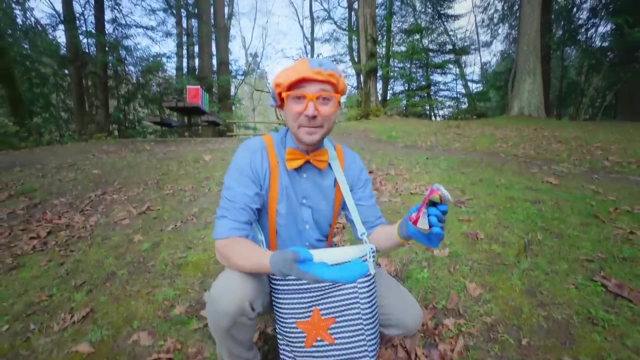 and use it for later. oh, good job. another one, yeah, and you know what? this is? a really loud plastic water bottle and water bottles that are plastic you can recycle. here we go, did you hear that? yeah, i stepped on an aluminum can, an aluminum you can recycle. 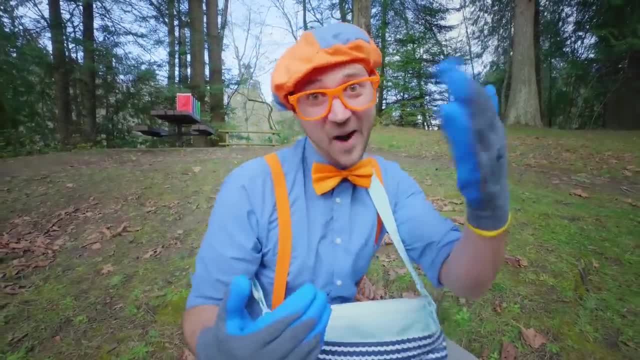 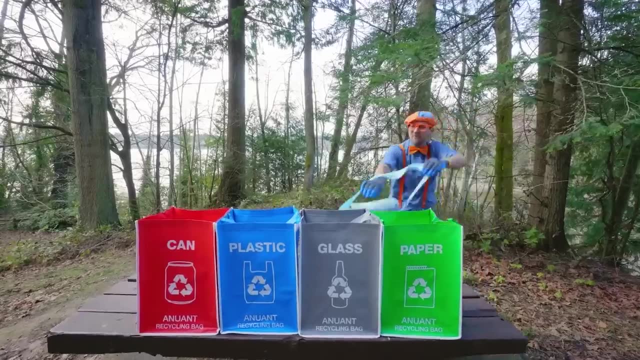 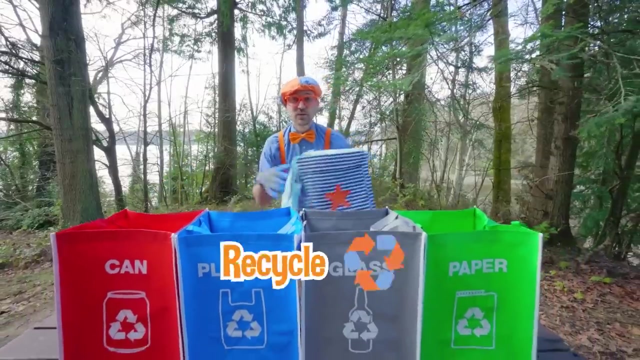 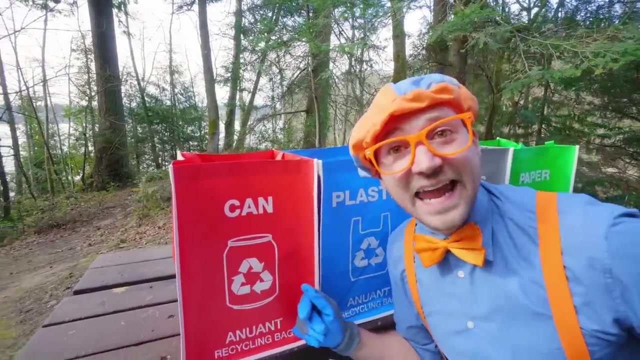 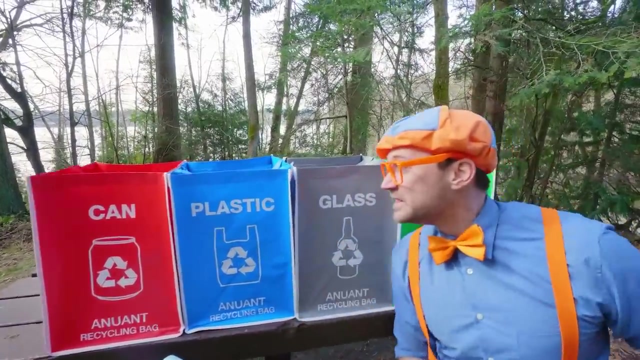 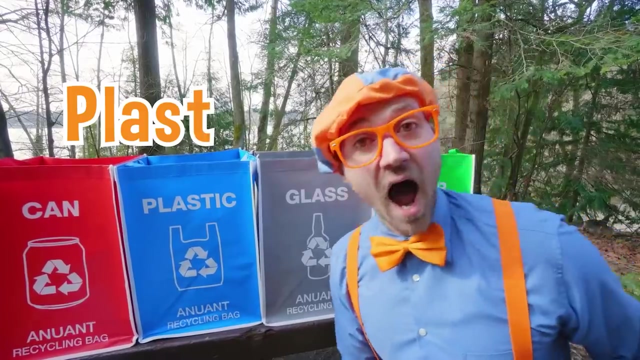 so let's put it in here and let's recycle. come on, wow, check it out. wow, four bins to put all the litter that we found, yeah, into them, so then we can recycle. all right, let's see what they read. this one says: can see a n can. this one says: plastic p l a s, t i s. 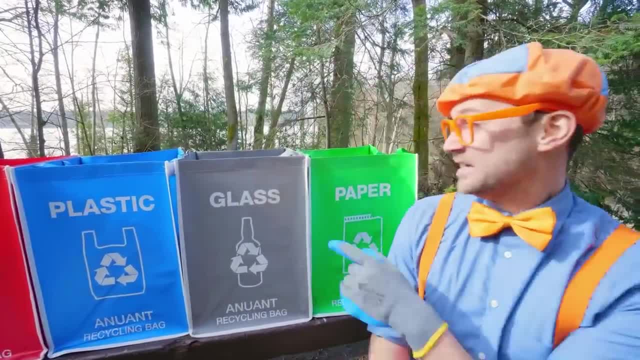 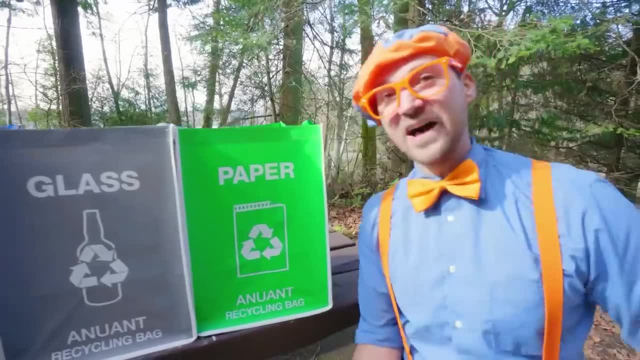 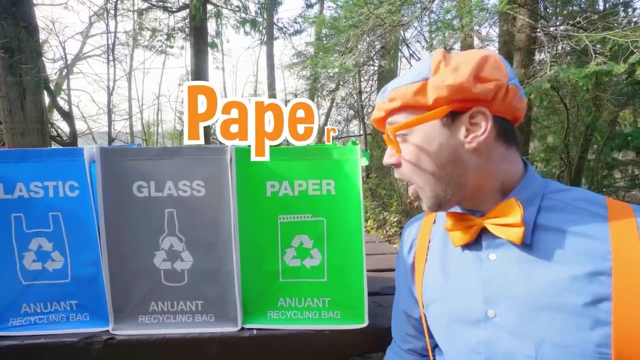 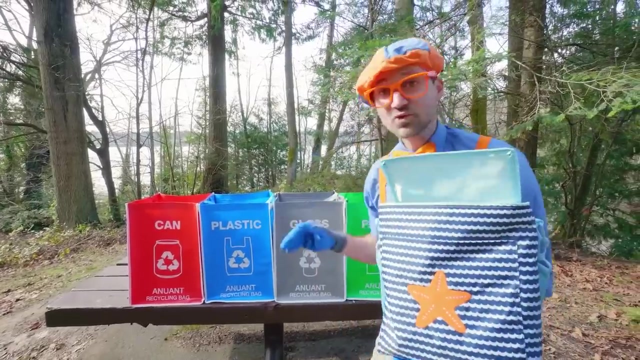 plastic glass, g l a s s glass and, last but not least, paper: P-A-P-E-R paper. Okay, now we need to take all the items that we just found and sort them, so then they can be recycled. All right, let's see. 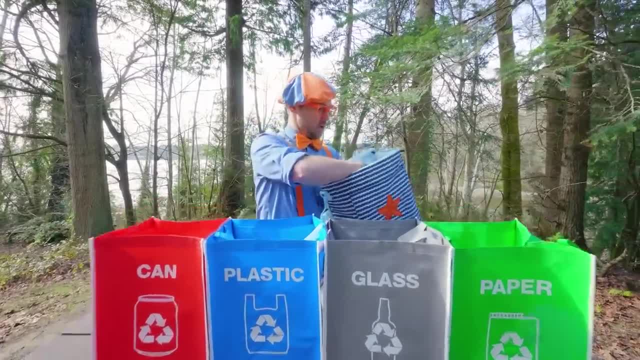 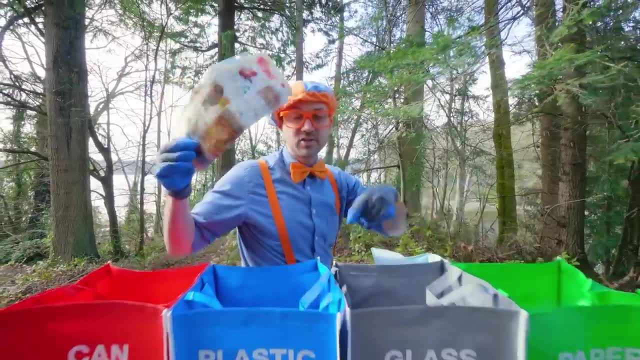 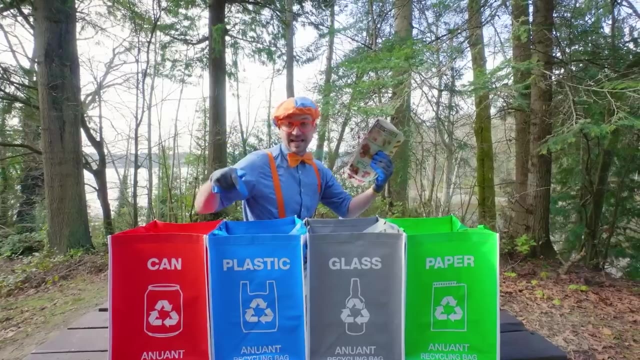 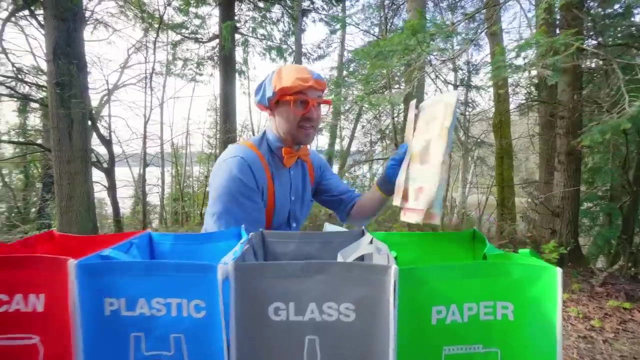 The first item that we found. Oh yeah, you remember what this is. Let's see which one do you think it goes in. Let's see Cans: No Plastic. No Glass. No Yeah, this is paper. 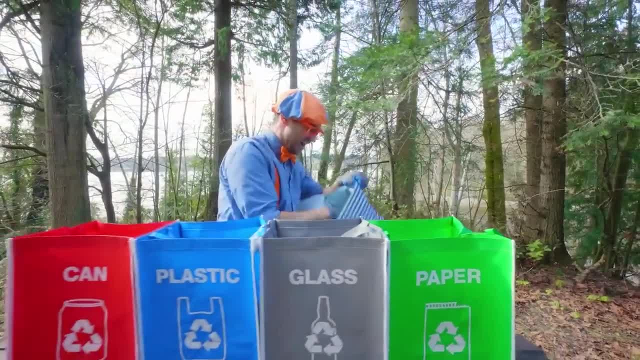 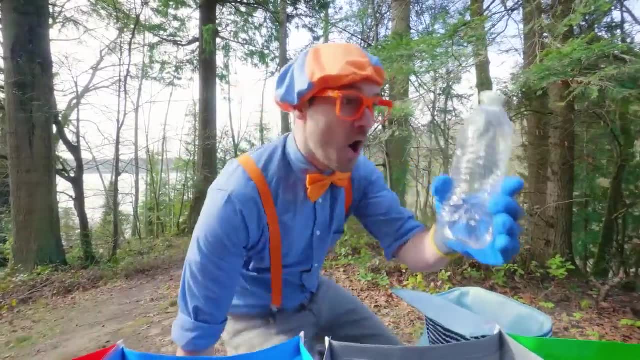 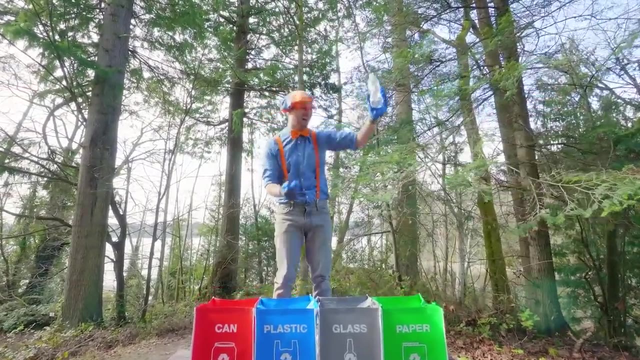 Yeah, there you go. All right, what else do we have in here? Let's close our eyes. Oh yeah, woohoo, The plastic water bottle. All right, which one of these is for plastic? Hmmm, Let's see. 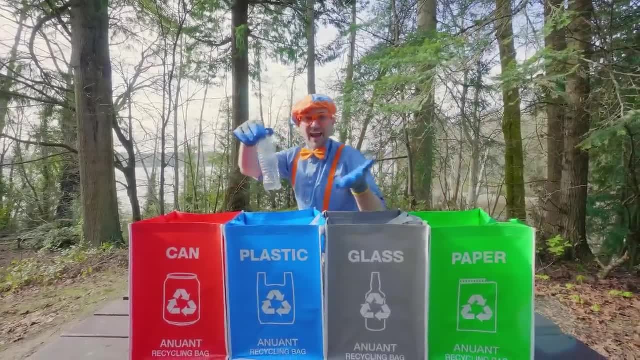 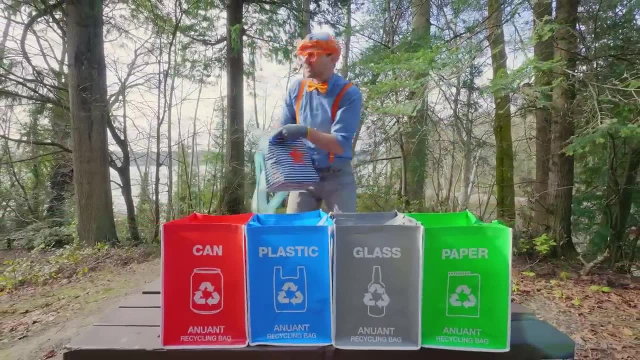 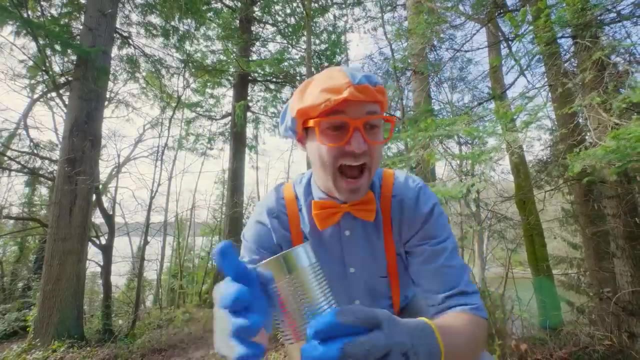 Oh yeah, plastic. All right, here we go, Let's close our eyes. Wow, remember this. Yeah, that's what I always said. This one, This is my broadly known pregnant figure. again, A little delivery hook. Ah, the musical instrument. 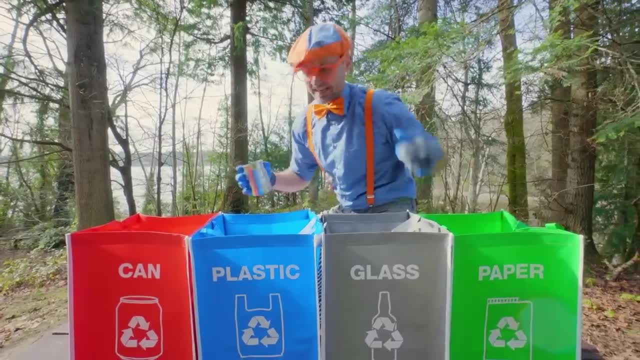 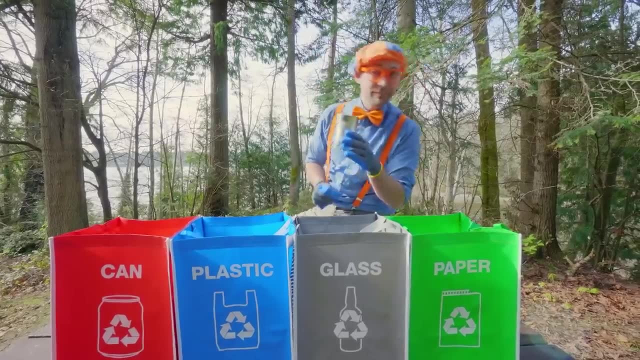 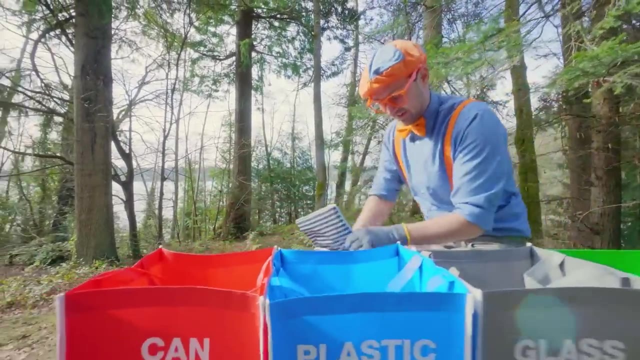 All right, enough playing around. We need to clean up our planet. All right, what is this? Is it a can, plastic, glass or paper? Yeah, it's a can. All right, just a few more things. Whoa, check this out. 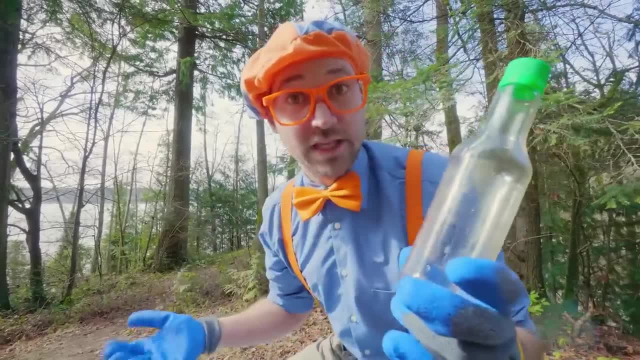 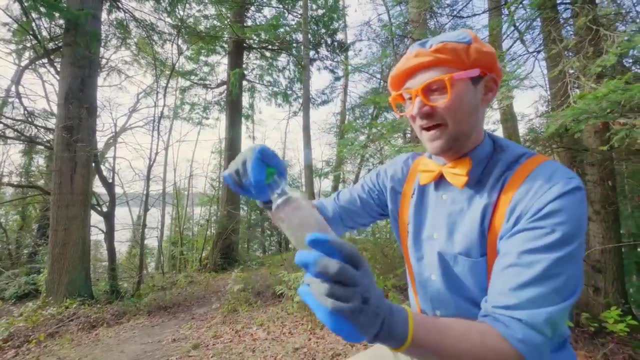 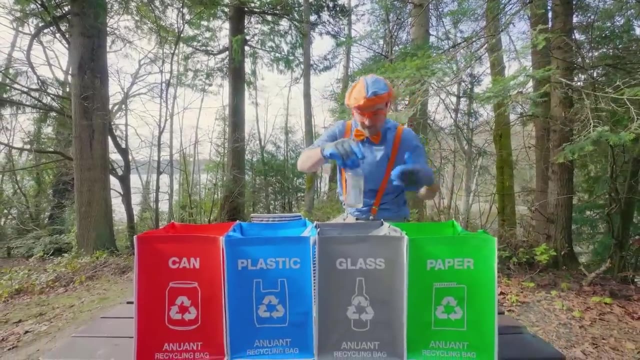 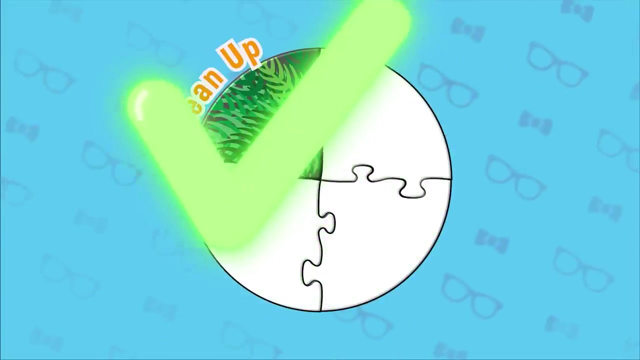 Yeah, this clear bottle. It's really hard. Wow, I can't crush it, but it's pretty delicate. Yeah, this is glass. All right, here we go. Yeah, We finished the first step on our great green adventure. 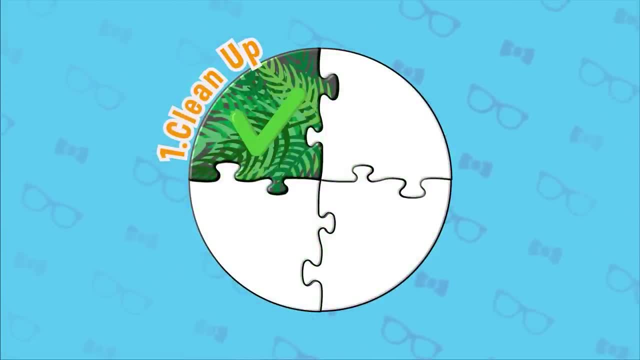 Nice job cleaning up the planet. Let's clean up all that litter and recycling. Remember: recycling is when we take paper, plastic, glass and cans and allow them to be turned into something else instead of thrown away- An easy thing we did to make the world a better place. 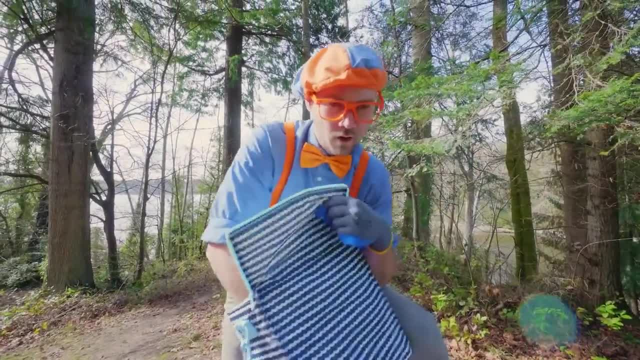 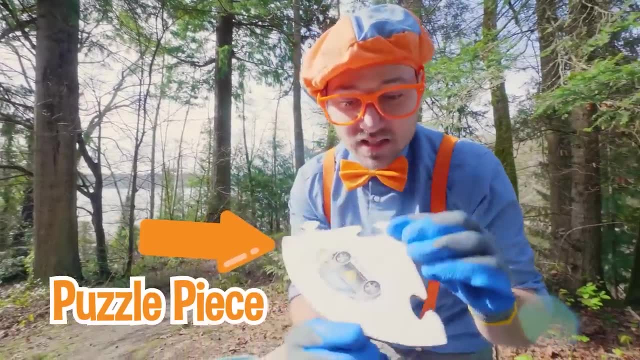 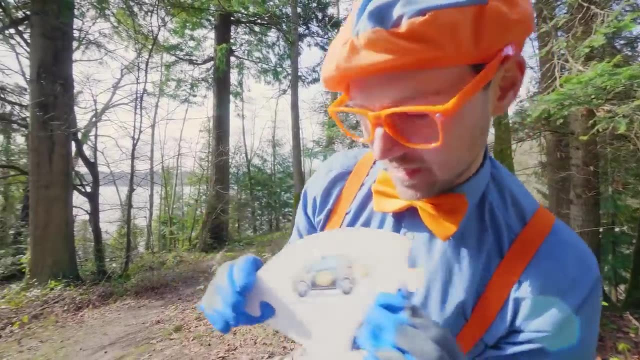 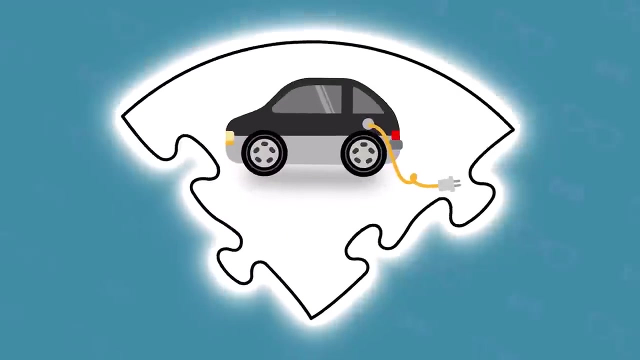 All right, what else is in here? Whoa, look at what we found. Another puzzle piece: Whoa, Good job. We are doing so great today. Hey, what's on it? Hmm, Yeah, this is an electric car. 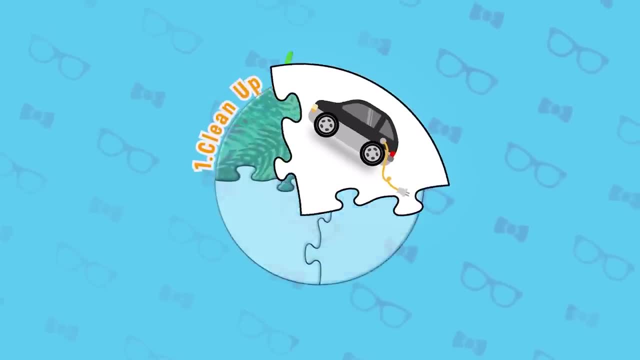 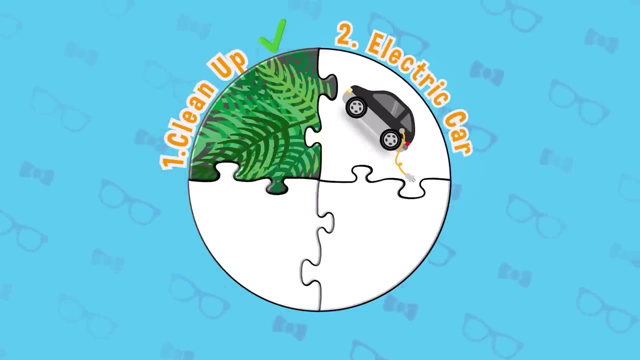 Another piece of the great green adventure puzzle. Woo-hoo, Step number two: let's check out an electric car. Electric cars are super cool because they run on electricity instead of gas, and that's great for our Earth. But before we do that, let's learn a little more. 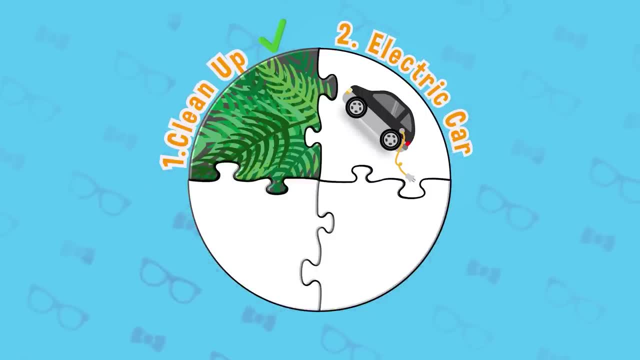 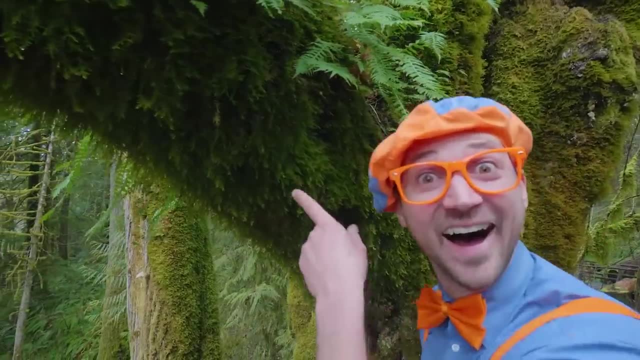 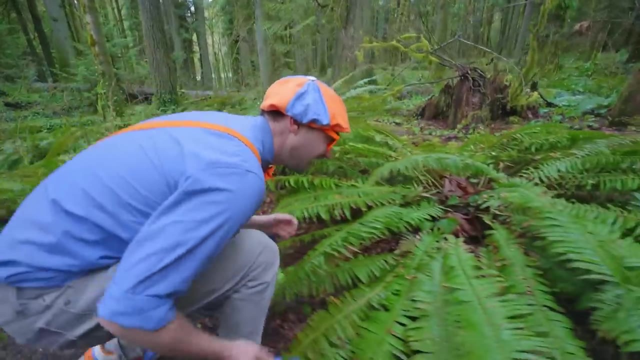 about respecting our planet Earth because it's our home. Look at the plants, look at the trees, all the beautiful colors, all the gorgeous leaves. Our Earth is green. our Earth is blue. Protect its goodness for me and you. Our Earth is rare and we only get one. 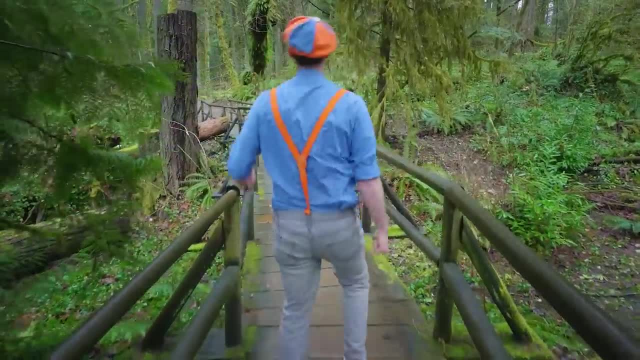 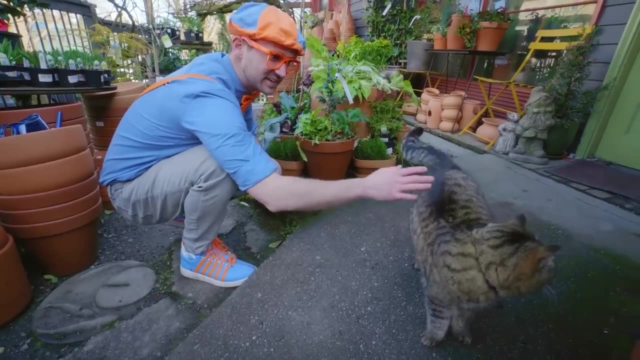 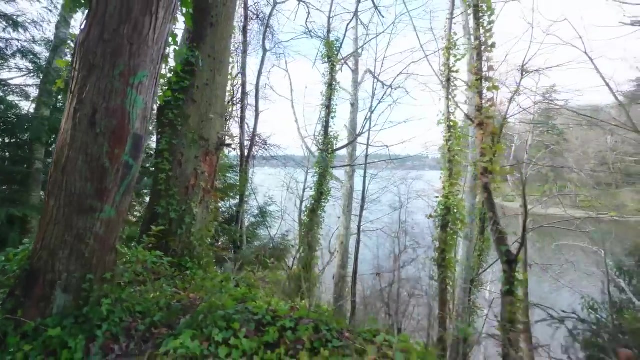 Let's help it along, Come on, it's fun. Respect the trees: they give us lots of air. Respect the creatures: give them lots of care. Respect the plants, because they help us all to breathe. Respect the water, the oceans and seas. 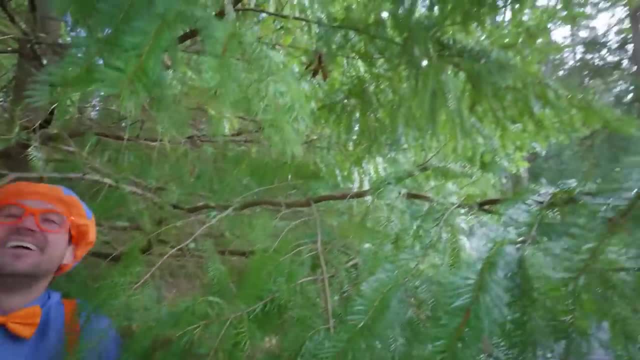 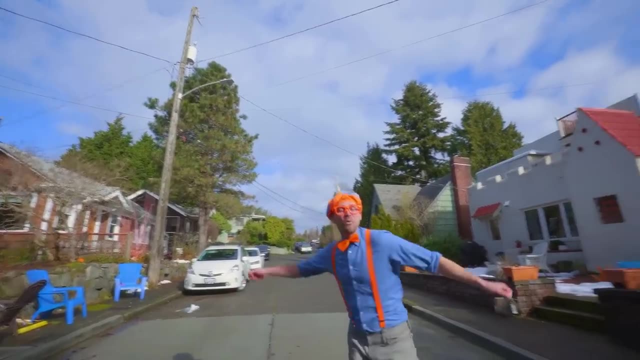 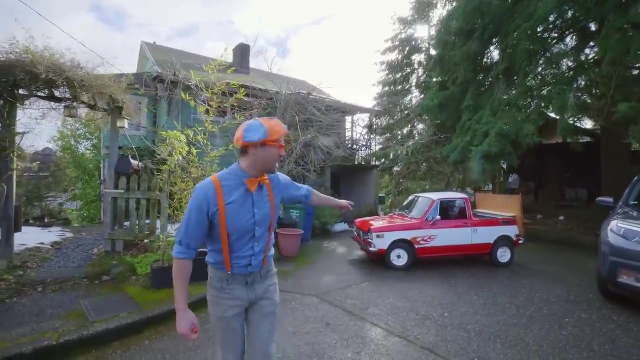 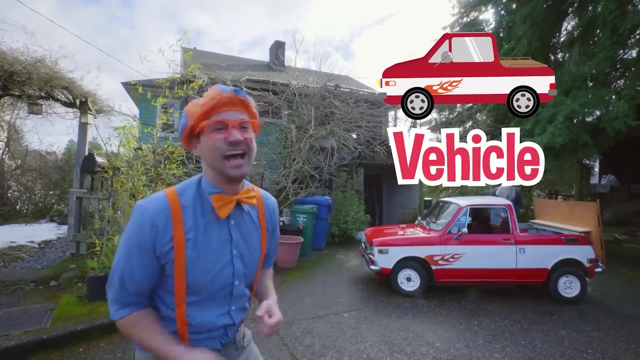 When we make a change, we'll see the worth. We all have to help and respect our Earth. Wow, what a beautiful day it is out here. Oh, Whoa, check it out. Do you see what this is? Yeah, this is a red and white vehicle. 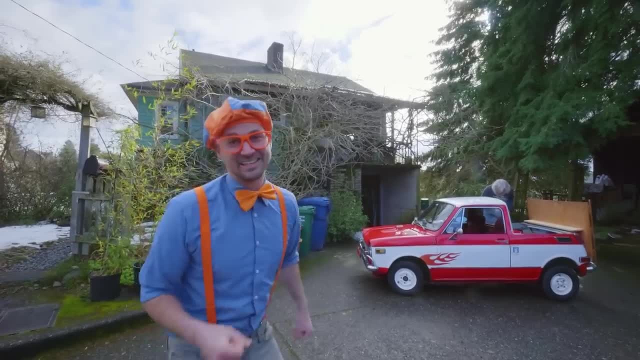 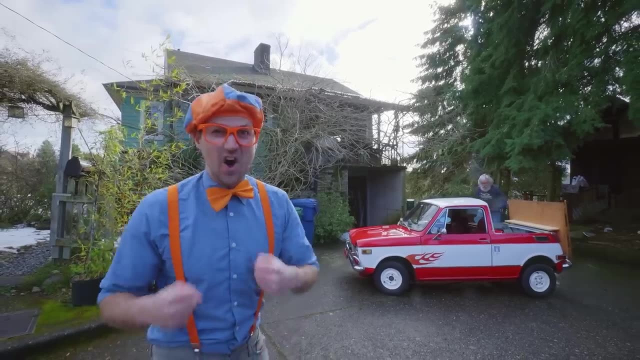 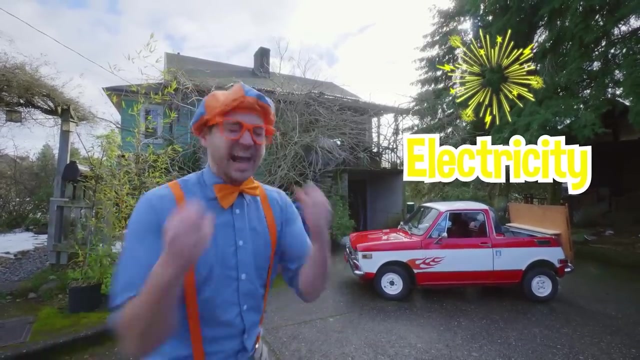 Looks like a small car or a truck, And today you and I are gonna meet someone really cool. That's Dave over there and he is awesome. He did something awesome. He took a gas-powered vehicle and converted it to run on electricity. 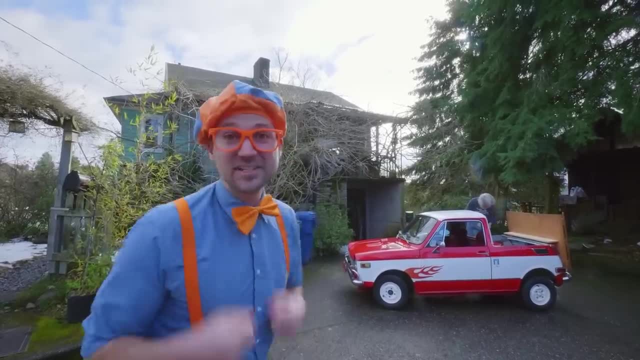 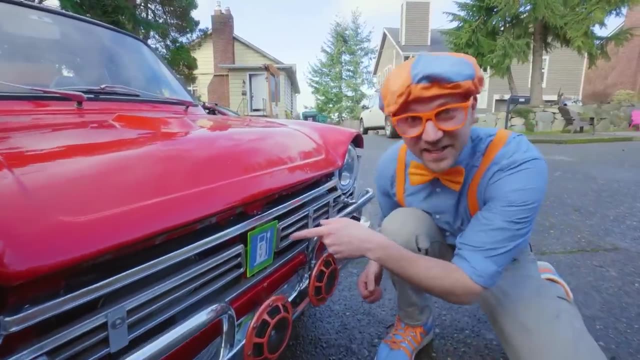 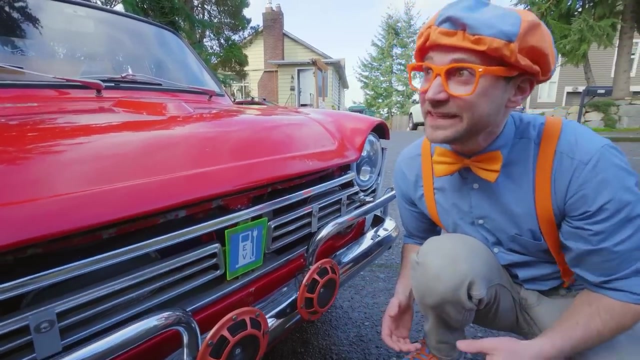 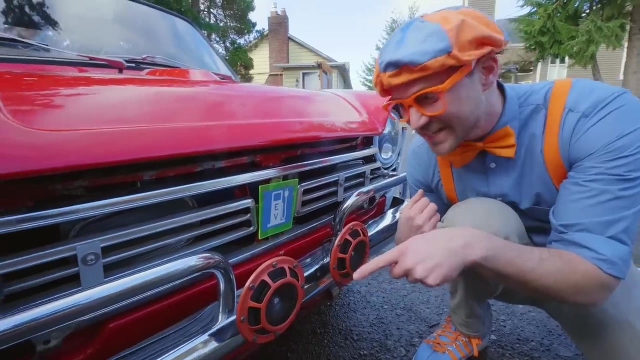 I am so excited. I'm excited to meet Dave and check out his cool vehicle. Let's go. Wow, check it out. This little logo says EV. Yeah, the two letters EV stand for electric vehicle, Whoa and these, these little speakers. 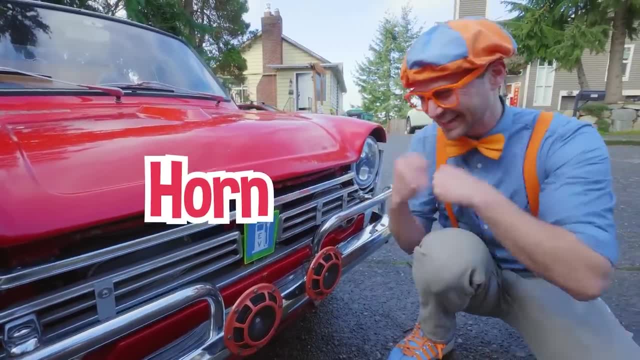 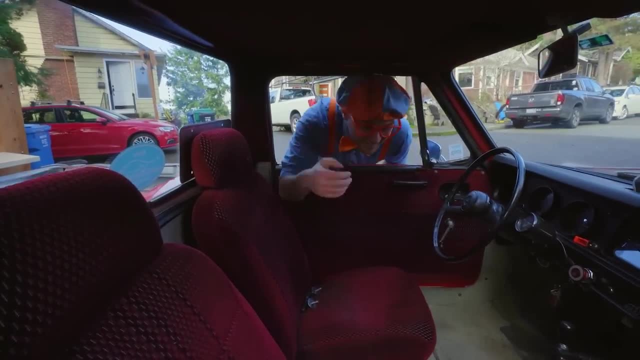 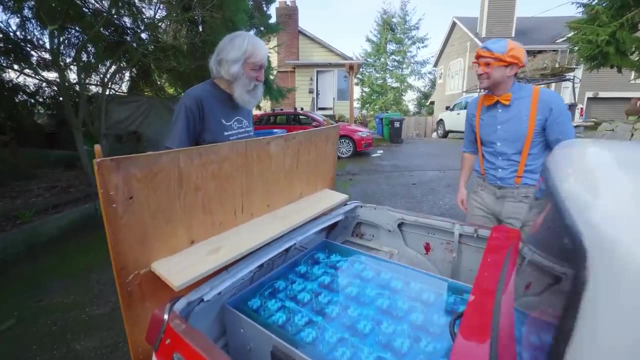 yeah, these are the horn. That's awesome. Wow, Wow, What a cool vehicle. Oh hello, Wow, what a great interior. Oh, hey, Dave, how are you? Hi Blippi, how are you? Oh, good, thank you for showing us your cool vehicle. 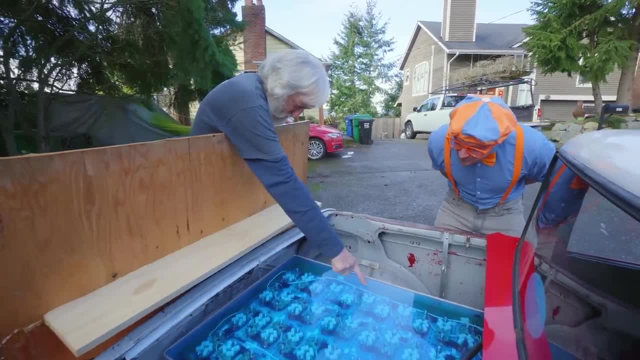 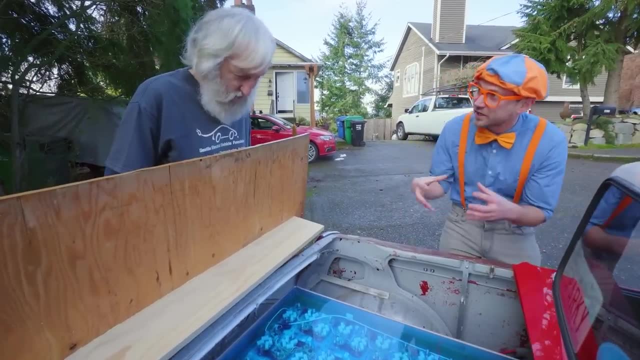 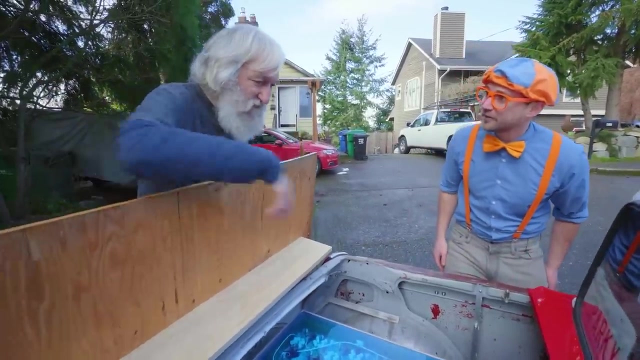 What's this? That's the battery. It's actually 48 batteries all connected together with these copper bars. Wow, you said it's 48 batteries all connected, Connected into one big battery. Wow, Hey, have you ever named this vehicle before? 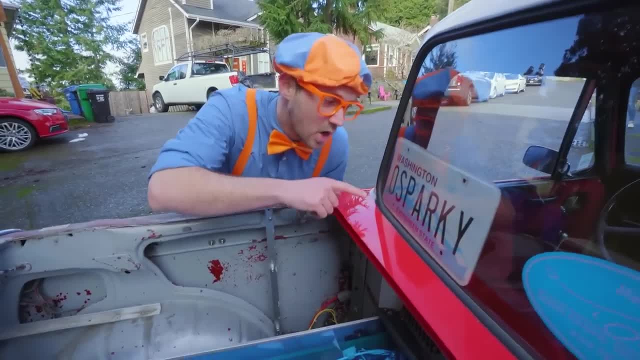 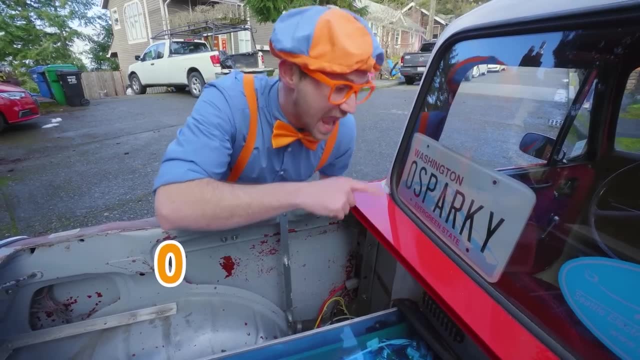 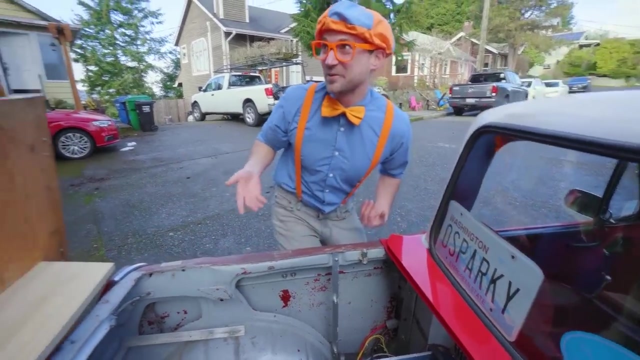 Yeah, it's O Sparky, O Sparky, Hey, yeah, this is this vehicle's name: O Sparky, O-S-P-A-R-K-Y. Oh, O Sparky, Is that because it runs on electricity? Yeah. 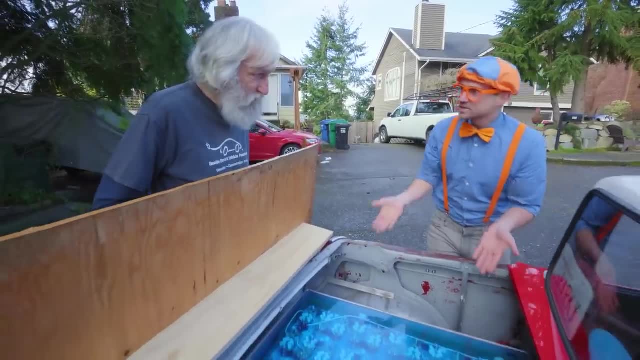 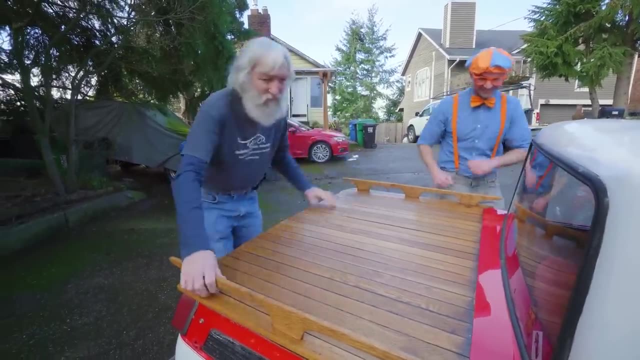 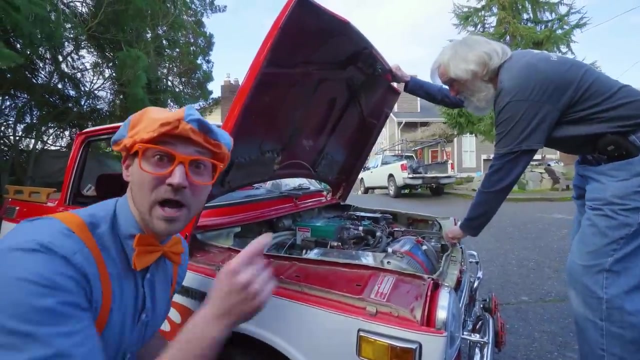 That's a cool name. Hey, if this is the battery, where's the motor at The motor's up front? You want to see it? Yeah, All right, Wow, Whoa, check it out. This is the motor of O Sparky. 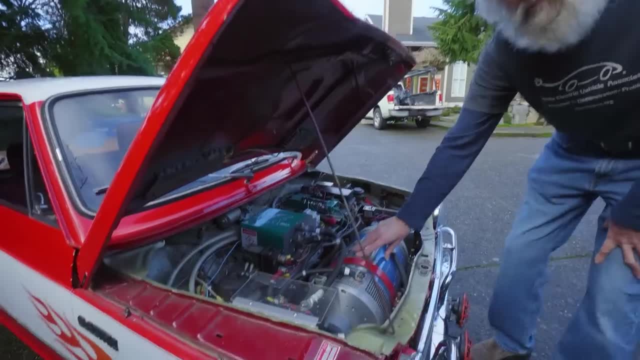 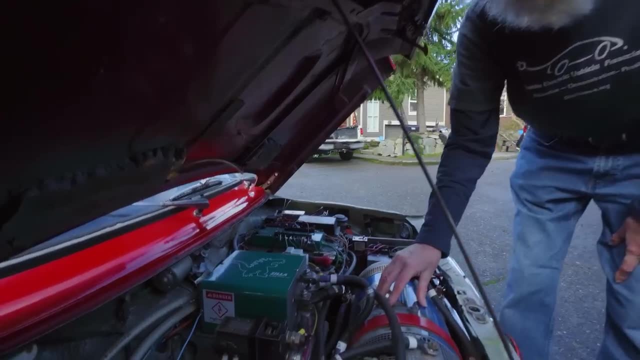 Can you tell us what all this stuff is? Well, this is a real big motor And this is the. this is what brings the power from the battery to the motor, And this is the brains that tells this how much power it needs. 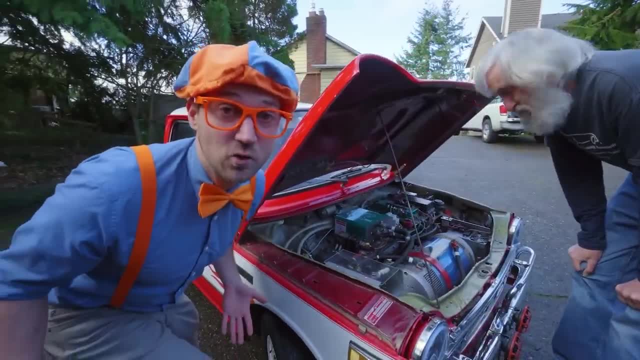 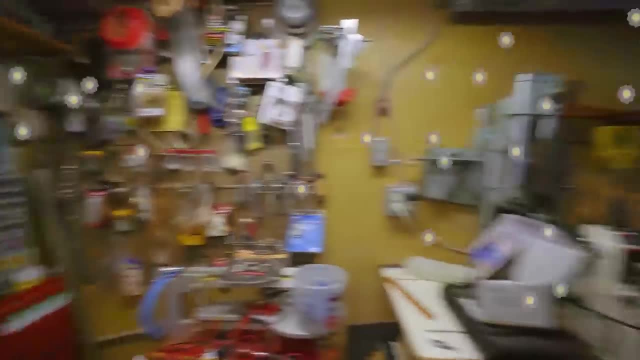 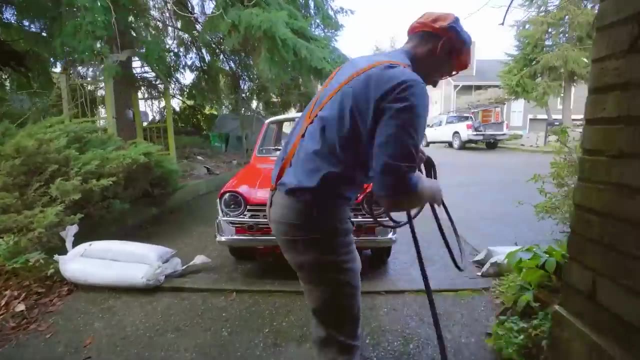 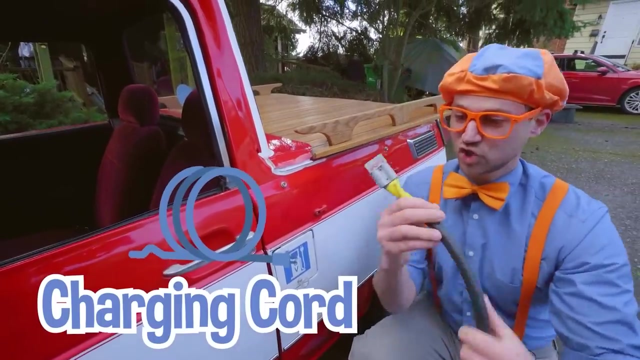 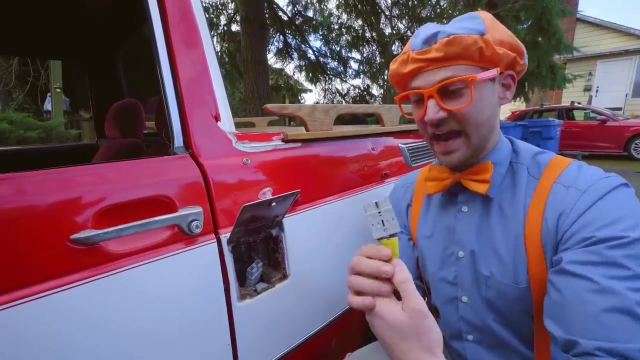 Wow, That is really cool. Hey, can I drive O Sparky today? Oh yeah, Yeah, Wow, check it out. Yeah, this is the charging cord of O Sparky. All right, There we go. Yeah, You know how gasoline vehicles have a little area. 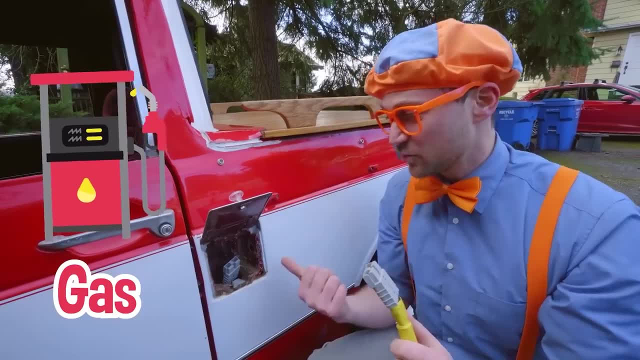 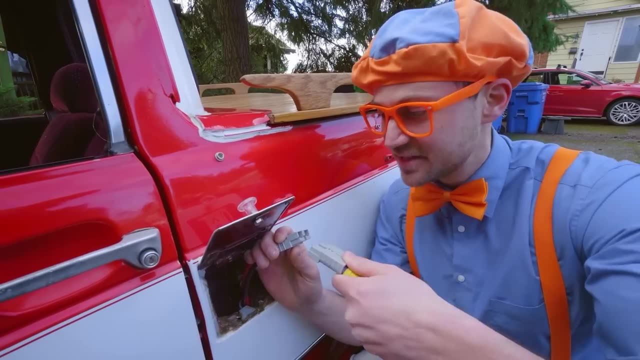 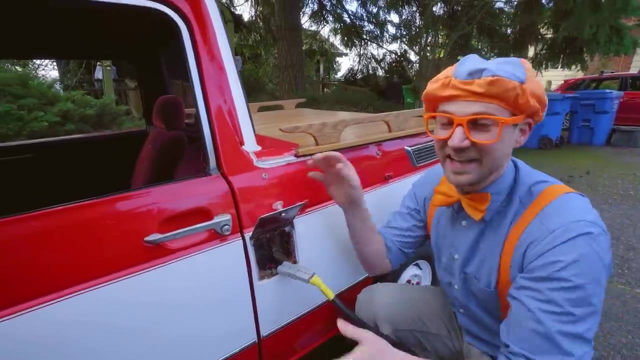 to fill it up with gasoline. Not this one. This one has a cable, Wow. And then this is how you charge the batteries. So first you have to plug it in, just like that, And then you let it sit In the meantime. let's check out the vehicle. 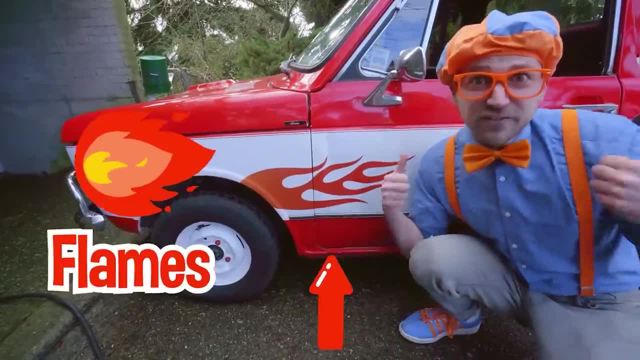 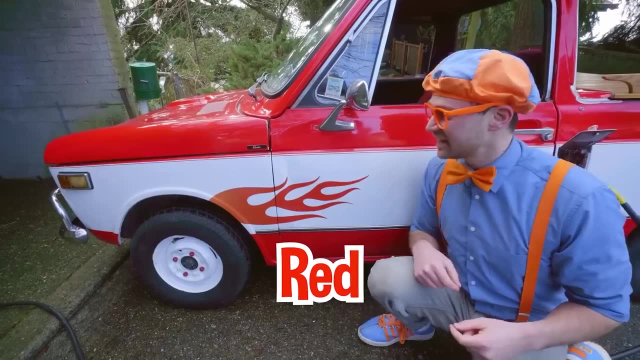 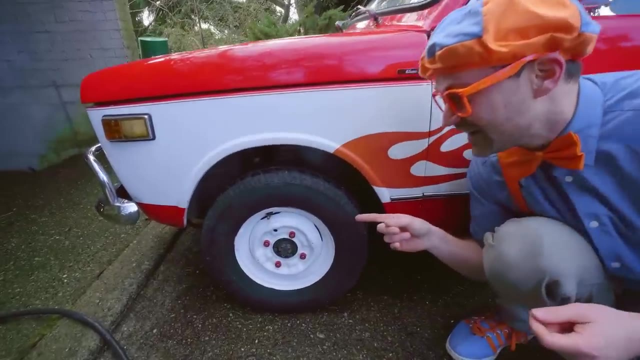 Whoa, look at this, Yeah, Flames. Wow, These flames are the color red. Yeah, just like this. Hey, and what color is this? White? Whoa, And look down here. Oh, some cute wheels and tires. 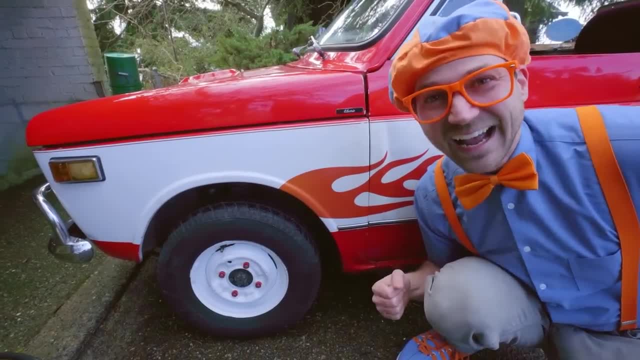 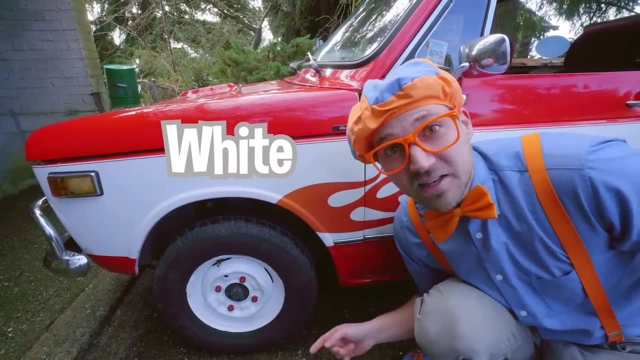 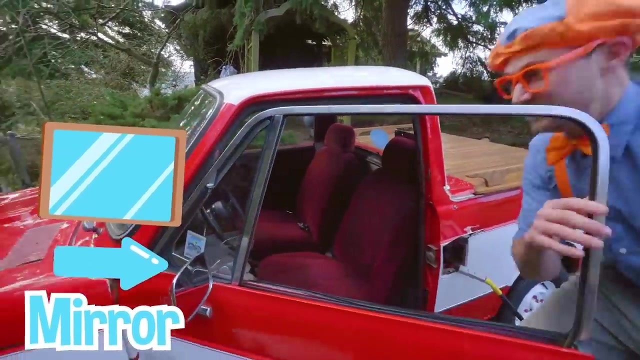 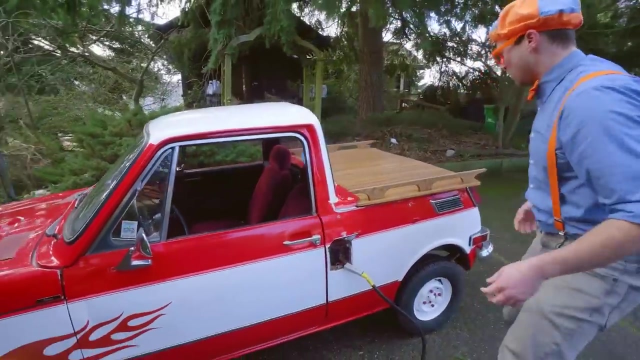 What color is the rubber on this tire? Yeah, it's the color black, And the wheel is white And the lug nuts are red. Wow, Hey. And the little mirror right here, Hello, Hey, Wow, Whoa. And then we saw this earlier. 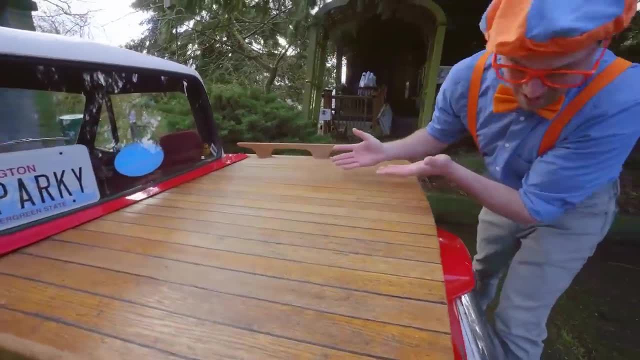 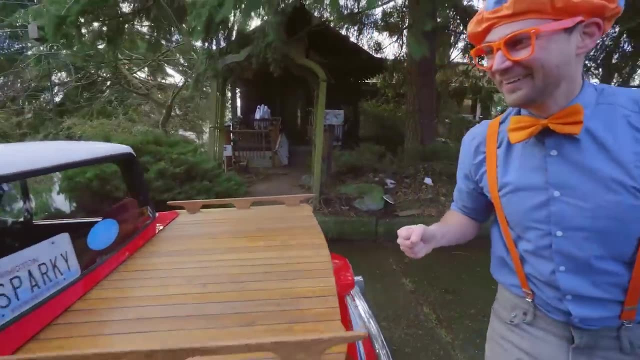 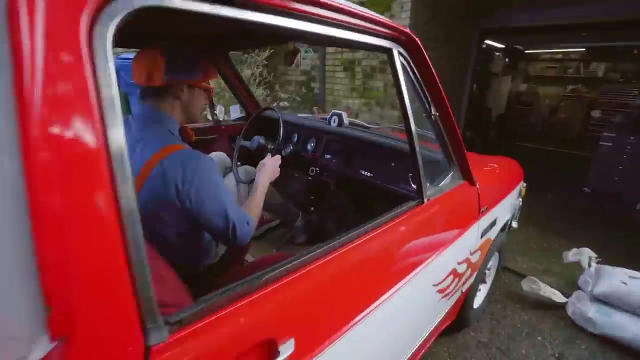 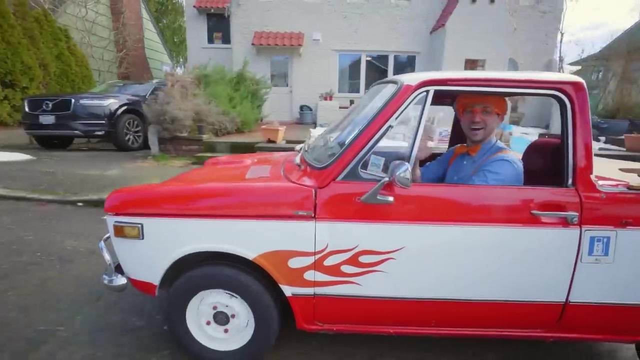 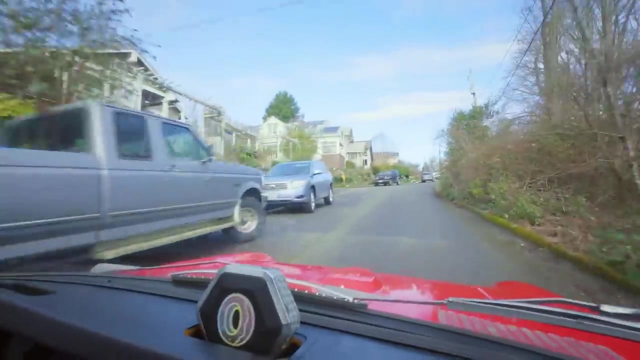 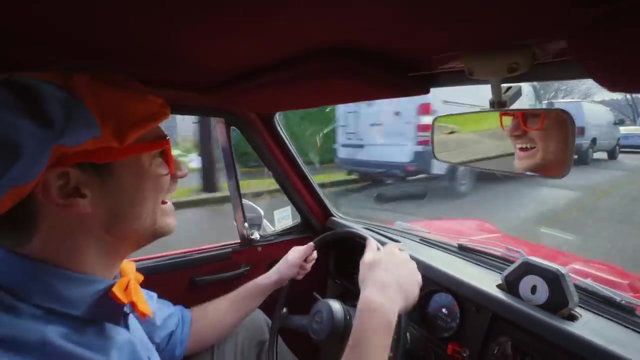 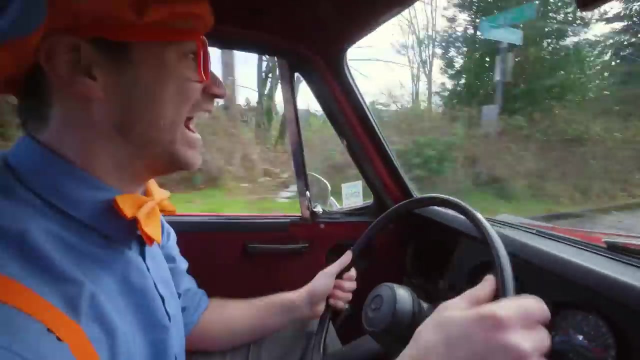 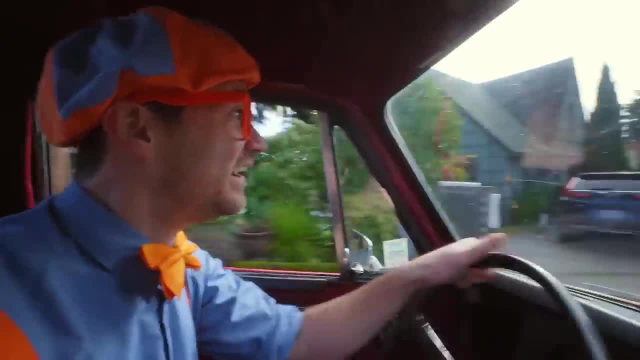 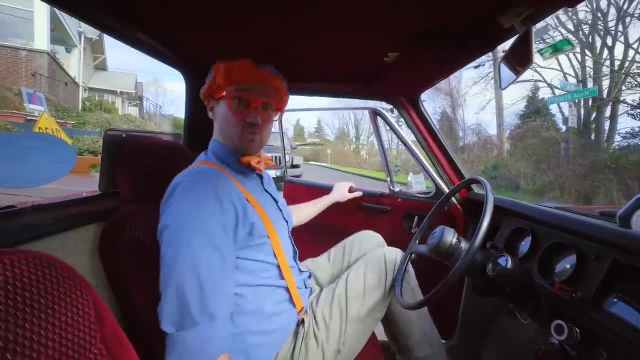 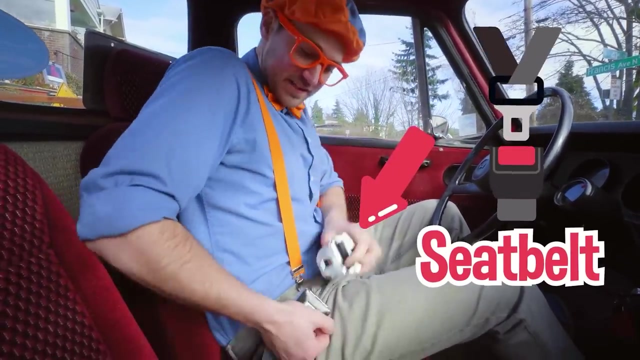 Woo hoo, Woo hoo, Woo hoo. Hey, Let's check out the inside of the super rad vehicle. Woo hoo, All right, First thing's first, Yeah, Safety first. That's why I'm going to put on my seat belt. 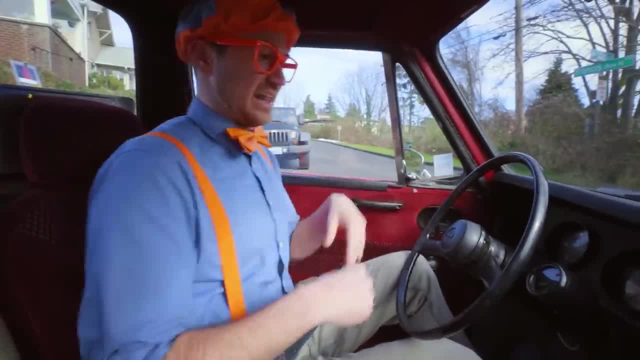 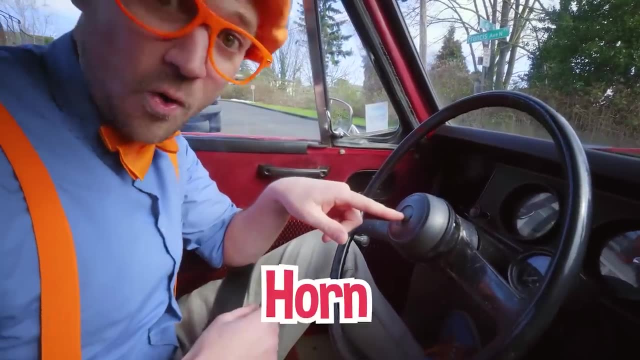 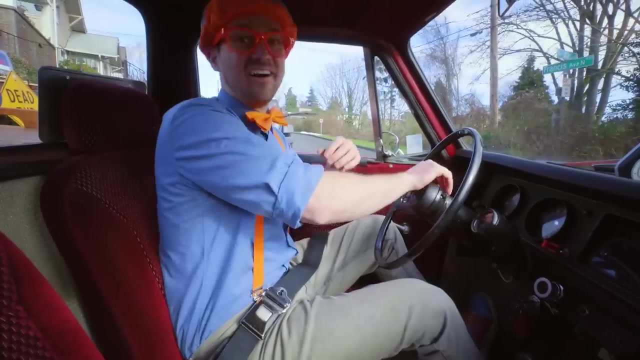 There we go, Tighten it up, Perfect, All right, Check this out. This is the steering wheel, And in the center of the steering wheel there's a little bit of rubber steering wheel. we have the horn. Listen, That's so silly. All right Down here we have some foot. 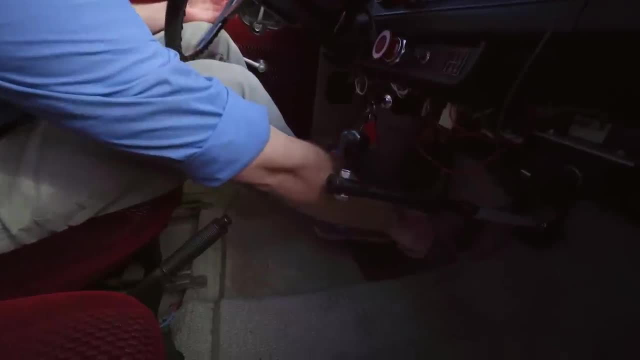 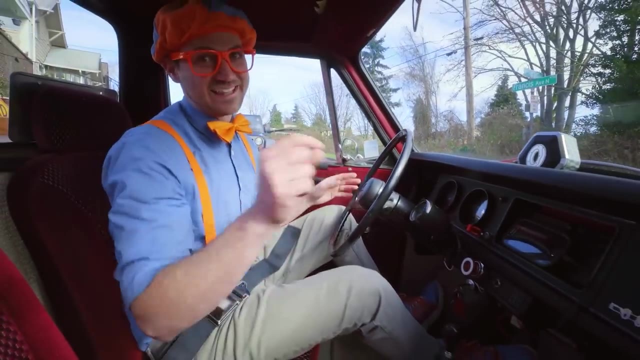 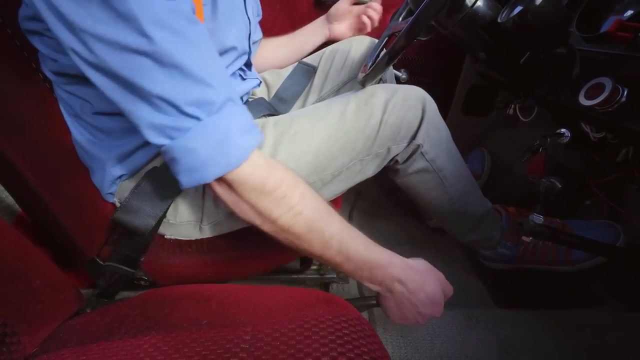 pedals. This, yeah, that is the throttle, This is the brake And the left one is the clutch. But you don't use that in this vehicle. All right, And right here, this is the parking brake. Okay, Here we go. Whoa, You see how I'm moving. Whoa, Okay, I put my foot on the brake because as soon as I 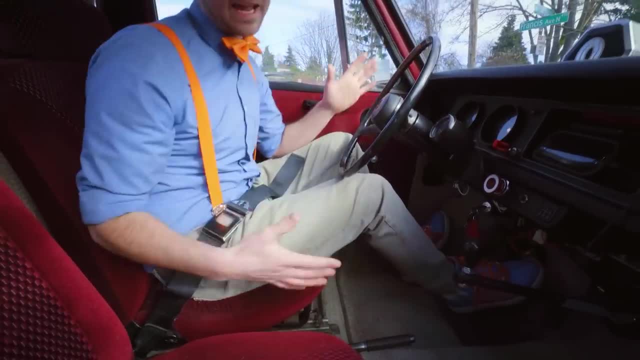 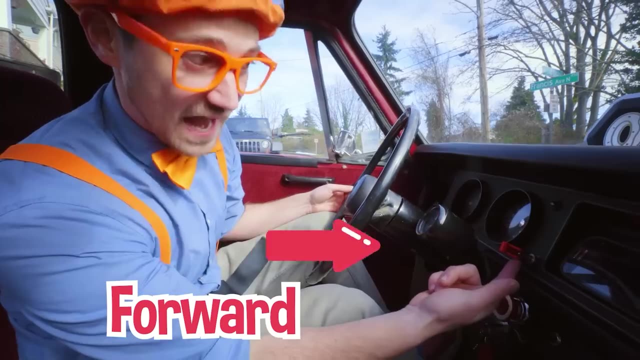 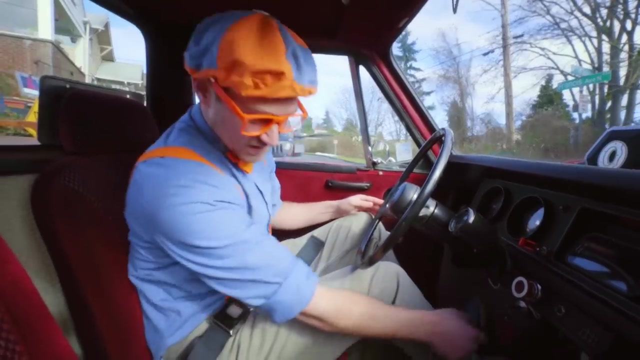 released this and didn't have my foot down there. then we started to roll. Okay, This is how you go forward And that is how you go backward. Whoa, Whoa, That is really cool. And then, just like a normal vehicle, we have a key down here. Wow. 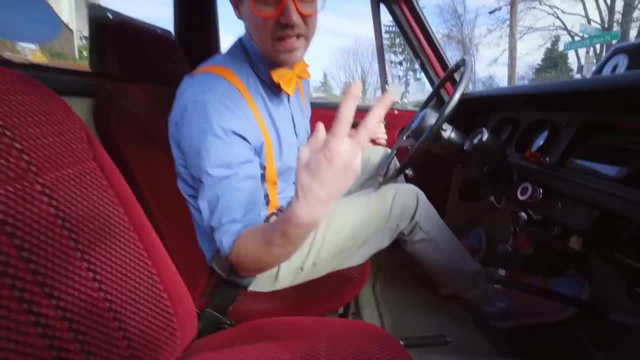 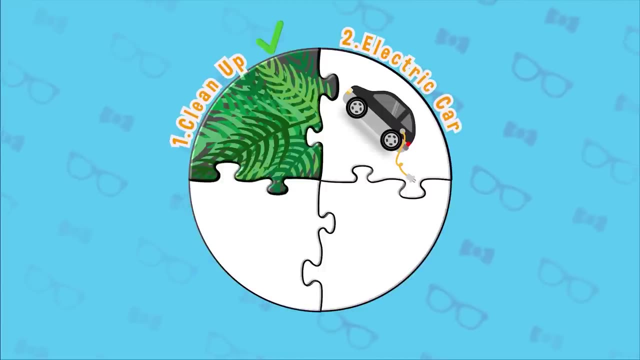 This is to change the gears. There's only two gears in this vehicle. Wow, This is such a really cool vehicle. We finished step number two on our great green adventure. That electric car is good for the environment and definitely helps with pollution. 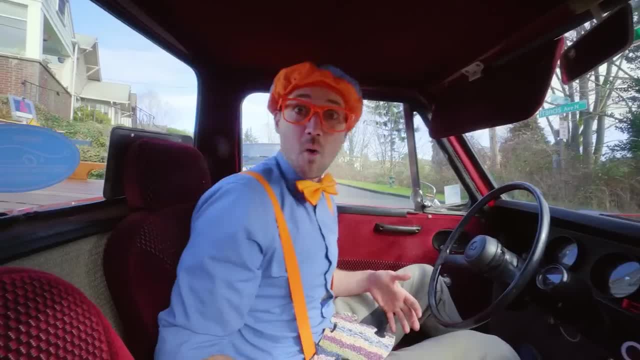 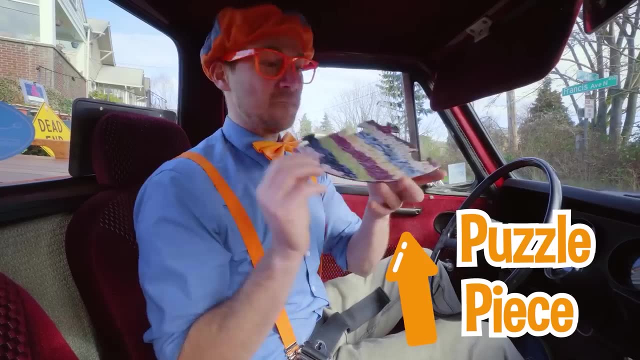 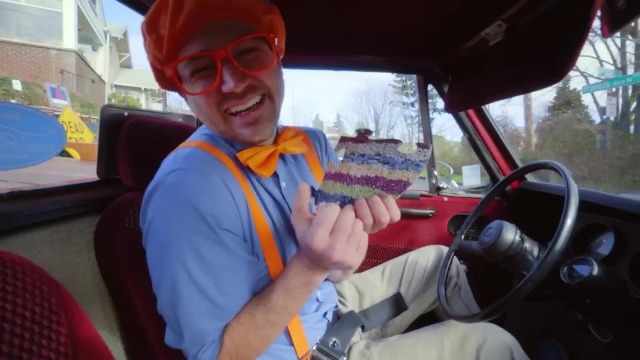 Hey, that was fun. Whoa, What was that? Whoa, Yeah, A puzzle piece. Whoa, And this puzzle piece has seeds on it. Whoa, Good job. Let's add it to our great green adventure puzzle. 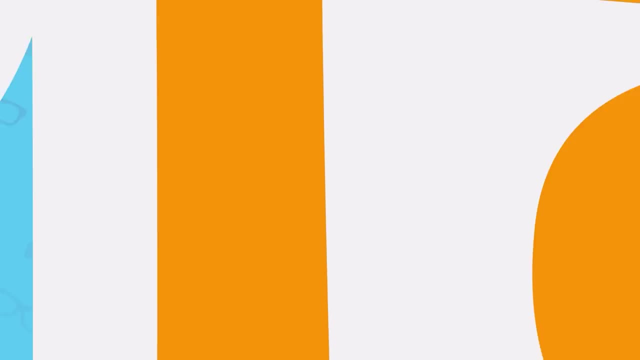 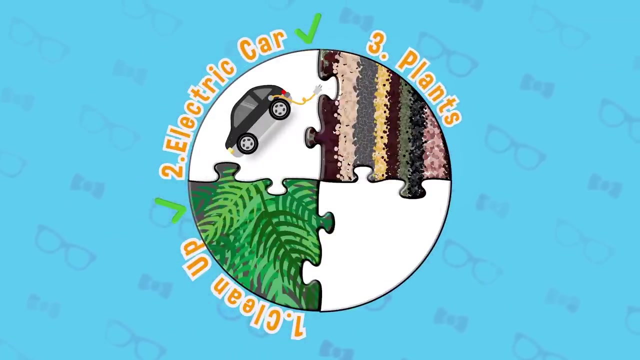 Step number three on our adventure, let's learn about seeds and plants. Did you know that plants come from little, itty bitty baby seeds? Yeah, that's right. Then they grow into big and tall plants that help make the oxygen we breathe. So plants are really important to a healthy earth. 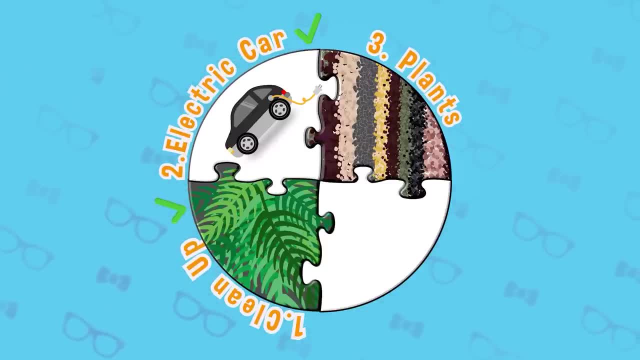 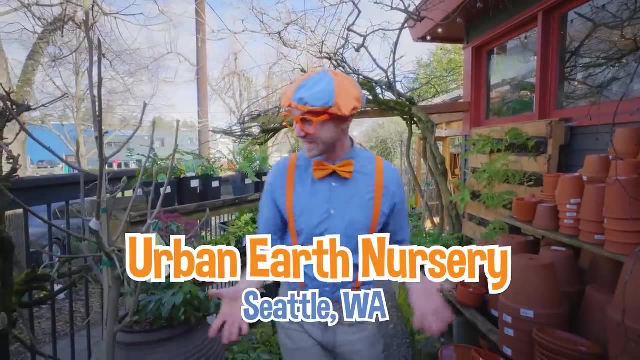 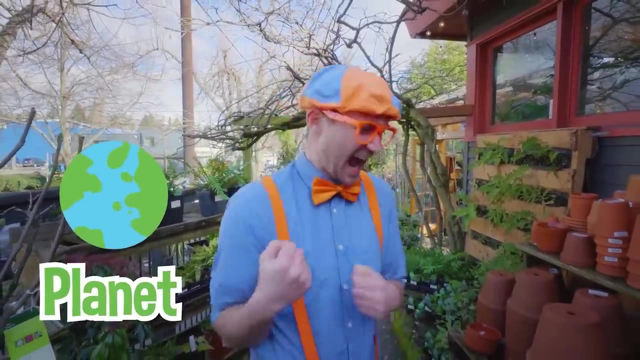 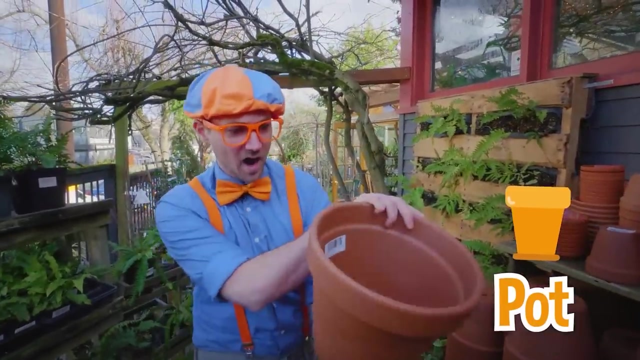 Let's go check some out. Check it out. I'm at Urban Earth Nursery in Seattle Washington And this place is so awesome. There are so many plants here, and plants are great for our planet. Whoa, Check it out. Whoa, This is a clay pot. Whoa, That's a really big pot And this is. 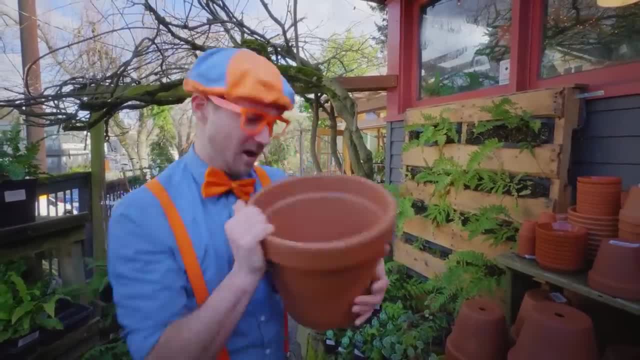 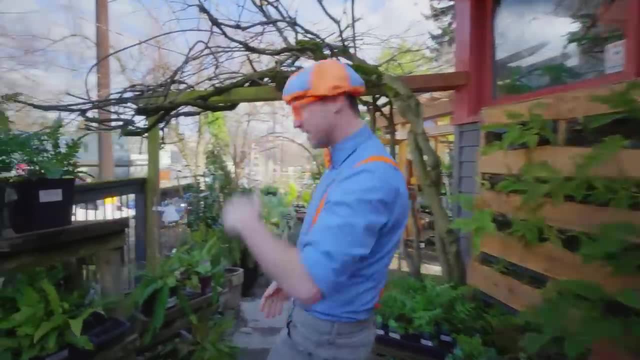 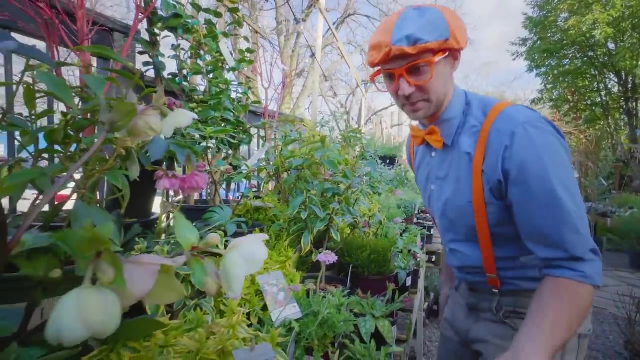 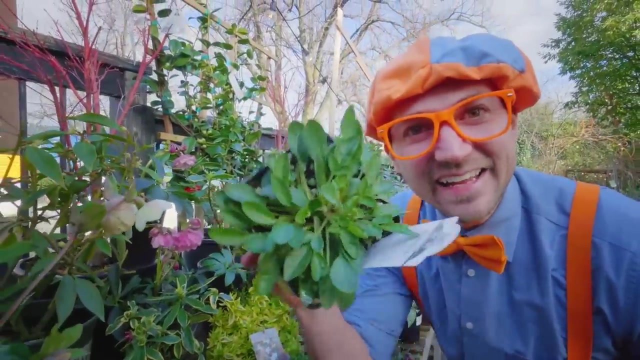 what you can plant some plants in. Hello, All right, Put that back right there, Let's go. Wow, I love all these plants. They're so colorful. Hey, what color is this plant? Yeah, it's the color green. Whoa, Hey, and check out this. 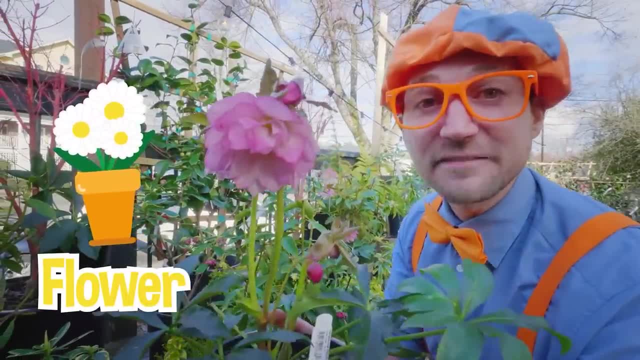 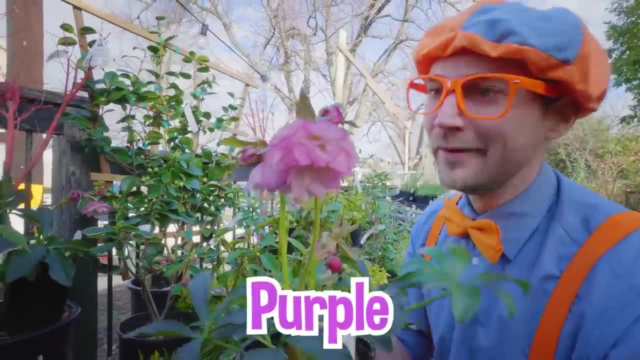 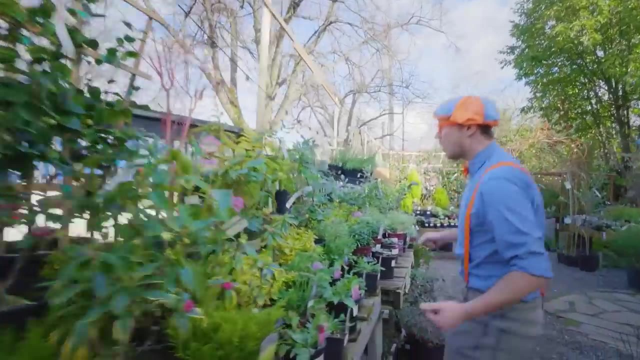 This is a flower. Do you see what color that flower is? Yeah, it's kind of like a pinkish, light purple. Let's just call it pink with white. Oh, so pretty, Wow, Oh, look at all of these. 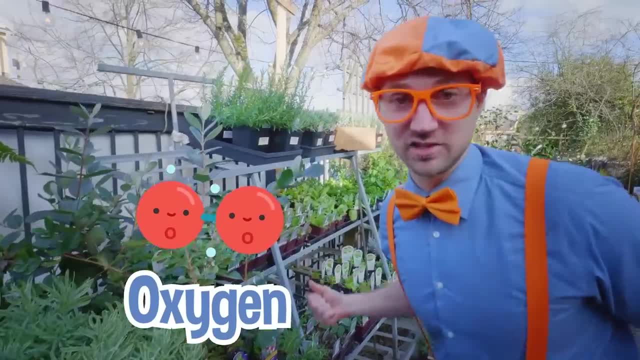 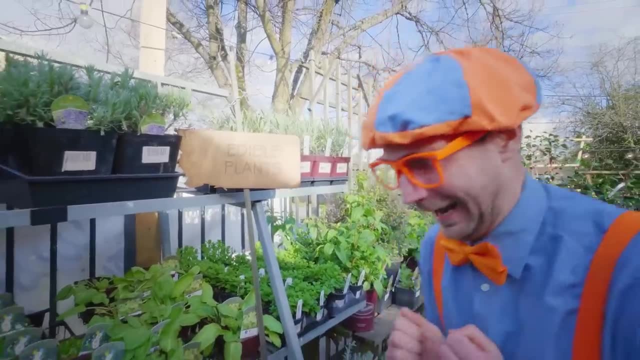 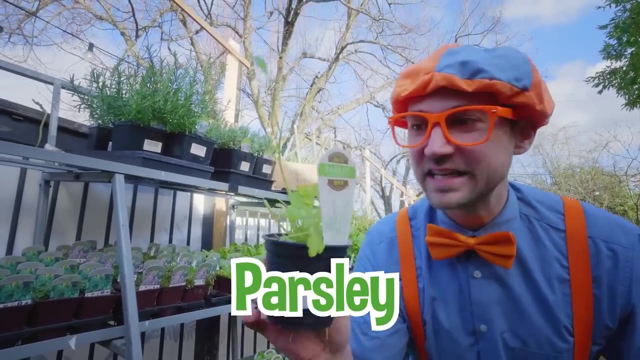 I love plants because they bring so much great oxygen to our planet. Oh hey, these are edible plants. That means you can eat them. Yum. There's a lot of herbs here like this. Check it out, That's parsley. 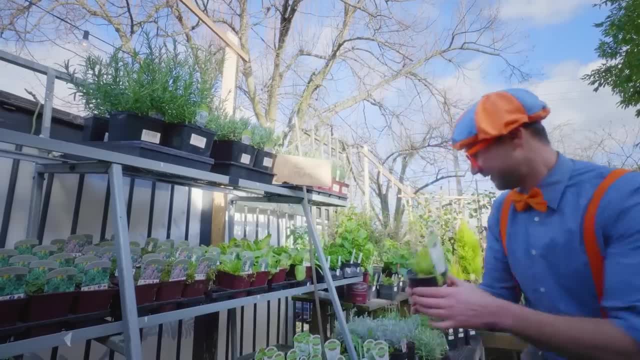 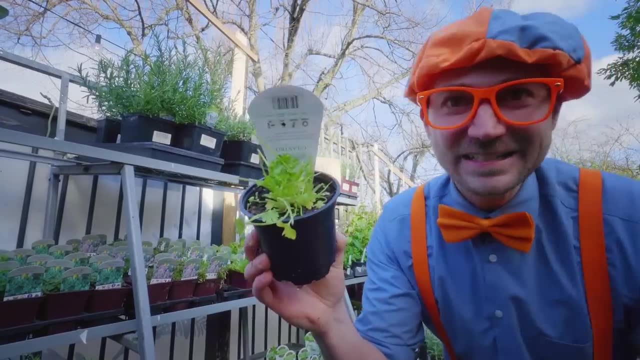 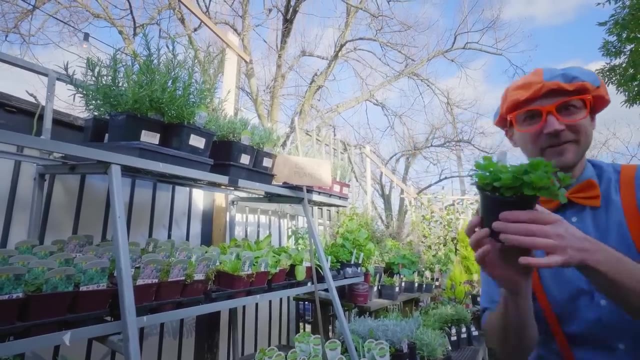 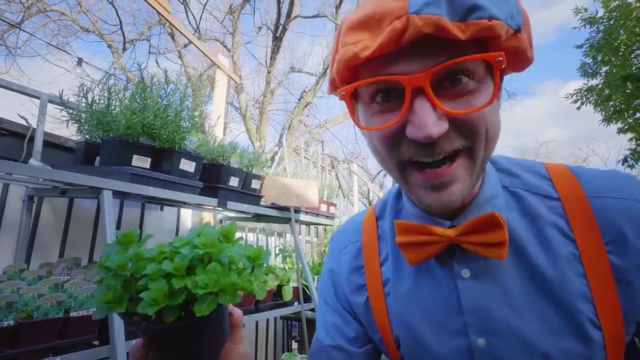 Yeah, you've probably had that in some of your food before. And then some cilantro- Oh, looks like a little animal ate some last night, Wow, Oh, and look at that, Looks like we have some mint. Smells minty fresh. 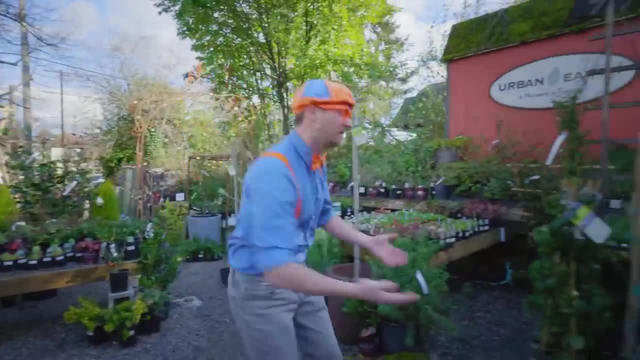 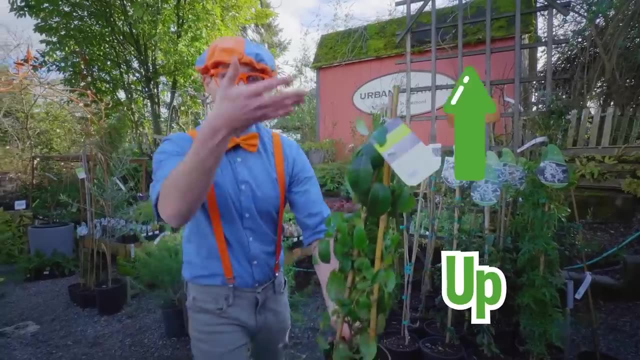 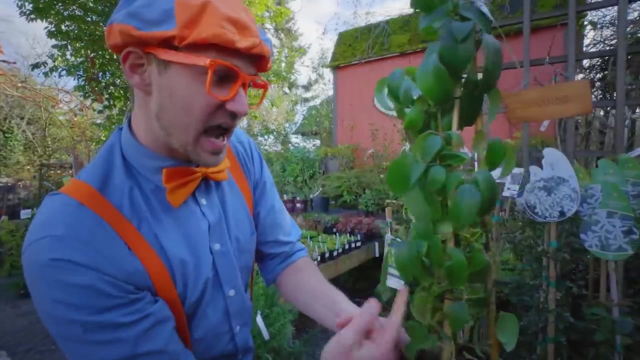 Hey, Looks like we have some vines. Vines are cool because they grow up. Yeah, They go around and around and they grab onto things. Wow, Look at it. You see how tall this plant is. It's because it's wrapping itself. 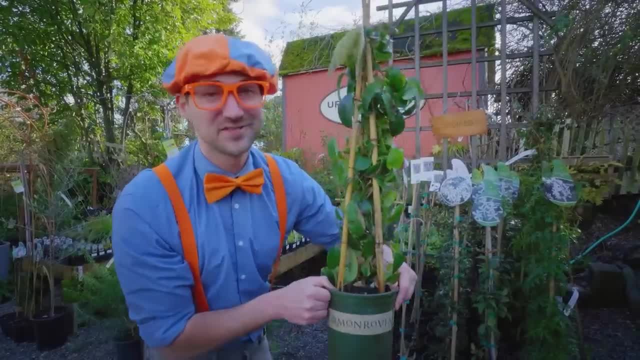 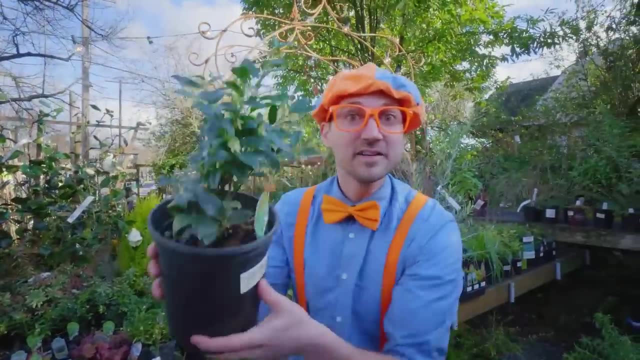 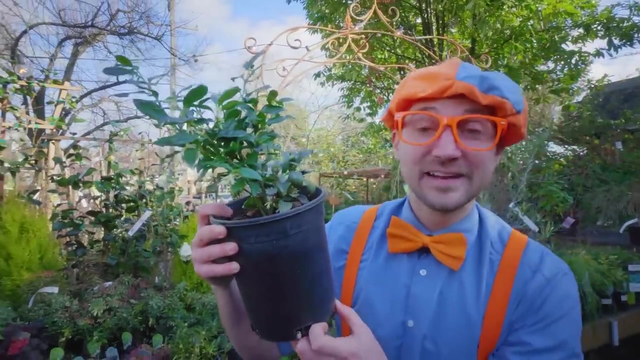 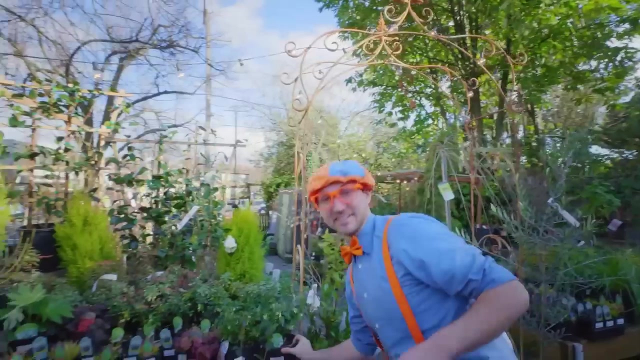 around these pieces of wood. That is really cool. What a smart plant. Looks like we have some sweet box. Sweet box. Yeah, sweet box is a great plant for hummingbirds. They love to eat this plant. Yeah, Well, the nectar at least. 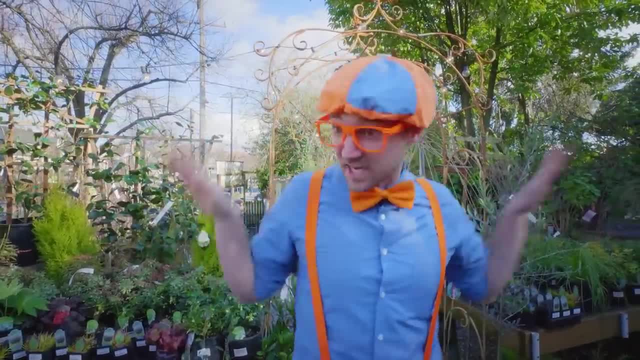 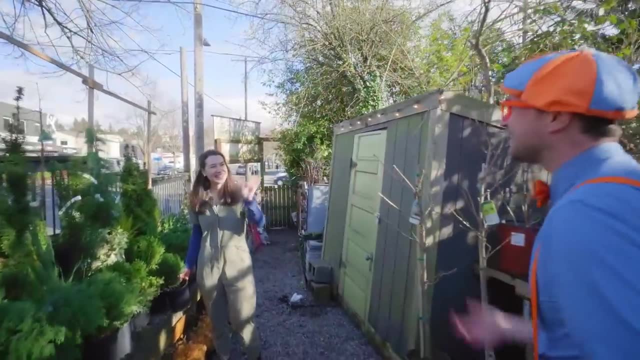 And did you know hummingbirds can flap their wings so fast? Oh look, there's a person. Hey Hi, Who are you? My name's Katie. Oh, nice to meet you, Katie, I'm Blippi. What are these? 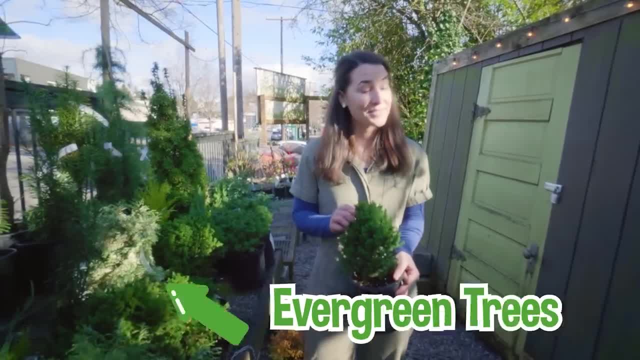 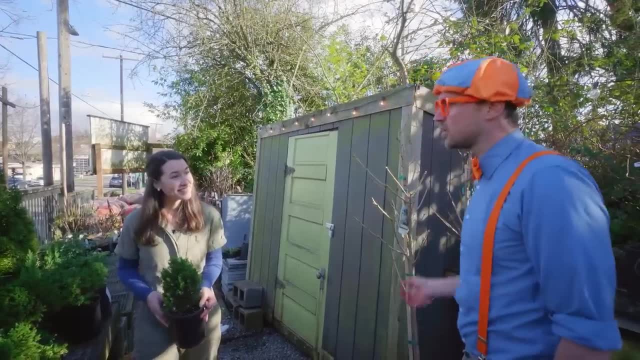 These are evergreen trees. Whoa, That means they keep their leaves or needles all year long. Wow, Wow, Wow, Wow. What lucky trees. Well, hey, I have a question: Do you know any place around here that I can plant some plants? 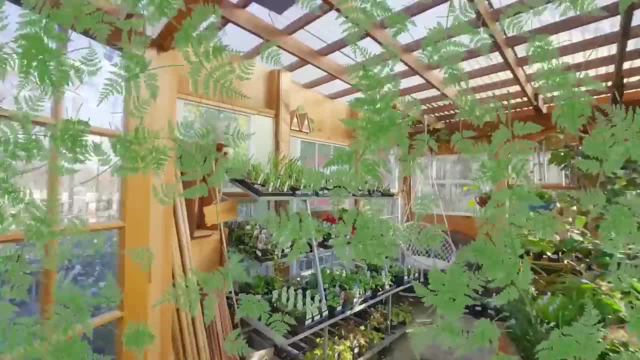 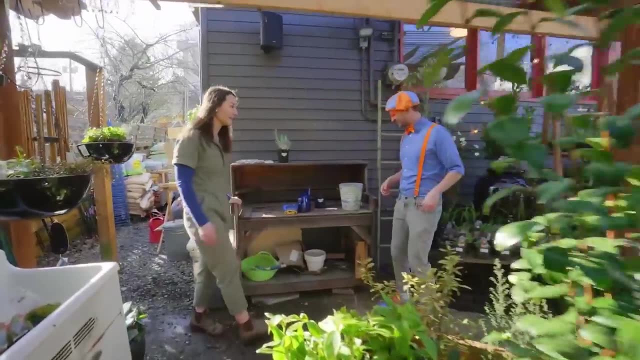 I do Follow me. All right, Here you go. Blippi, Here's a great place to plant some plants- Cool, Awesome. Well, thank you so much. Yeah, Do you know what you're doing? Yep, I think I got it. 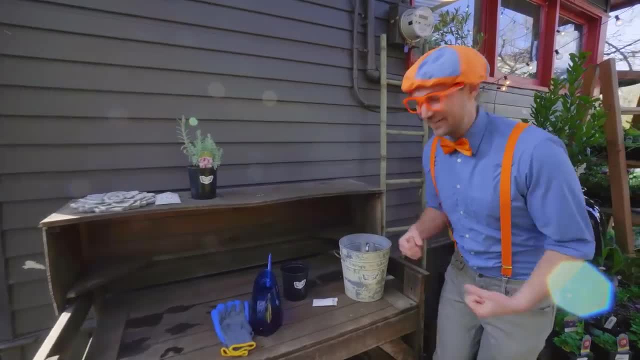 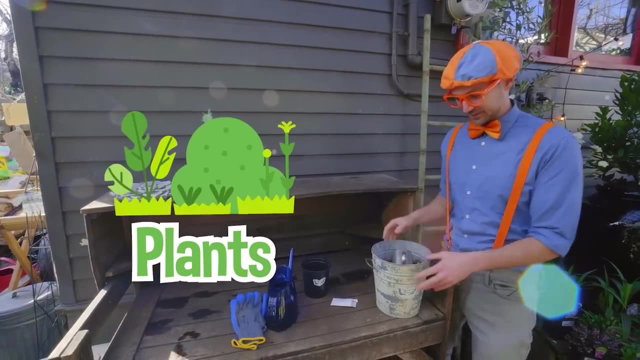 Thank you. All right, Have fun, See you. Wow, I am so excited. OK, So it looks like we have all the things that we need to plant some plants. Looks like we have a lot of soil- Whoa Wee. 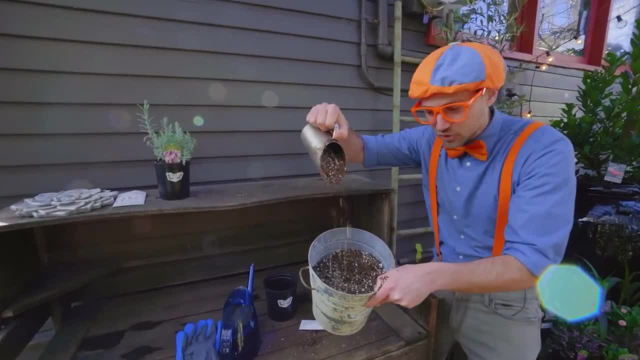 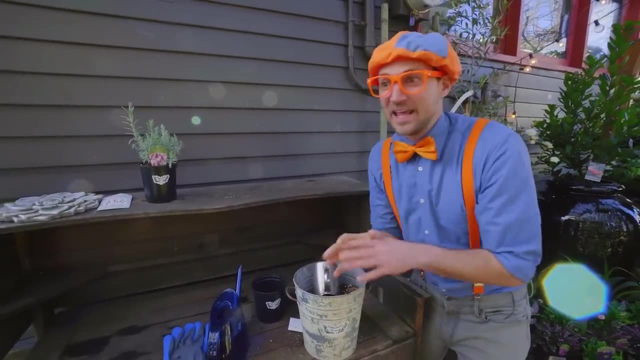 Yeah, and this soil is packed full of organic nutrients. Wee Whoa soil is so fun. I love adding water and then it gets all muddy and it's so fun to splash and play in. But today we're planting plants. 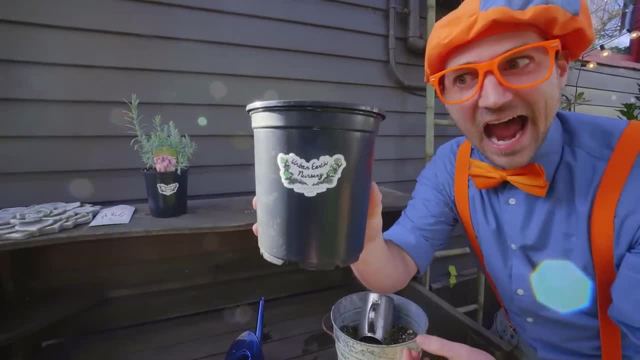 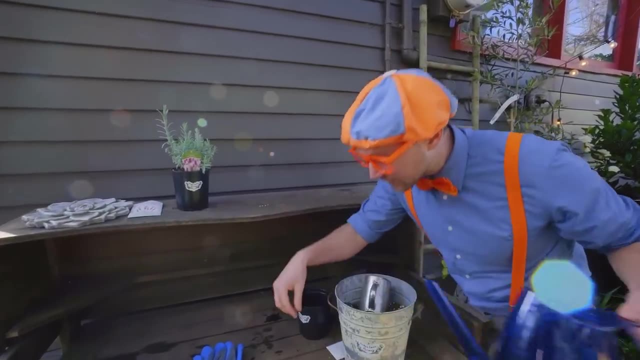 OK, And then we have a little container. OK, And then we're going to put some soil in the container. Yeah, And then what we need to do is put some soil in the container And then, after we put the seeds, oh, there they are. 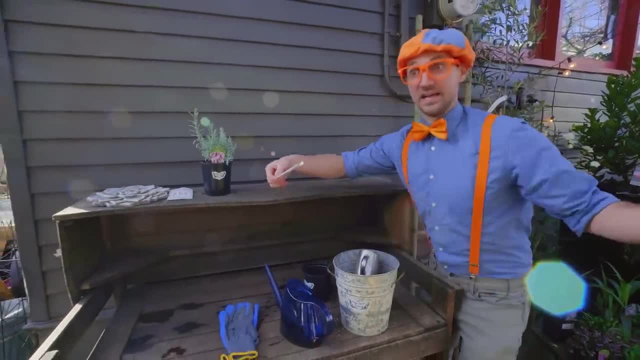 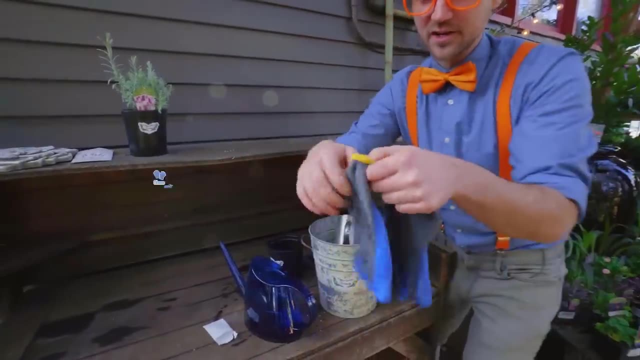 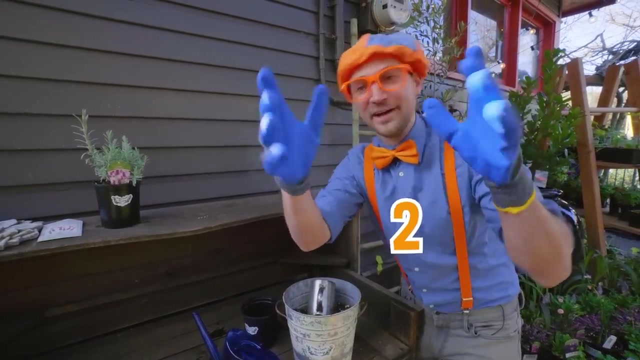 the seeds in the soil, then we water them, and then sun goes on it and then the plants will grow. OK, So let's do that now. First, let's put on our gloves: One glove on, Two gloves on. 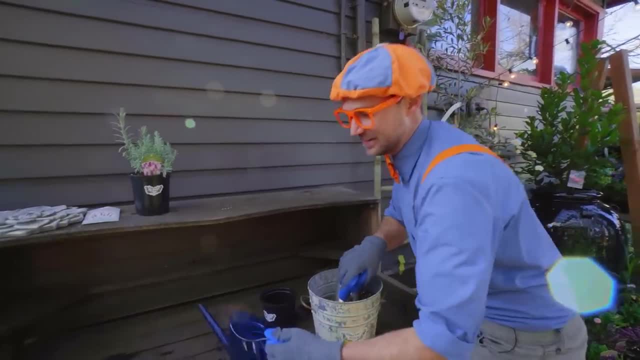 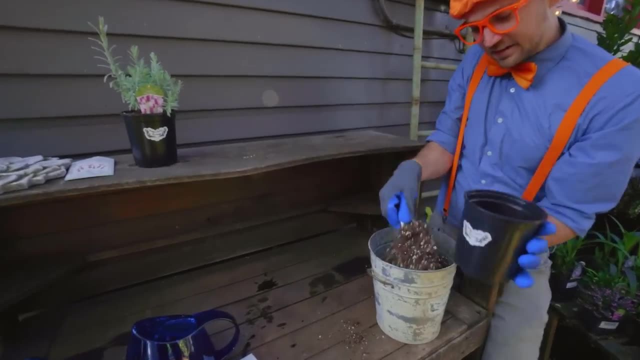 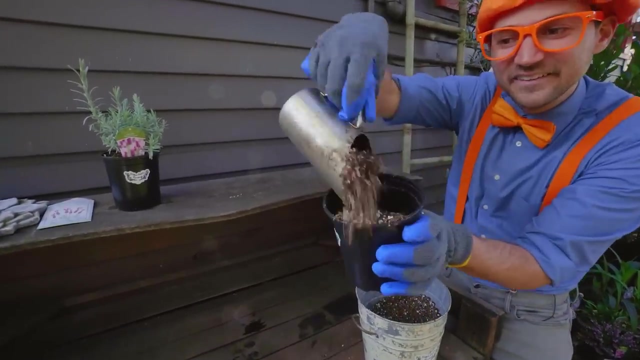 Ha, So now I won't get dirty. All right, Put that over there. Whoa, All right, Let's take our container and fill it up with soil. There we go. Three scoops filled up this container, All right. 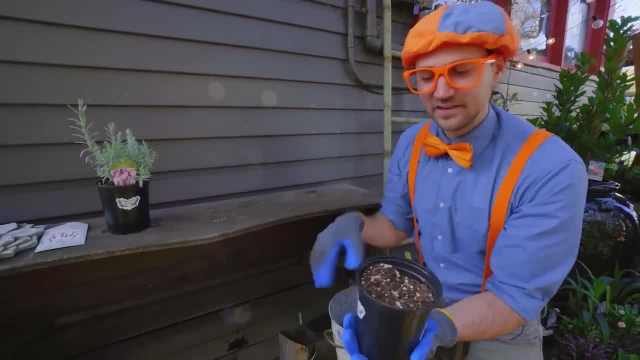 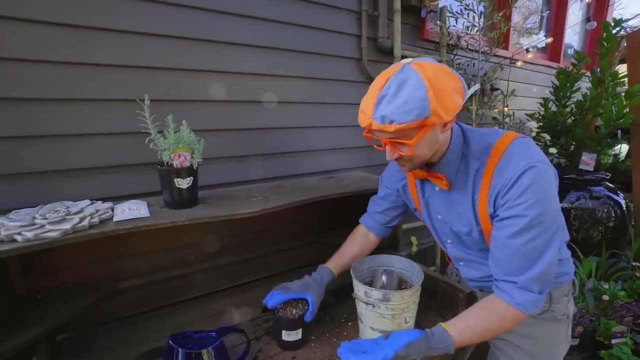 Now, let's pack it down just slightly. There we go, Actually, let's add a little bit more, All right, So now what we're going to do are take these seeds and put them in the holes that we poke in there. OK, 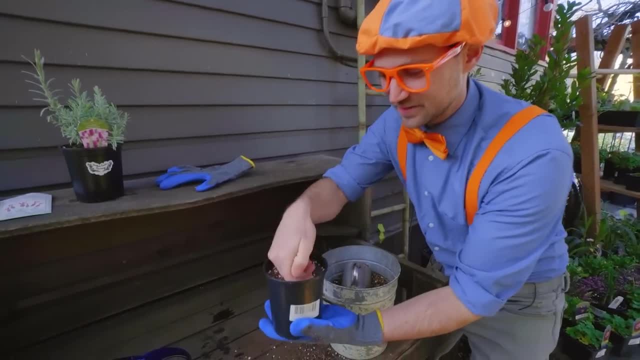 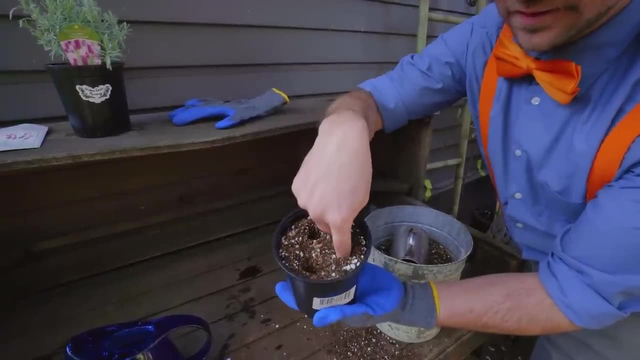 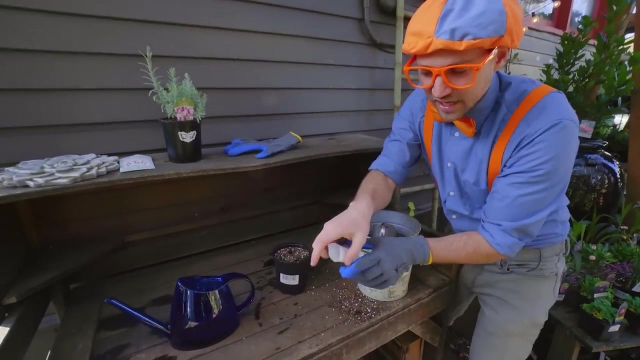 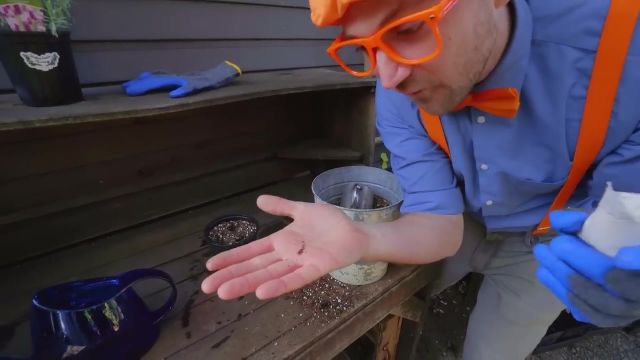 But for this I'm going to use my hand. So let's poke one hole, two hole, three holes. There we go, Perfect. And now check this out. OK, These seeds are so small. You see how small those are. 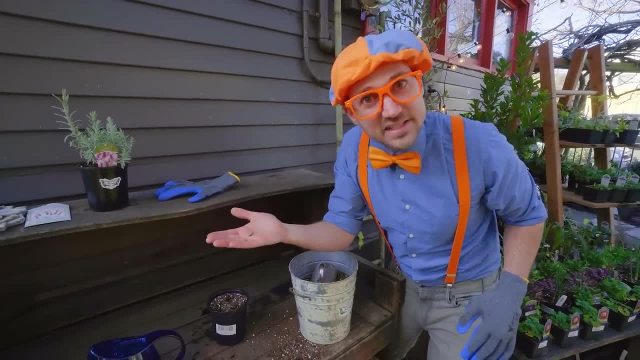 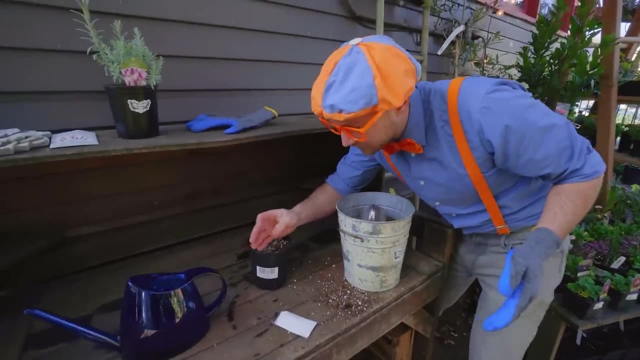 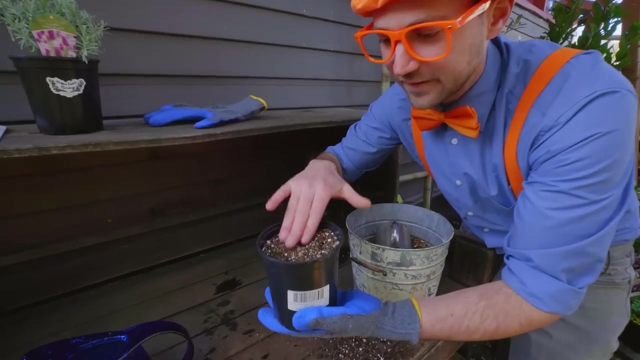 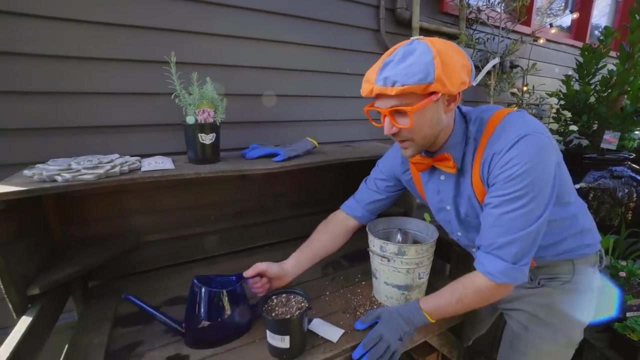 Wow, It is so crazy to think that these little seeds will grow into plants. There we go. Now, let's cover up the holes. Perfect, Now that there's seeds in there, covered up nice and gently. now, OK, We get to water it. 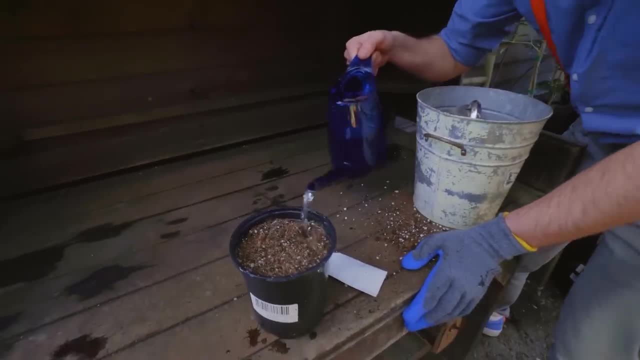 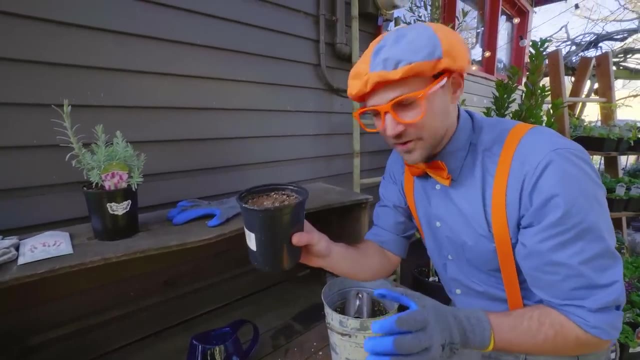 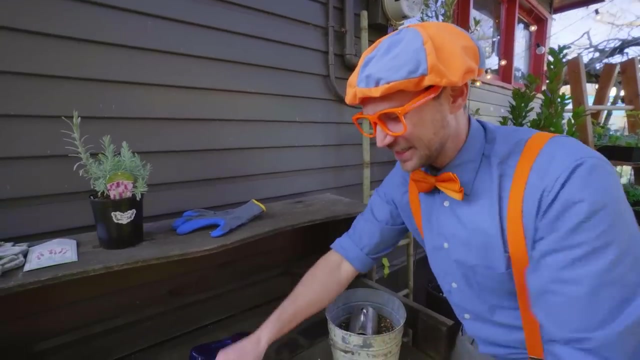 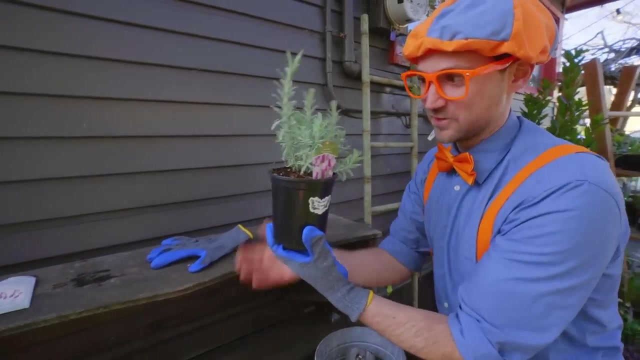 Wow, Perfect. Well now, have you ever wondered what seeds we just planted? Yeah, I didn't tell you, did I? Yeah, we actually planted lavender seeds. Oh, hey, check it out, And when those seeds grow up to get bigger, this is what we're going to do. 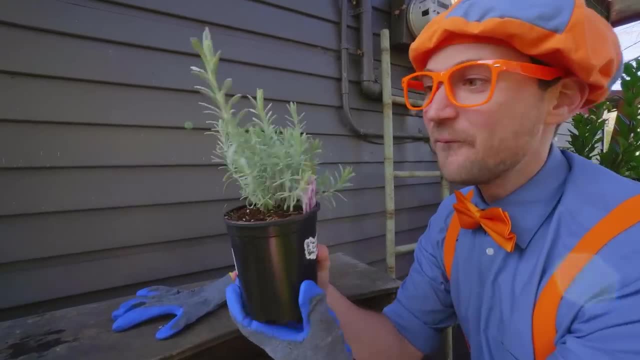 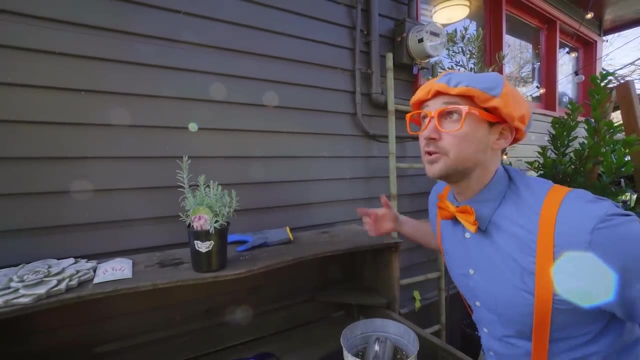 This is what they're going to look like. This is a lavender plant. Whoa Smells so good, You can eat it, And when it's spring and summertime it blooms into a beautiful plant like this Whoa. I am so excited. 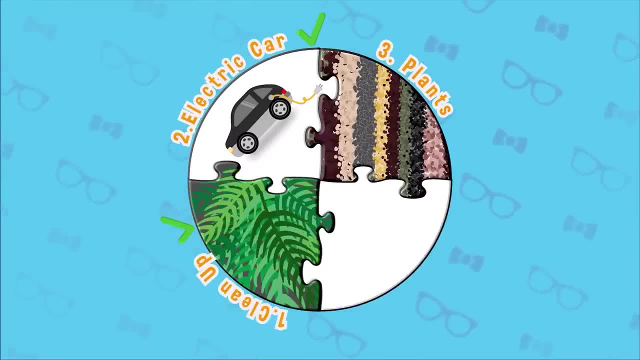 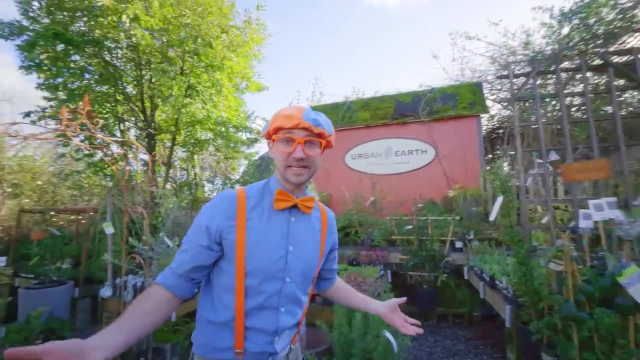 Hey, good job. Step number three on our Great Green Adventure Check. Our little plant will give the world some much needed oxygen that we breathe every day. Ah, Great, Great job. Woo hoo hoo. That was so much fun planting those seeds. 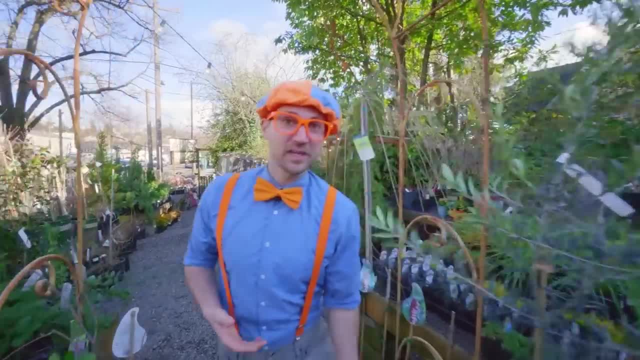 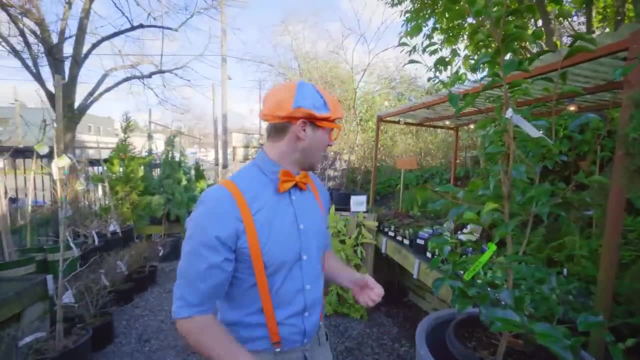 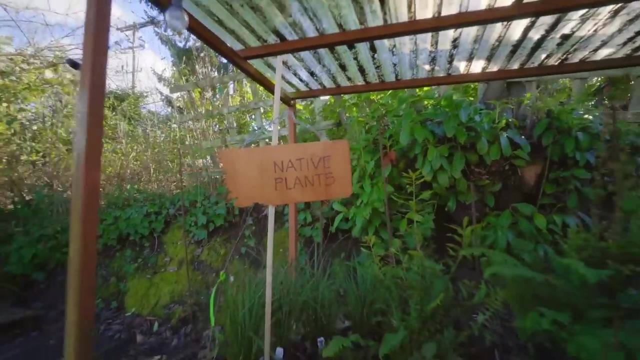 Well, hey, I think we should find some plants that we could go plant in the wilderness, and then we'll make our Earth even prettier. OK, Let's see. Oh Hey, This area is called the native plants area. Yeah, 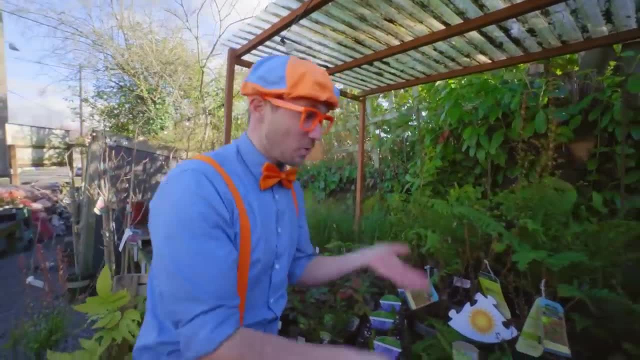 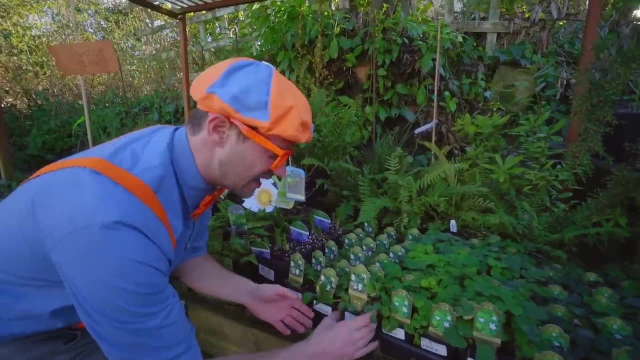 All of these plants are perfect for planting around here. Yeah, Which are plants that are native? They're native to where we're at right now. Wow, These look so cute. Oh Oh Yeah. The last puzzle piece. This is a picture of the sun. 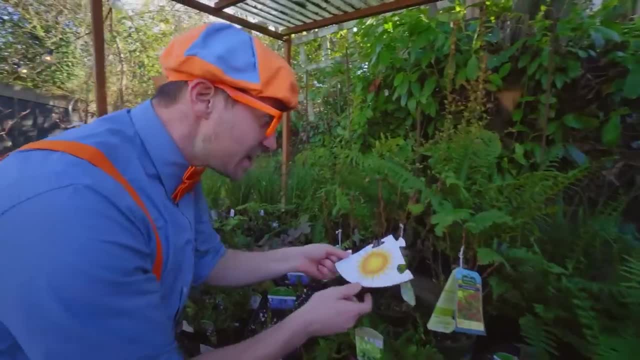 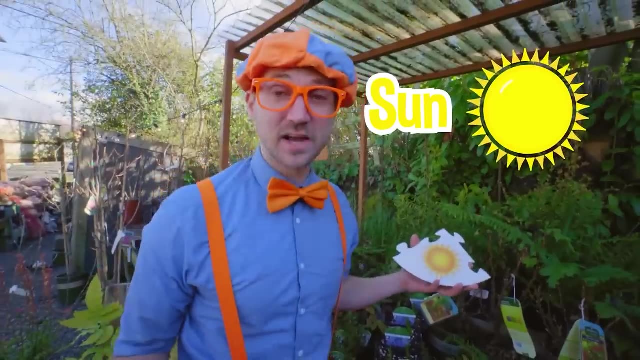 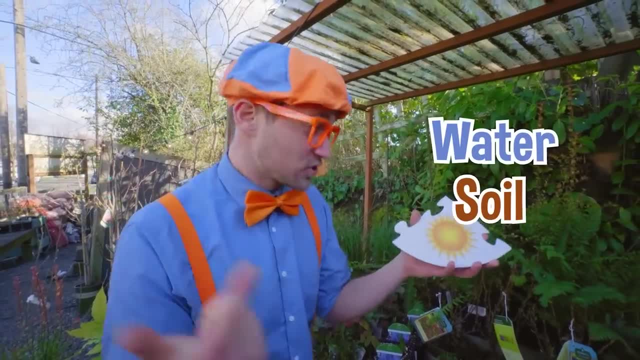 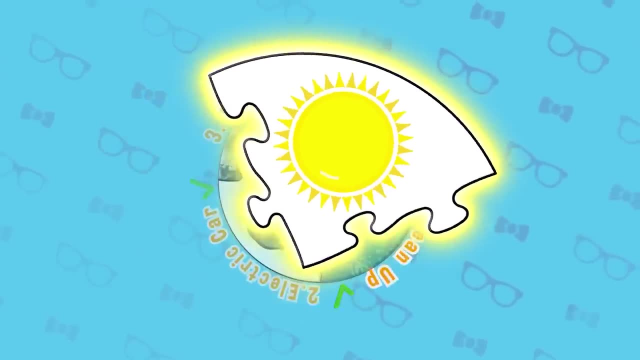 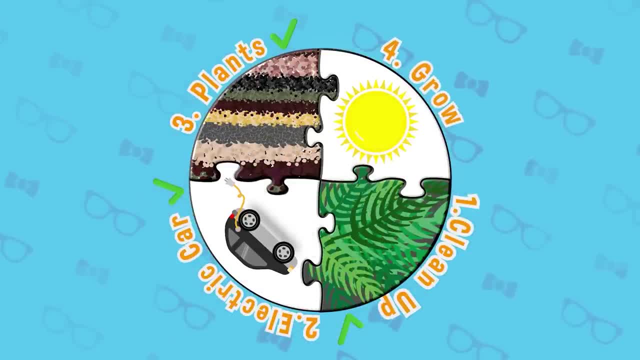 Awesome. Step number four on our adventure is learning how to help our plants grow. By giving our plants room to grow, their roots can spread and get even bigger. With the right amount of soil, water and sunlight, they'll grow up and get nice and 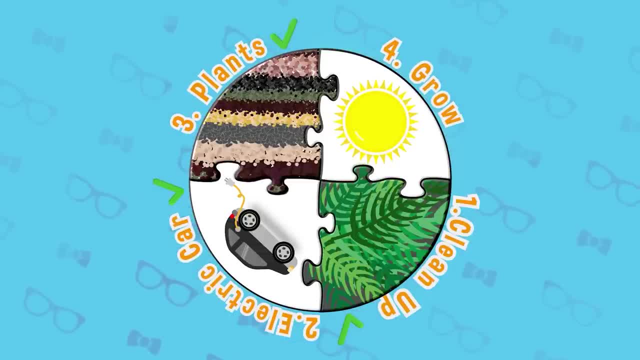 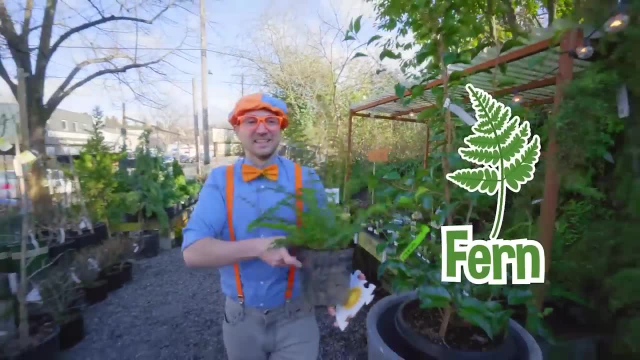 strong, Happy, healthy plants will make for a happy, healthy Earth. Let's grab one of these. Hey, This looks pretty perfect. This is a fern. Wow, this fern is great. Whoa, whoa, whoa, check this out. 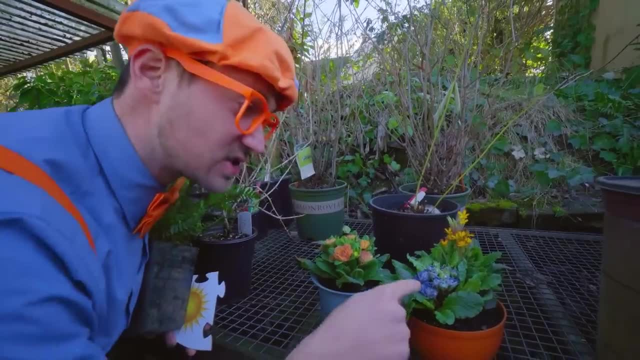 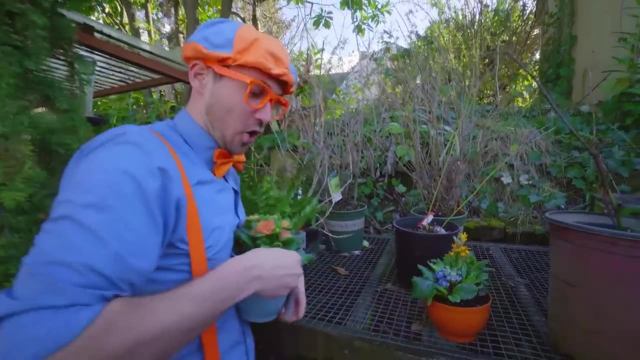 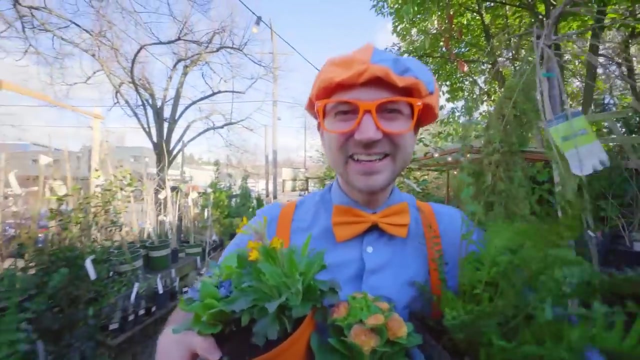 Yeah, my two favorite colors: A blue flower, Oh, and that's kind of orange, Whoa. I think we should totally take these as well And plant them. Yeah, good job. Right here on Earth, we have all we need. 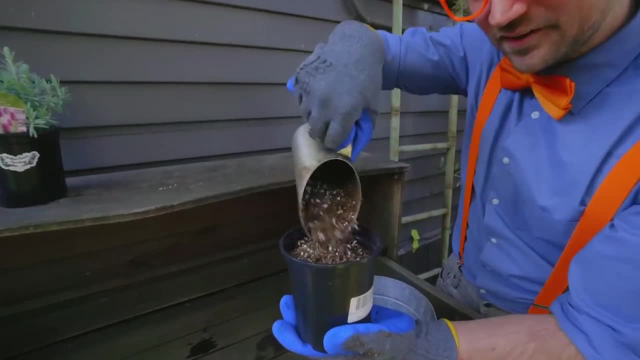 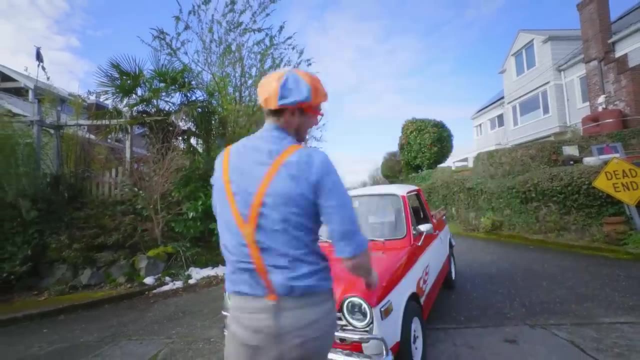 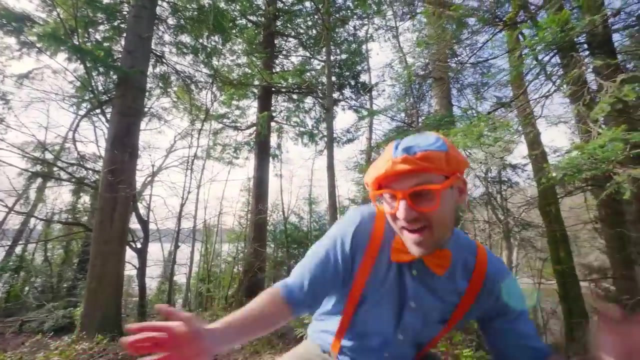 Our friend, our home. we plant the seed. From the air we breathe to the water we drink, to the land we live on, really makes you think. From the mountains high to way down below, we all share the Earth. now it's time you know. 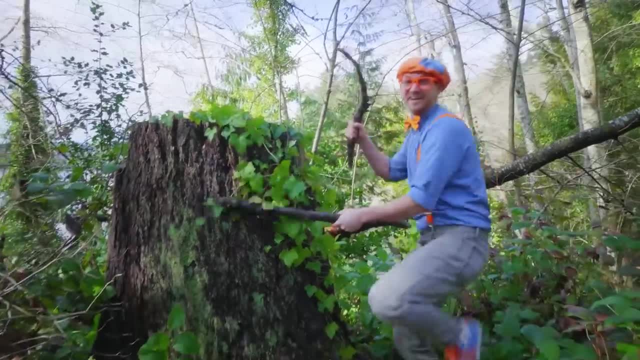 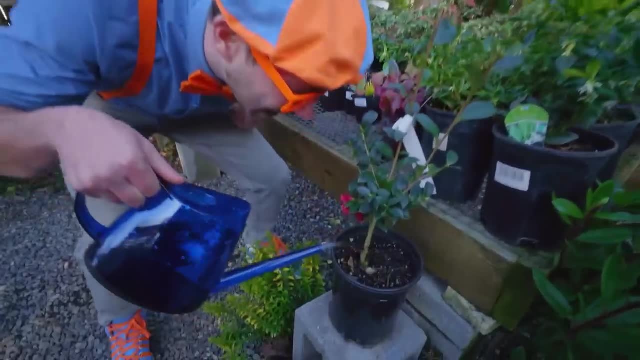 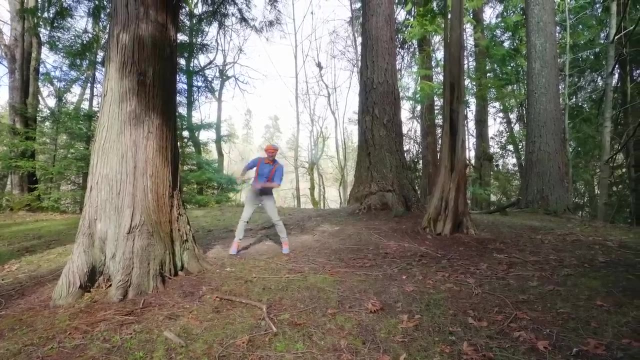 Respect the trees- they give us lots of air. Respect the creatures- give them lots of care. Respect the plants cause. they help us grow, Help us all to breathe. Respect the water, the oceans and seas. When we make a change, we'll see the worth. 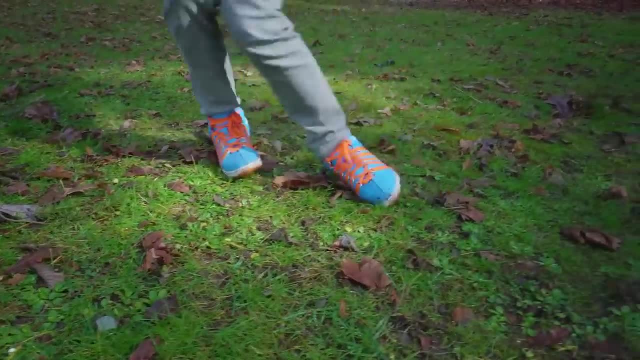 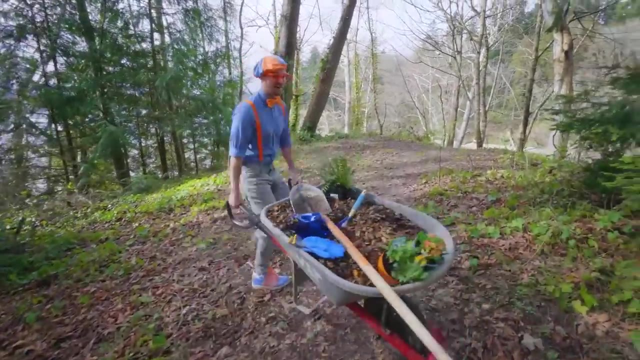 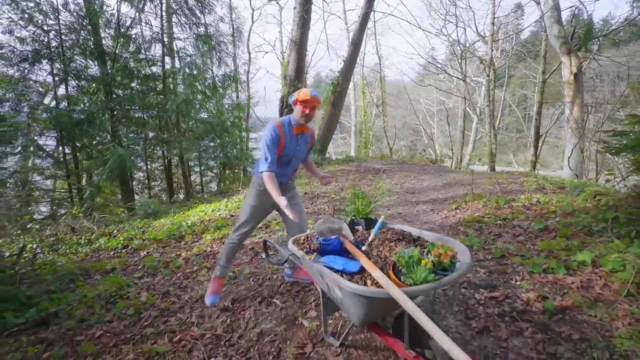 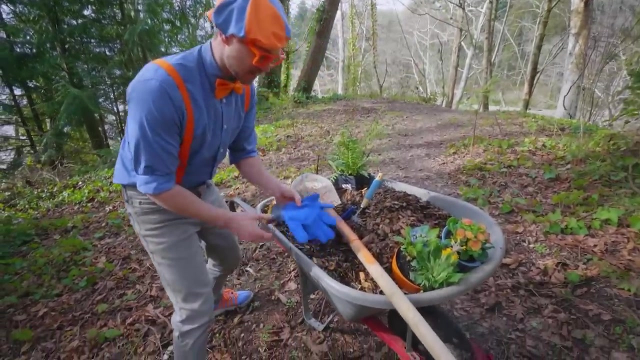 We all have to help and respect our Earth. Whoa, that was a big hill, And what I'm doing is taking all of these items up to the top of the hill and we can plant the plants. Hey, let's check out what I brought up here. 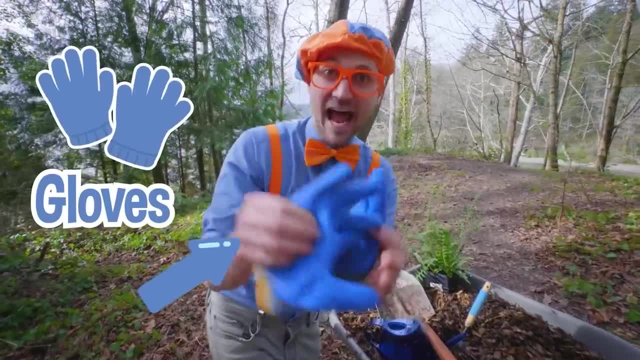 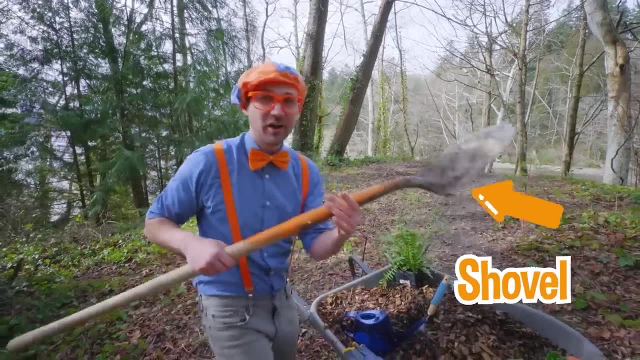 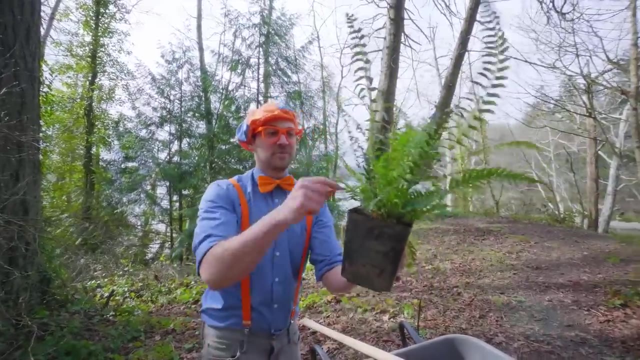 Yep, I brought my gardening gloves. Looks like I brought my big shovel. Yeah, so we can dig in the dirt. So then we can put our plant that we brought from the nursery into the hole, And this is a fern, And this fern is native to this area. 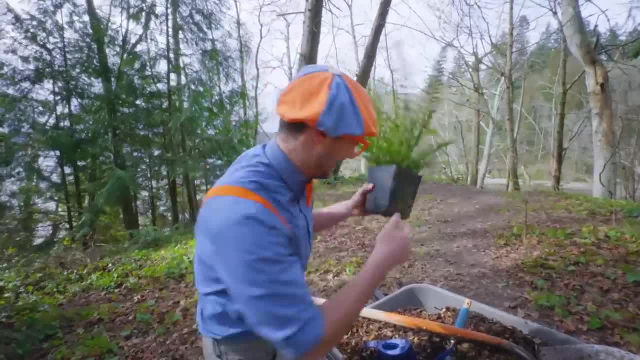 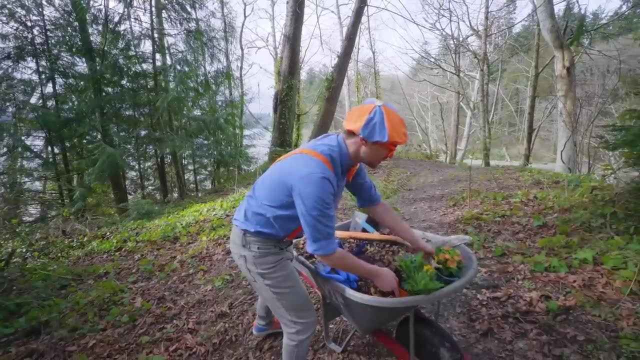 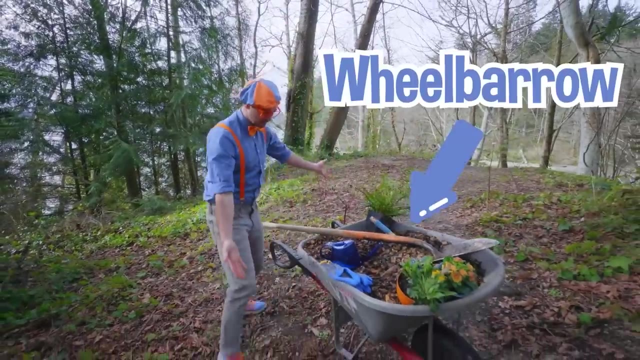 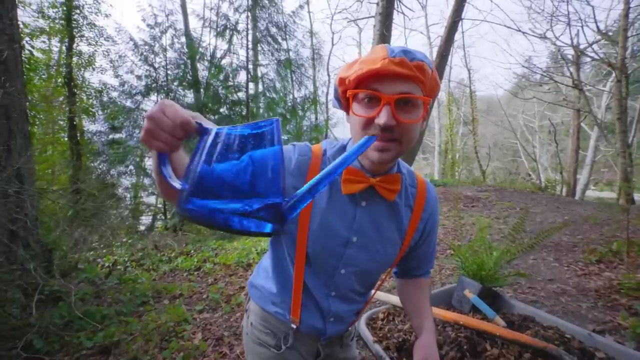 So it's gonna thrive, in this environment. Ooh, a little hand shovel, Whoa. And then the two cute flowers, So cute. Oh, can't forget about the wheelbarrow. Wow, Hey, and some water, Yeah, so we can plant. 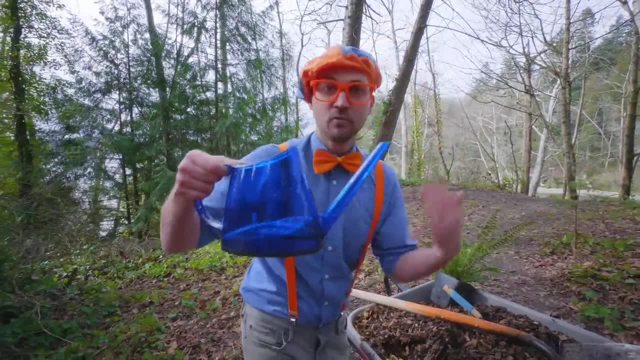 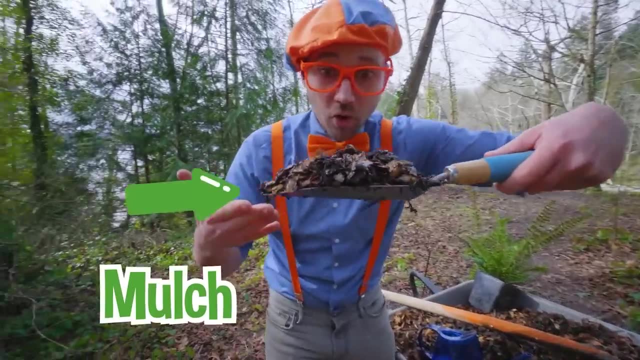 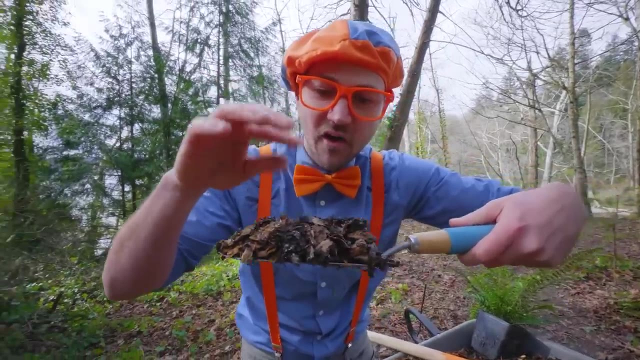 So we can water the plant after we plant it. Oh and last but not least, yeah, mulch. Whoa, check it out. Mulch is actually just chopped up pieces of bark. Yeah, check that out. Bark and wood and plants. 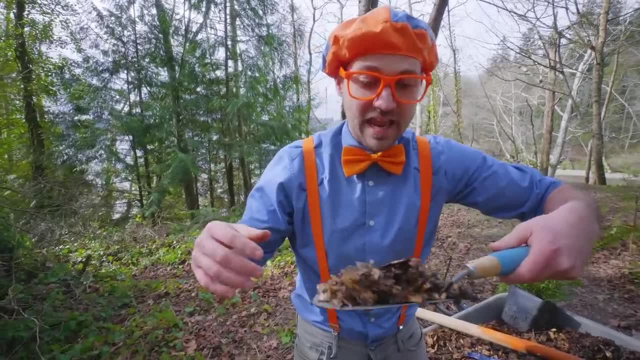 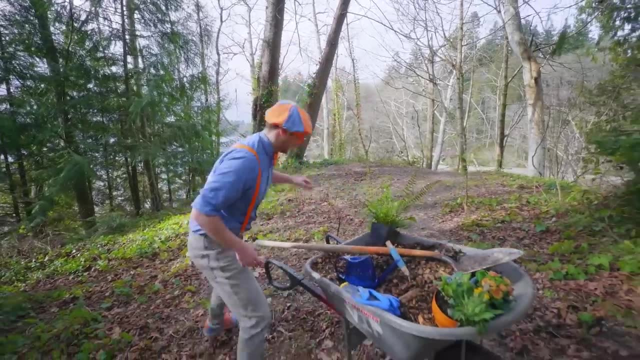 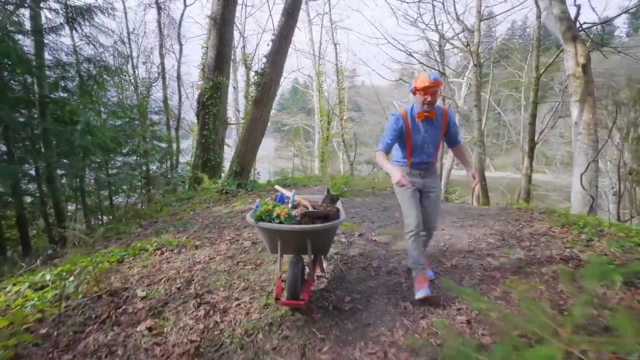 Yeah, it actually provides nutrients to the soil And also it helps make sure the soil maintains its moisture. Okay, let's get to planting. Whoa, whoa, whoa. Check it out. Do you see this tree? Oh, what a cute little tree this is. 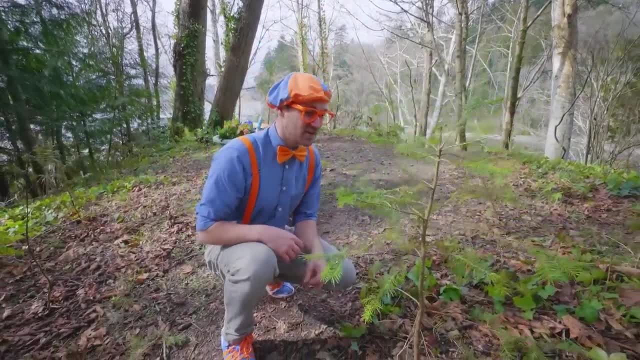 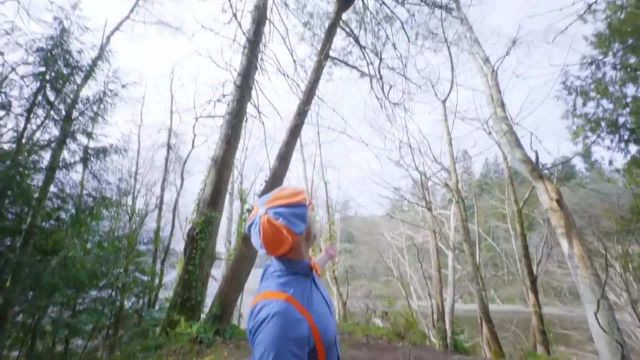 Hey tree, how are you? Thank you for being you, But hey, this is a young tree. It's really small, But check this out, Whoa, When it grows up it's gonna be really big, like that tree. 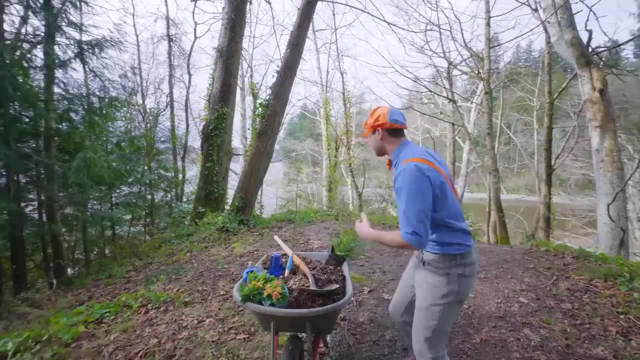 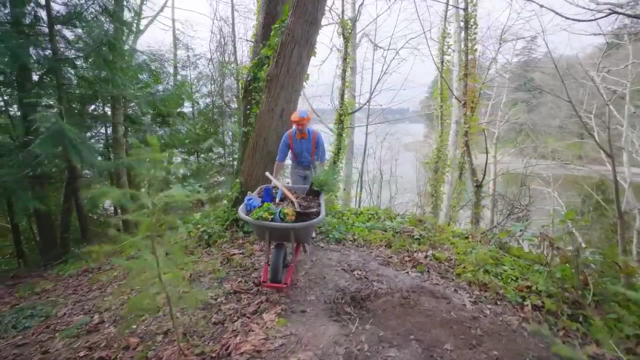 Wow, I love trees. They're so great for our planet. All right, let's see here. All right, Okay, first thing we need to do is find a great place for our fern. Let's see How. about right here? 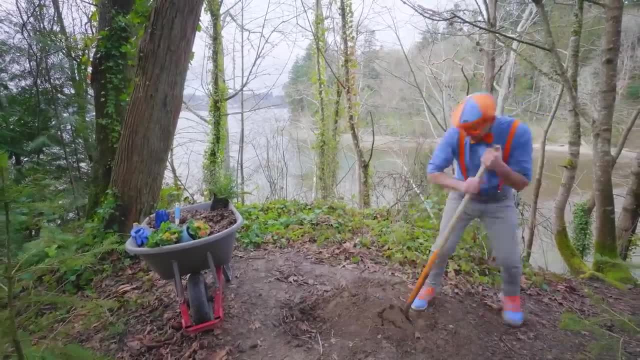 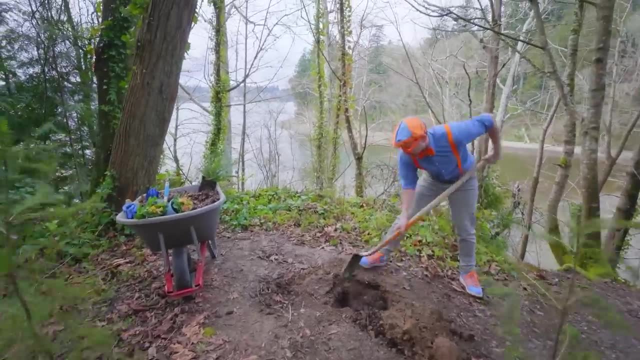 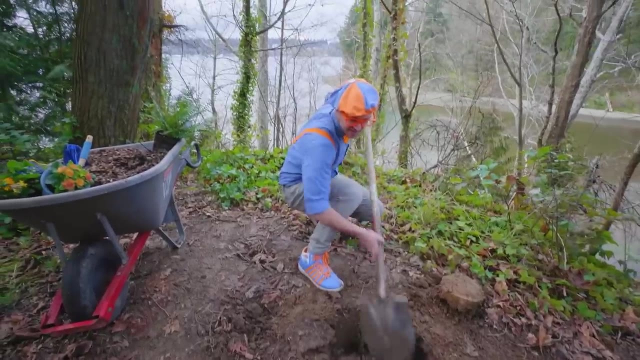 All right, Here we go, All right. So what I'm doing is making sure I dig a hole that's about two times the size of the fern's pot. Yeah, there we go. Perfect, That looks real good. All right. 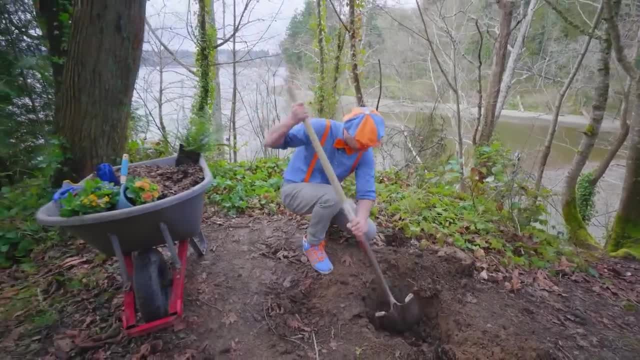 Hey, I'm about to get really messy, So let me put on my gloves. I probably could have put the gloves on before I used the shovel, But that's okay. Okay, There we go. Perfect, Let's take this fern. 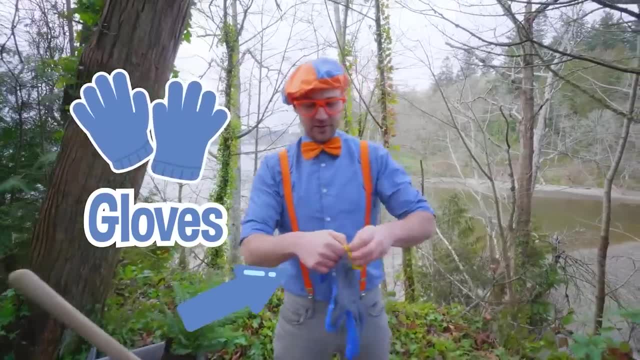 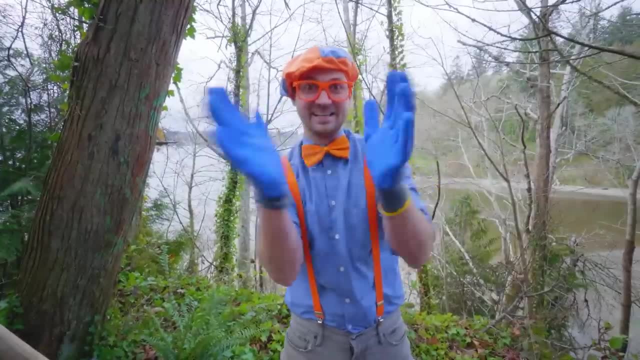 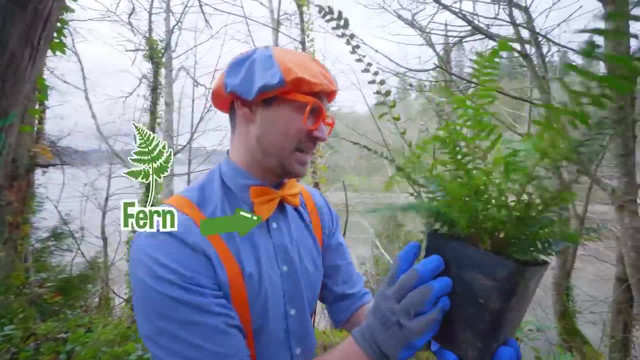 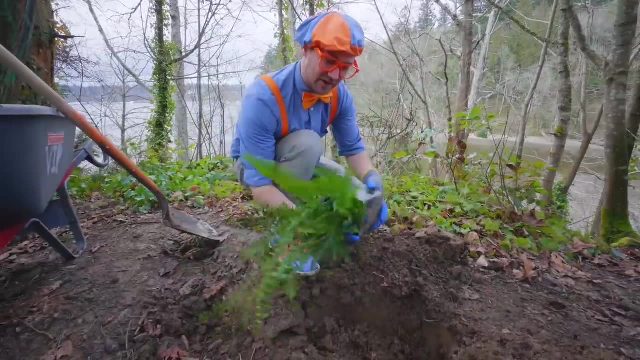 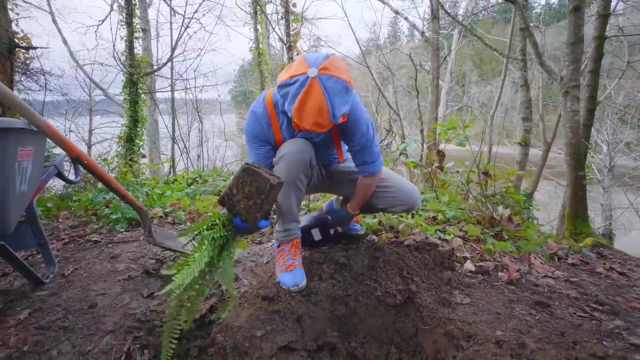 Look at that. Okay. So now that I have my fern, are you ready to be in your new home? fern, Yeah, Okay. So I'm going to be very careful and flip it upside down, Shake it. There we go. 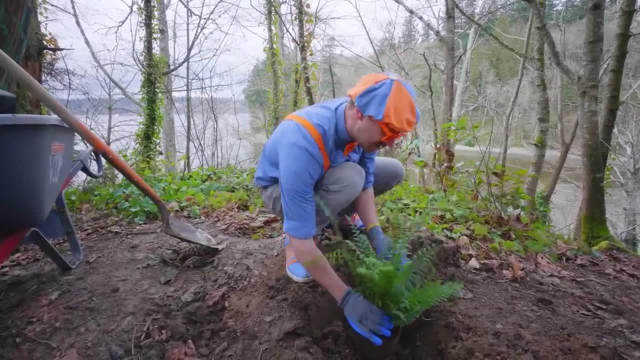 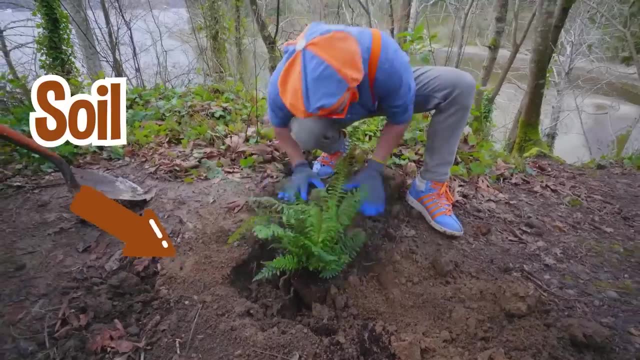 And then I'm going to place it nice and gently right here and put the soil back. There we go. See how I'm putting the soil all around the edges and the sides- Perfect, Wow. And I'm breaking up all the big clumps. 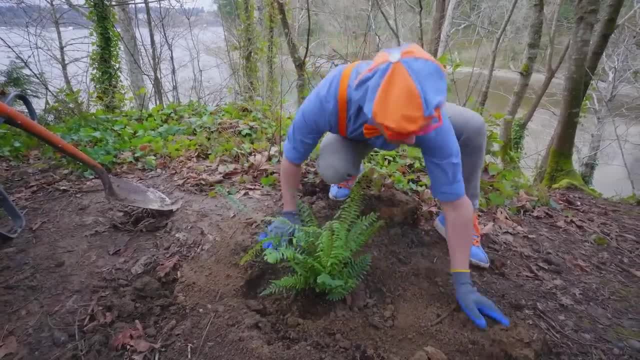 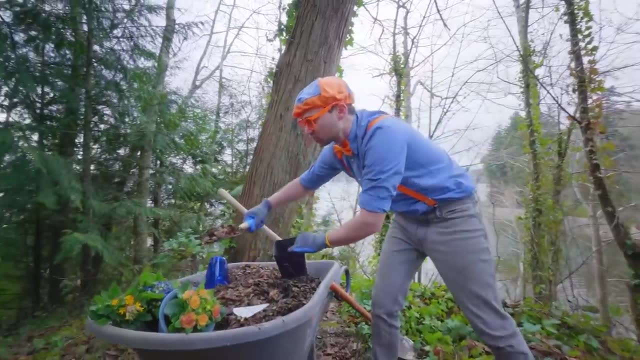 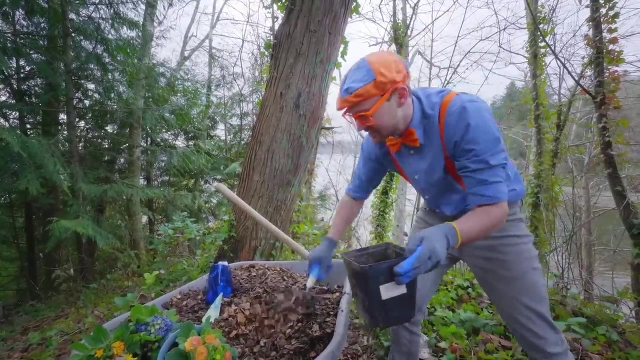 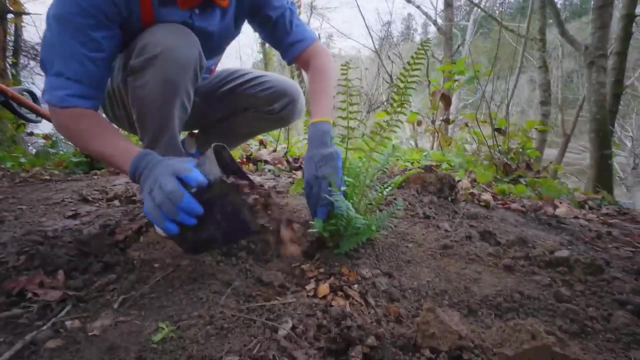 Wow, This fern is going to grow up to be really big and strong. Perfect. Let's scoop up a few scoops of mulch, put it in our little planter bucket And what we're going to do is put this on top of the soil all around the fern. 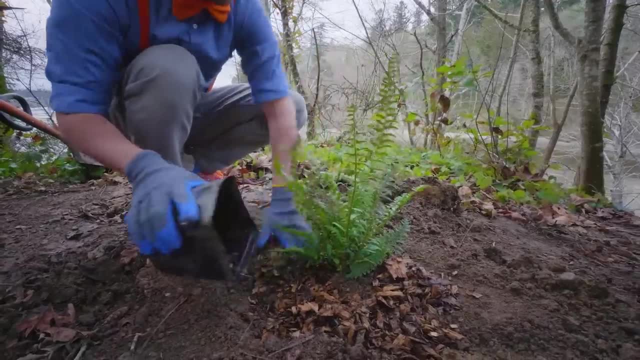 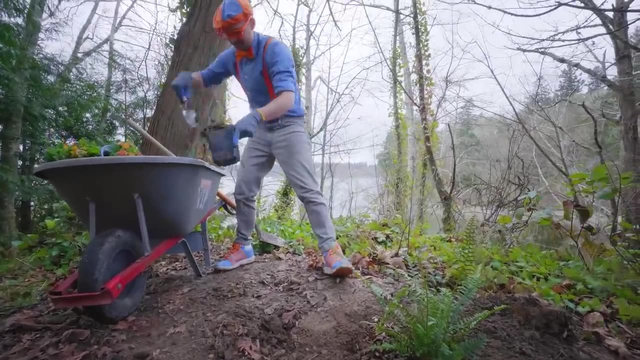 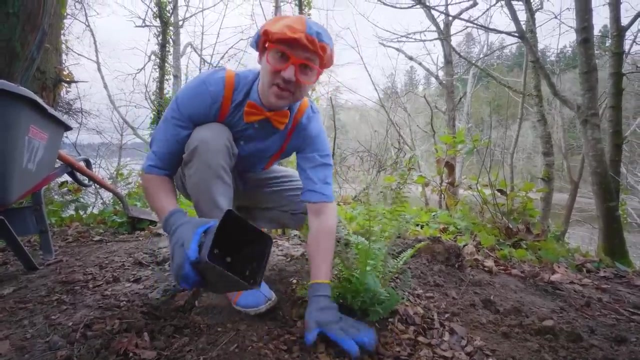 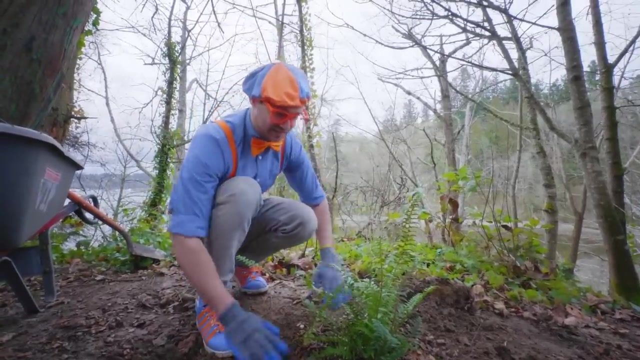 There we go. Perfect. Wow, Let's get a few more scoops. Wow, This is awesome. Good job. I love planting plants. Like I said, it's really good for our planet to be able to plant plants, Haha. 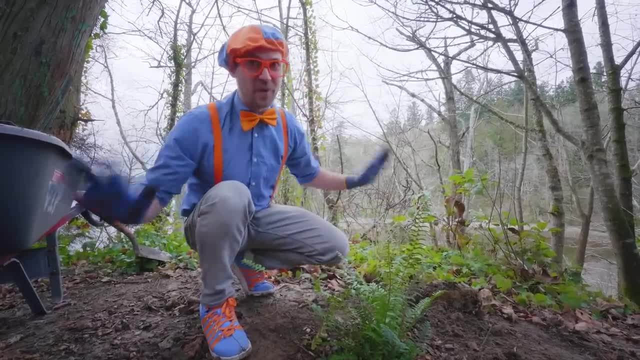 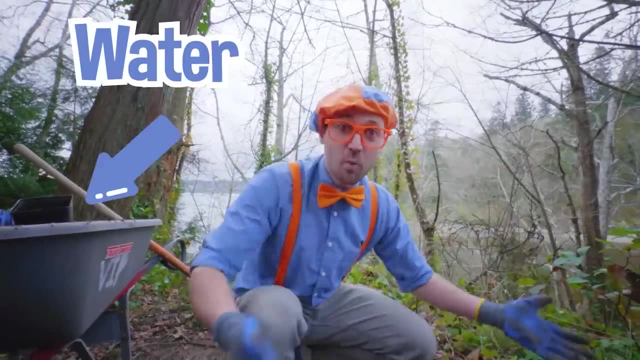 This is a native plant. Like I said earlier, it's going to thrive around here. But hey, what else do we need to do? Yeah, we need to water it. All right, Here we go. All right, Here we go. 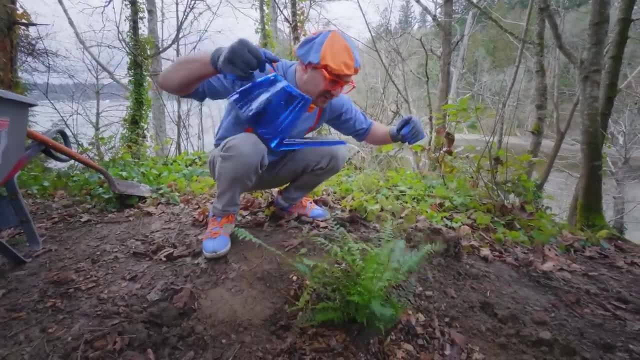 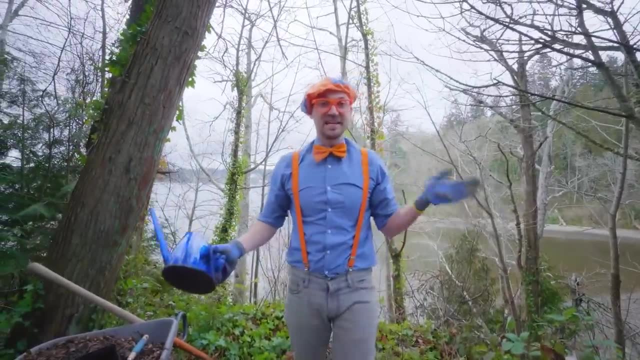 Here you go. Woo hoo hoo, There we go. That's a good amount of water for now, But since it's a native plant, yeah, the rain around here is going to be a little bit more rain, But the rain around here is going to provide a lot of water, so we don't have to come out. 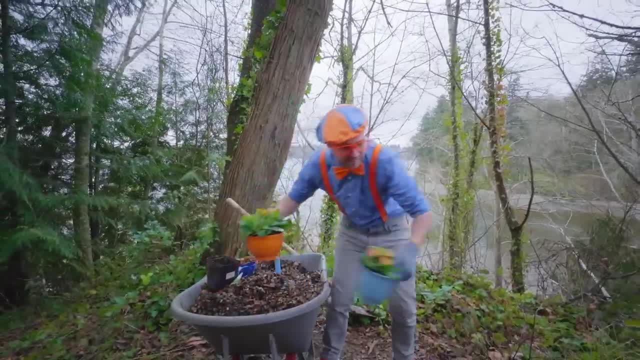 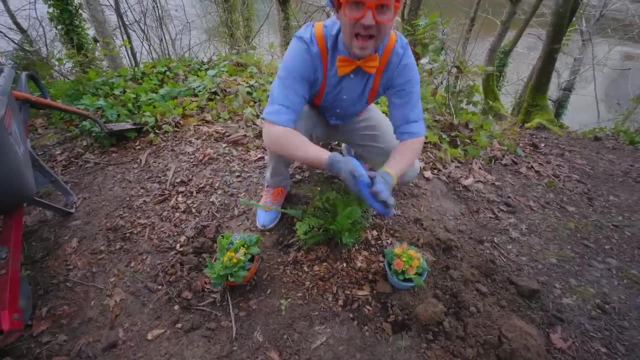 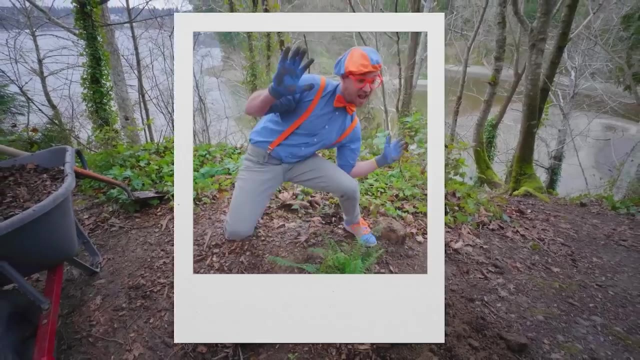 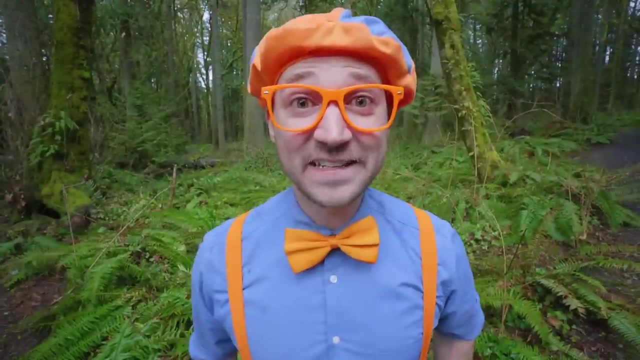 here every day to water it. Let's put these two plants around here, So then it looks nice and pretty. Wow, How does it look? Yeah, I think it looks so good. we should probably take some photos. All right, I have a fun game. 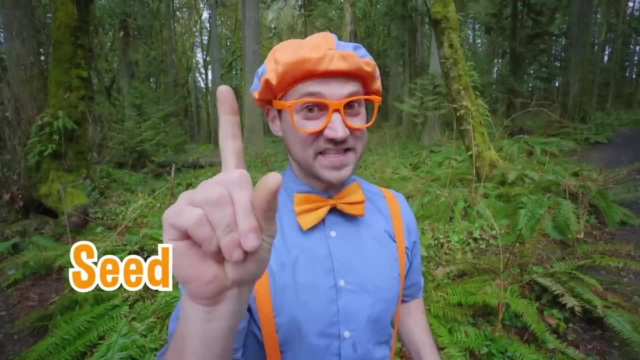 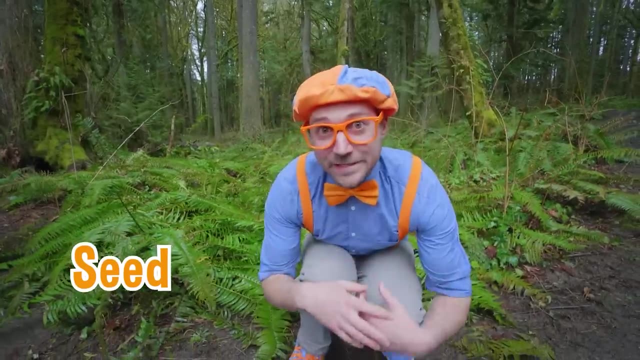 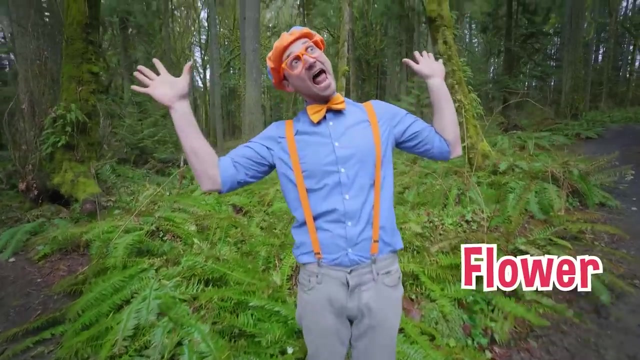 First, we're going to act like three different things: Seed, stem and flower Ready. First act like a seed: Get nice and small. Now act like a stem. And now act like a flower. All right, Here we go. 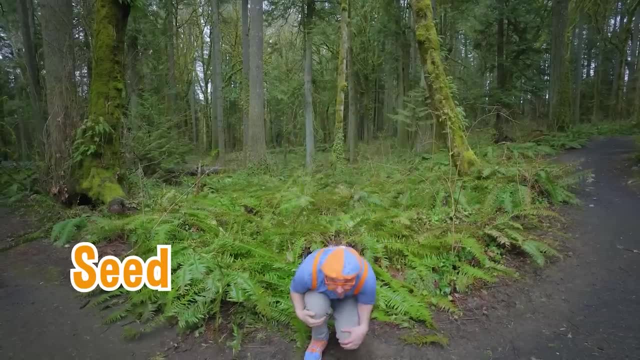 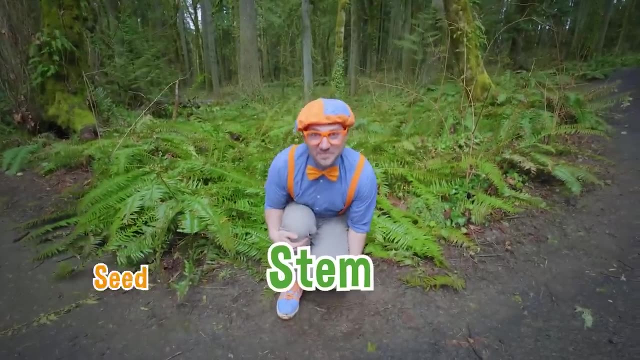 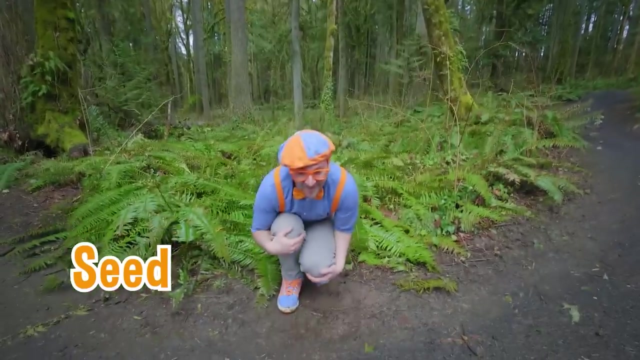 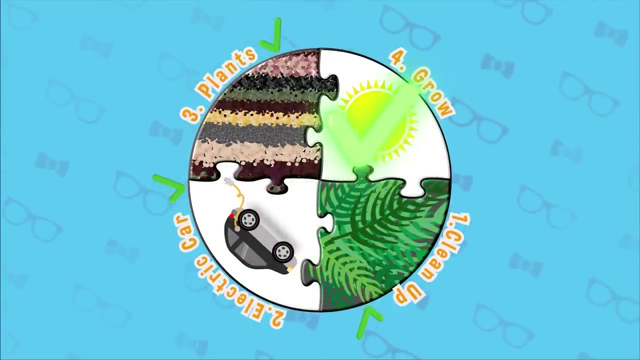 Yeah, Seed Stem Flower. Seed Stem Flower. Stem Seed Flower. The last step on our great green adventure: Check. We gave our new friends soil, water and sunlight that they needed to grow big and strong. 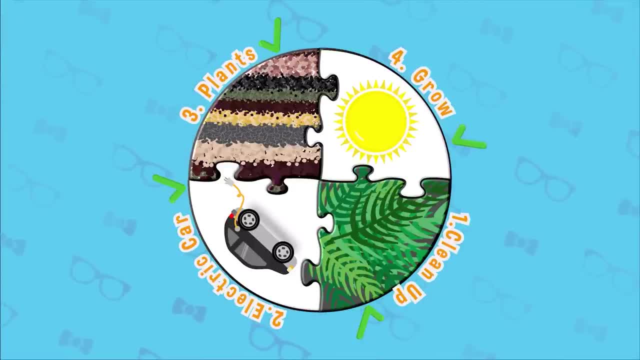 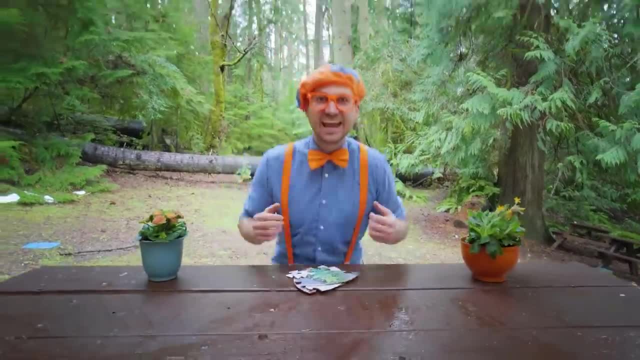 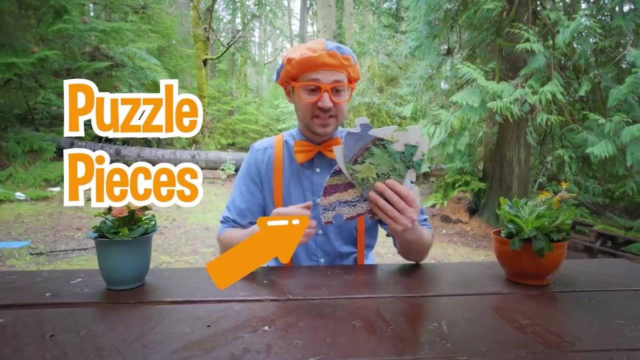 And more plants is always great for the earth. Great job, Yay Woo. Have you had fun today? Yeah, I sure have had a lot of fun with you as well. Yeah, We found a lot of puzzle pieces, Whoa. 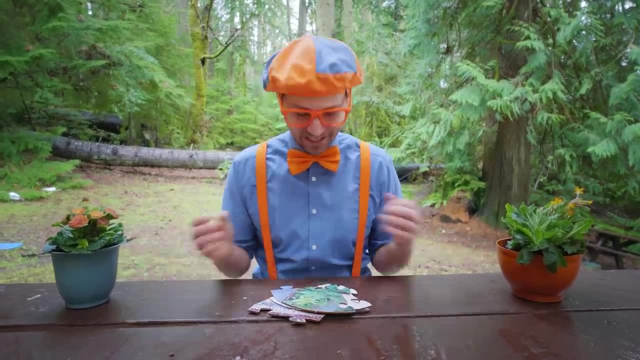 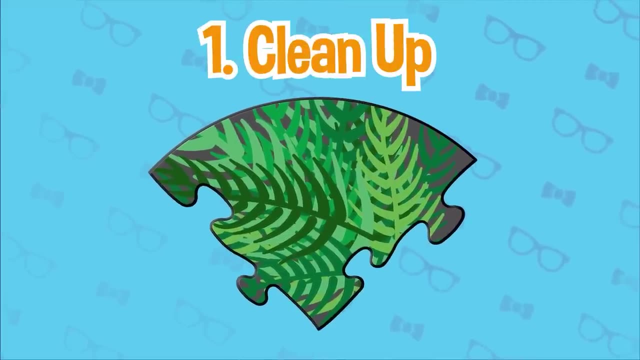 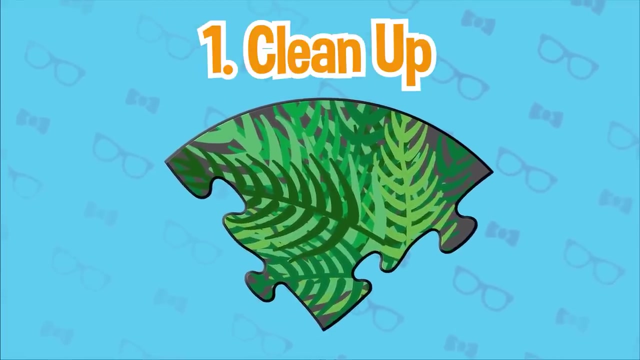 I love puzzles- They're so challenging. Hey, let's go over the four puzzle pieces that we found today. Puzzle piece number one taught us to clean up and recycle. Cleaning up and recycling helps things to grow and gets rid of pollution, And that's really healthy for our earth. 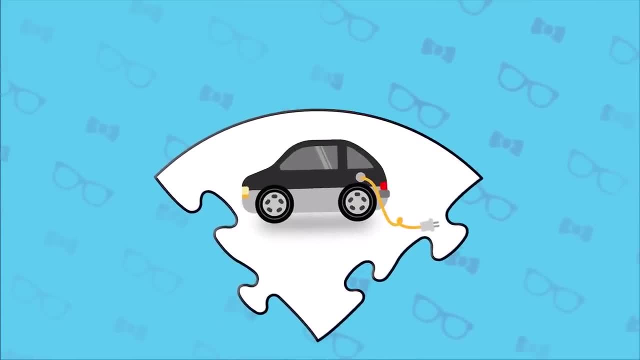 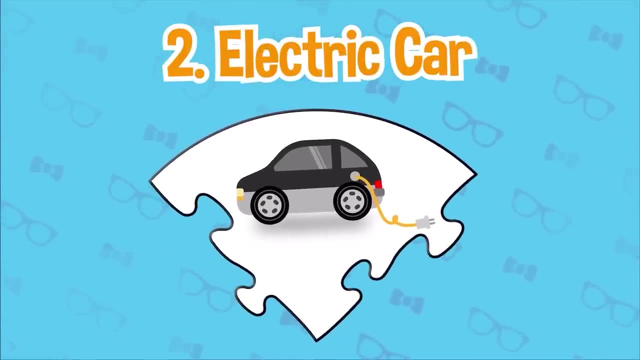 Puzzle piece number two took us to Oh Sparky and taught us about electric cars. Remember, they use electricity instead of gas And that's good for the environment because they don't create as much pollution. Plus, he was such a cute little car. 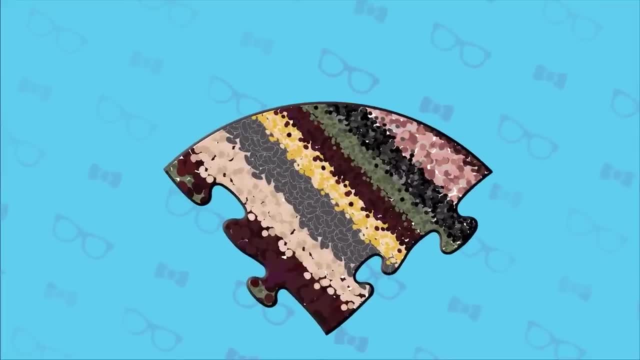 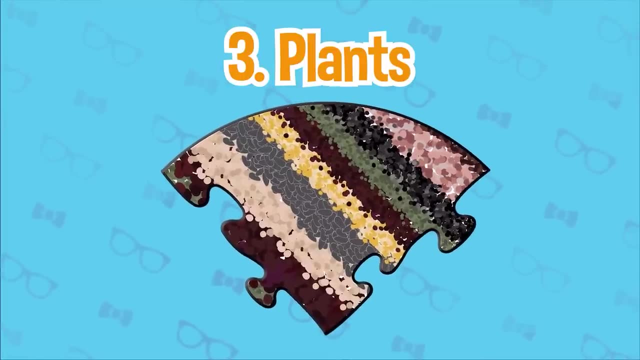 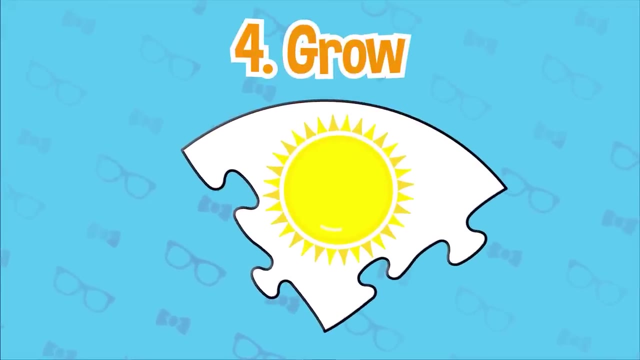 Beep, beep. Puzzle piece number three was all those little tiny seeds. Remember them. We visited the different plants at the nursery and even learned how those tiny seeds grow to become adult plants and flowers that give us life. And finally, puzzle piece number four taught us what our plants need to grow big and strong. 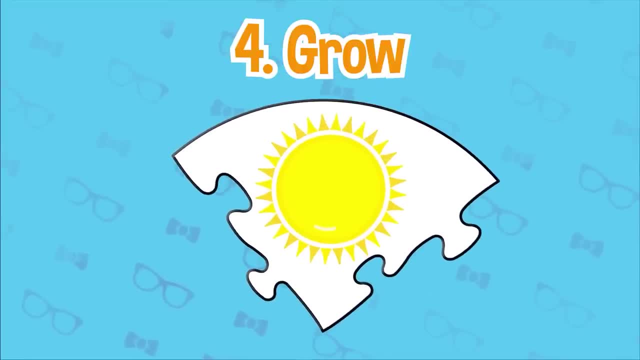 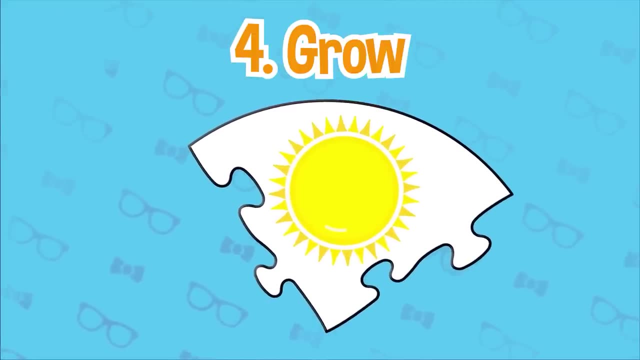 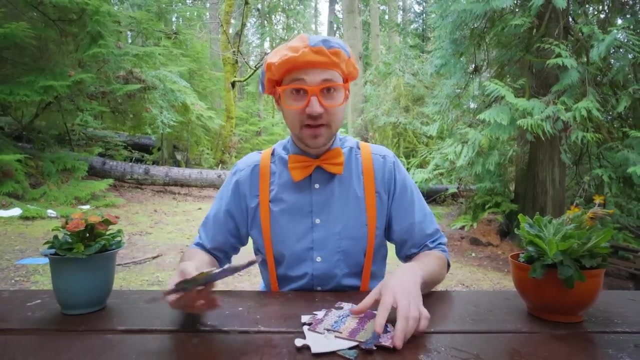 When there are more plants in the world, there are more homes for animals, more food to enjoy and cleaner air for us to breathe. Great job, Okay, I have an idea. Why don't I try and put all these puzzle pieces together and see what it looks like? 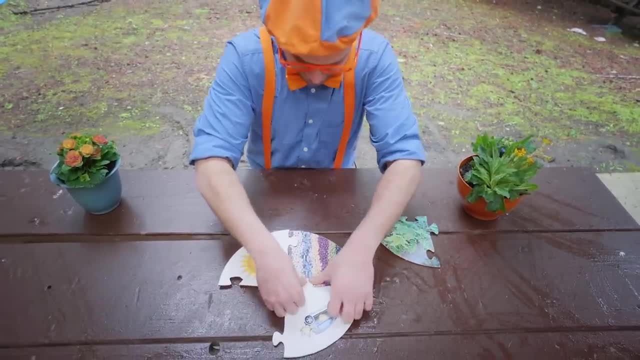 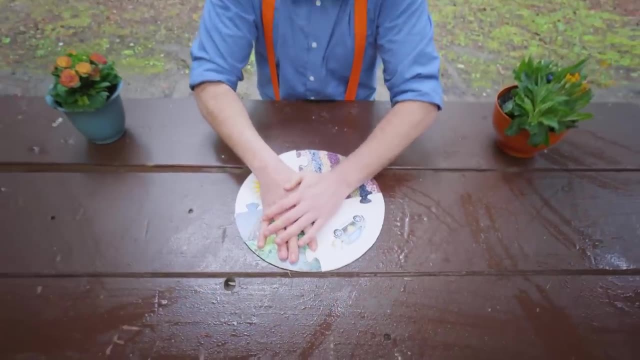 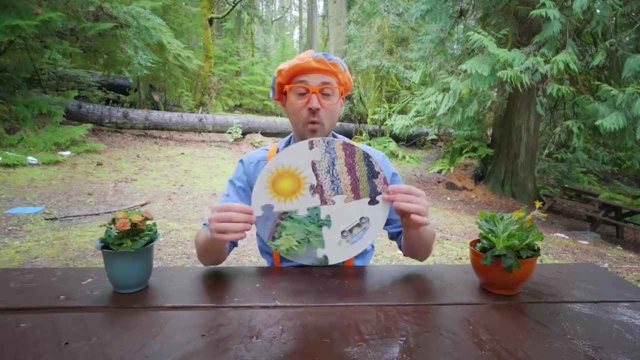 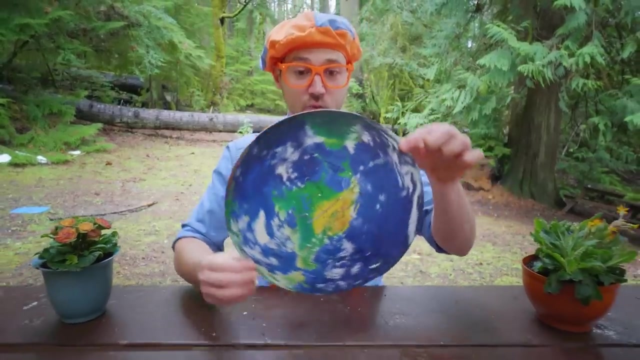 Huh, There's two. All right, There's three. Wow, We have four puzzle pieces all put together. Hey, What shape is this? Yeah, It's a circle. Whoa, And look at what we made. Yeah, 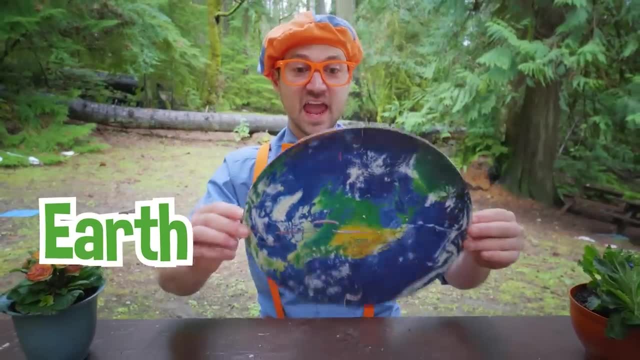 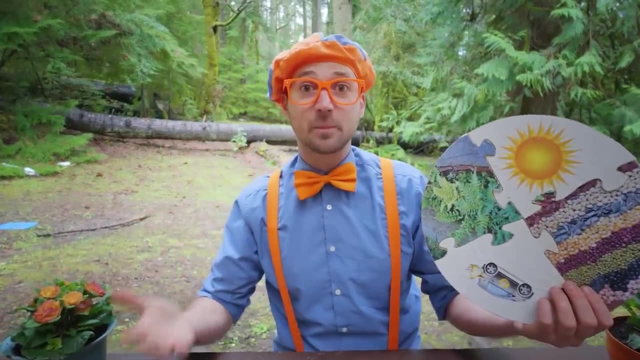 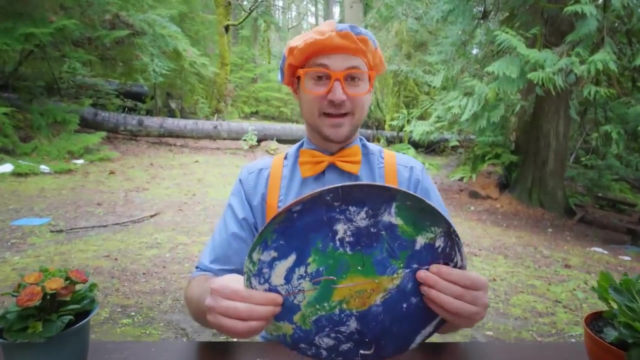 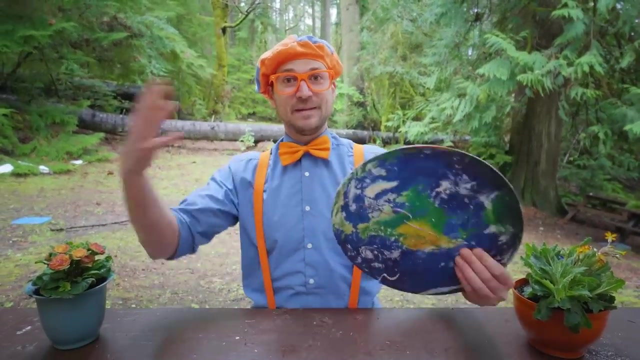 A puzzle of our planet Earth. Hey, And all four of these things on these puzzle pieces are just a few ways that we can make our planet a healthier, happier place. Whoa, I love our planet Earth and I love you. Thank you so much for being my friend and thank you so much for helping me, Blippi. 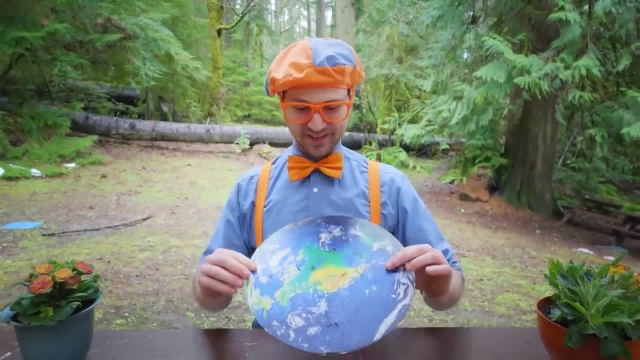 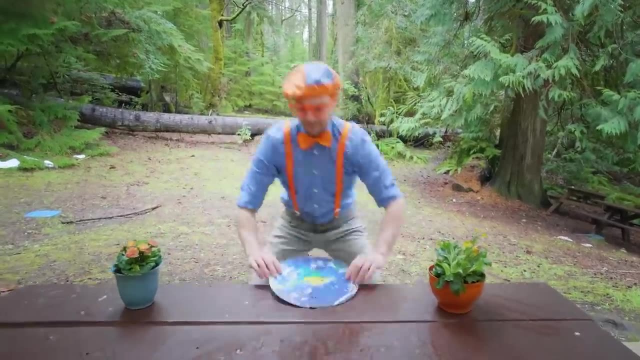 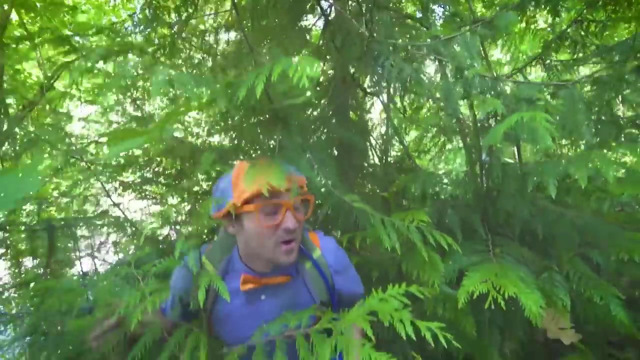 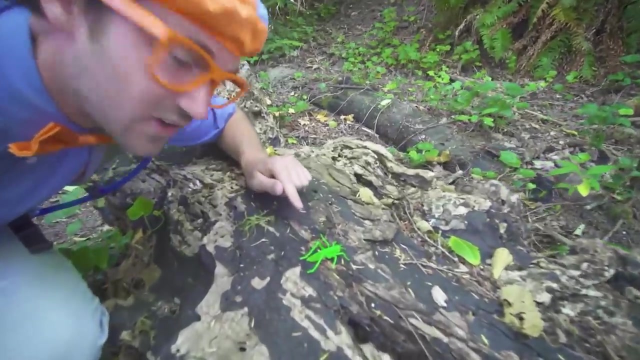 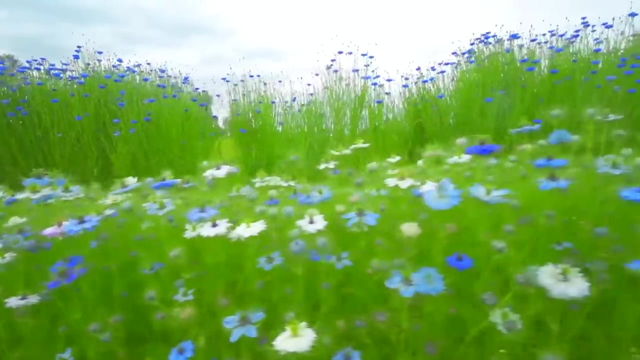 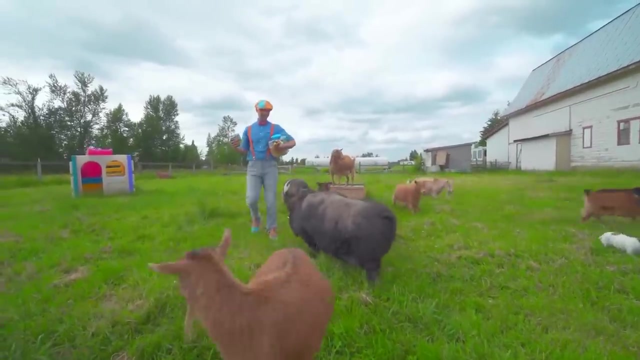 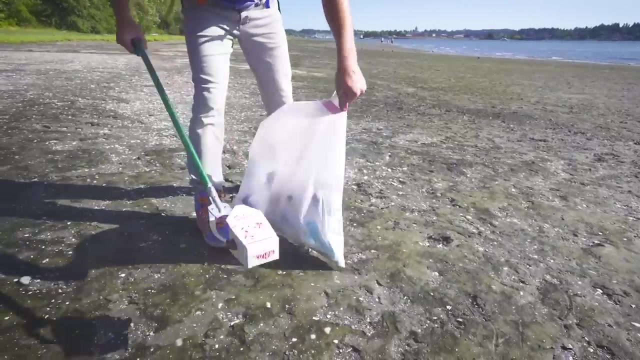 make our planet a happier and healthier place. Woo Appreciate it. Thank you, See you soon. Take care Bye. NOW I' LL W Creatures, even me and you. We're singing the Earth song. We're helping the planet Together together. 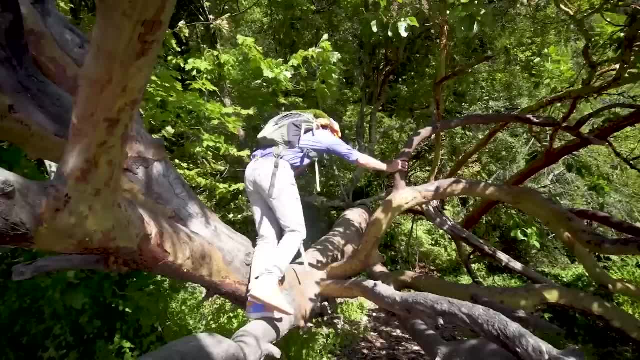 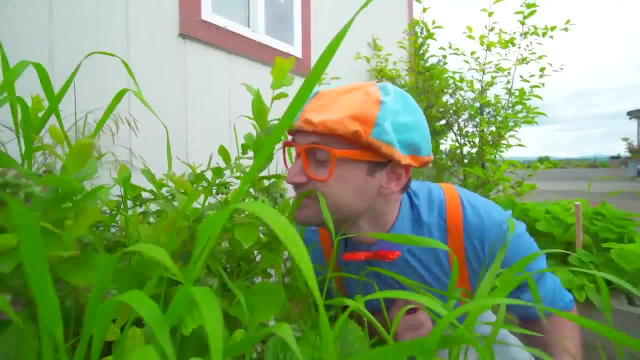 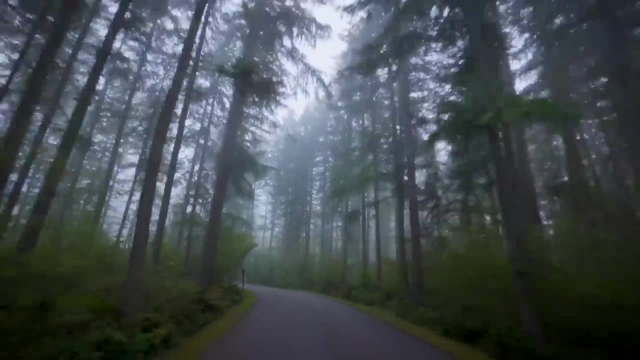 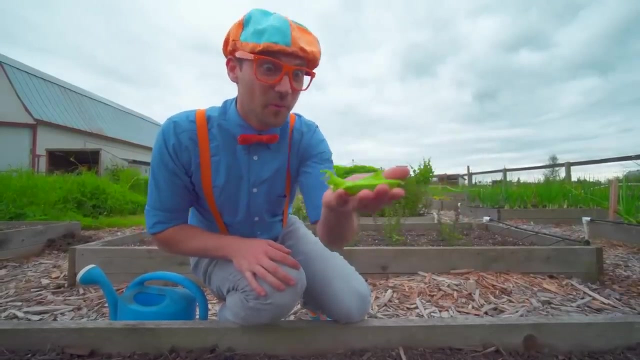 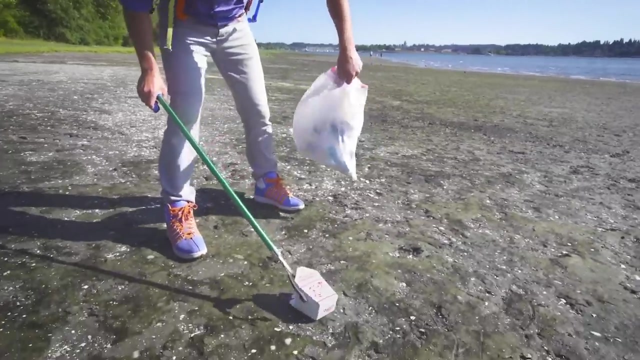 We can make a change. We're singing the Earth song. Come, learn all about it Together, together. It's time we start. Let's do our part. We can all help wherever we are. Use a little less water. that goes really far. Make sure to recycle paper, glass and plastic. 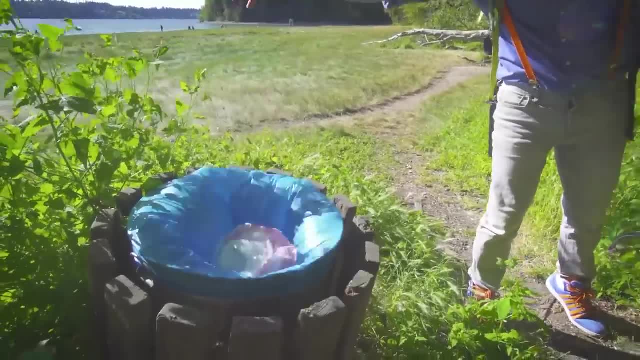 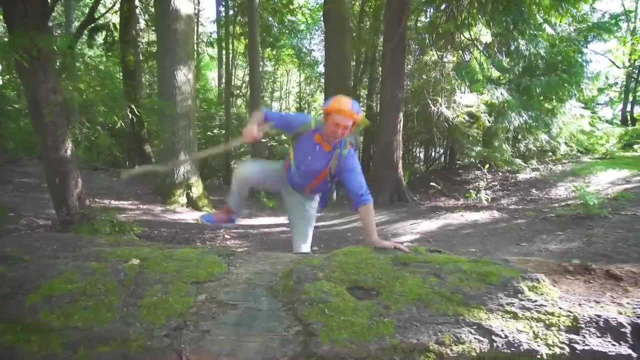 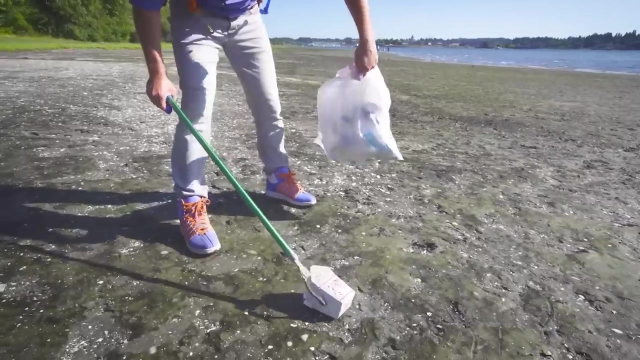 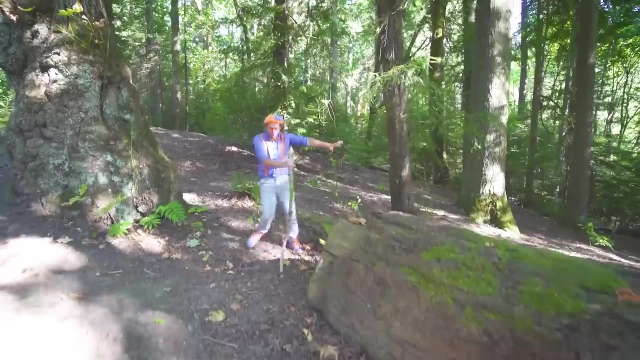 Taking care of the Earth will make you feel fantastic. You can plant a tree or pick up some trash. Ask a friend for help, Then it'll be a blast. We're singing the Earth song. We're helping the planet. Together, together, We can make a change. We're singing the Earth song. 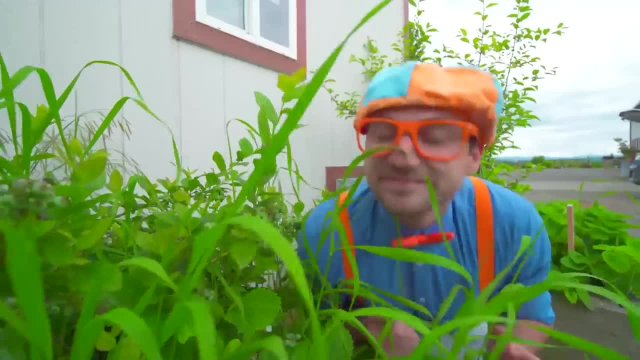 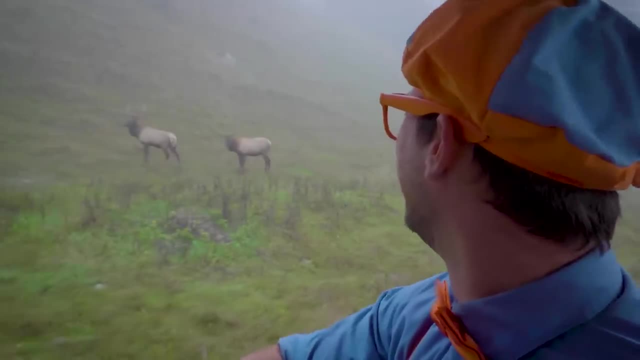 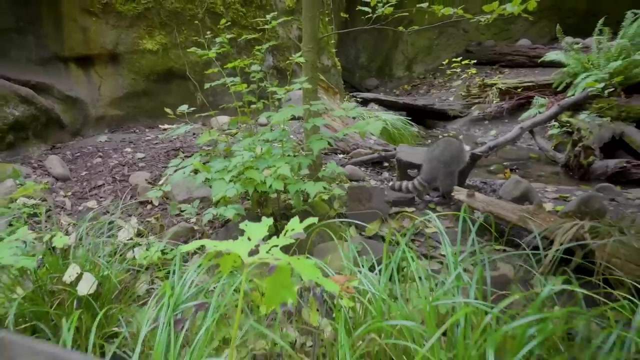 Come learn all about it. Together together, We can make a change. It's time we start Together together. Let's do our part. Let's do our part. Together together, We can all help wherever we are. Use a little less water. that goes really far. Make sure to recycle paper, glass and plastic. 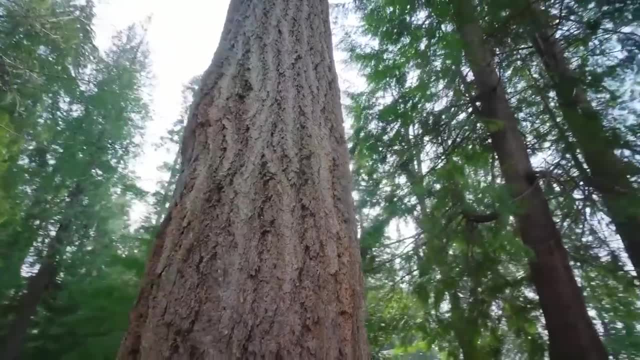 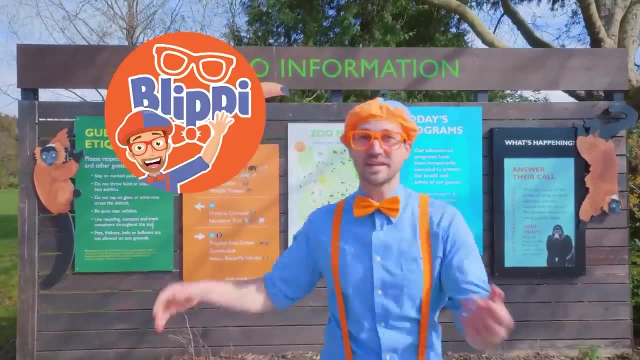 Take care of the planet Together. together, We can help wherever we are. Use a little less water. that goes really far. Make sure to recycle paper, glass and plastic. Take care of the planet Together together. Hey, it's me Blippi, and today I'm at Woodland Park Zoo in Seattle, Washington. 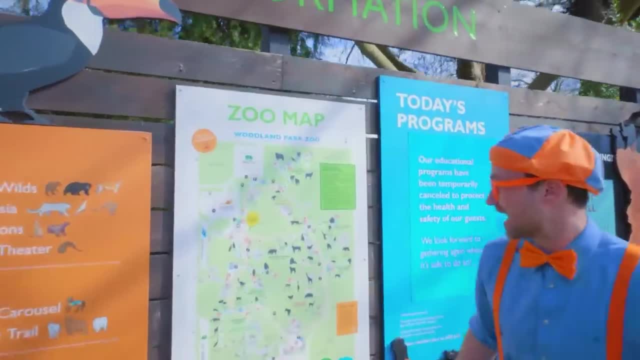 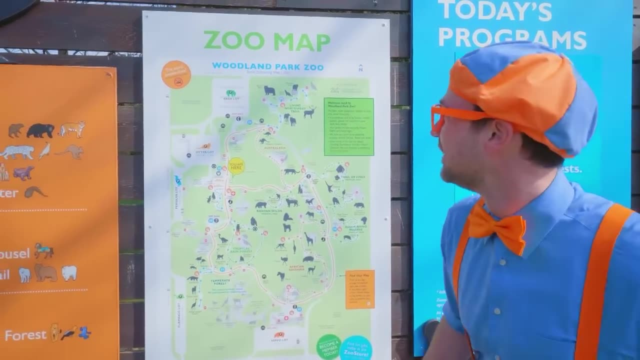 Hey, check it out. This is the zoo information area. Yeah, it has a map of the zoo. Hmm, I wonder what animals we're gonna see today at the zoo. Oh, maybe we'll see, ooh, a grizzly bear. 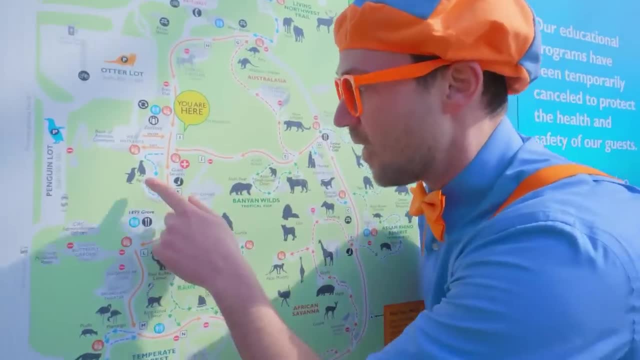 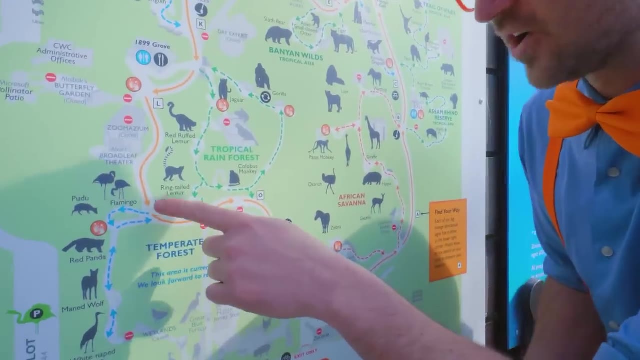 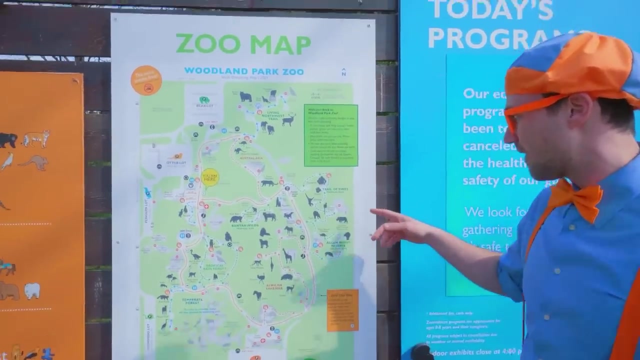 That would be so cool, Or oh, they have gorillas here too. Oh, and they have so many different kinds of animals like flamingos. wow, oh, whoa. Look at this tall animal. This is a giraffe. 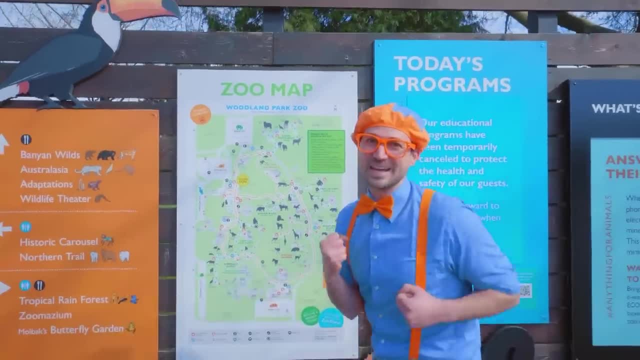 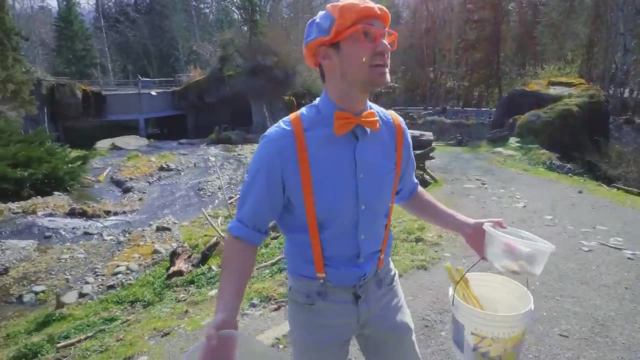 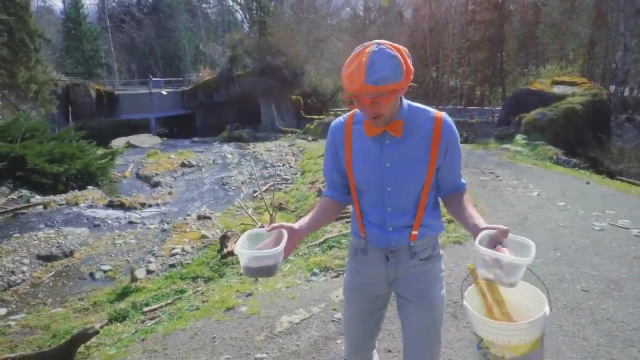 That is such a tall animal. Well, there's some animals for us to go learn about. Let's go. Oh, look at this place. Yeah, this habitat looks like Alaska or the Pacific Northwest or Canada. Yeah, and I have some enrichment for this animal. 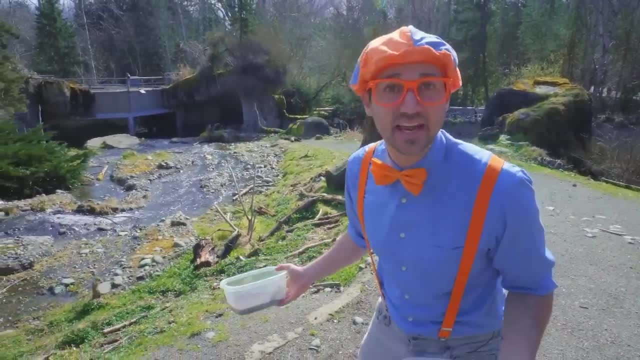 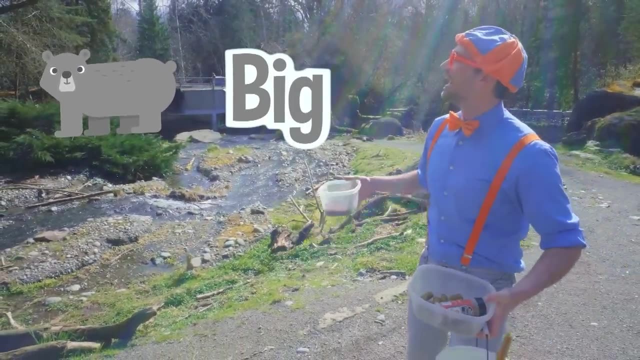 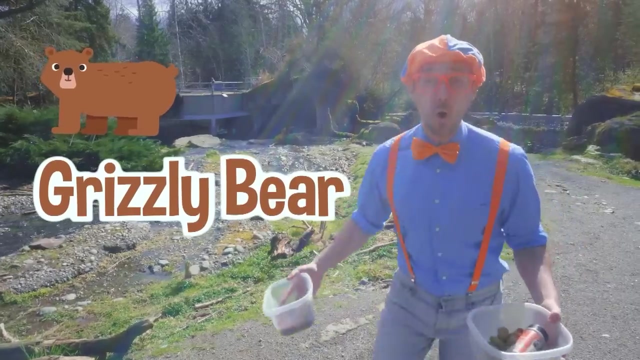 But hey, let me have you guess what animal this habitat is for. Yeah, it's a bear, It's a real big bear. Oh, it's brown. Yeah, it's a grizzly bear. Whoa, that is so crazy. 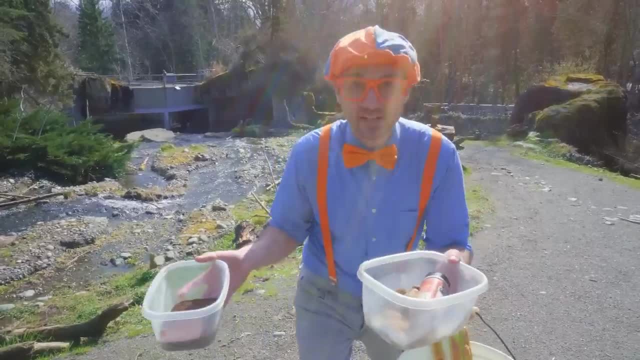 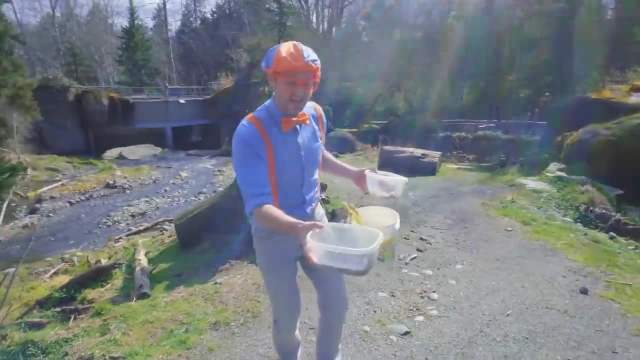 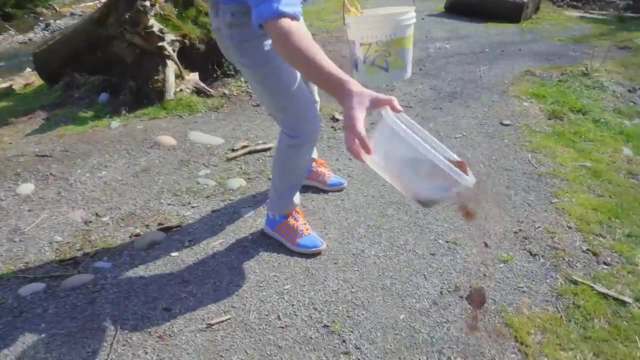 Hey, all right, I got permission that I can spread this food and enrichment out, so then the bear can enjoy it. Let's go Okay. first I have some coffee grounds. See this? Yeah, that's just normal coffee. So if you sprinkle some right here, 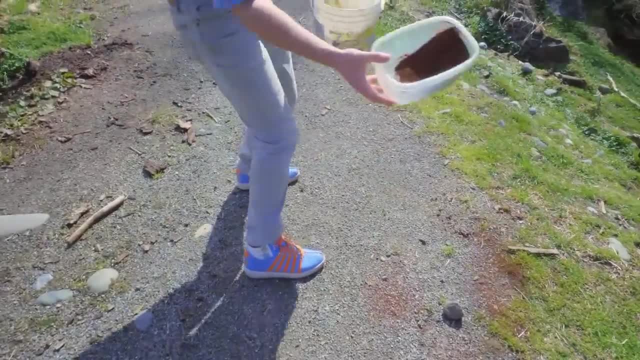 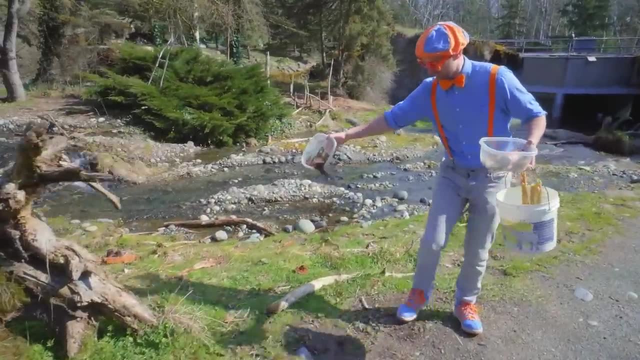 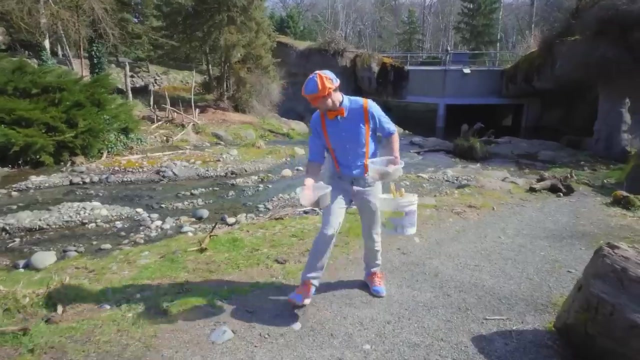 yeah, maybe the bear will roll in it. The bear loves to roll in coffee. Okay, how about right here? Yeah, there we go. Oh, and maybe maybe some right here, There we go. all right, let's put this right here. 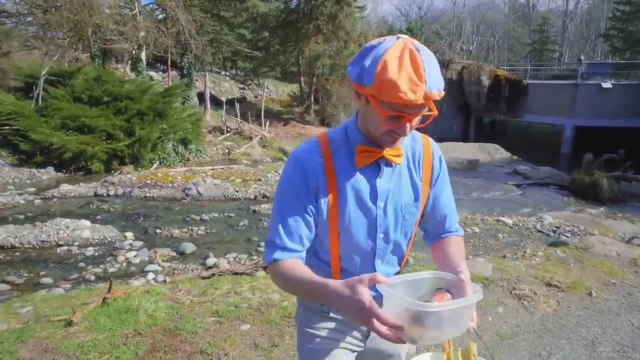 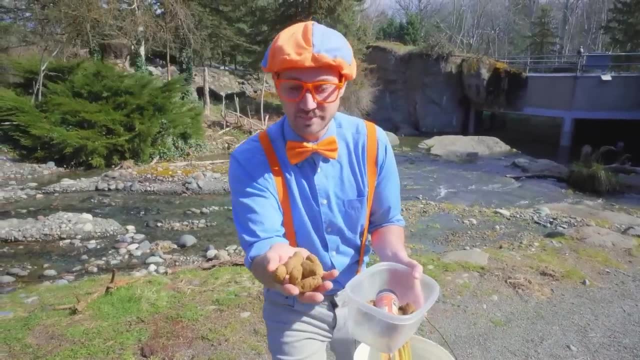 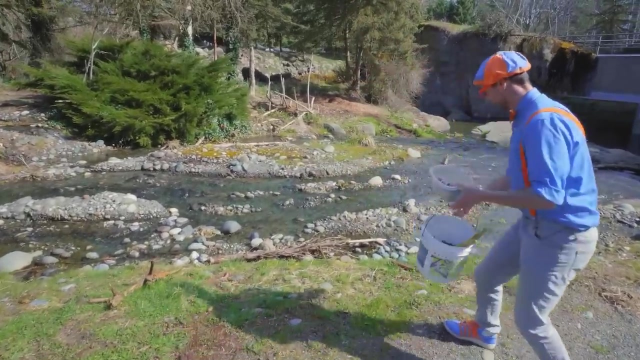 and we will definitely grab that before we leave. Okay, Okay, look at these. These are biscuits. Yeah, this grizzly bear loves these biscuits, So I'll just try, and you know, put some around here. Ooh, there we go. 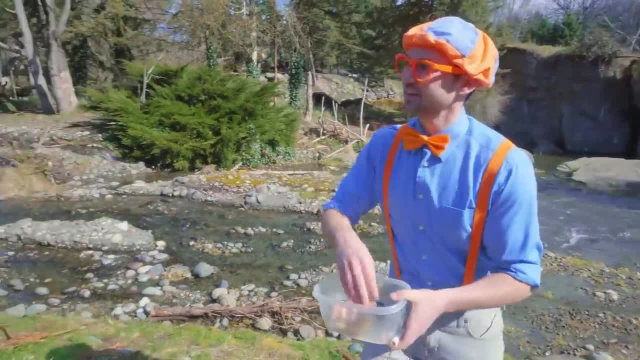 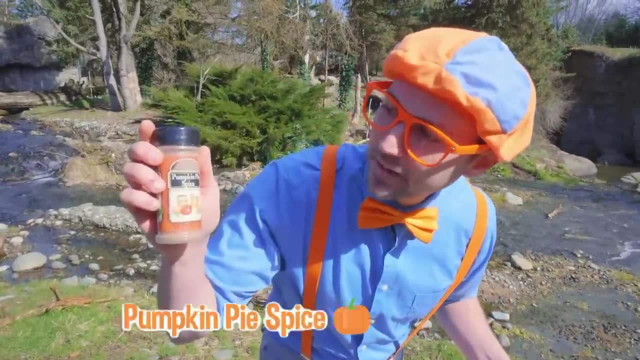 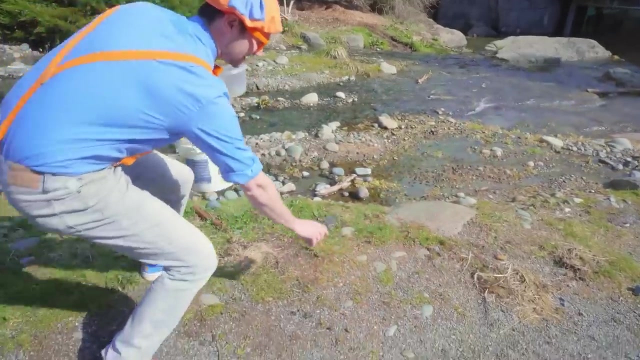 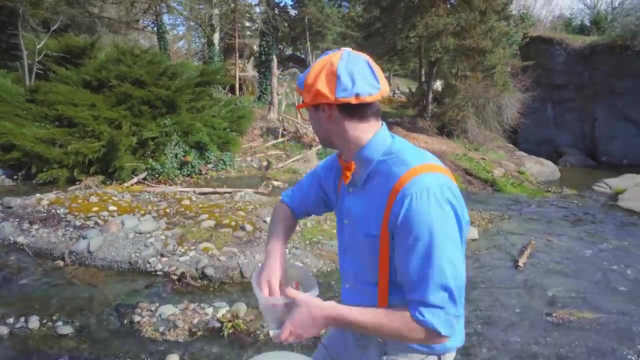 All right, let me throw some to give it a nice pat. Hey, ooh, what is this? Pumpkin pie spice? Yum. all right, let's just sprinkle some of this right around here. All right, I still have some biscuits. 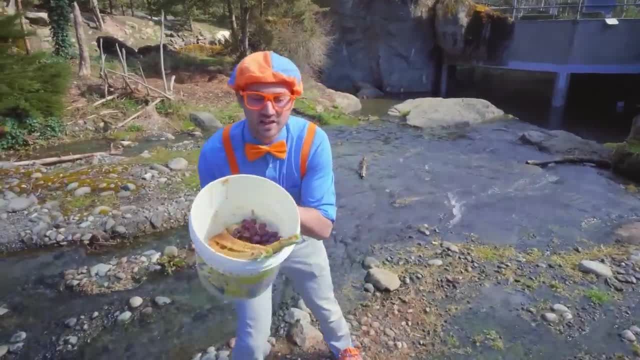 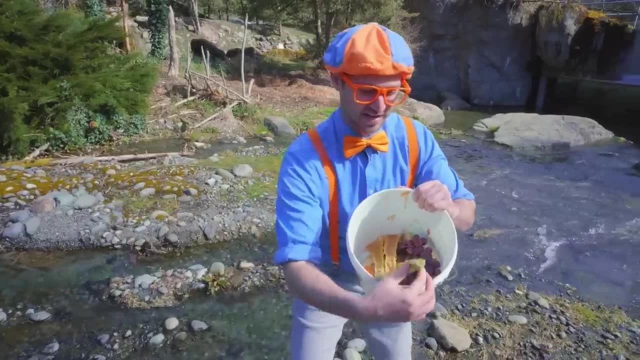 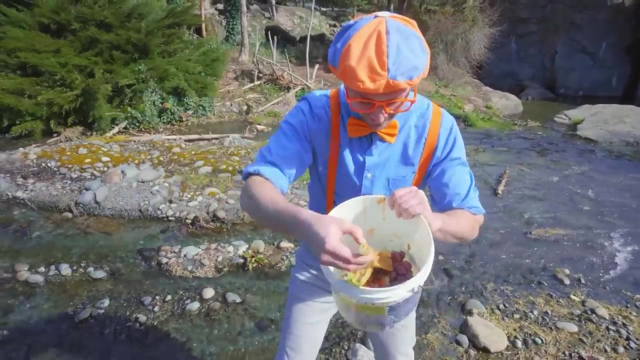 Check this out. Yeah, there's a lot of fruits and vegetables in there. Yeah, I love fruits and vegetables. Yeah, like celery with some peanut butter And honey on top. yum, Ooh, looks like we have some grapes, yum. 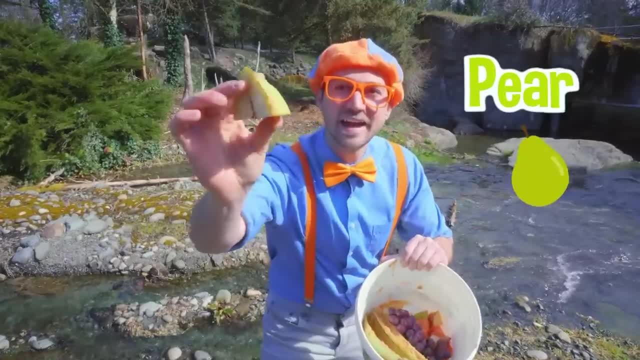 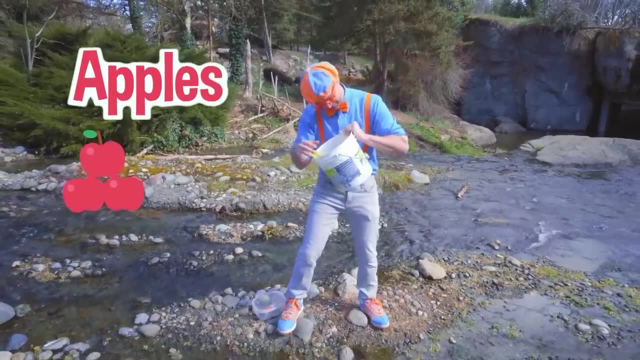 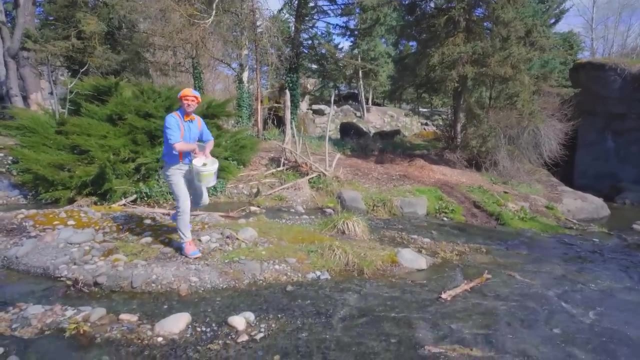 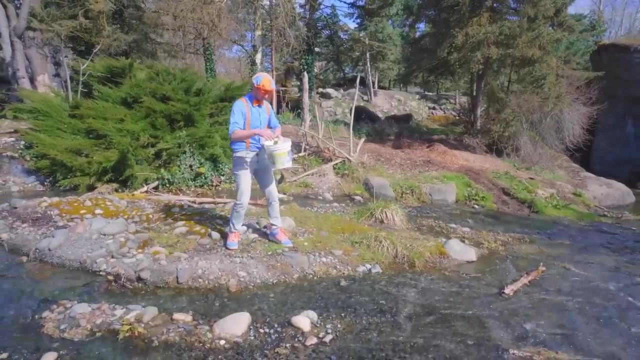 Ooh, and we have some pears, and we have some carrots, Whoa, and some apples and some watermelons. Yeah, put some biscuits right here on this little island, All right, perfect. Ooh, this fruit smells so good. 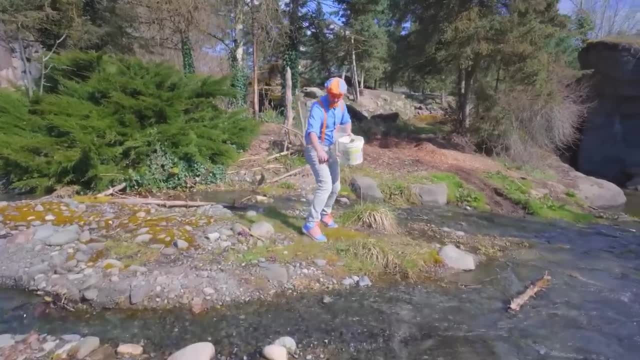 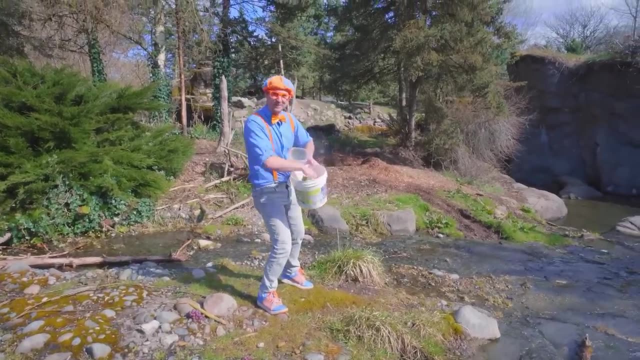 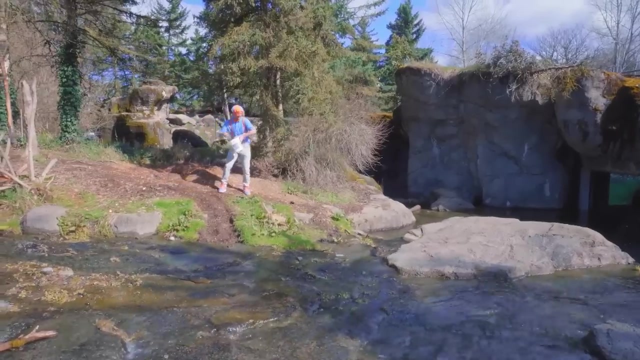 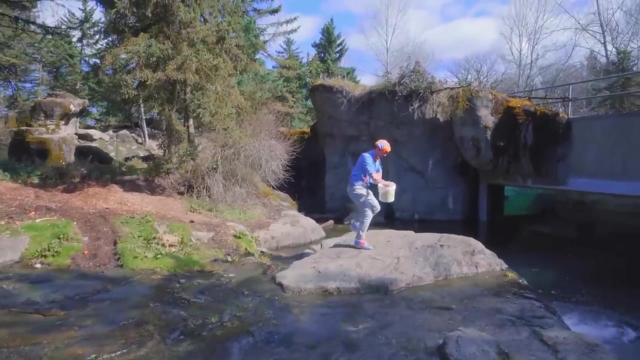 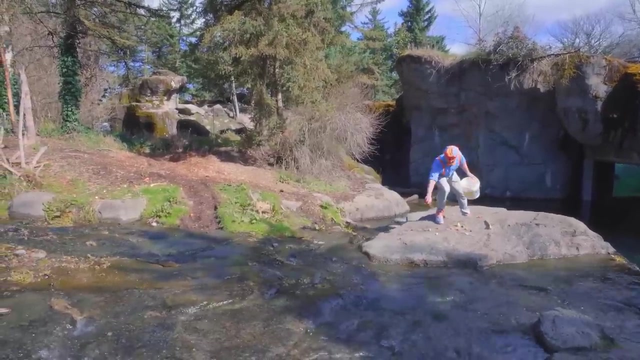 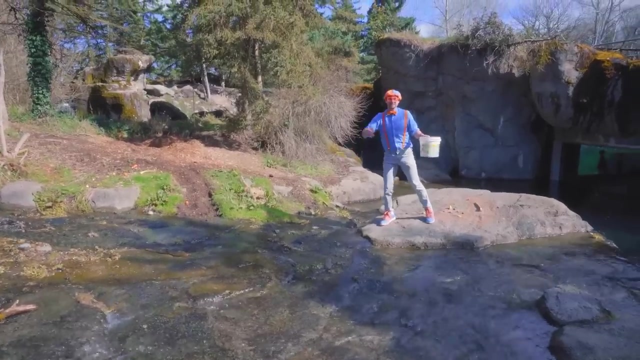 All right, sprinkle some more pumpkin spice, All righty, and then I'm going to make it all the way down there to put some more food down there. Wow, this bear is going to have some good eating around here. Hey, and now let me get my container, and then we'll let the bear out, so then he can have some yummy snacks. 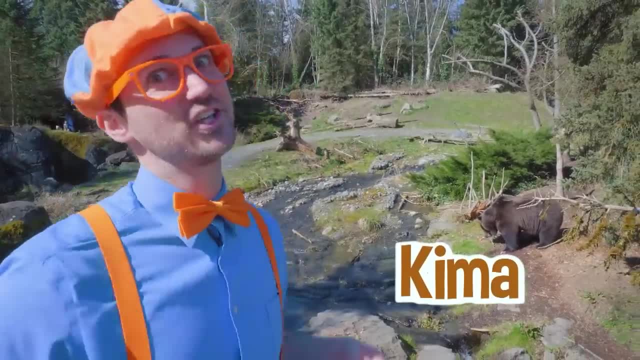 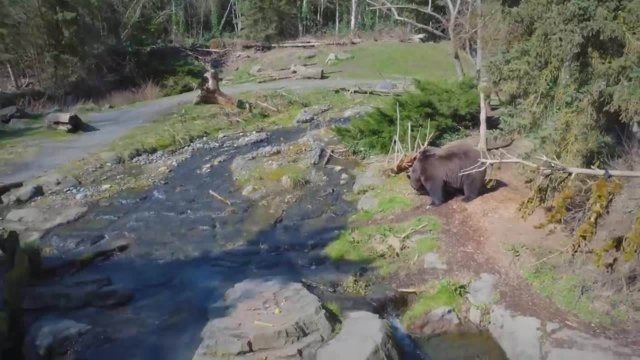 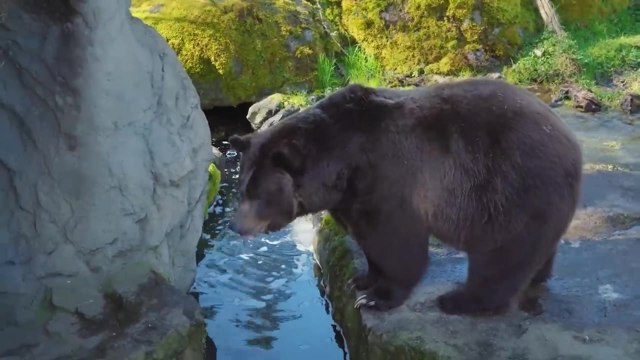 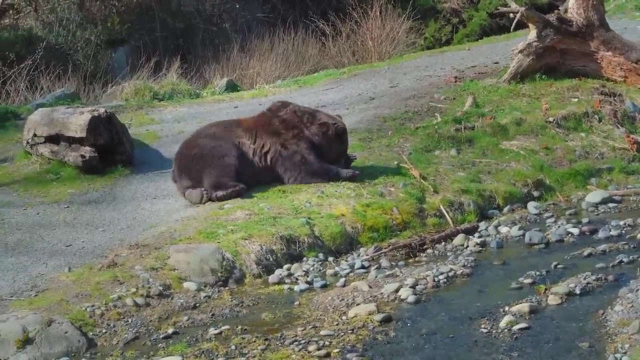 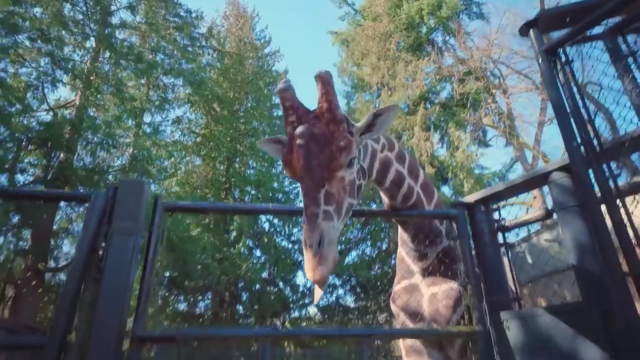 Whoa, check it out. There's Kima. Kima is a giant grizzly bear and he is loving those snacks we put out for him. Good job, Let's check him out. Whoa, check it out. Yeah, this is Dave, and Dave is a giraffe. 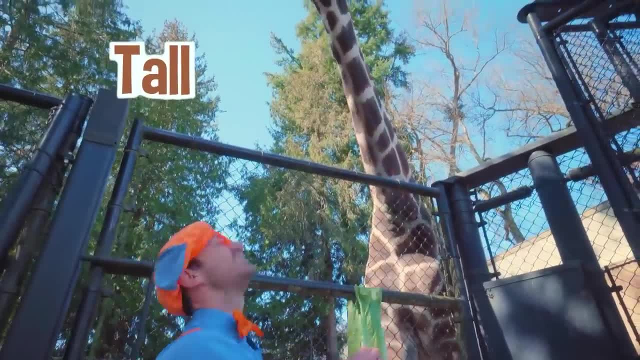 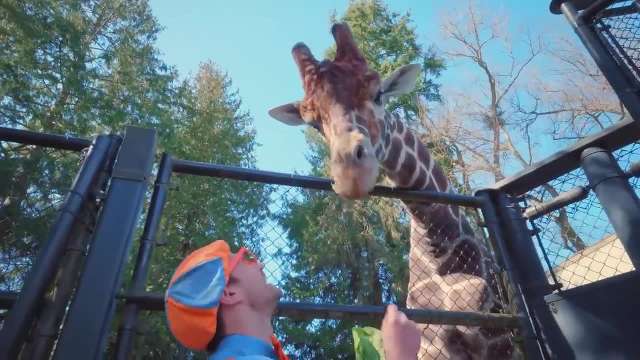 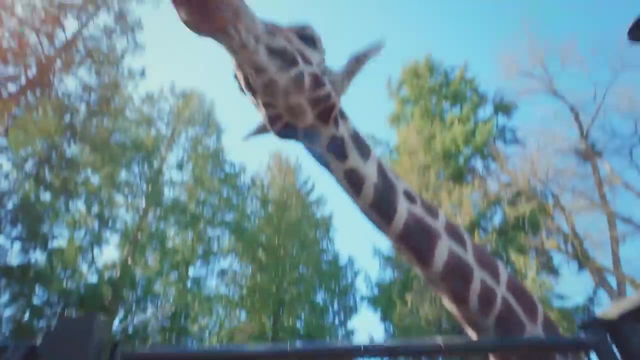 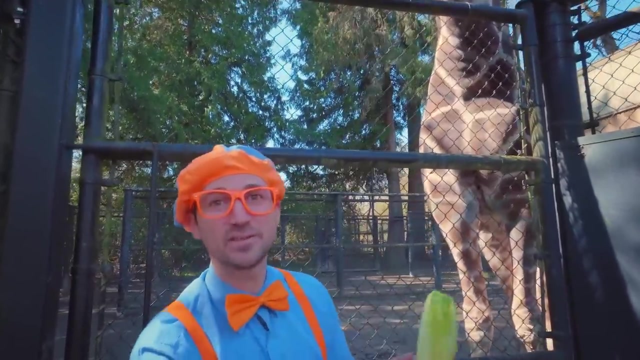 He is so tall. Here you go, Dave. I'm feeding Dave some romaine lettuce. Dave loves lettuce and romaine. Hey, how are you Whoa check this out. Dave is using his tongue, kind of like a hand, to grab his food, to pull it up into his mouth. 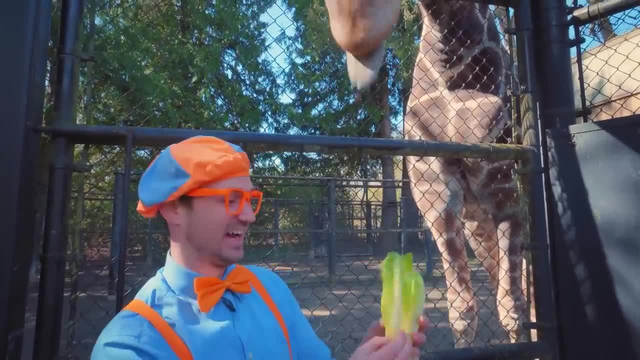 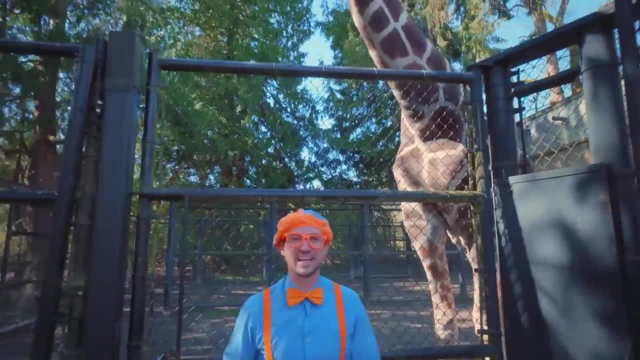 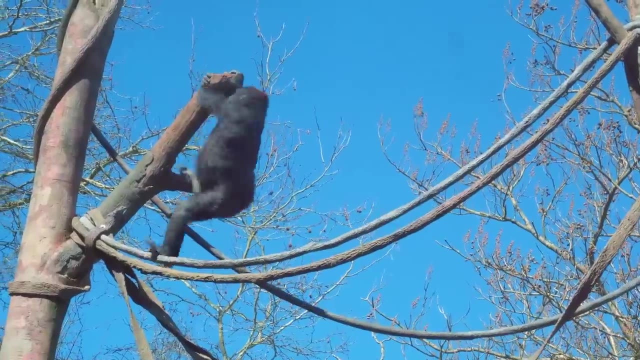 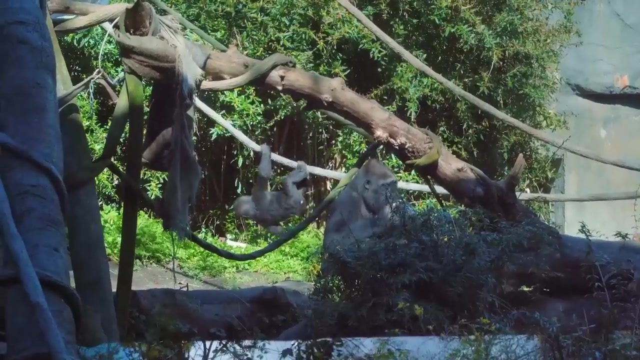 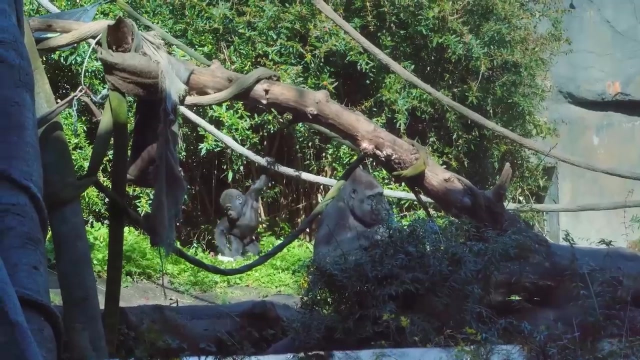 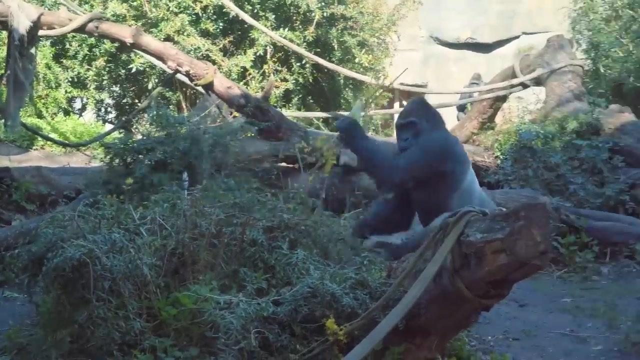 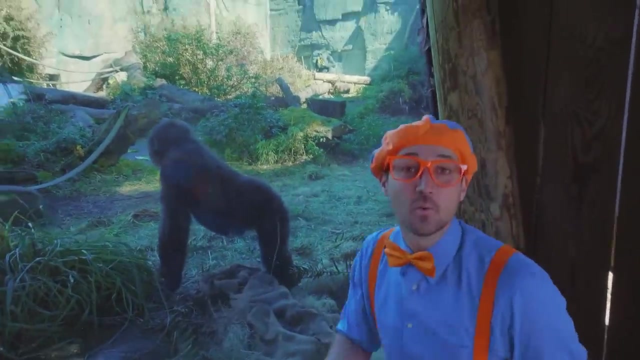 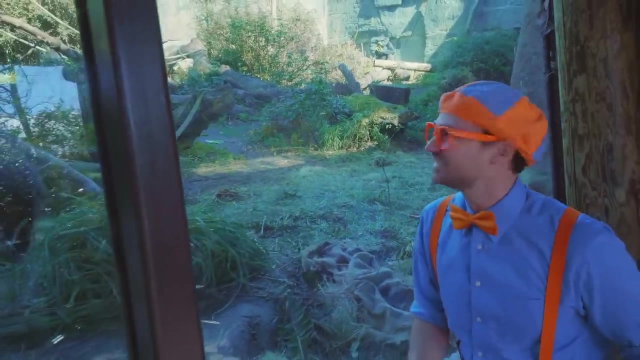 Wow, Dave is so cool. Here you go, Dave. Alright, okay, see you later, Dave, I have more animals to go visit. Let's go. Oh, Whoa, Check it out. We are at the gorilla habitat, Whoa, Look at her, She is so cute. 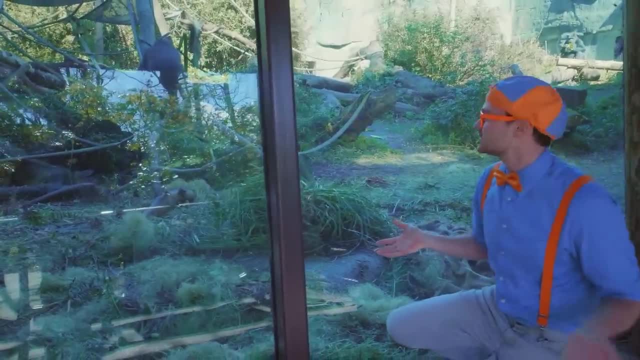 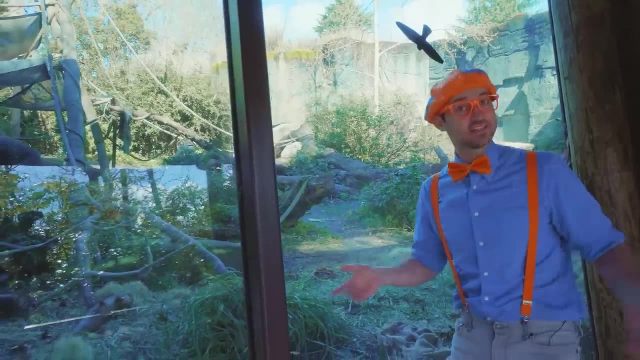 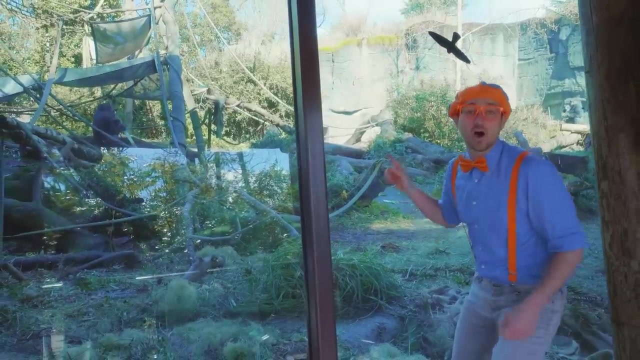 Whoa, Yeah, they're throwing some enrichment out. Then the gorillas have some snacks. I love snacks. All these gorillas here. the group is actually called a troop Whoa- Group rhymes with troop. Wow. All of these gorillas are actually females except for two Did. 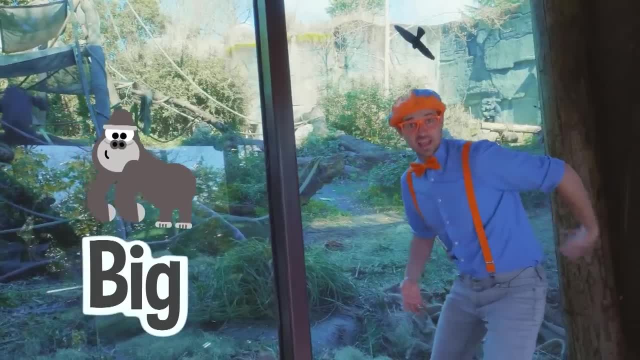 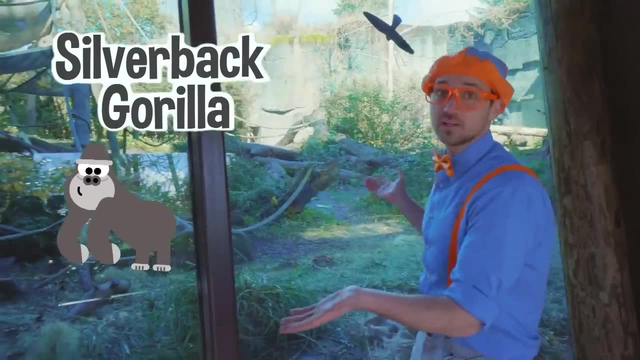 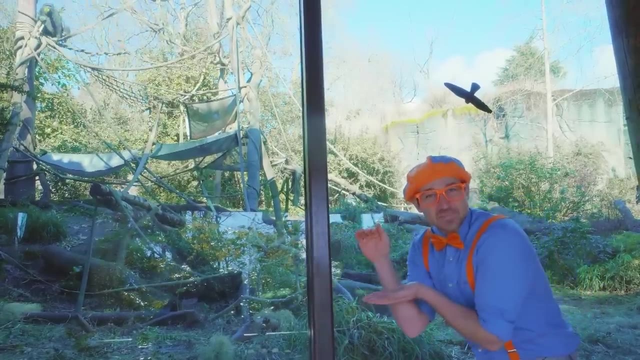 you see the big one. Yeah, with the silver back. Yeah, that gorilla is the head honcho of this troop and that is a silverback. And all of these gorillas are western lowland gorillas, Whoa, And there's also a second male: It's the little baby. Oh, so cute. All right, let's. 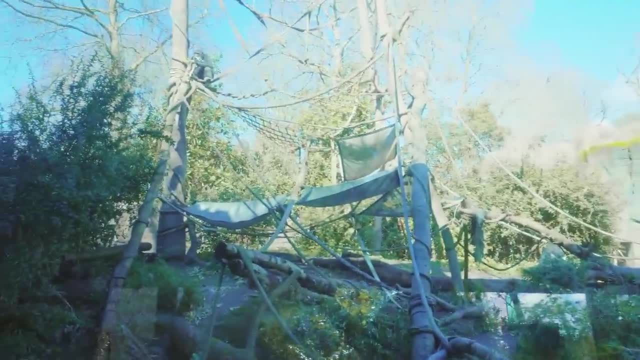 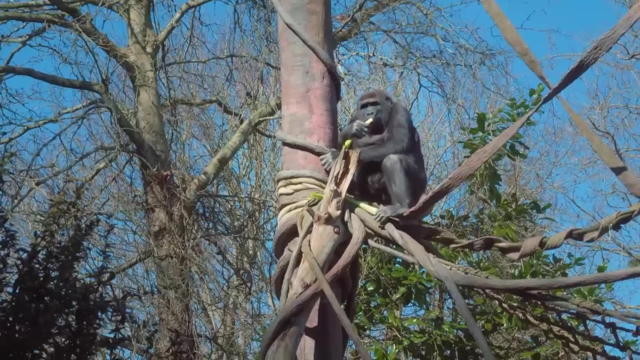 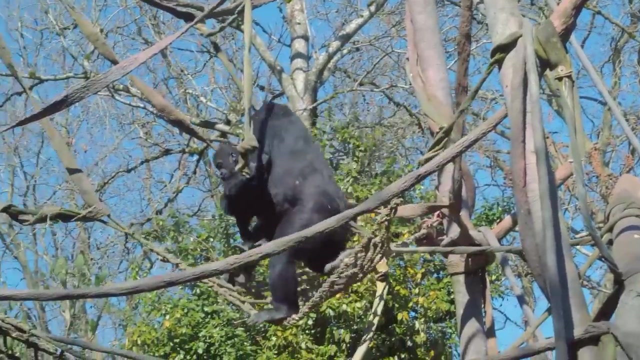 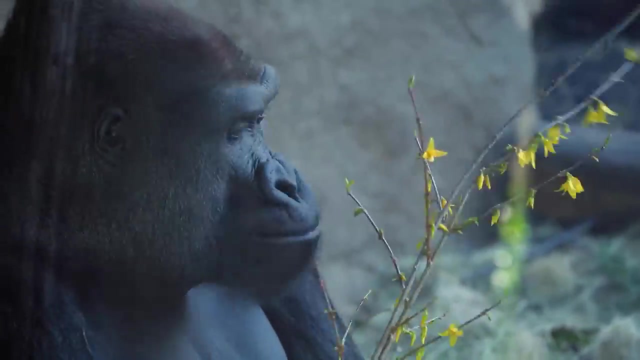 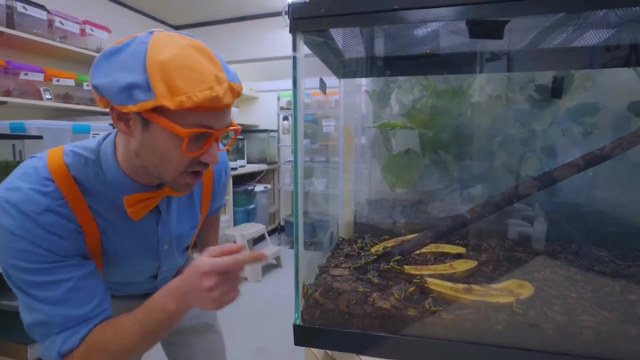 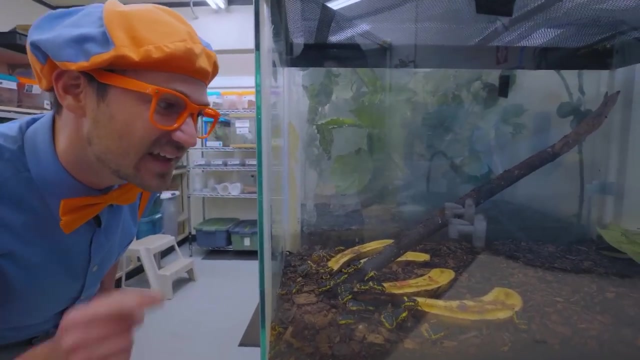 watch him eat some food. Whoa, Check it out. Yeah, these are garden fruit chafers. It is a type of beetle. Do you see what kind of food they're eating? Whoa, Yeah, It looks like bananas. Yum, I. 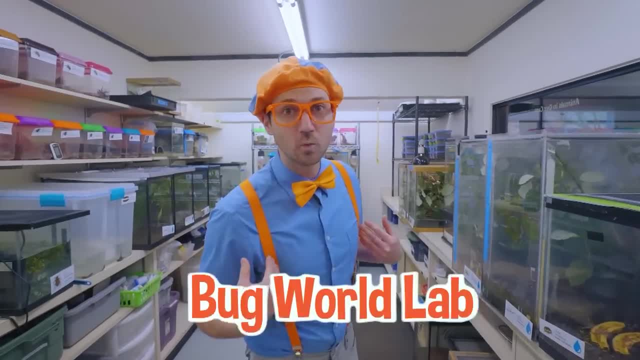 like bananas too. Whoa, Look at where I'm at. I'm at Bug World Lab. Yeah, this is where all the bugs hang out in the world. Yeah, I've never seen a worm before. It's awesome. I want this. Yeah, it's a human giant worm. It's a little cute human now. Yeah, it's. 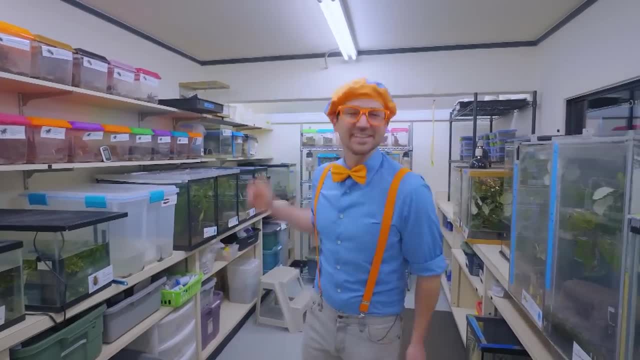 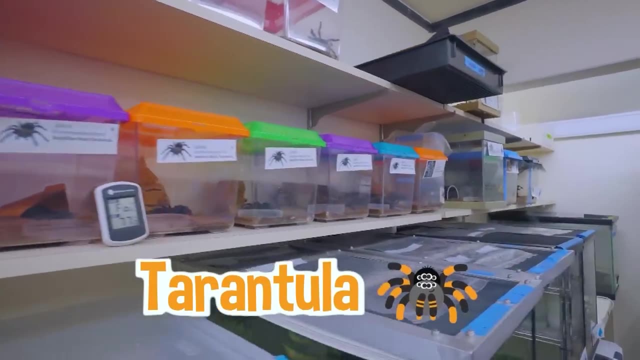 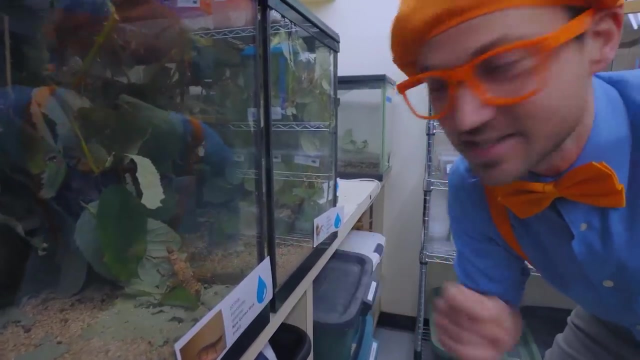 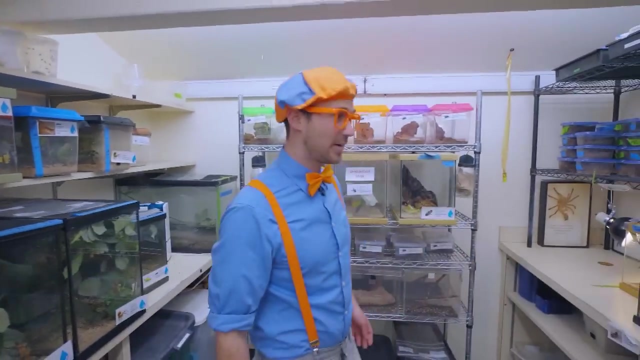 bugs hang out and eat and sleep. yeah, this is where they primarily live: whoa. looks like a lot of tarantulas, up there, whoa, and down here a stick insect, a new guinea stick insect, whoa. that is so crazy. wow, there's so many different types of bugs and insects back here. 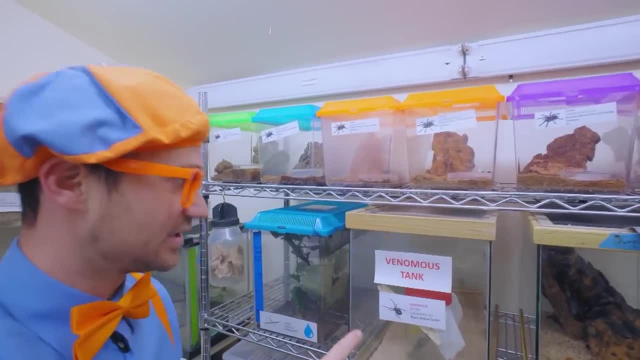 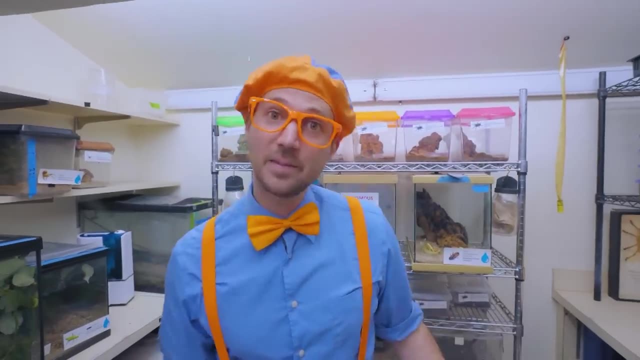 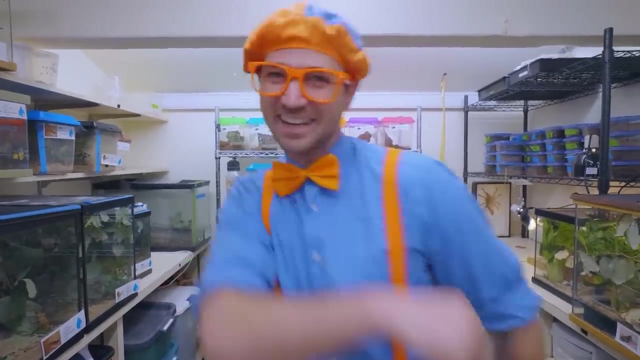 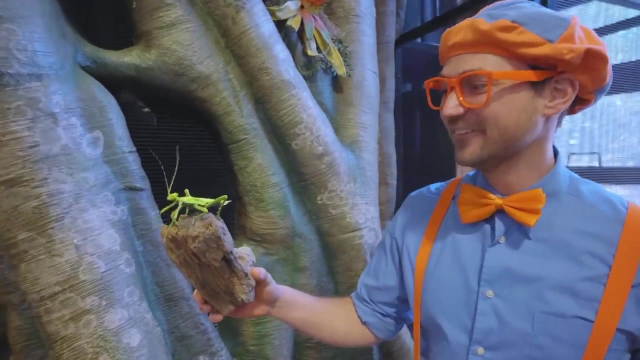 whoa, even more whoa spiders. ooh, and a venomous spider. we definitely don't want to open that one up. but hey, maybe if we go in the other room they'll bring out some bugs for us to see up close and personal. yeah, let's go. whoa, check it out. whoa, this is a jungle nymph. wow what. 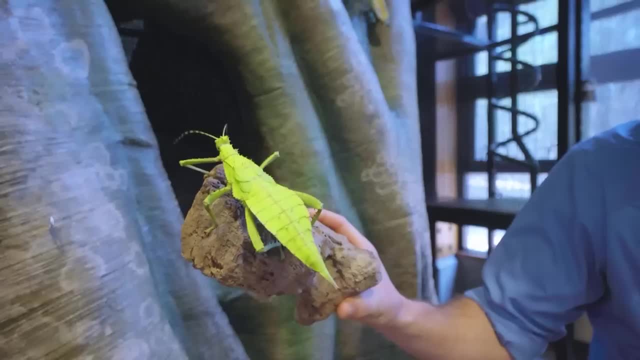 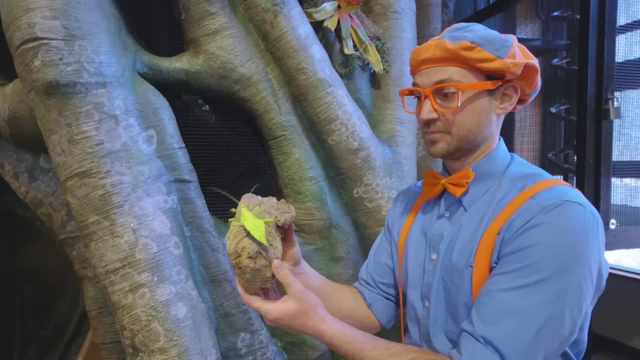 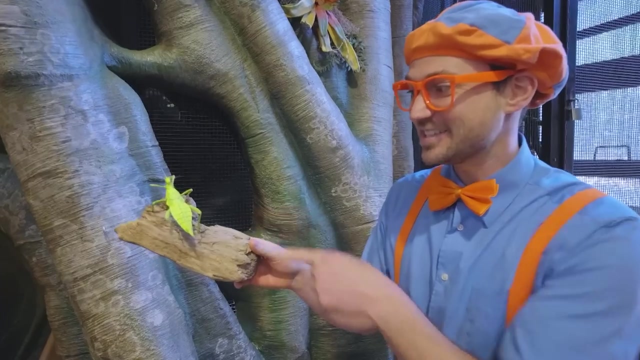 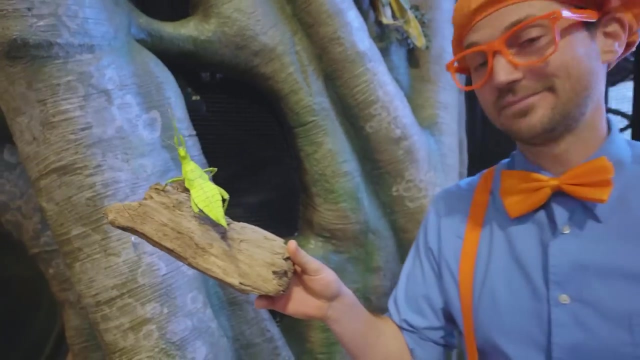 color. is that color? is she? Yeah, Yeah, she is the color green. I actually knew it was a she, because the males are brown and she is green. Yeah, Do you see how she looks like a leaf? Yeah, she looks like a green leaf, But if it was a guy, he would look like a brown leaf. Wow, 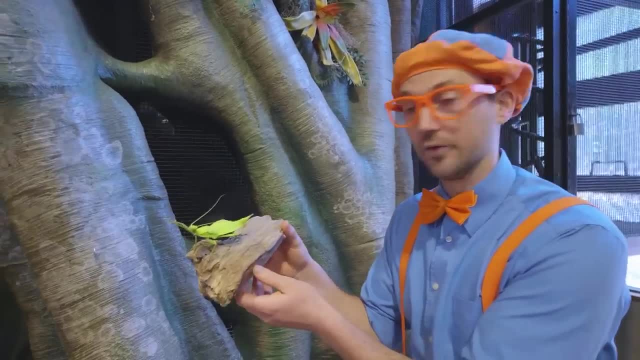 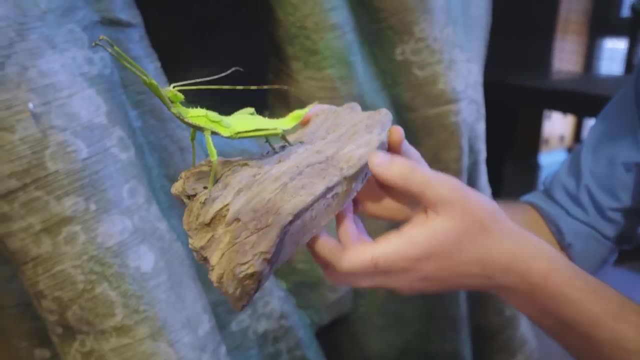 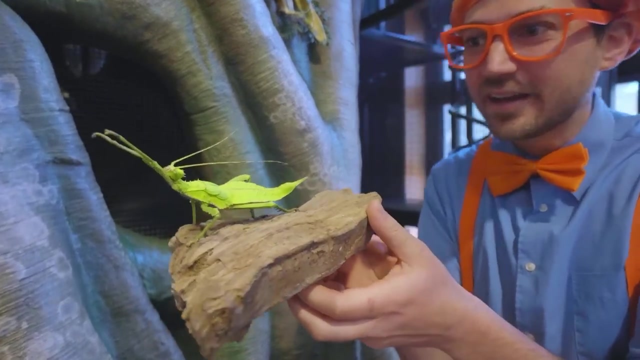 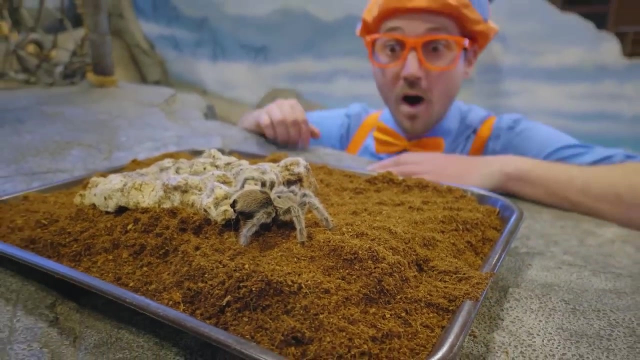 Little nymphs are the heaviest insects in the world. Yeah, she's not even full grown yet. and look how big she is. Whoa looks like she's just doing some stretches. That's so silly. Wow, she is so cool looking. Whoa, Whoa, check it out. Yeah, this looks like. 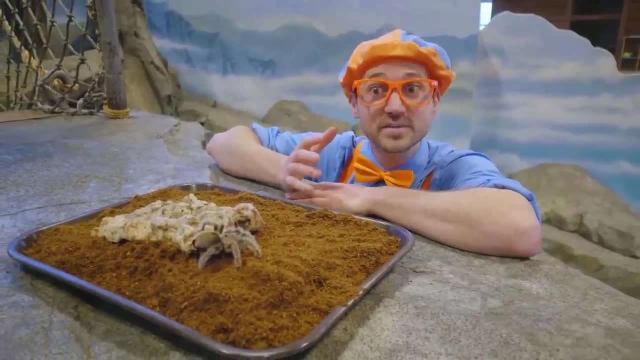 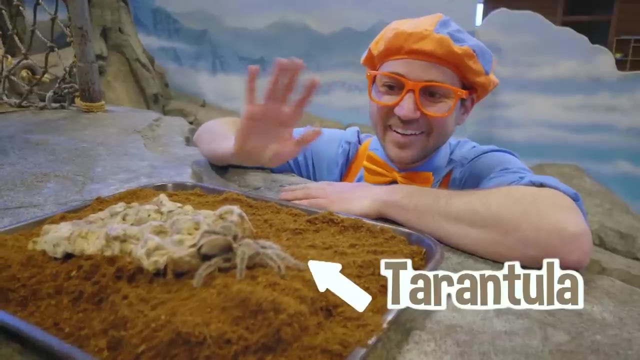 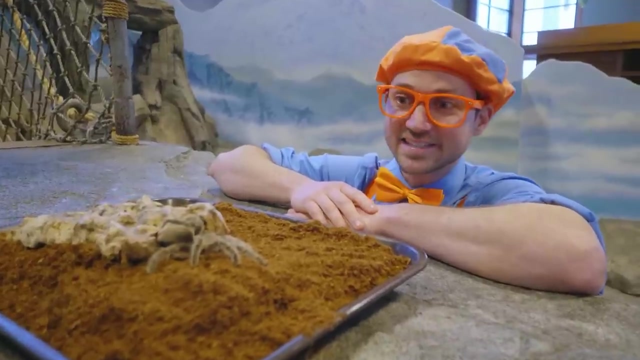 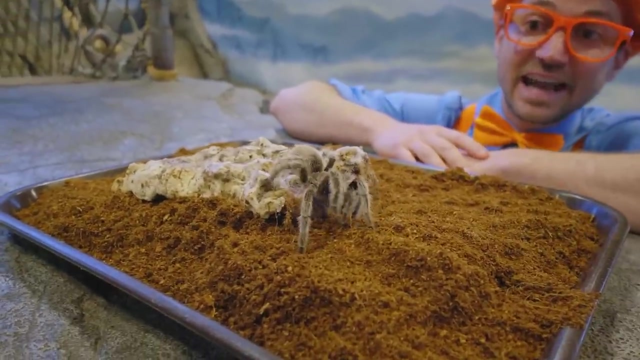 a spider. Whoa, it is such a big spider. This is actually a Chilean rose-haired tarantula. Whoa hello. I used to be really afraid of spiders, but not anymore. This one's actually really nice. Yeah, if I let it crawl on me, it wouldn't even bite me. This one is very nice and 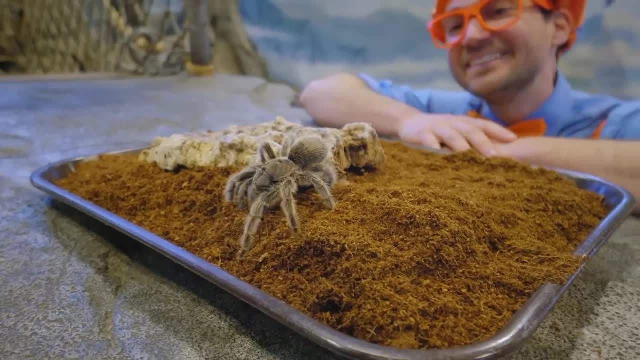 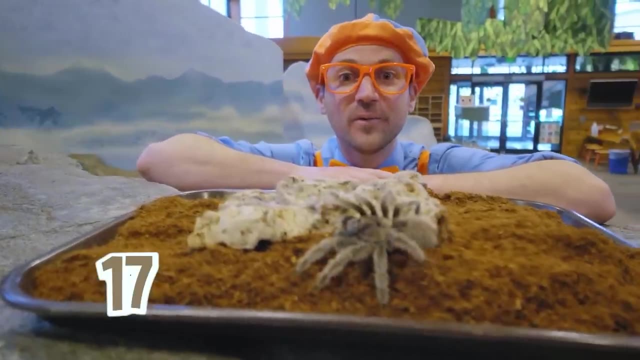 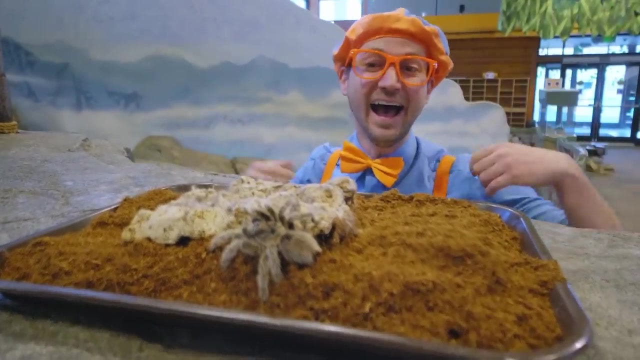 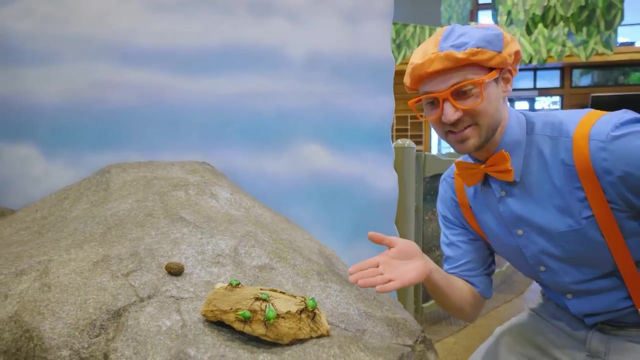 it looks really hairy. Look at her. Oh yeah, This is actually a female Whoa and she is about 17 years old. Wow, what a cute little insect. Well, not little, so big Whoa. what are these? These are flamboyant flower beetles, Wow. 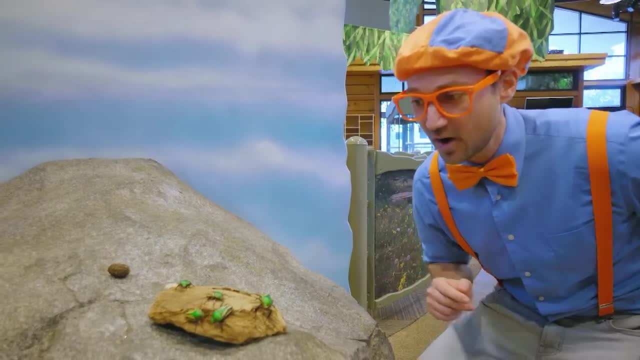 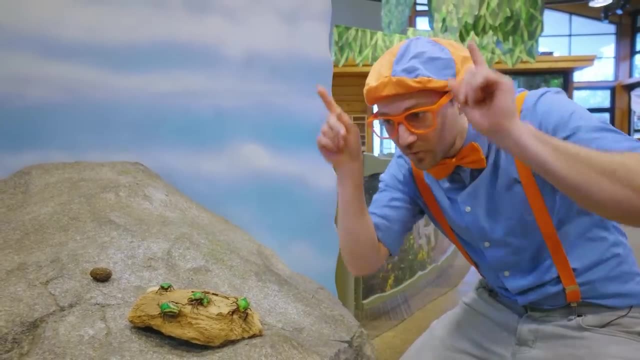 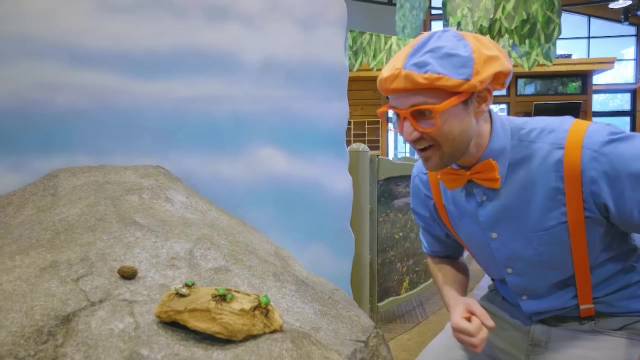 and they're so shiny. Yeah, the two colors that I see on them are green and yellow. Oh, and they're little horns, the males? Yeah, they have horns. It looks like it's the color red orangish. Whoa, they're just hanging out on this log. They love to eat fallen fruit. 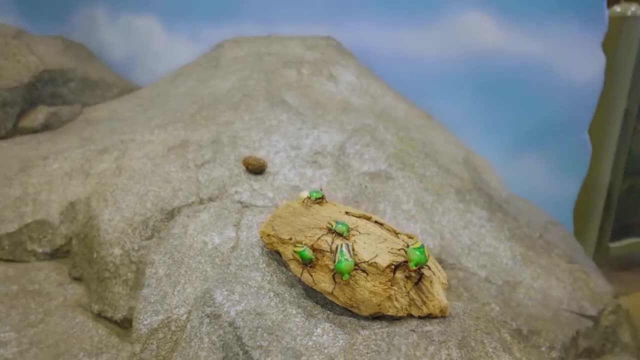 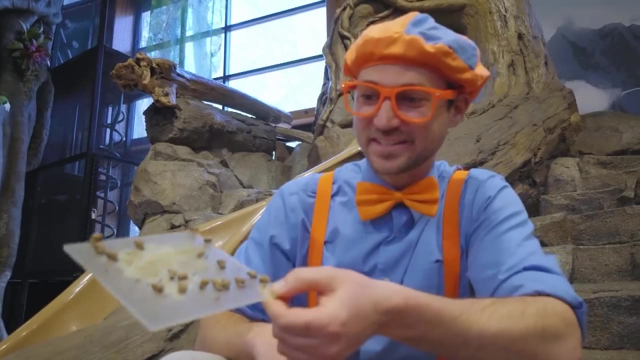 Yum, I love fruit too. Wow, check it out. I have some crustaceans on this piece of plexiglass. These are perchula snails. Wow, they have great teeth. Wow, Yeah, they're really rocky. Whoa, look at that. This one has. 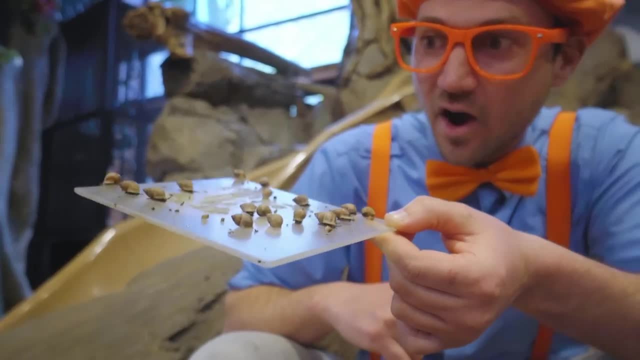 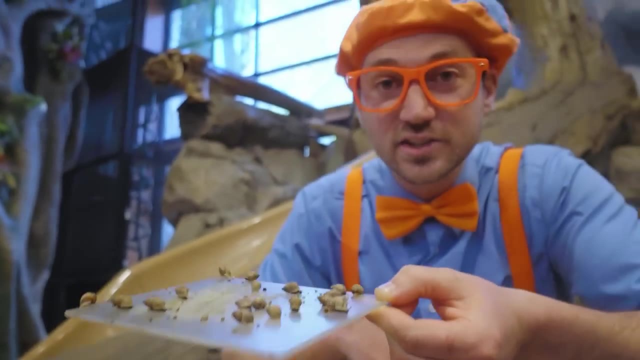 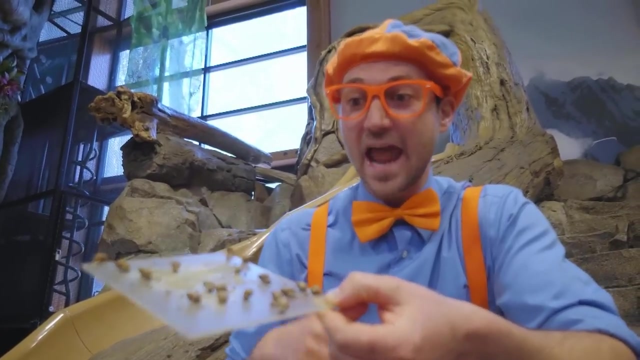 They are so cute. Do you see how they have little hard shells? Yeah, that helps protect them. Well, they're from the location of Tahiti. Wow, I love Tahiti. It's so sunny and beautiful there. Well, actually, there's none of these left in the wild. 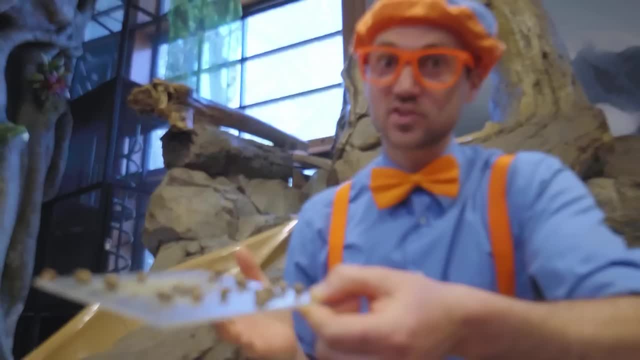 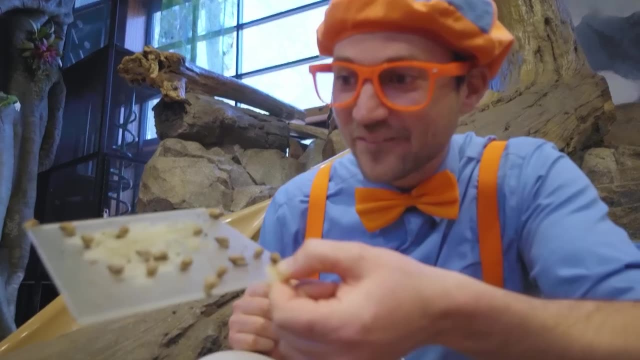 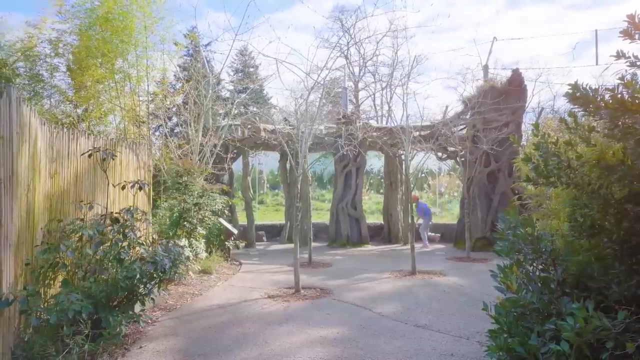 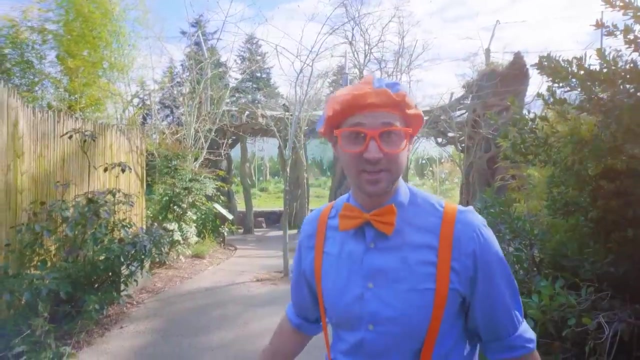 They're only in zoos captivity and we're actually trying to put them back out into their normal habitats. For now, we can just observe them and watch them eat their food. Hello, Wasn't that fun learning about animals today at Woodland Park Zoo in Seattle Washington. 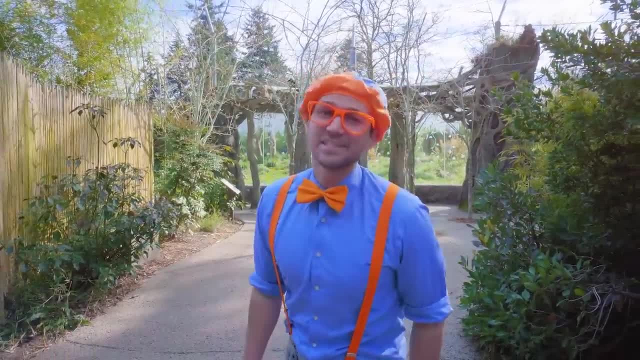 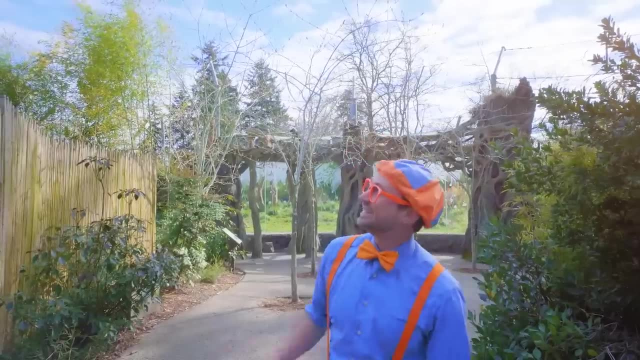 Yeah, it sure was. Well, this is the end of this video, but if you want to watch more of my videos, all you have to do is search for my name. Will you subscribe? Will you spell my name with me: B-L-I-P-P-I. 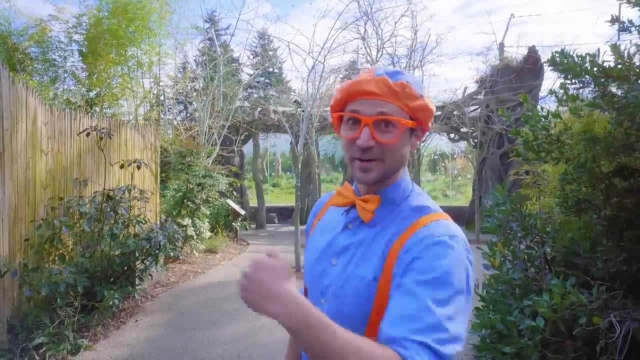 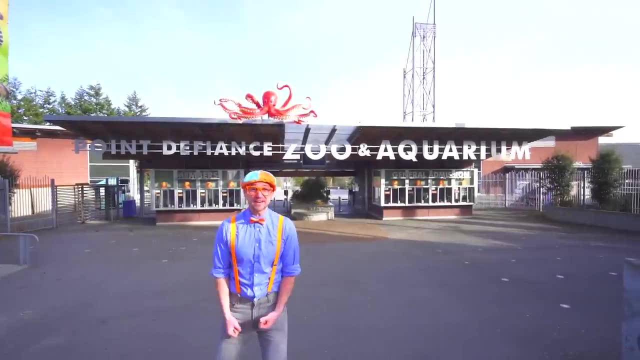 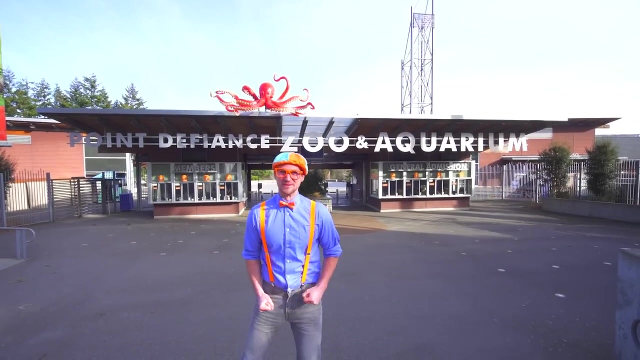 Blippi, Good job. Well, I'm going to go learn more about animals. Here I go. We are at Point Defiance Zoo and Aquarium in Tacoma, Washington, and today we are going to see some awesome animals. Let's go. 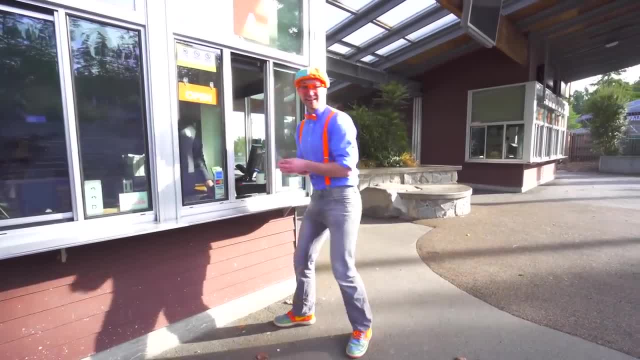 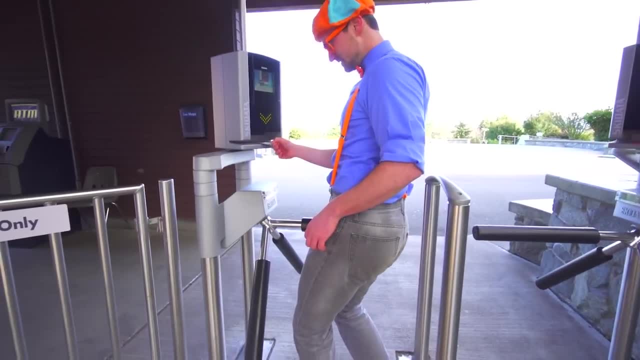 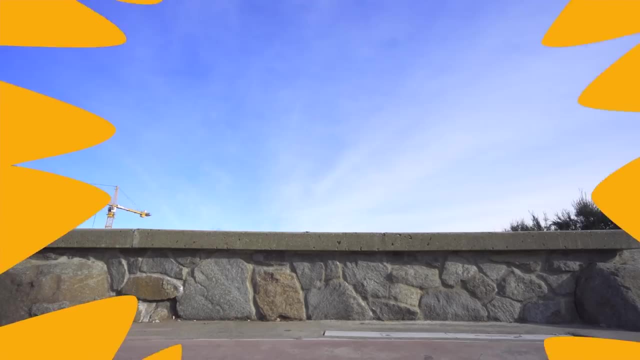 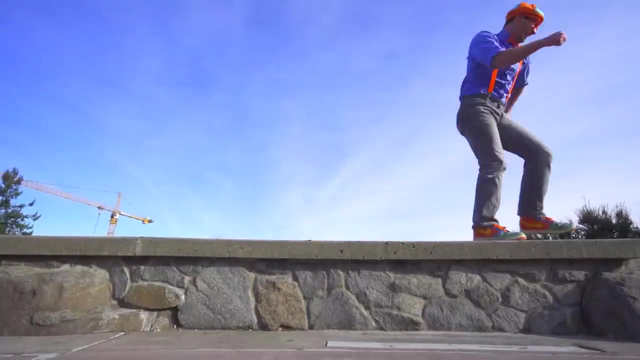 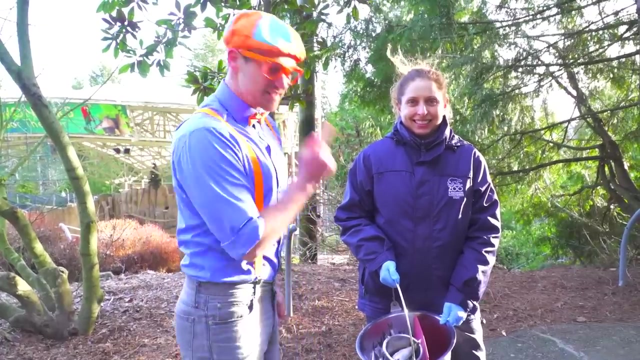 Got my members card, All right, OK, come on. This is going to be so much fun. Yay, Here we go. Hey, This is Cindy. And what do we have here, Cindy? That is a Pacific herring. 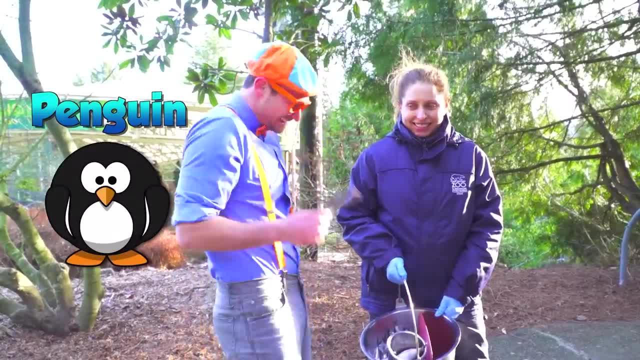 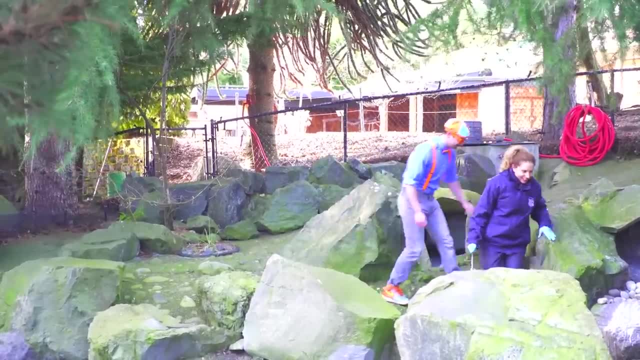 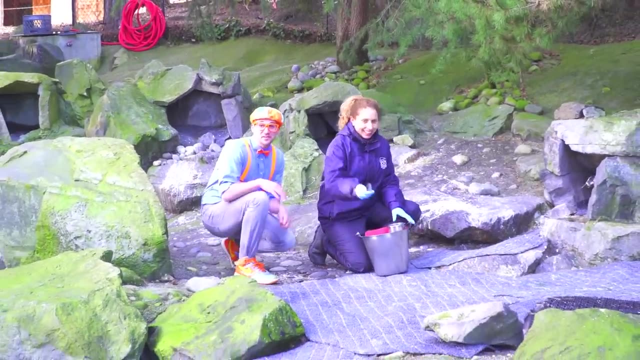 Ooh, and we are about to go feed some penguins. Mm-hmm, Woo-hoo. Did you see how we walked up really low? You've got to stay low, so then they don't get scared. Oh, Oh. 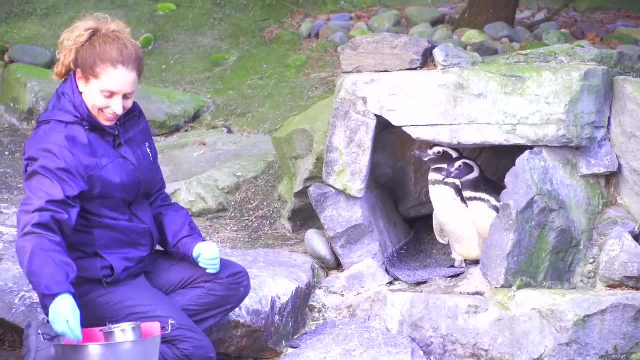 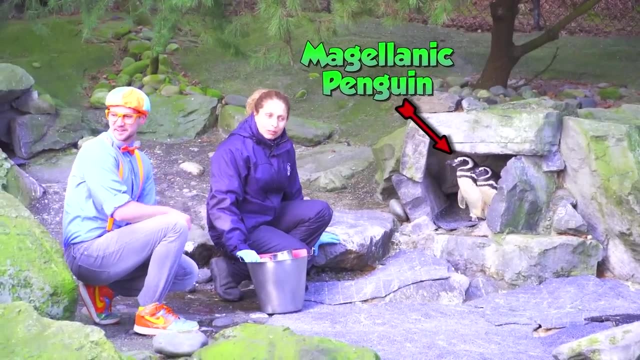 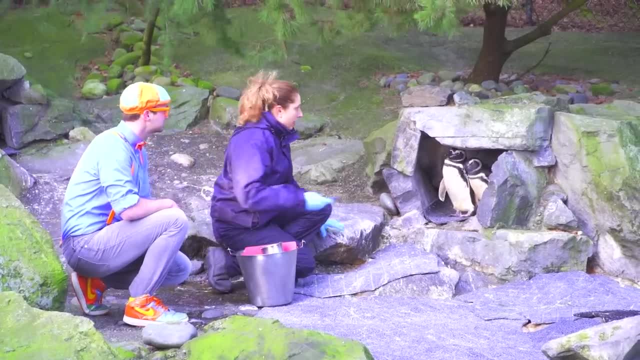 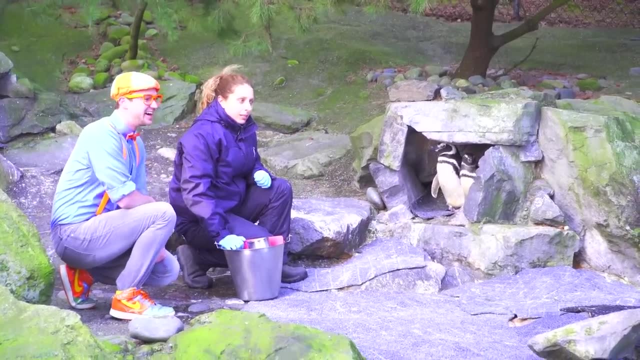 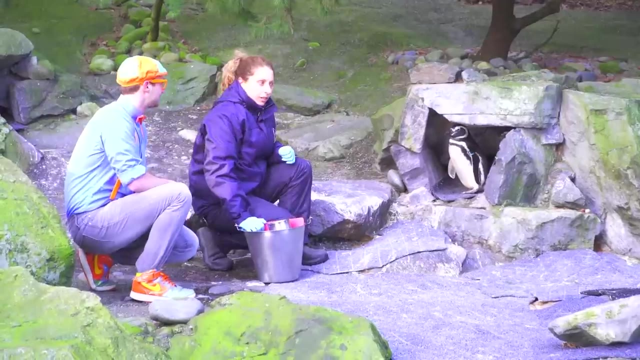 in an environment that is very similar to here- Ooh, Argentina and Chile. and so they love to swim. it looks like, huh, They do. These guys spend all winter out at sea and they can swim really fast. and they have to swim really fast so they can chase fish, which is what they eat in the ocean. 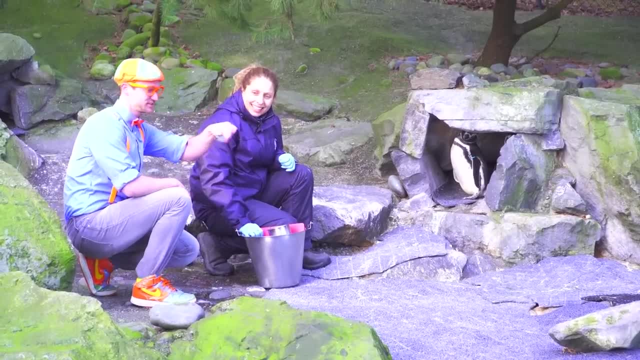 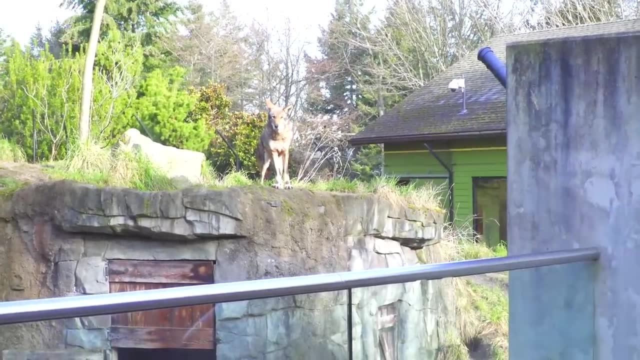 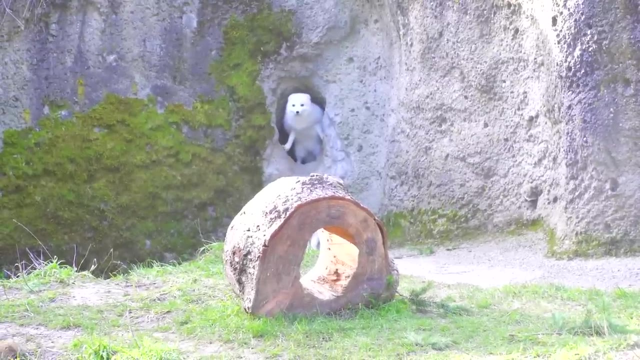 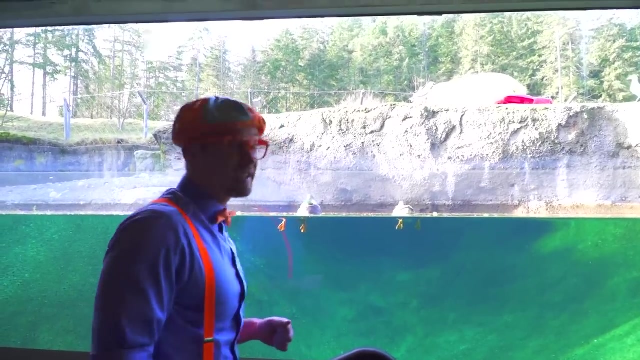 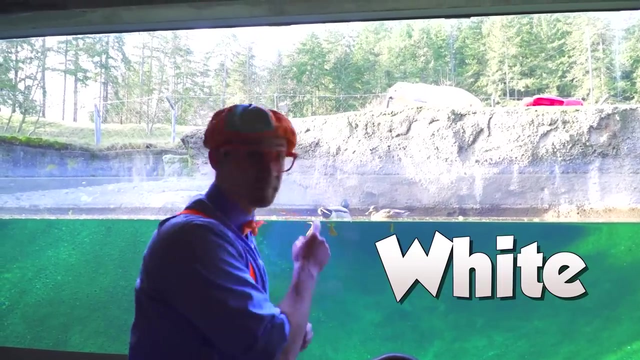 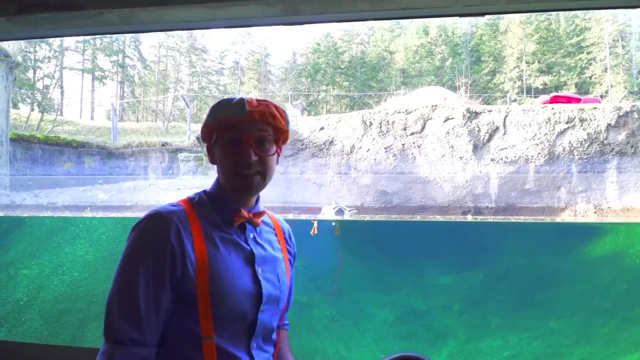 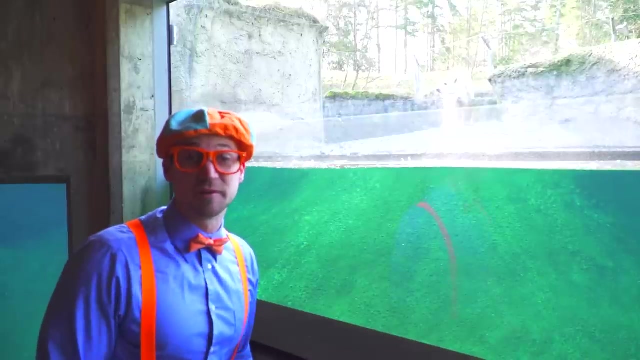 Ooh, like these Whoa. Look at what it is. It's a polar bear, And polar bears are the color white. That polar bear? Yeah, His name is Boris And he's 31 years old. Boris was rescued from a circus, a traveling circus in Mexico. 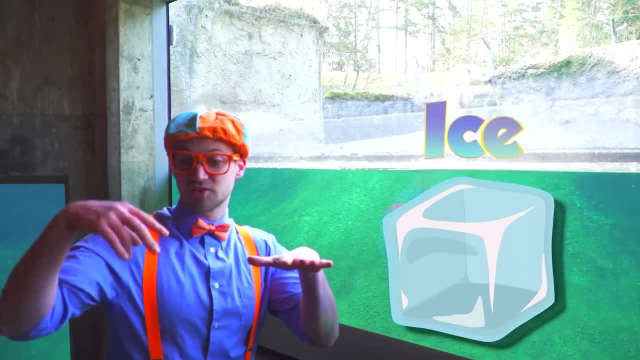 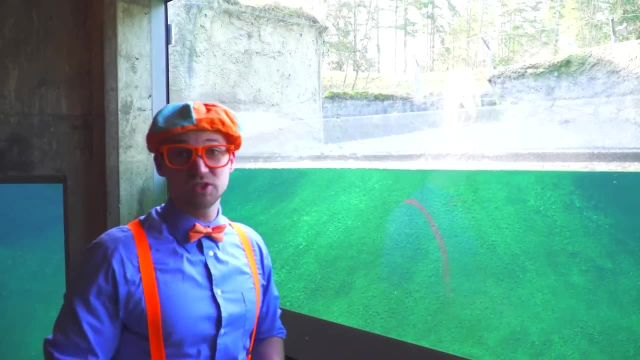 And it's really important to have ice so polar bears can hunt off of and get seals in the Arctic. So we should be really aware of what polar bears eat And what we do to our planet. so polar bears can have a lot of ice. 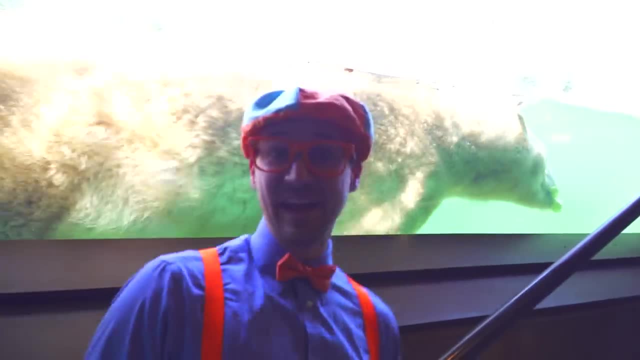 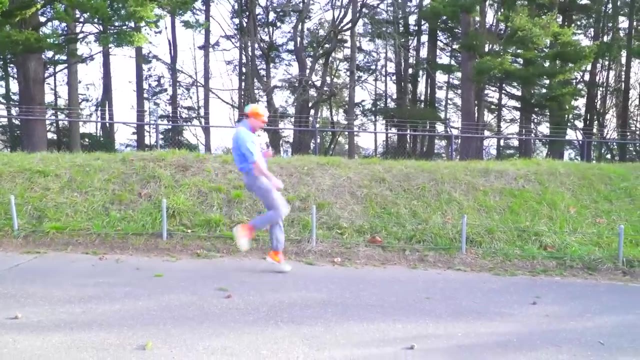 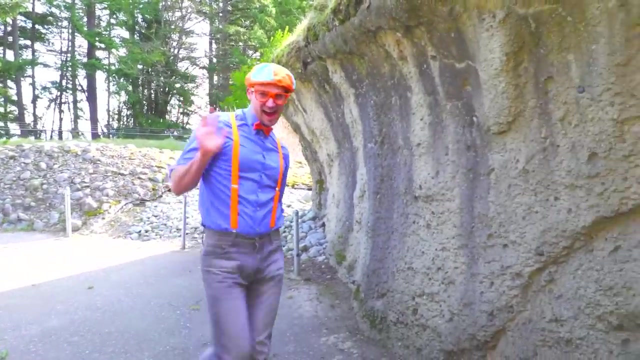 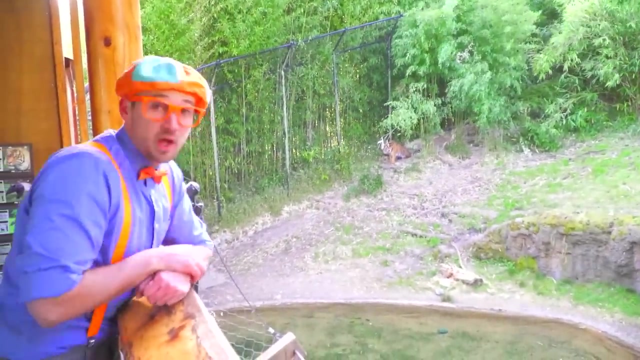 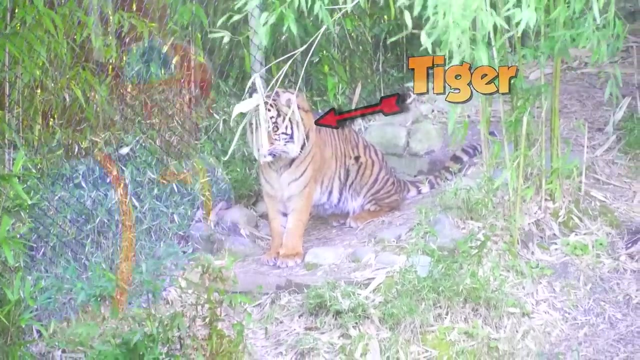 Whoa, Boris is so pretty. Wow, Whoa, It's a tiger. Whoa, Do you see what that is? Yeah, That's a tiger. Meow, That's a really big kitty cat. That's actually a Sumatran tiger, to be exact. 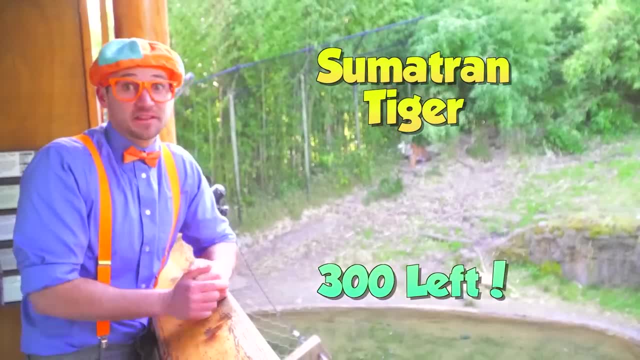 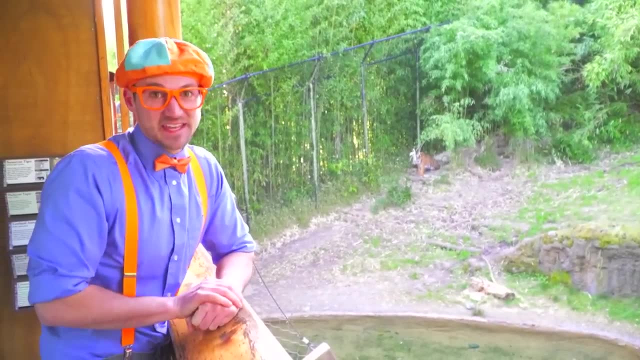 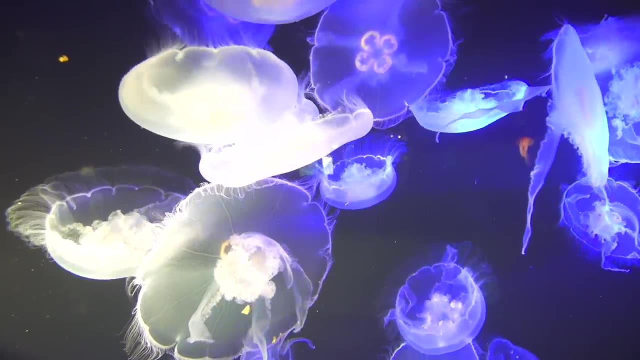 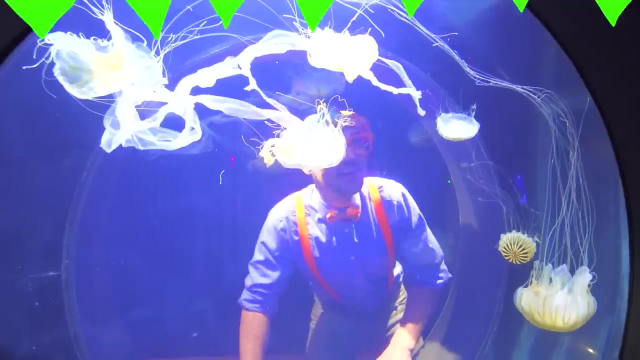 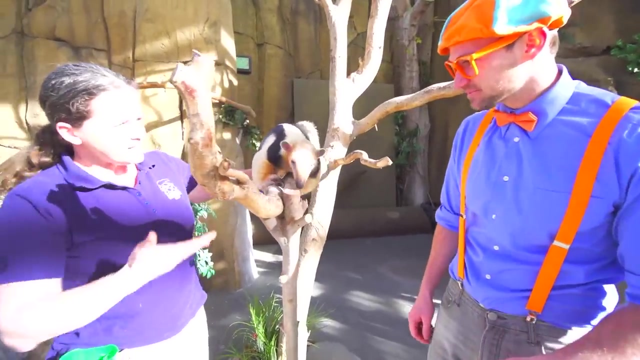 And there's only about 300 left on this entire planet in the wild. So here at Point Defiance Zoo and Aquarium, this tiger is an ambassador. So this is Sarah. Hi And Sarah. what do we have here? This is Gonzo, and he is a tree-climbing ant eater. 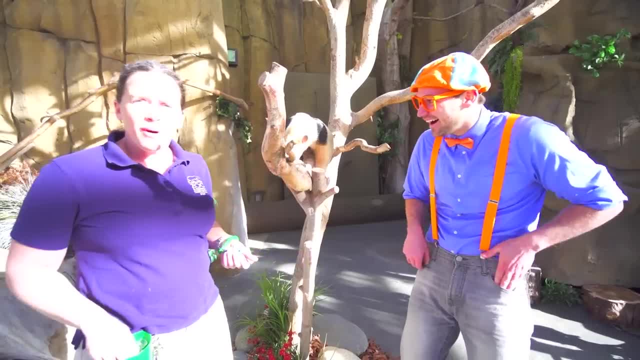 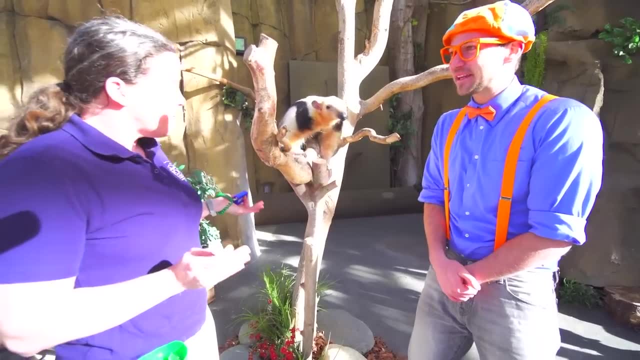 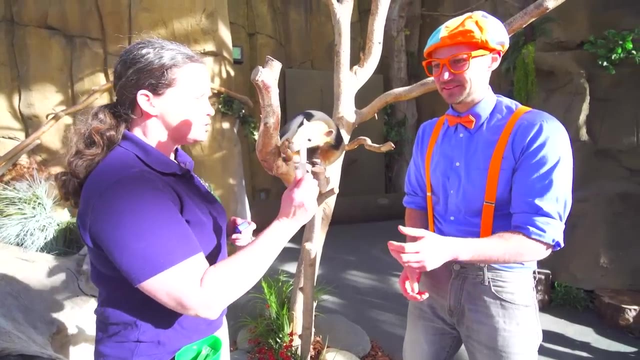 And here at Point Defiance Zoo and Aquarium, we're training him to be part of our Wild Wonders outdoor theater show. That's brand new this summer. Hey, Gonzo, What are we going to be doing right now? You're going to help me train Gonzo to eat vanilla yogurt from a tube. 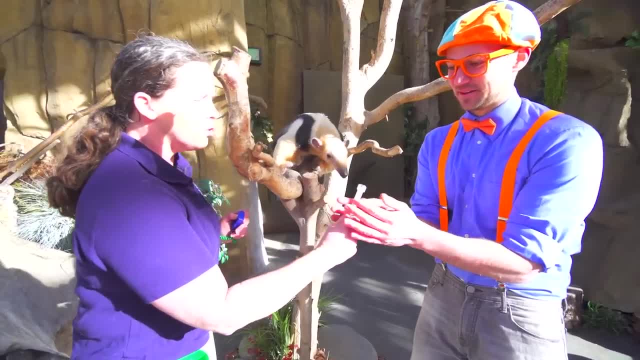 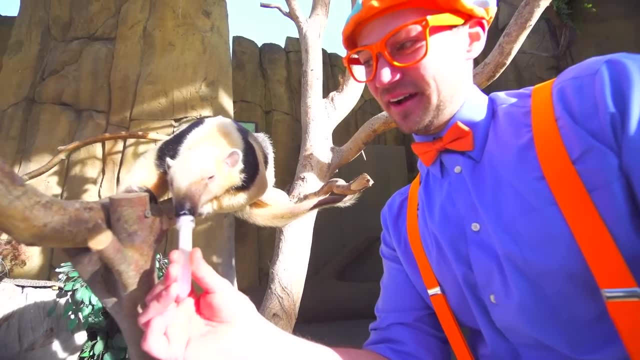 So this is something that he will love to do. Hold that right up to his little nose And he's going to slurp that vanilla yogurt right out with his super long tongue. Whoa, Check that out. Look at Gonzo's tongue. It's so long. 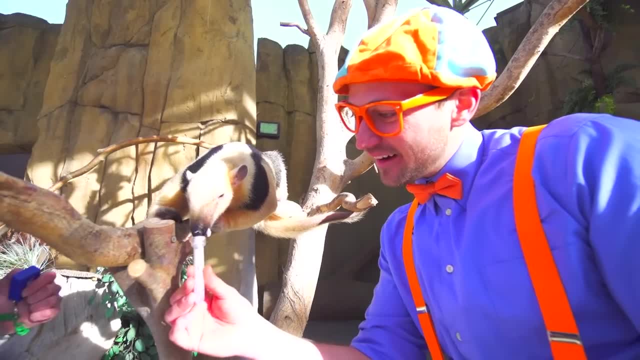 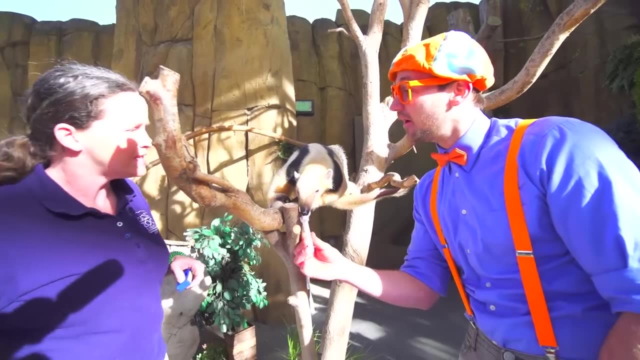 Now, of course, in the wild Gonzo would not eat vanilla yogurt, He would eat ants, And he has really big claws that he can use to break open ants' nests and termite bounds, And then he'd use his long tongue to slurp those bugs right up. 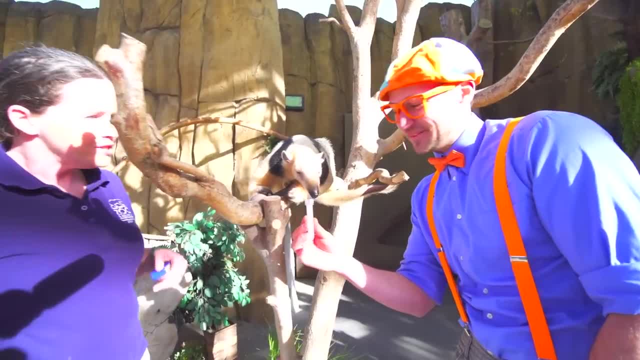 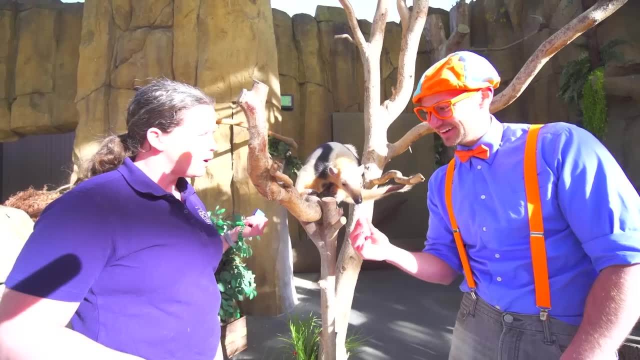 Ooh yum, That looks pretty tasty, Yeah. So Gonzo has been around people his whole entire life, And when he first came here, we started training him to be part of the show, So that's why he's so comfortable hanging out with us out here. 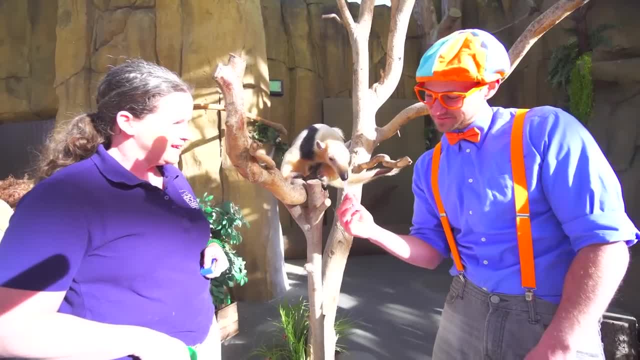 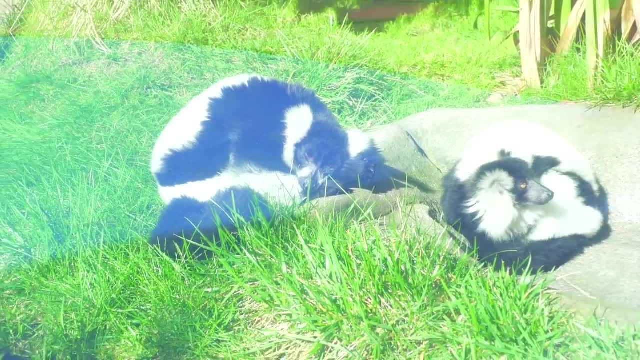 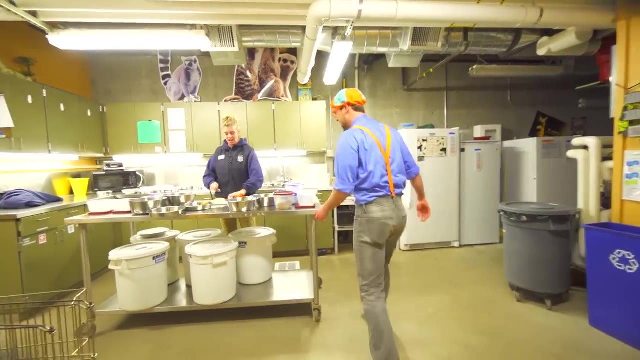 Yeah, He seems like a really great and fun anteater. How's it going? Oh, pretty good. What are you doing? I'm making some diets for the meerkats, Meerkats. I love meerkats. What else are you going to do today? 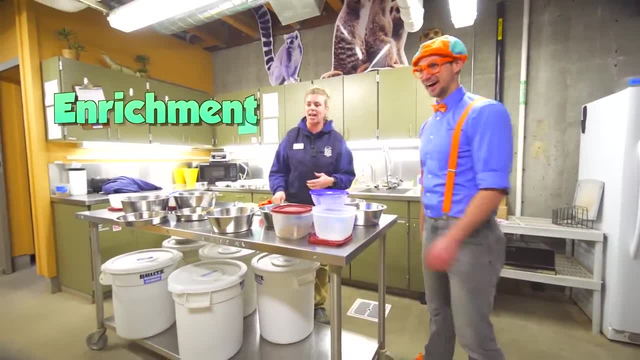 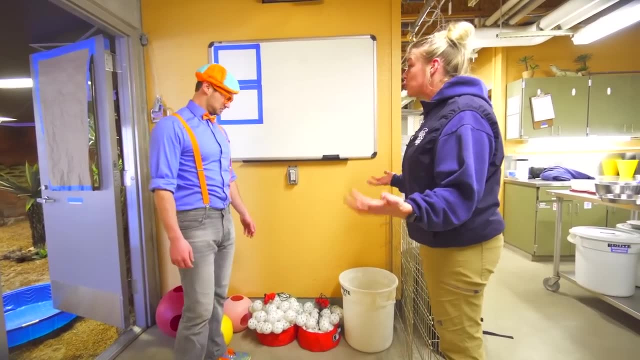 Well, you know what I was going to do: some enrichment. Do you want to help me? Yeah, Excellent, Let's go over to the exhibit. Okay, Okay, And what's enrichment? Enrichment is giving our animals choices. 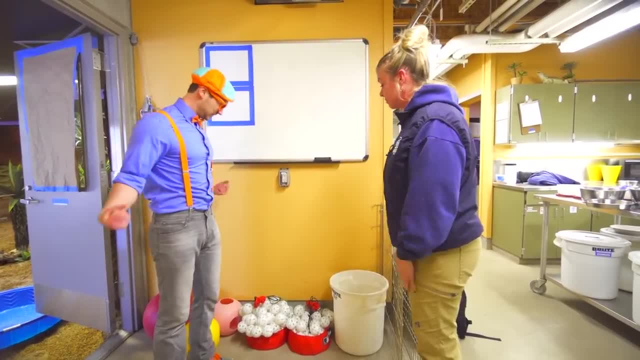 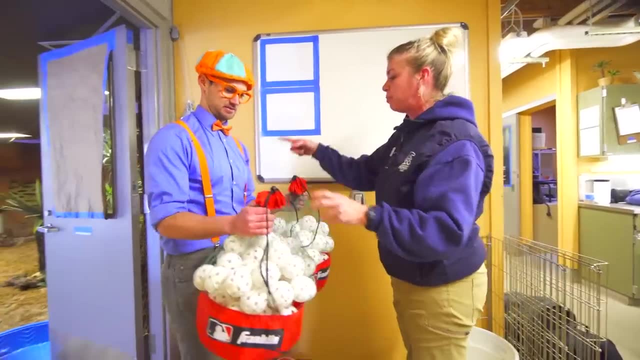 Things to do, things to play with, Kind of like kids on a playground. Ooh, that sounds fun. I like playing, So let's give them some choices. Okay, Let's put these wiffle balls and the blue pool on exhibit. 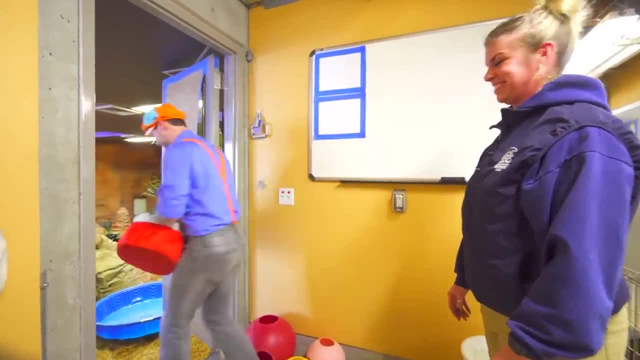 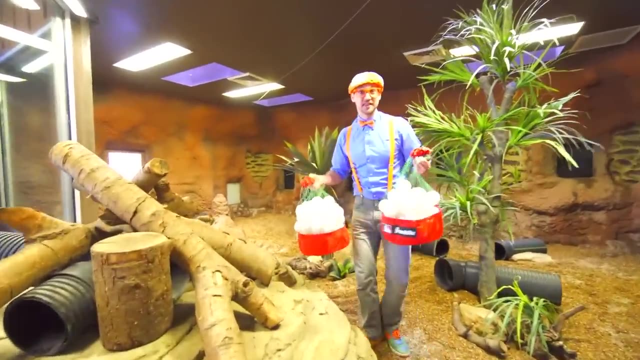 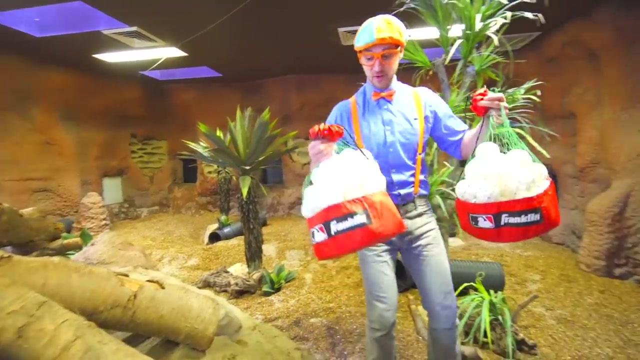 Okay, All right. Wiffle balls, blue pool- Got it? Whoa. Look at this place. This is the exhibit from the habitat of where meerkats play. Whoa. Okay, Anyhow, back to it. Wiffle balls, blue pool- Right. 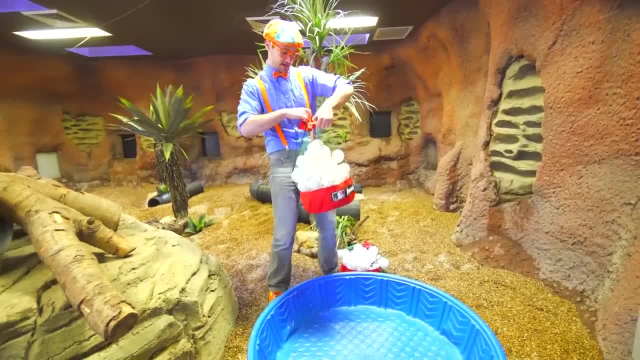 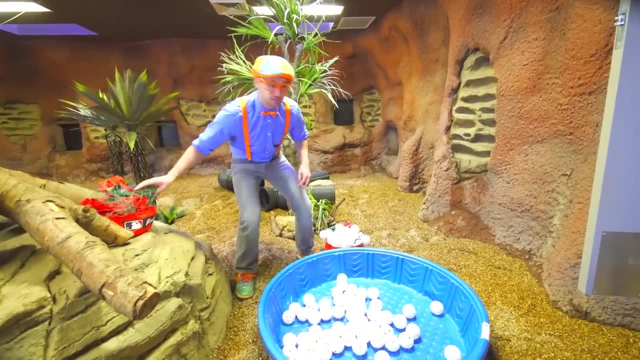 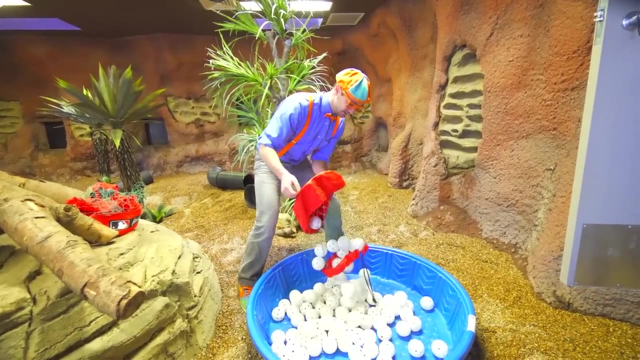 Okay, Let's put these in here. This is going to be so much fun to see the meerkats play with these wiffle balls that we're putting in here. Okay, And the second one. Wow, Okay, Here we go. 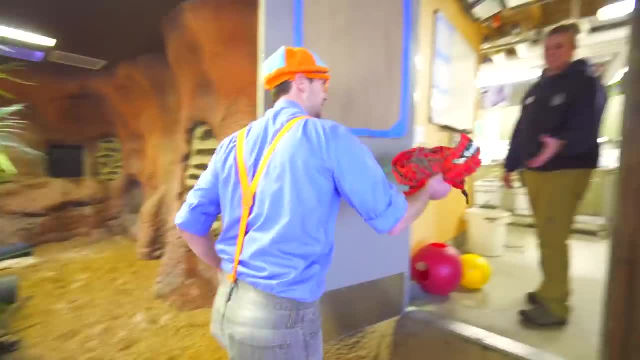 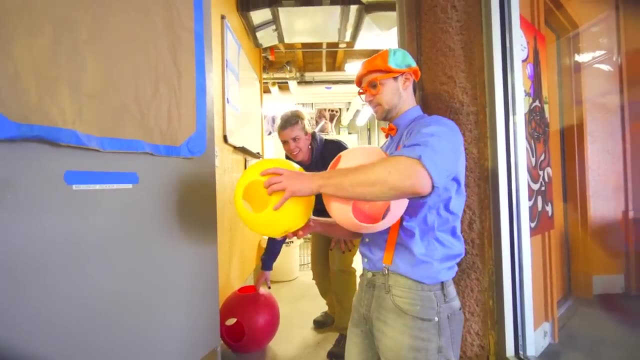 Let's see what else she wants us to do. Okay, Here you go. Thank you. What else do you have for us? Well, I've got some more fun toys. Let's put these out on the exhibit as well. Okay, Where should I put these? 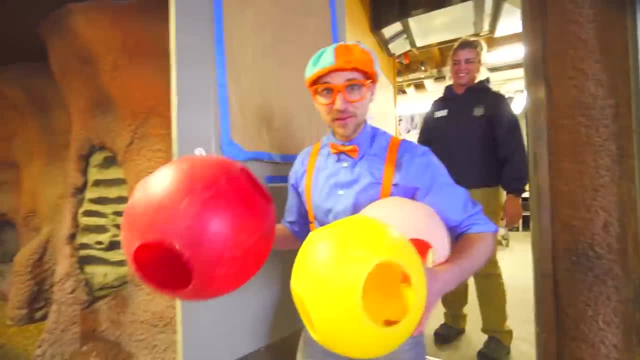 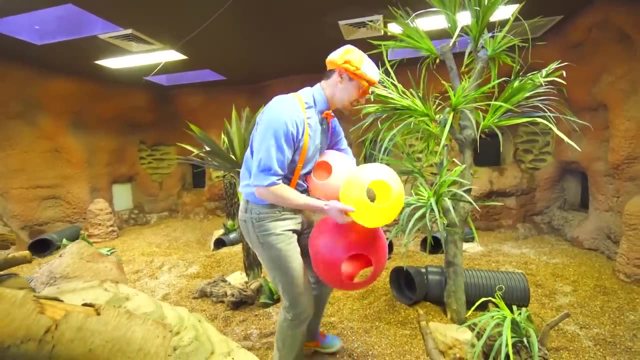 Wherever you want. Ooh, this is going to be fun. Where should we put these Here? come on, Okay, Let's see. Oh, let's see. I think the yellow one should go. Oh, do you see this? 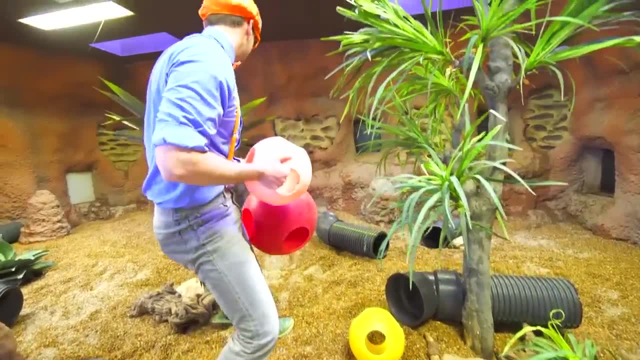 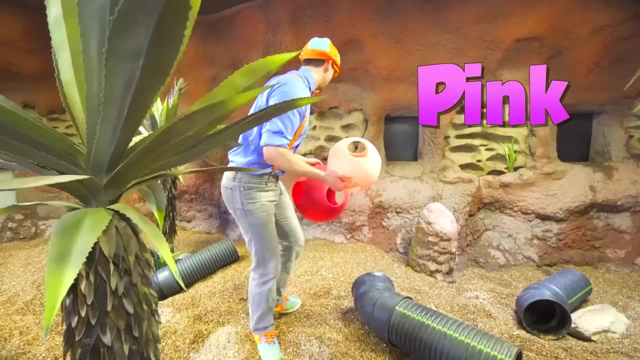 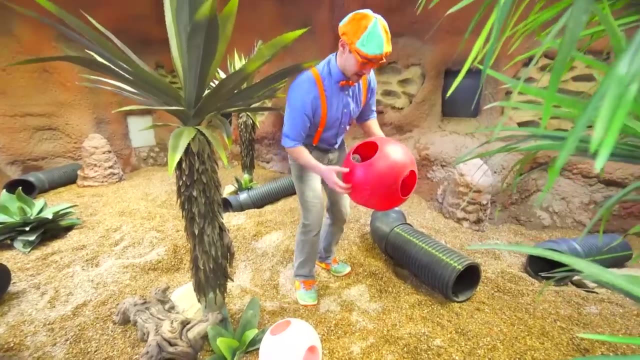 Let's put it right there. And then, ooh, come back here. Let's put the pink one right. Let's do this one right here, actually Right next to the yellow one, And the really big red one let's put over here. 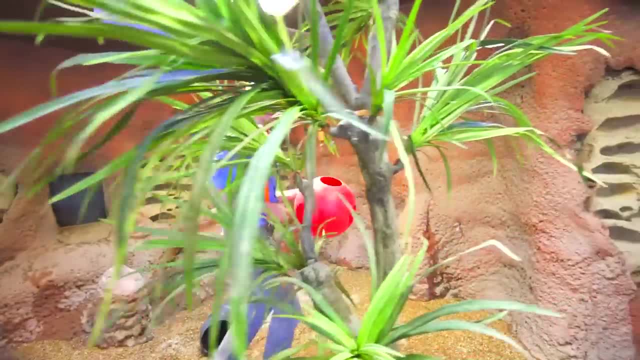 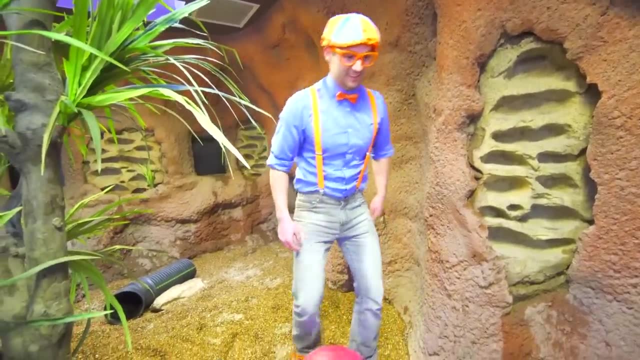 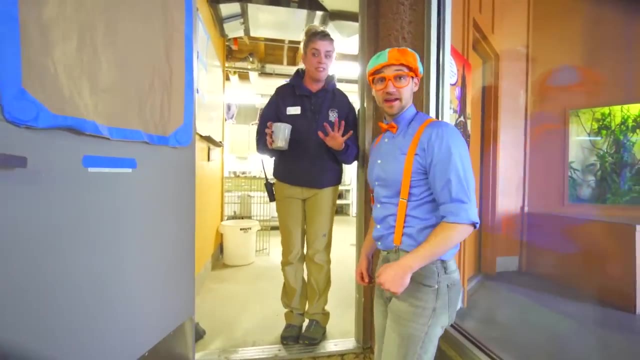 Here, I'll meet you over. that way It's like I'm a meerkat Watch. Okay, let's see what else we need to do. Come on, Okay, is that all? No Blippi, Let's take the fun up a notch. 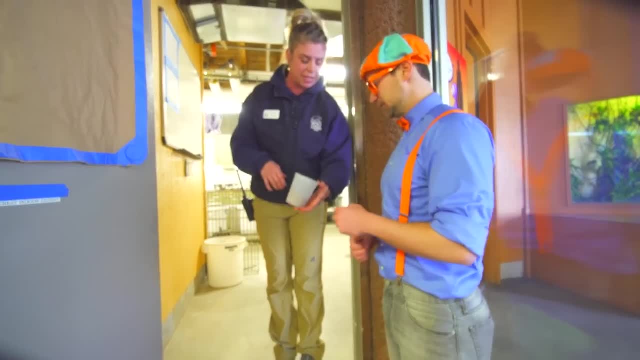 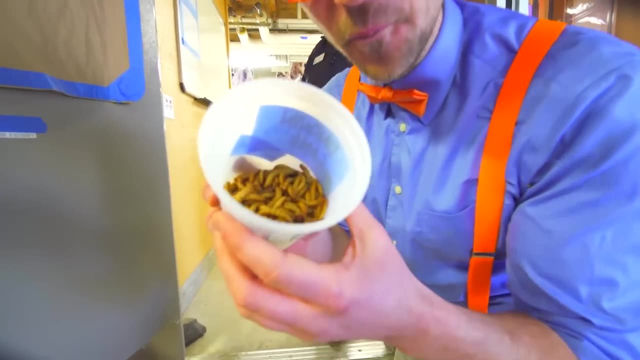 Let's add some food enrichment to the toy enrichment. Here's some mealworms. It's like chocolate for meerkats- Ooh yum. Look at this. Ooh yum. So where would you like me to put this? 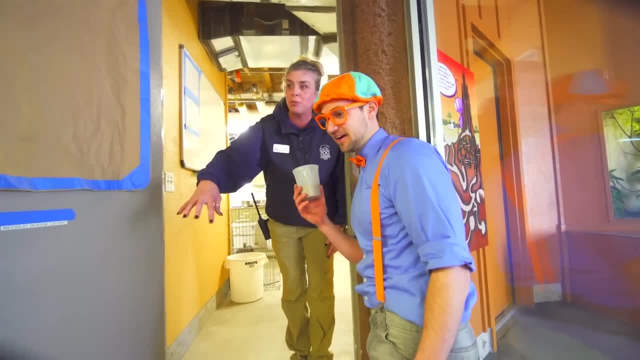 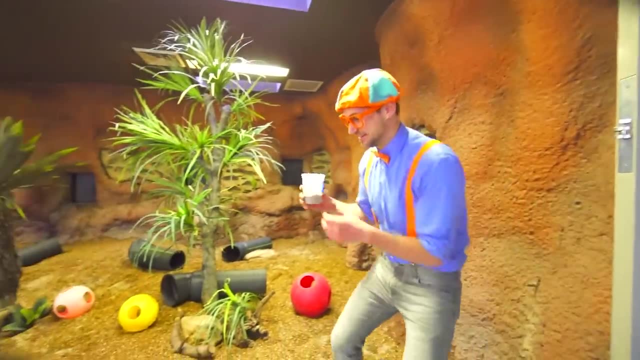 You know what? Let's sprinkle some in the wiffle balls, And if you want to put some elsewhere in the exhibit, you can do that too. Okay, It's kind of like a search and find, Because we'll put some right here. 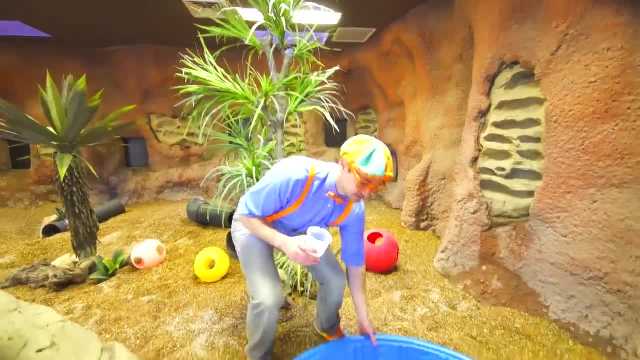 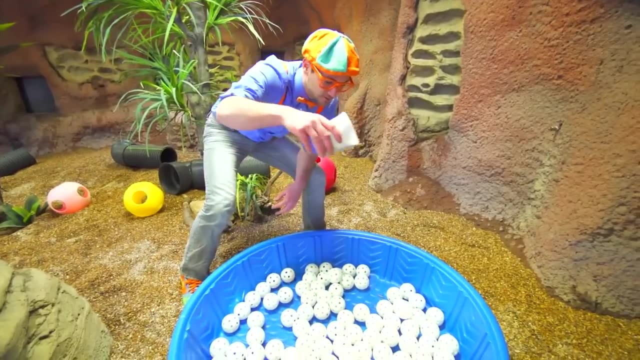 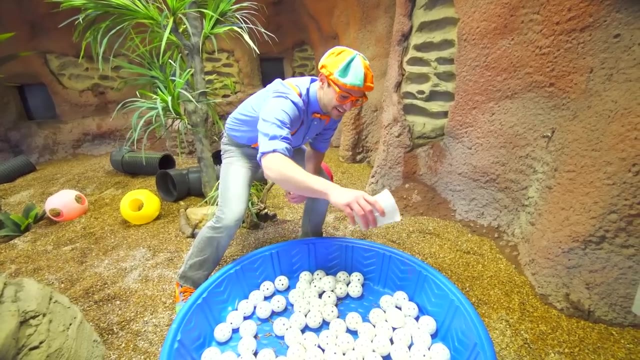 and then we'll hide some for them to find it. Okay, Spread out the wiffle balls And let's sprinkle some on top of the wiffle balls. Wee Ooh, this is going to be fun, Okay. 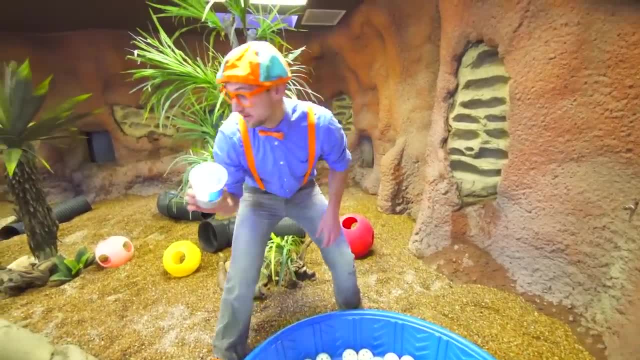 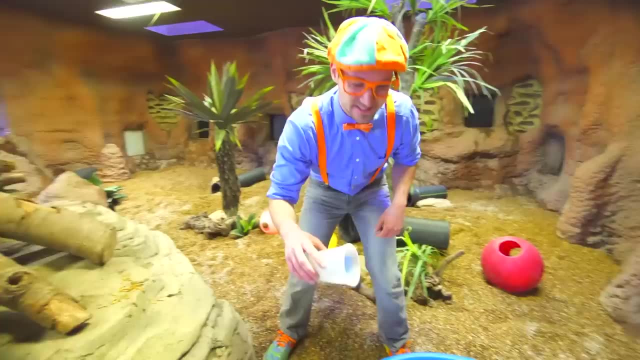 Okay. Okay, there's a little bit more. Let's put some right on this ledge. Mmm, those look tasty. Okay, let's just put the rest in here. All right, I think we're ready. Are we all done? 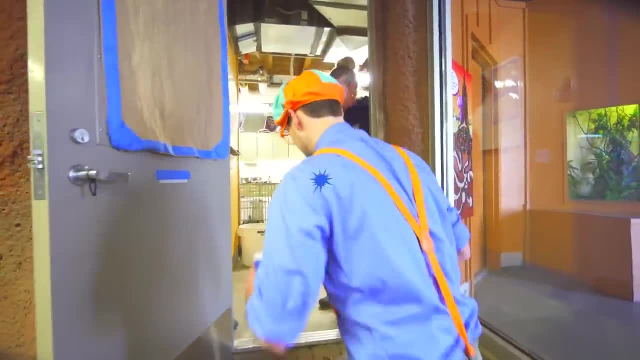 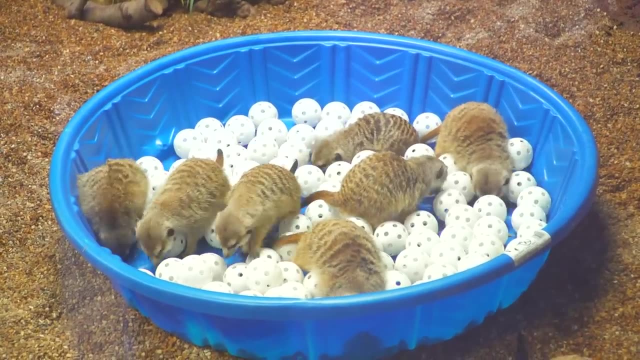 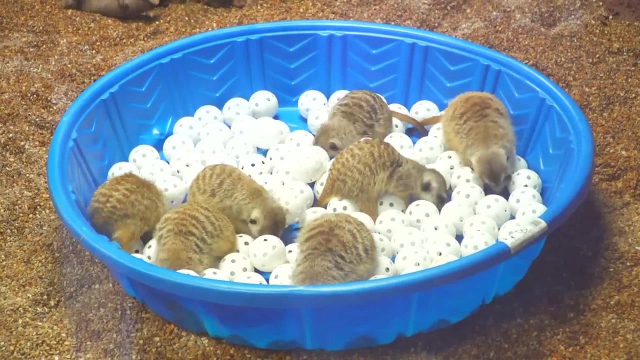 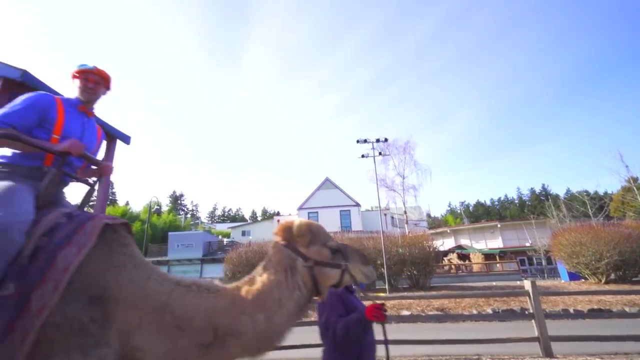 Great job, Blippi, Let's let them out. Okay, Let's go, All right. All right, I think we're ready to go. Let's go All right, Let's go. Let's go All right. Whoa, we're done. 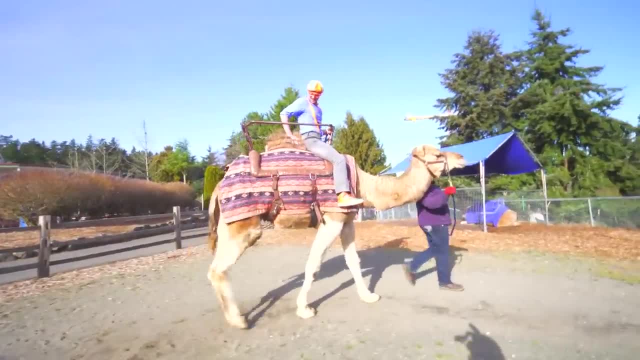 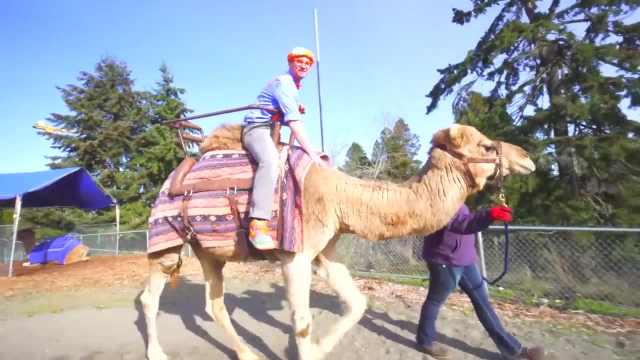 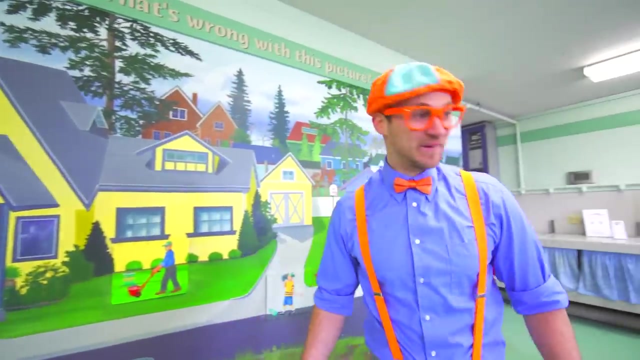 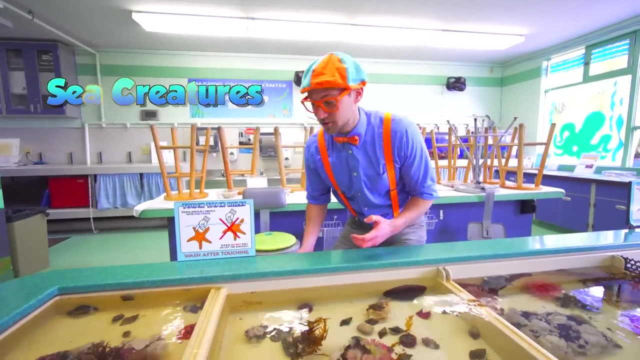 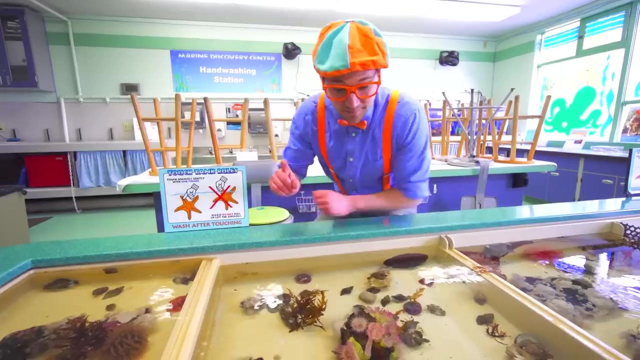 Bye-bye, Bye, Bye. Wow, we are in the Marine Discovery Center And this place has amazing sea creatures and we can actually touch them. See, You can touch, but with only one finger, okay. 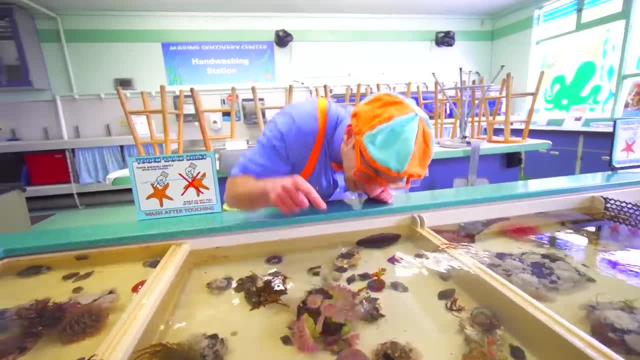 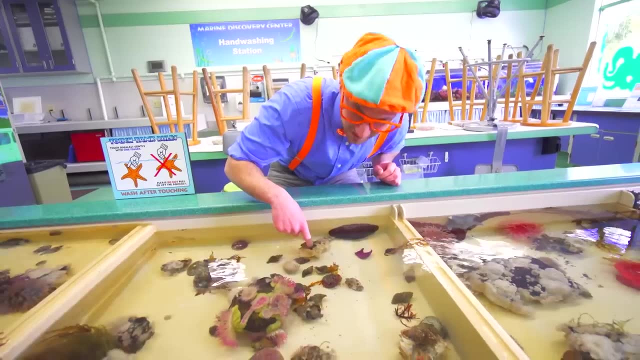 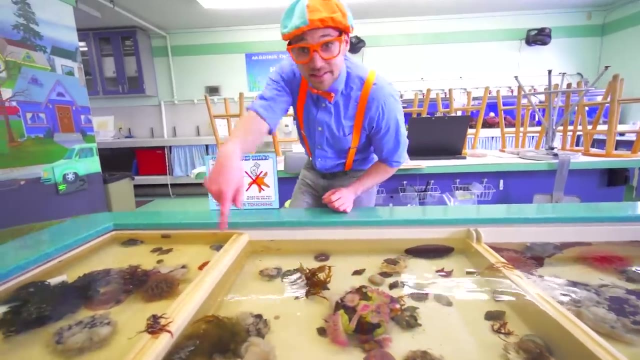 Oh, look at these right here. Oh, that was scary, That scared me. Oh, look, here's a snail. Hello Hi, little guy. Hey, little girl, Hello Whoa. Oh, look at this over here. 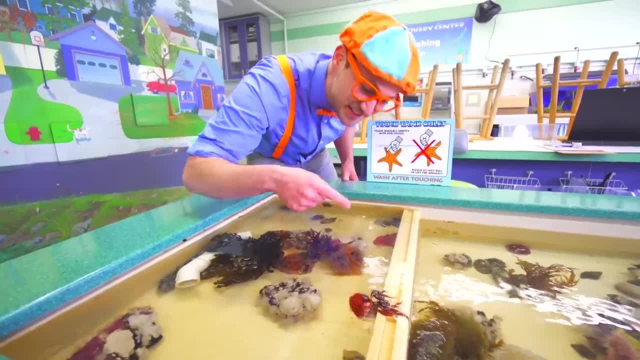 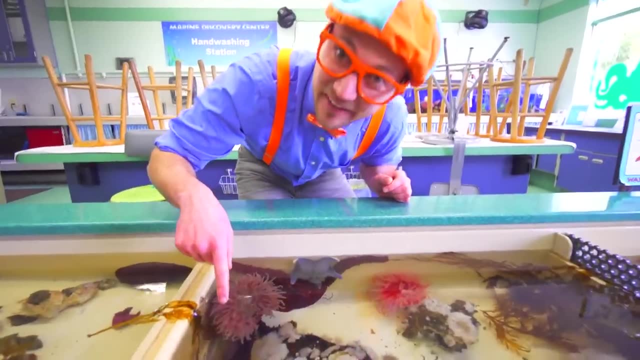 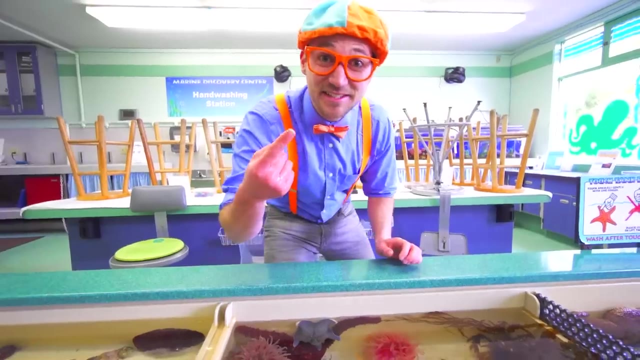 One finger. Oh, did you see it? The leg attached to my finger. Here, get a really good close. Oh, look at how big this one is. Okay, ready, Oh wee. Oh, it attaches to your finger and it's so soft. 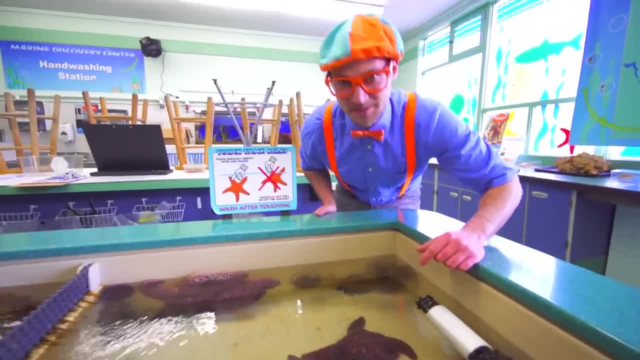 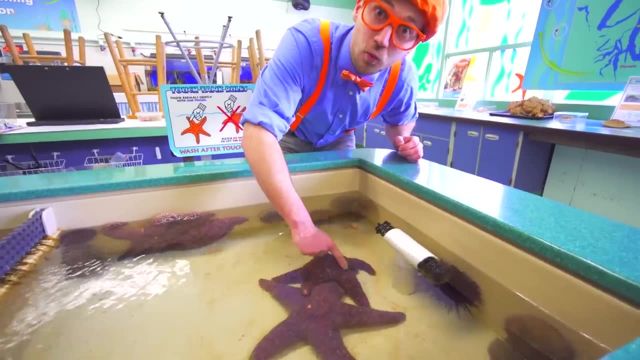 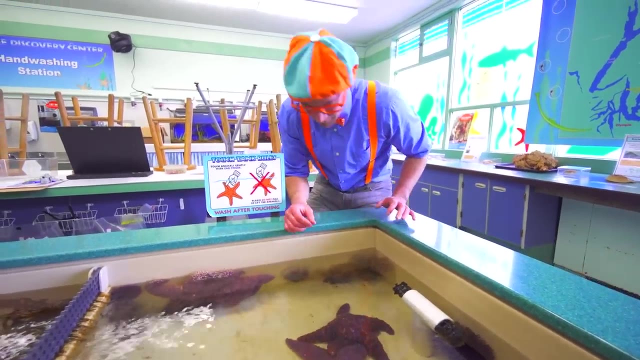 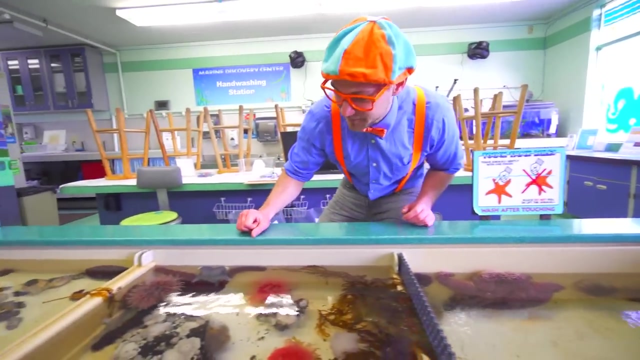 Oh, Last but not least, starfish: Whoa, Whoa. They're really hard. It's so cool And these are actually alive. They're real sea creatures. They don't move very much, but they do move Really slowly. 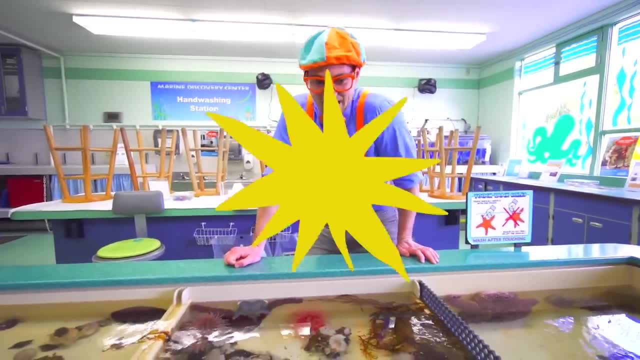 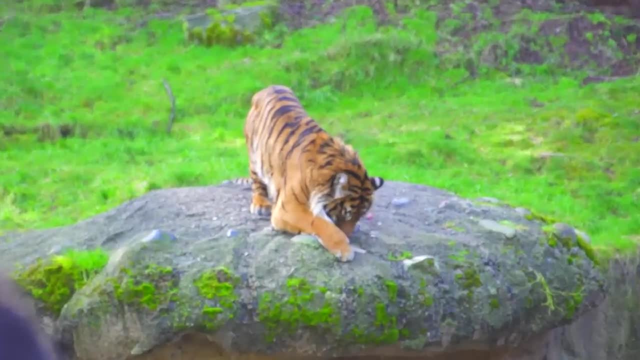 I really love the Marine Discovery Lab. I like this little school. I think it's going to really get to the point where we can by themselves. Oh, they're all in the same pool. I'll take you to the next one. Okay, we'll be right back. 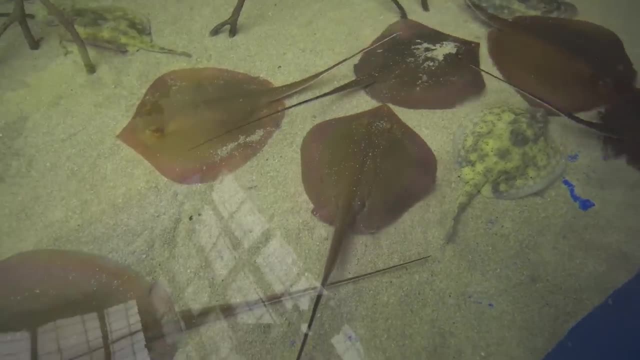 I'm not going to go to the next one. Oh, I think I'm going to go to the next one. I think I'm going to go to the next one. Oh, I think I'll go to the next one. I think I'll go to the next one. 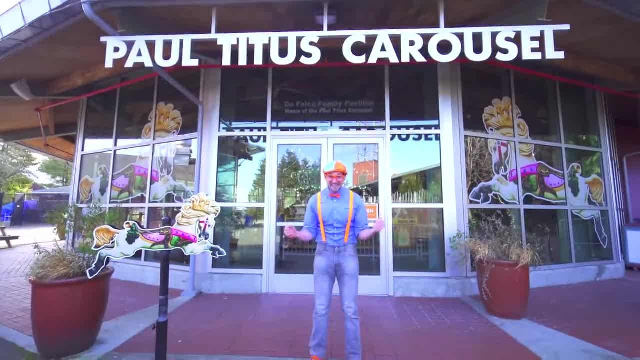 I'm going to go to the next one. You can see, Oh, look at that. Oh, look at that. That's a real native snail. You thot. you can see some of the Skittles, Oh look. 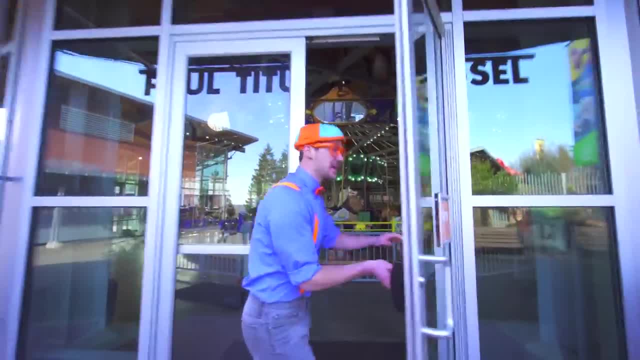 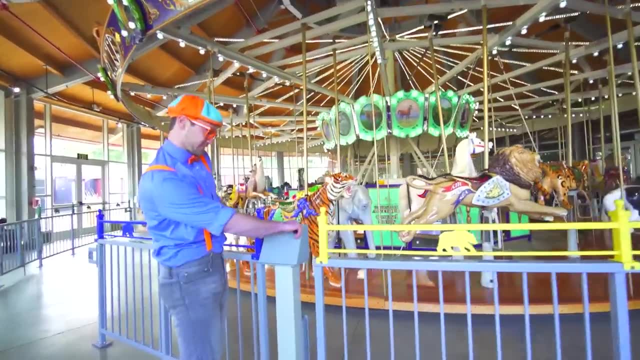 Crazy. That is some real native snail. That's the real name. This is going to be so much fun. See, it's a carousel, And right here this is the instrument panel that turns on the carousel. And I got the key. 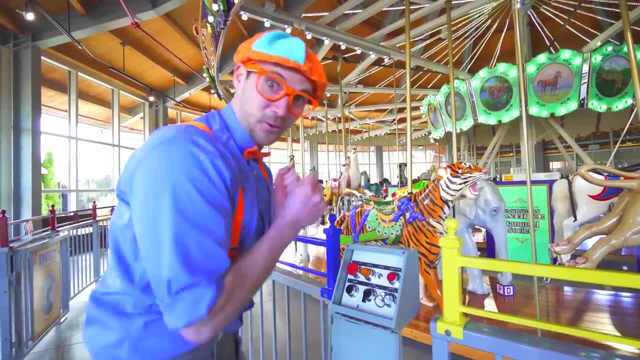 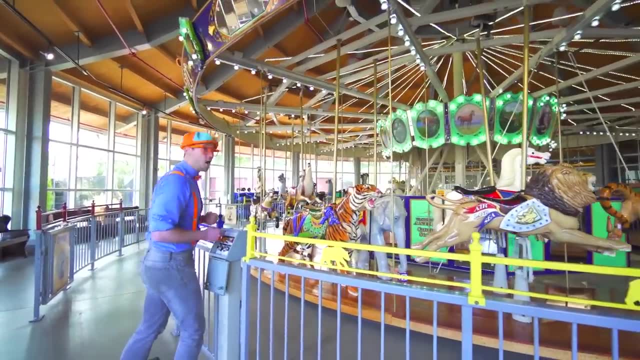 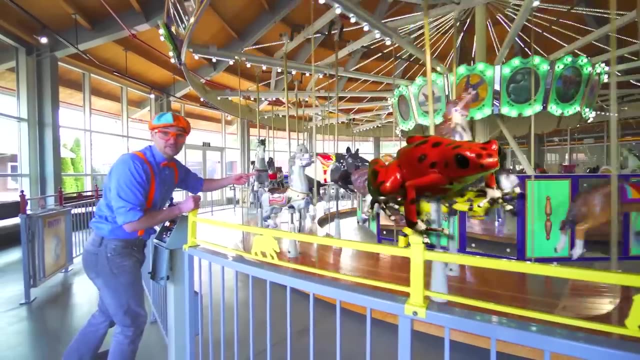 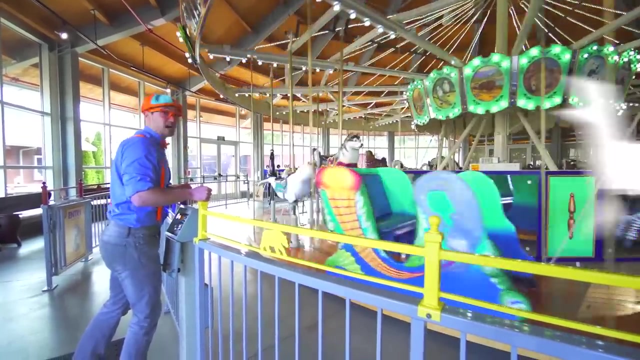 Okay, let's put in the key right there. And yeah, Whoa, look at all these animals. Yeah, a horse, A poison dart frog. Some more horses. Oh, a polar bear. We saw one of those today. A zebra- Did you see the zebra? 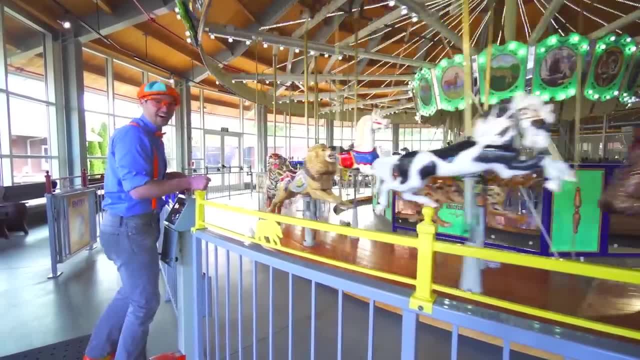 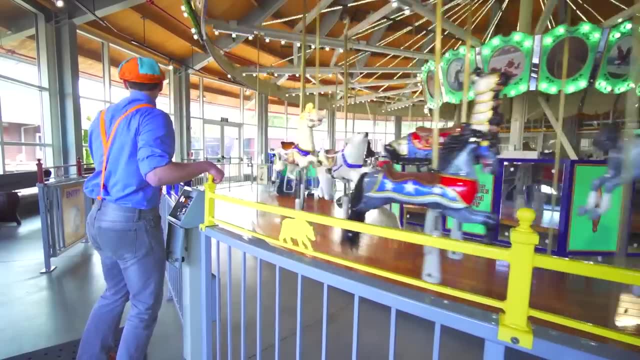 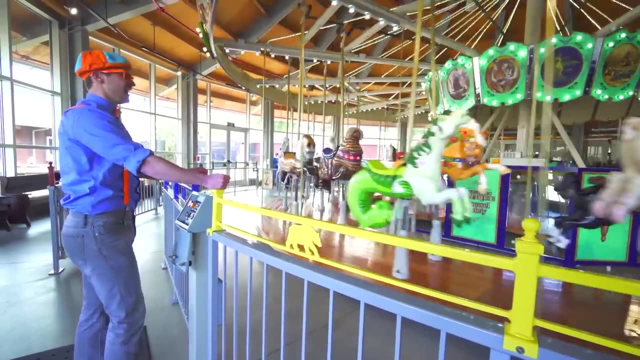 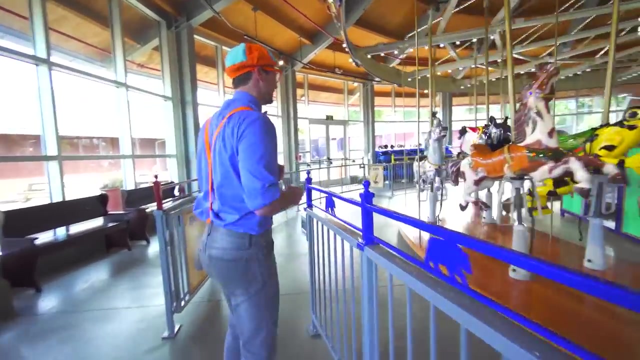 Oh a pig, Ooh tiger, Ooh an anteater. Okay, Okay. Now I think it's time for us To ride the carousel. Come on, But first we need to pick our favorite animal. We gotta wait for it to stop. 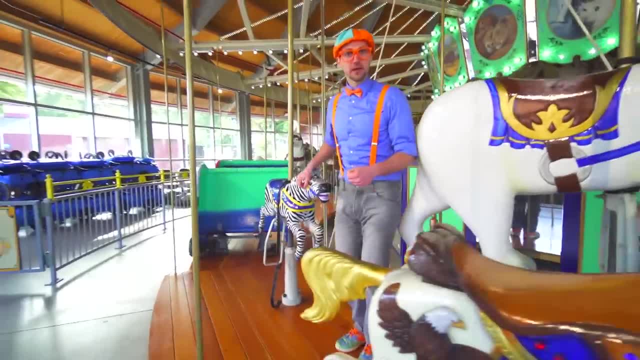 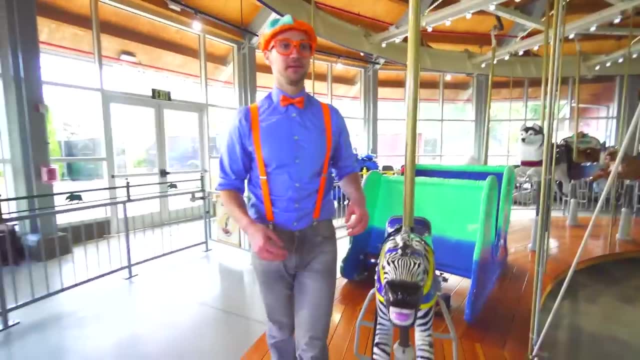 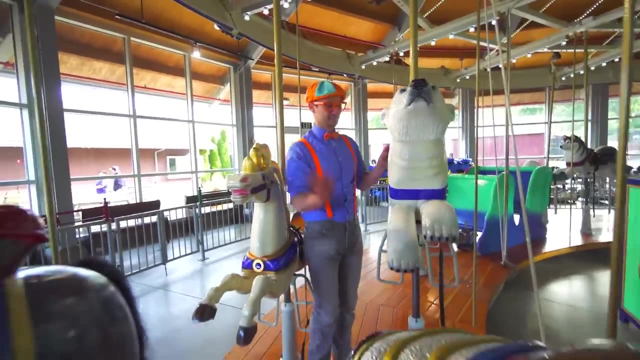 Come this way. Wait, The zebra. Hmm, I don't know if I want to ride the zebra. Let's see what else. A horse, A polar bear? Hey horse, Where'd the carousel go? Oh, I don't know. 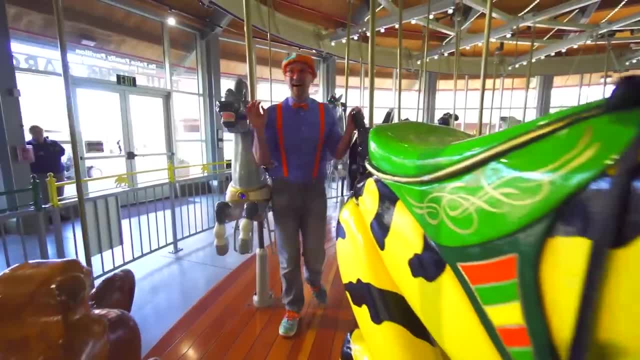 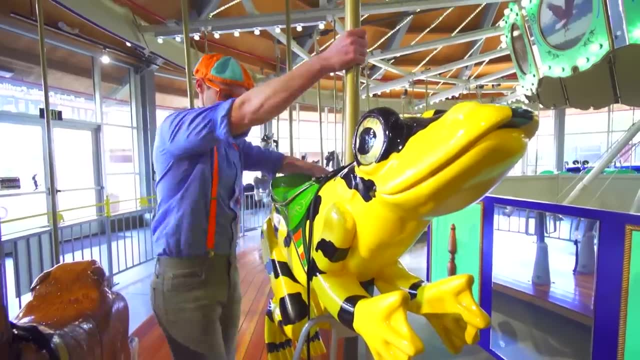 Look he's flying. I'm so excited. It looks like he's gonna get a chance to win. Yeah, He's so excited. Yeah, All right, here we go. All right. Okay, Look at that, You're gonna have to wait. 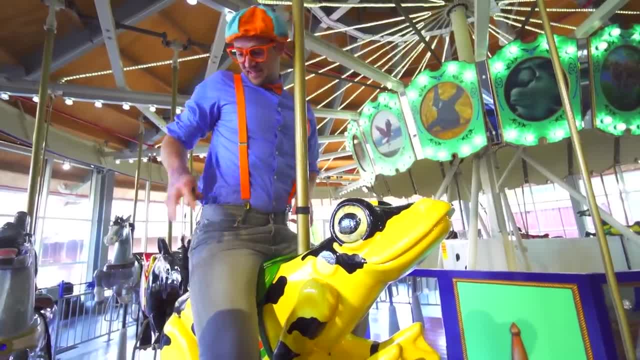 It's even more interesting than the last one. That's right, I'm gonna change the way these animals are brightened up. It's all got to be this way. Yeah, All right, And now I wanna do a sprint. Yeah.